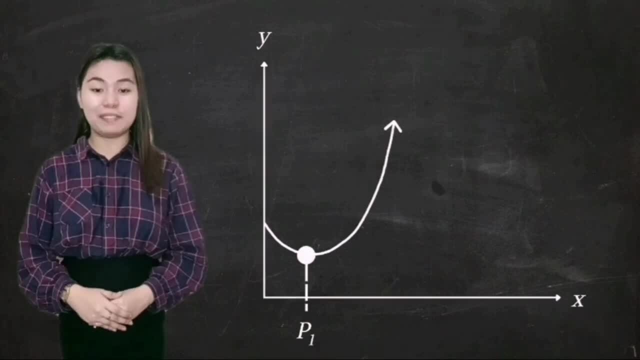 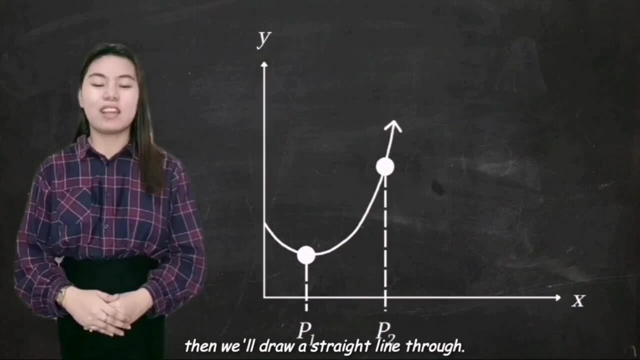 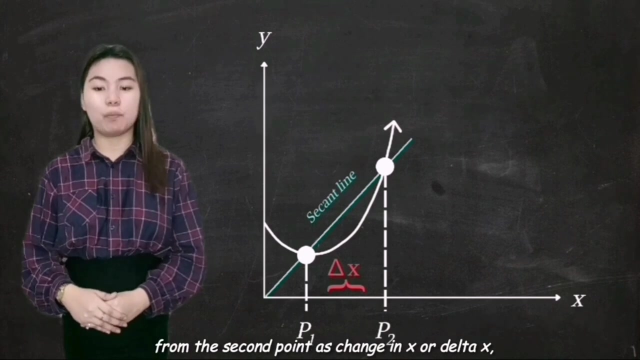 refer to as point 1 or P1,. we will use this graph with a curve at just a second point That we will call P2.. Then we'll draw a straight line through. Let us label the horizontal distance of the first point from the second point as change. 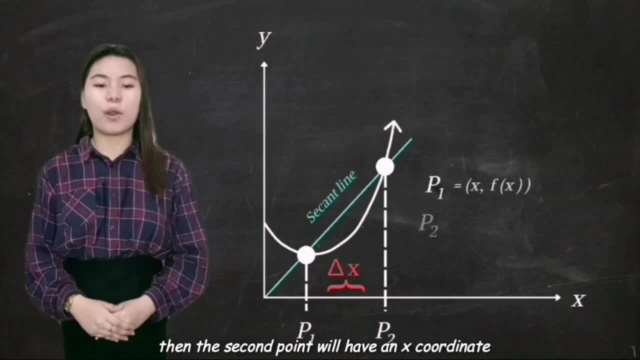 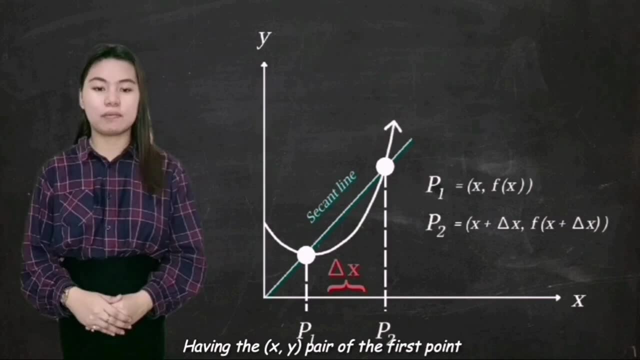 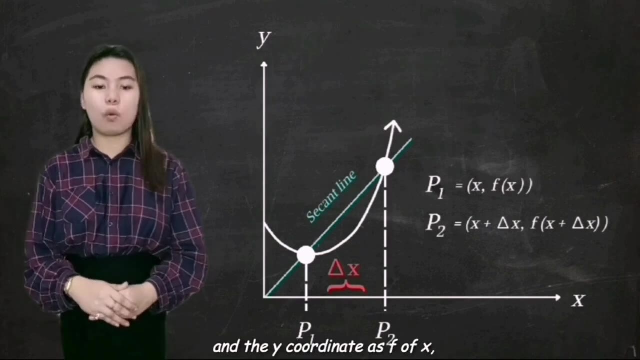 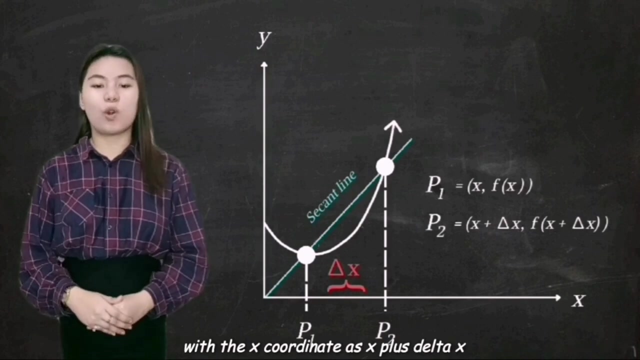 in x or delta x, Then the second point will have an x coordinate of delta x more than x or x plus delta x, Having the x and y pair of the first point with the x coordinate as x and the y coordinate as f of x, and the x and y pair of the second point with the x coordinate as x plus delta. 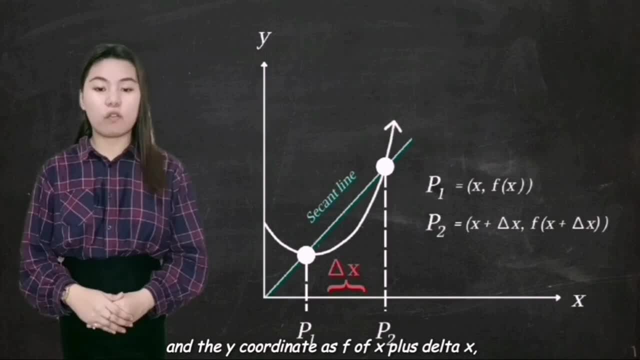 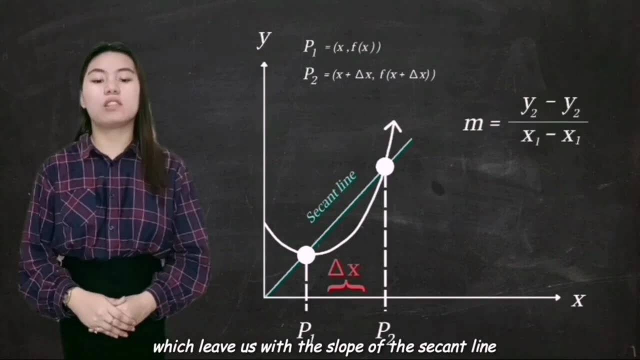 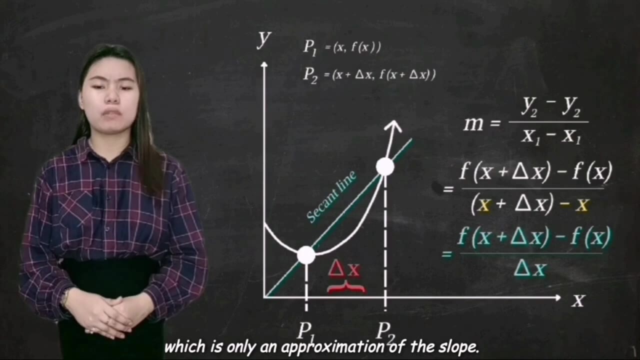 x and the y coordinate as f of x, delta x. we can now use the slope formula, which leave us the slope of the second line, or the difference quotient, which is only an approximation of the slope. How we will turn this into the slope of a tangent line. 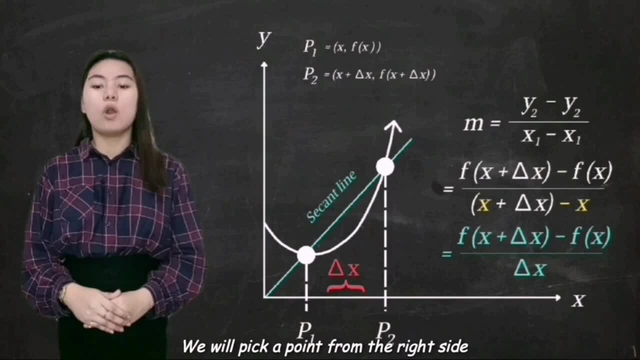 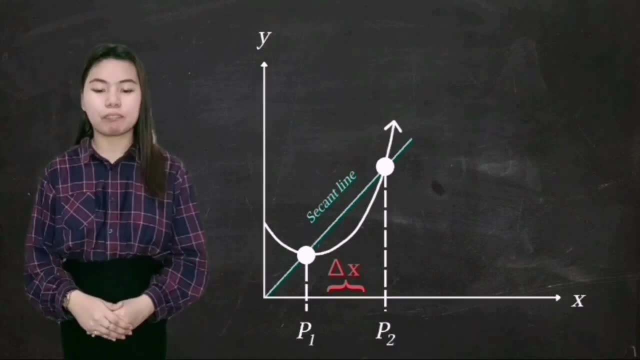 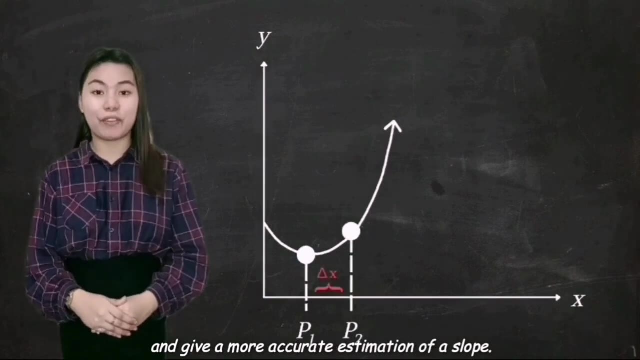 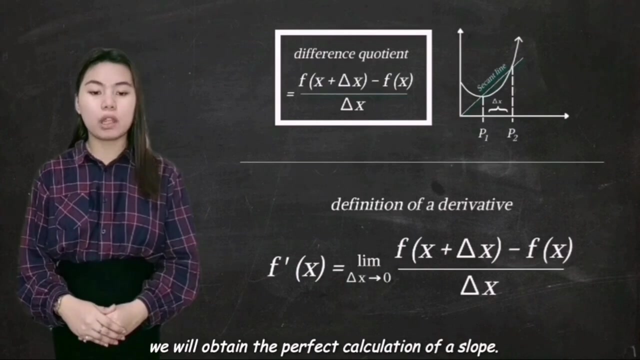 We will pick a point from the right side of the curve that moves closer and closer to the left side, and it will cause the horizontal distance to get smaller and give a more accurate estimation of a slope. By taking the limit of the rate of change in x as it approaches to zero, we will obtain 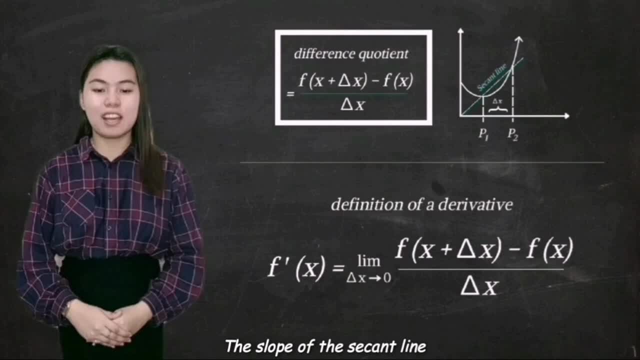 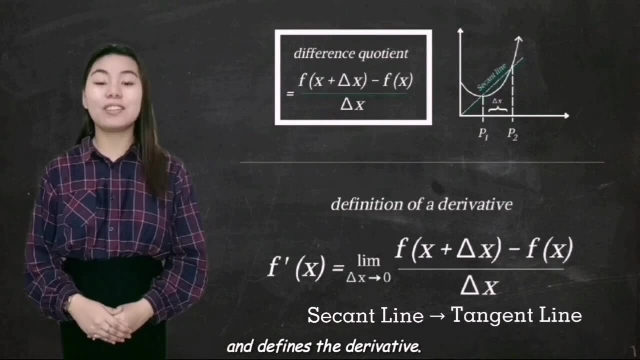 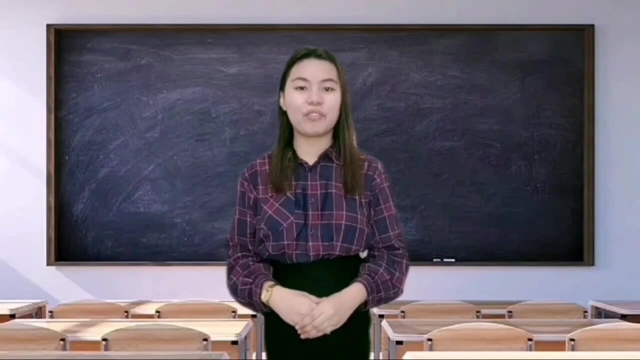 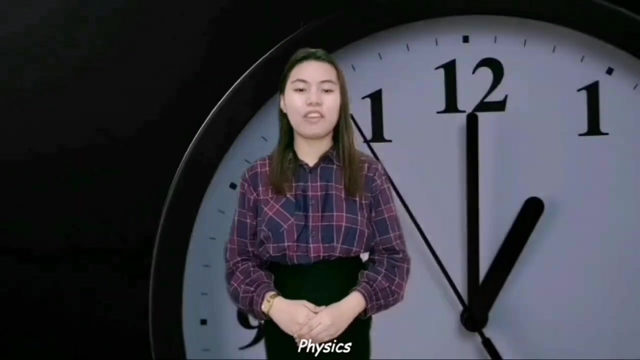 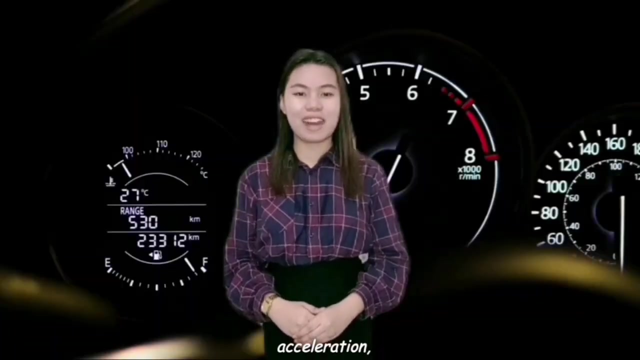 the perfect calculation of the slope. The slope of the second line now becomes the slope of the tangent line and defines the derivative. This topic can be applied to various fields. A few common examples include: business to estimate profit and loss. physics that concerns derivatives with respect to time, including velocity, acceleration and speed. 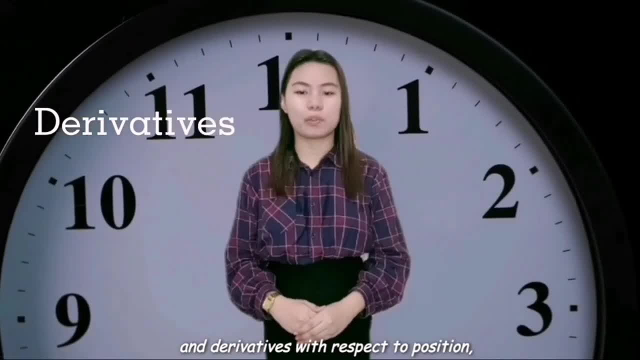 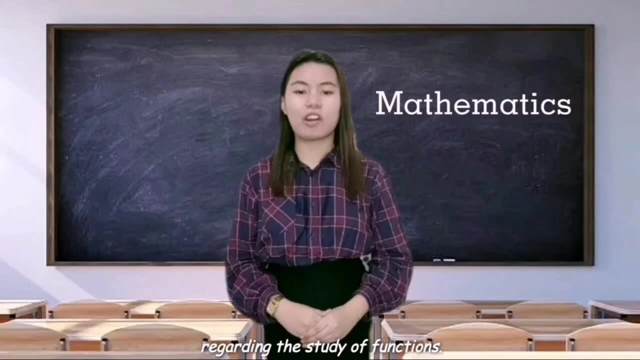 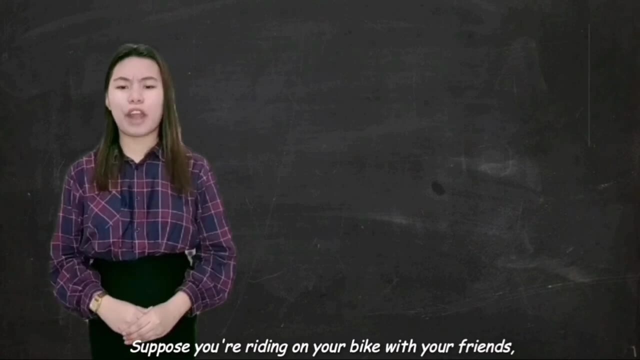 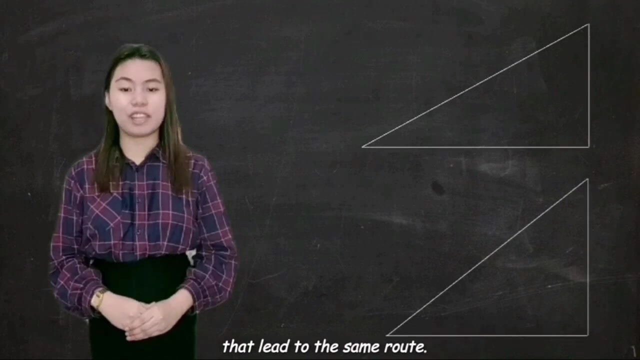 Momentum and derivatives with respect to position, the potential and kinetic energy And, of course, mathematics regarding the study of functions. Let us use a simple scenario. Suppose you are riding on your bike with your friends. Then you encounter two steep roads that lead to the same route. 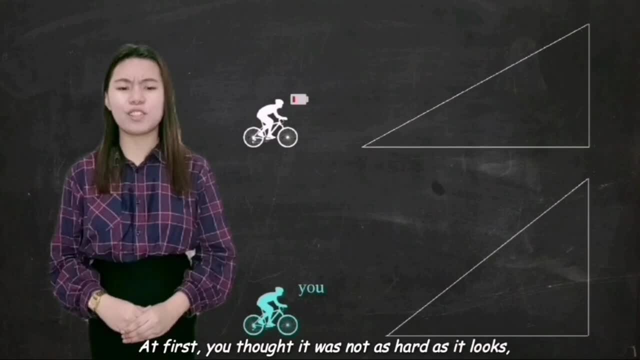 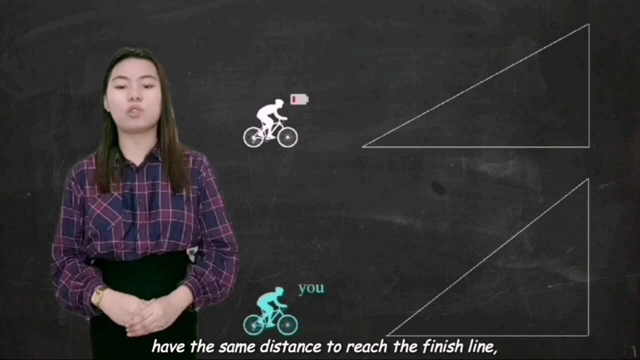 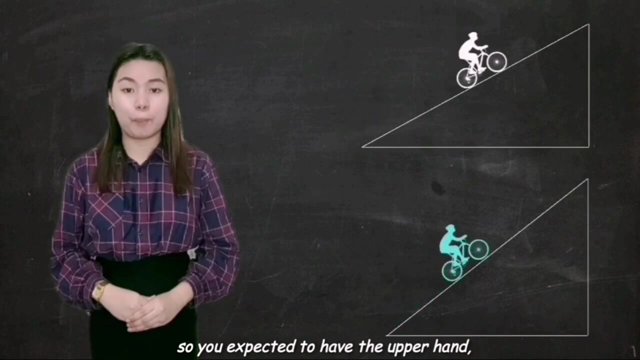 One challenges you to a race. At first you thought that you are going to win, But it was not as hard as it looks, considering that both hills have the same distance to reach the finish line And your opponent seemed tired, so you expected to have the upper hand. 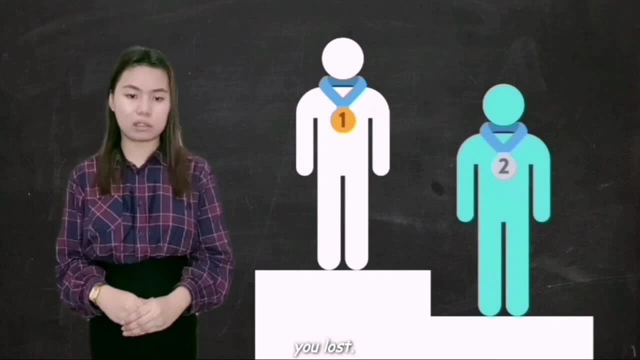 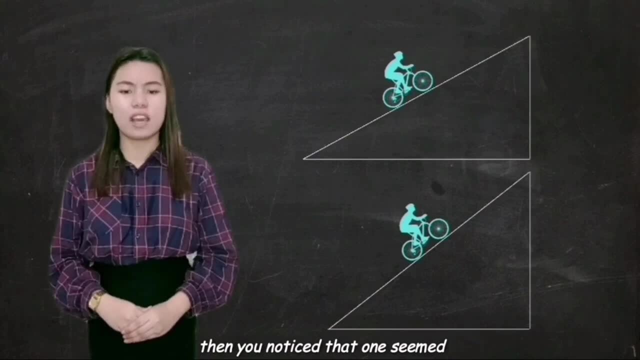 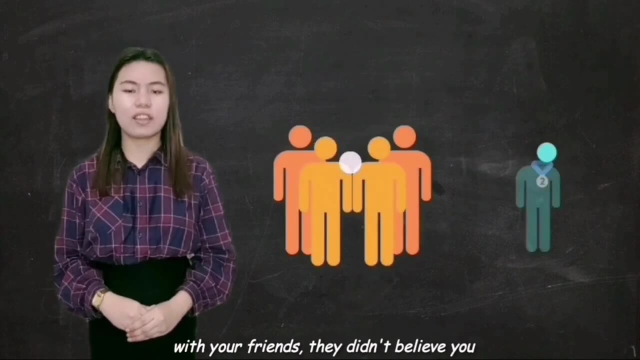 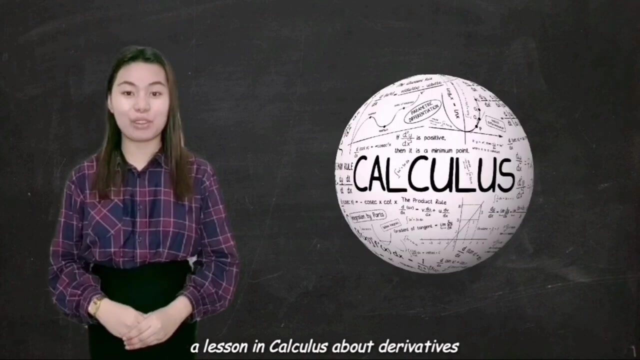 But surprisingly you lost. After the race, you decided to climb both hills. Then you notice that one seems steeper than the other one. When you express your concern with your friends, they didn't believe you. So you used what you learned from a lesson in calculus about derivatives and proved. 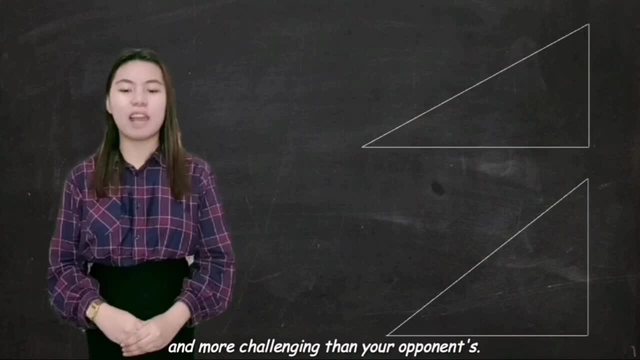 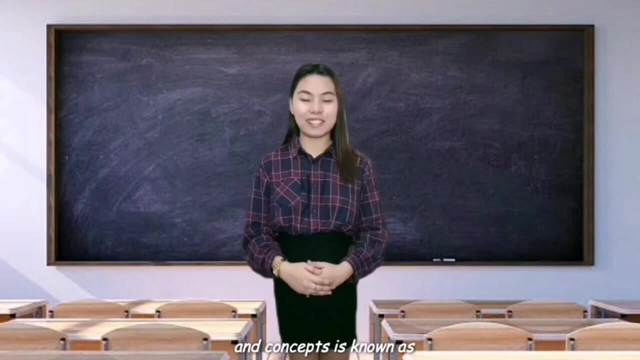 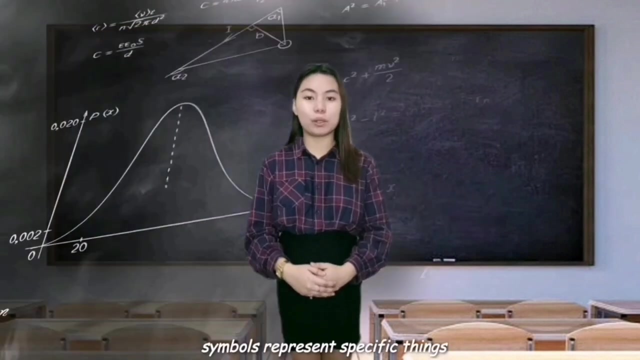 that the slope you climbed was higher and more challenging than your opponent's. A symbolic system for representing mathematical objects and concepts is known as notation. Notation is constructed in such a way that certain symbols, such as numbers, numbers and certain symbols, represent specific things, and communication is efficient. 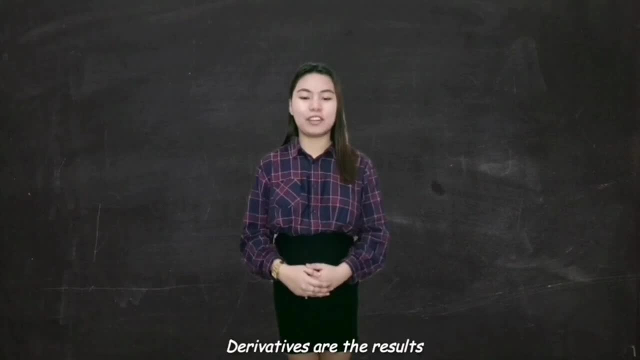 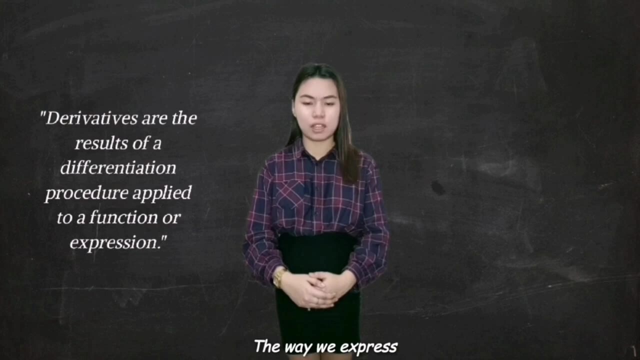 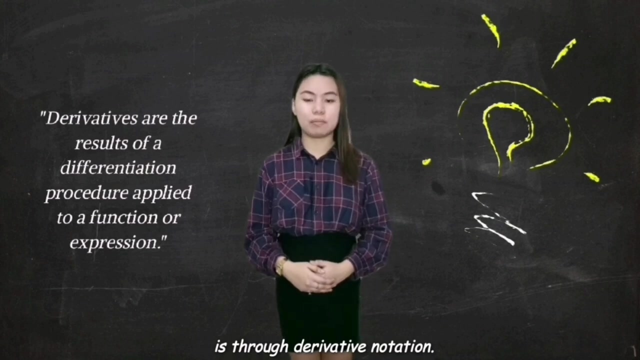 So what is a derivative notation? Derivatives are the result of a differentiation procedure applied to a function or expression. The way we express derivatives theoretically is through derivative notation. Similarly, the derivative of a function, which is a function that represents the slope. 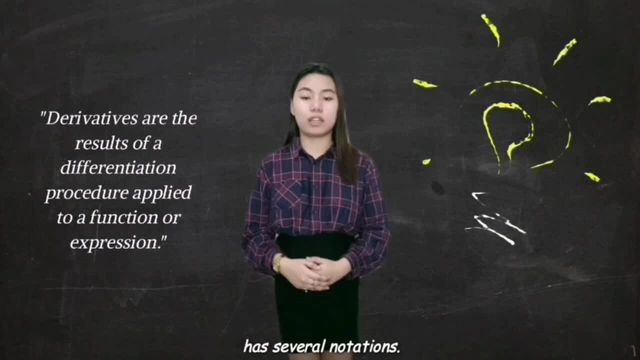 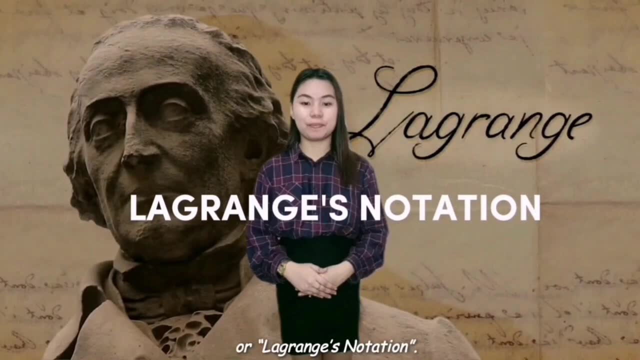 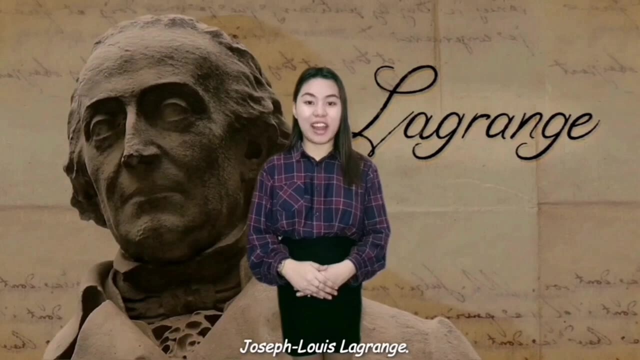 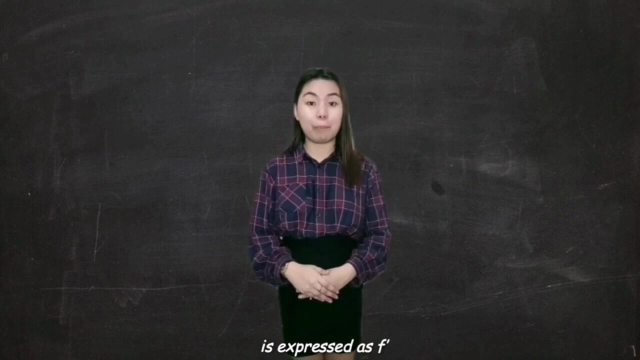 of the tangent line to the original has several notations. The first one is Lagrange's notation. This was introduced by the Italian-French mathematician Joseph-Louis Lagrange. In Lagrange's notation, the derivative of f is expressed as f', pronounced as f'. 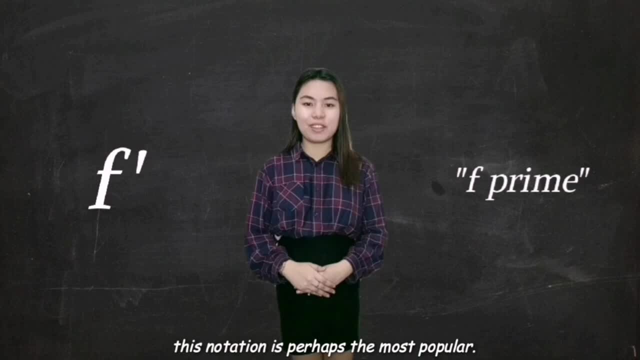 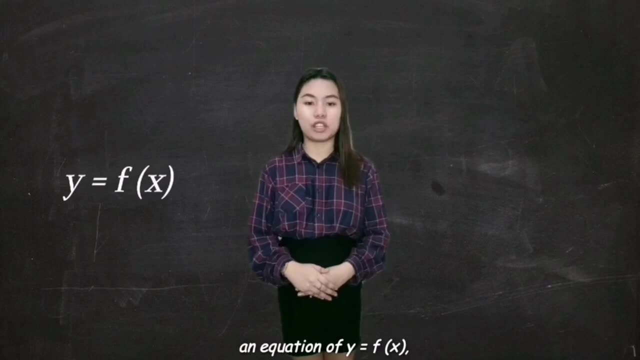 When dealing with function with only one variable. this notation is perhaps the most popular Instead of a function. for example, we have an equation of y is equal to f. we can write it as y' to represent the derivative. The second one is the Leibniz notation. 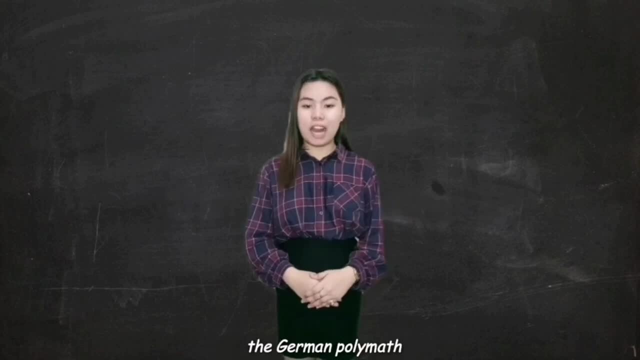 This notation was introduced by the German polymath Gottfried Wilhelm Leibniz. This notation was introduced by the German polymath Gottfried Wilhelm Leibniz. In Leibniz notation the derivative of f is expressed as d over dx of f. 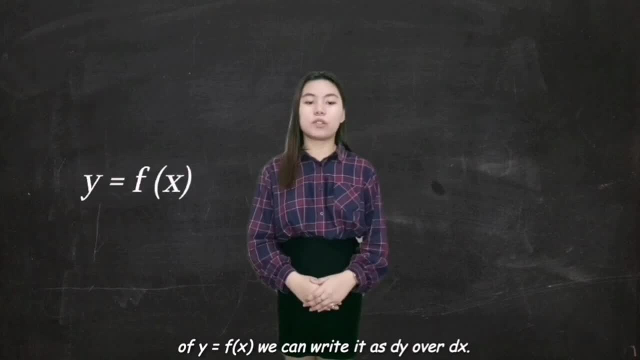 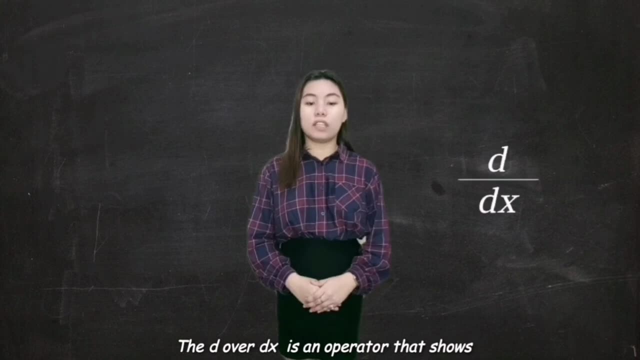 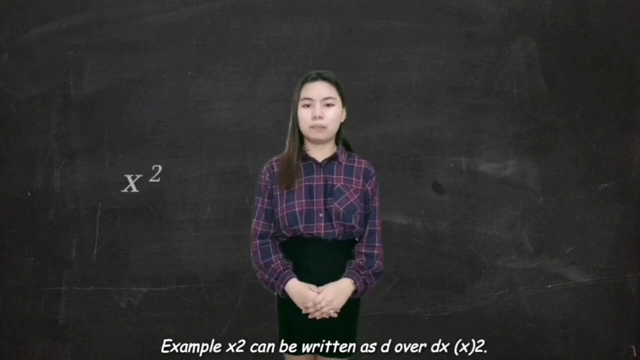 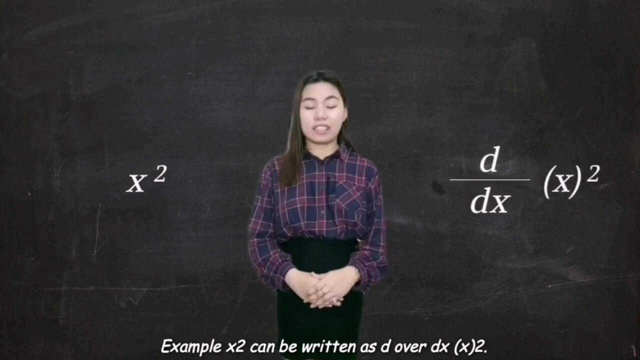 For example, we have an equation of y is equal to f. We can write it as dy over dx. The d over dx is an operator that shows a differentiation with respect to x. Example: The derivative of x squared can be written as d over dx of x squared. 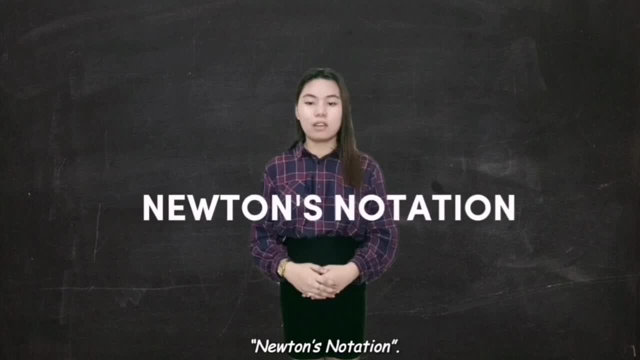 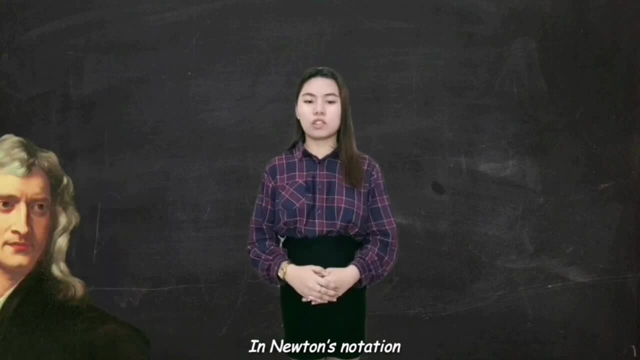 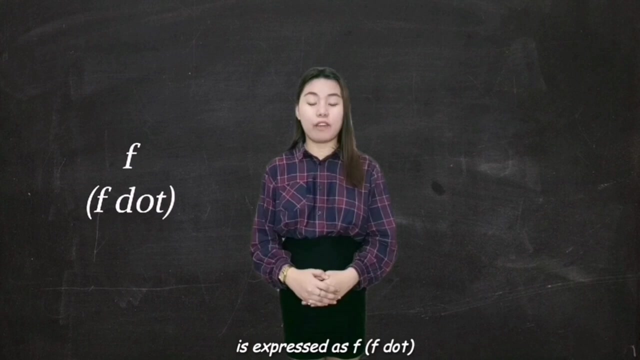 The third one is the Newton's notation. This notation was introduced by an English mathematician, Isaac Newton. In Newton's notation, also known as the dot notation, the derivative of f is expressed as f- dot and the derivative of y is equal to f. of x is expressed as y, y, dot. 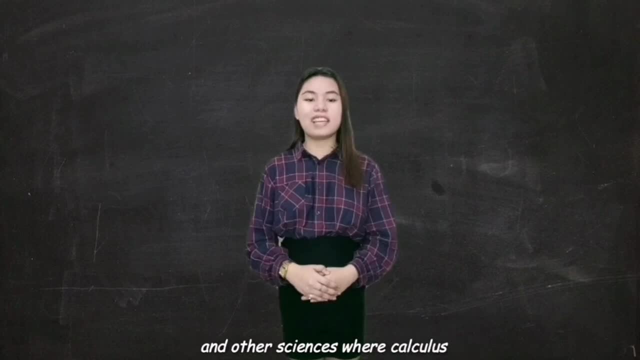 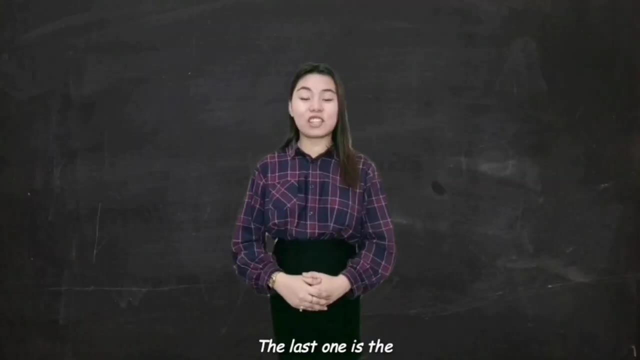 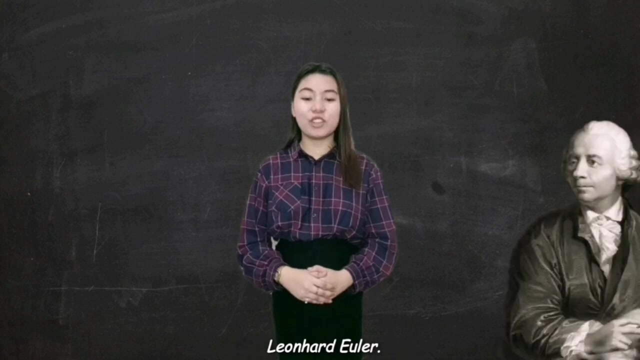 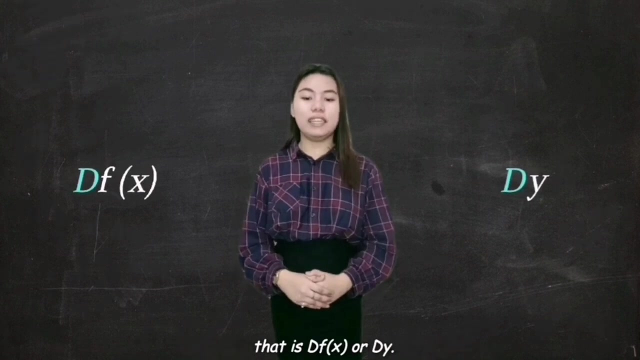 This notation is mostly common in physics and other sciences where calculus is applied in real world context. The last one is the Euler's notation. This notation was introduced by a Swiss mathematician, Leonhard Euler. In this notation we denote a derivative with a capital E, that is, d, f of x or dy. 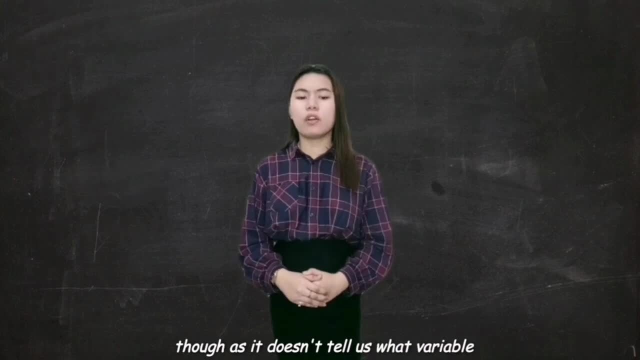 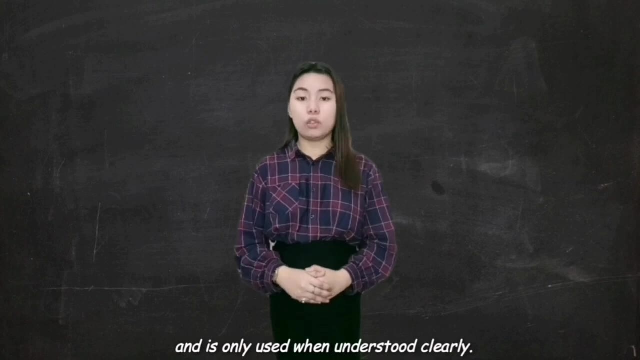 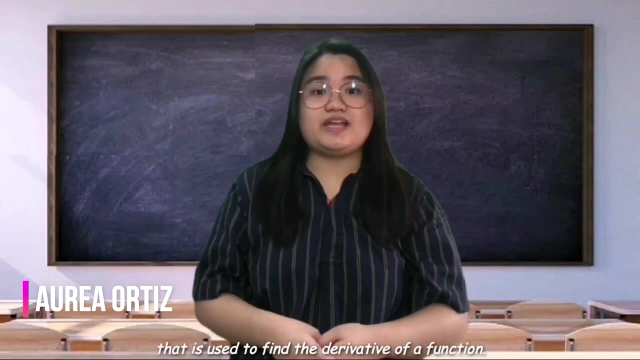 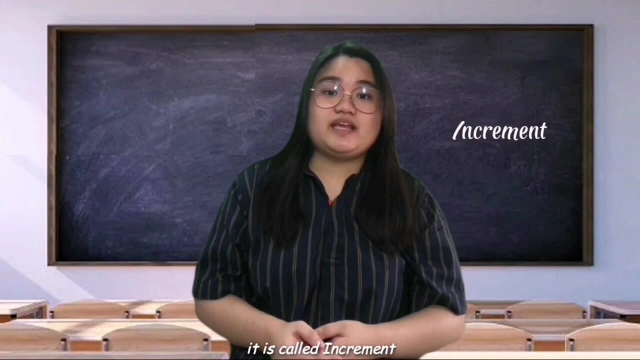 This notation has its own limitation, though, as it doesn't tell us what variable to differentiate with respect to and is only used when understood clearly. The increment method is a long method that is used to find the derivative of a function In calculus. if there is a change in a variable, it is called increment and is denoted by the Greek. 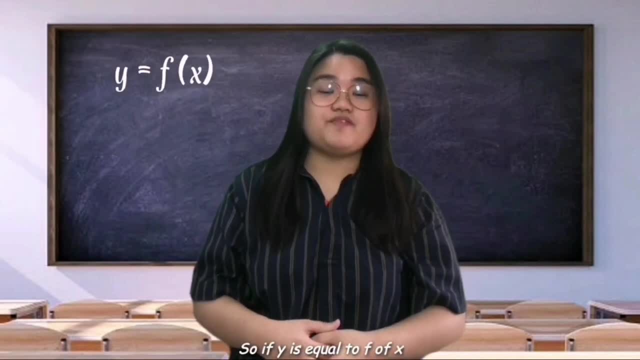 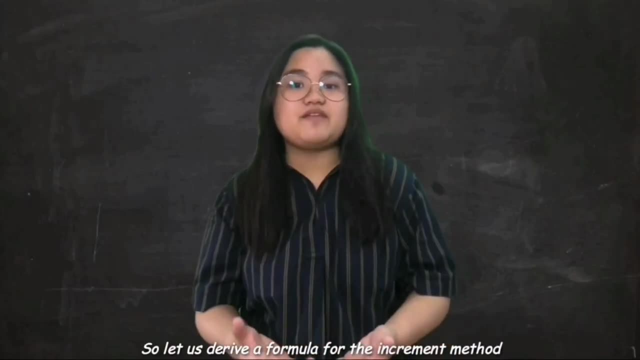 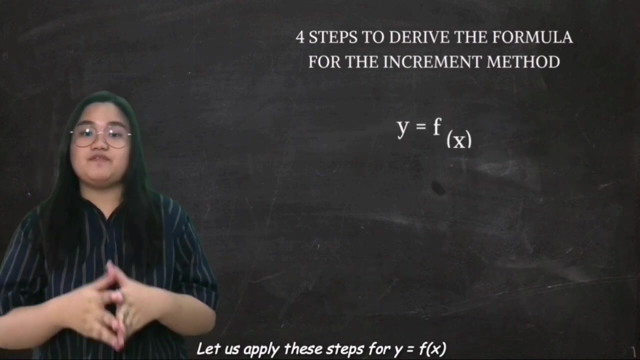 letter delta. So if y is equal to f of x and there is a corresponding change in y, then there will also be a change in f of x. So let us derive a formula for the increment method by following these four steps. Let us apply these steps, for y is equal to f of x. 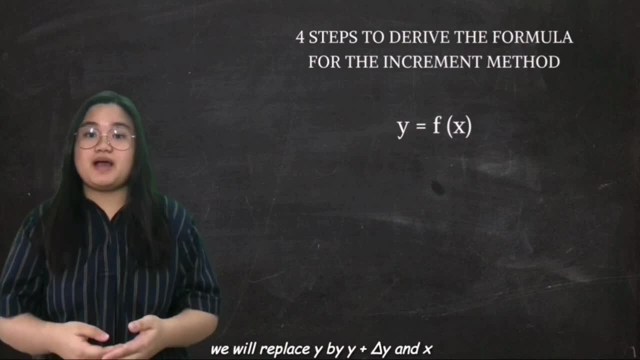 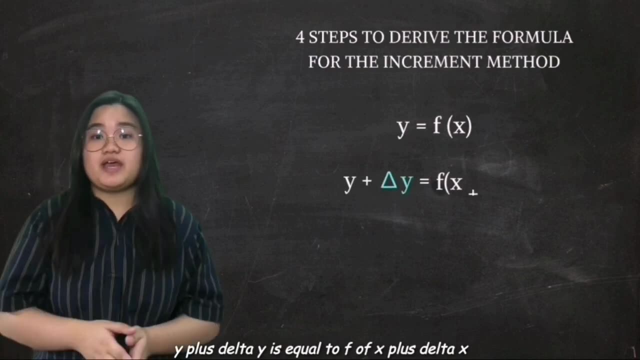 By the first step. we will replace y by y plus delta y and x by x plus delta x. So we will get y plus delta y is equal to f of x plus delta x. Next we will subtract y from y plus delta y and the value of y in the other side of. 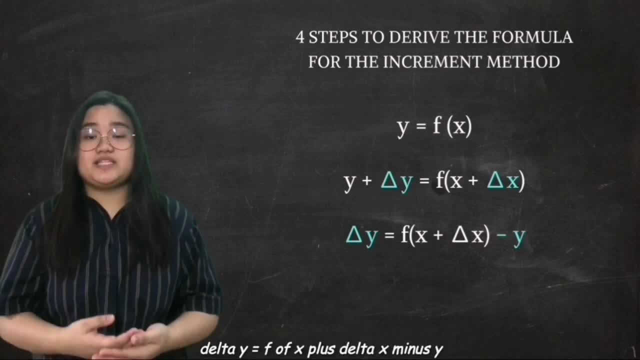 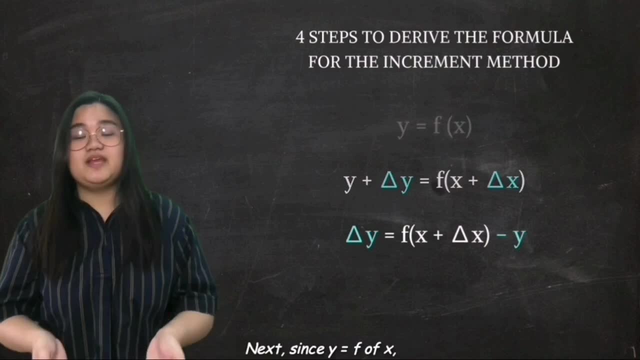 the equation. So we will come up with: delta y is equal to f of x plus delta x minus y. We basically transpose y to the other side of the equation. Next, since y is equal to f of x, we can say that delta y is equal to f of x plus delta. 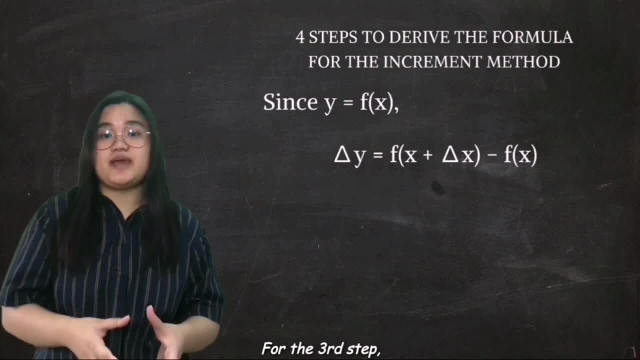 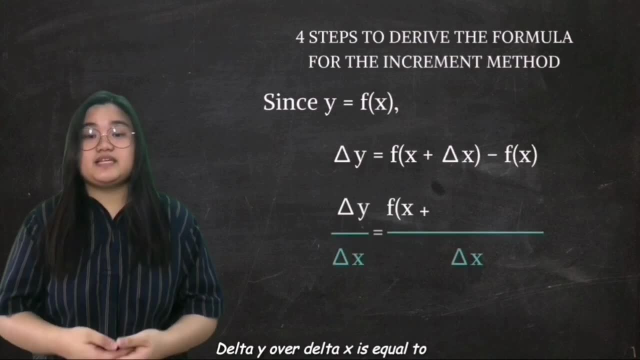 x minus f of x. For the third step, we will subtract y from y plus delta y. For the third step, we will divide both sides of the equation by delta x, So we will come up with delta y over. delta x is equal to f of x plus delta x minus f. 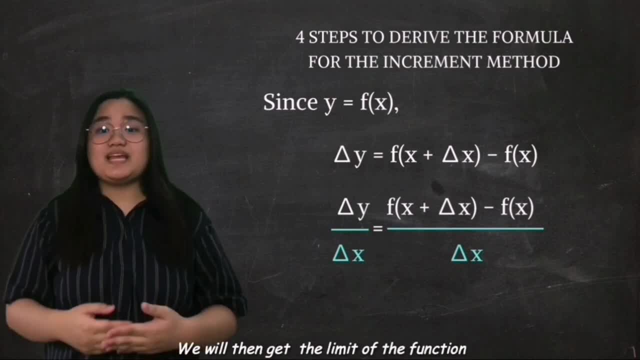 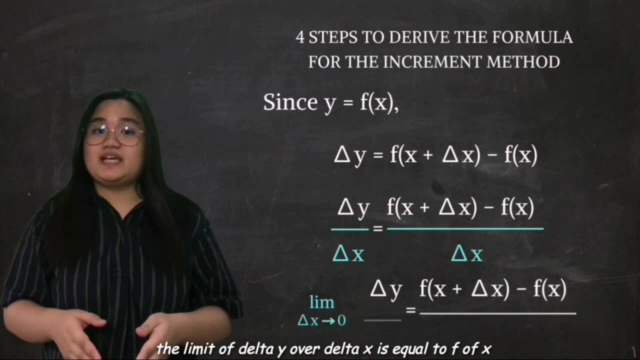 of x over delta x. We will then get the limit of the function as delta x approaches 0.. So we will have: the limit of delta y over delta x is equal to f of x plus delta x, minus f of x over delta x as delta x approaches 0.. 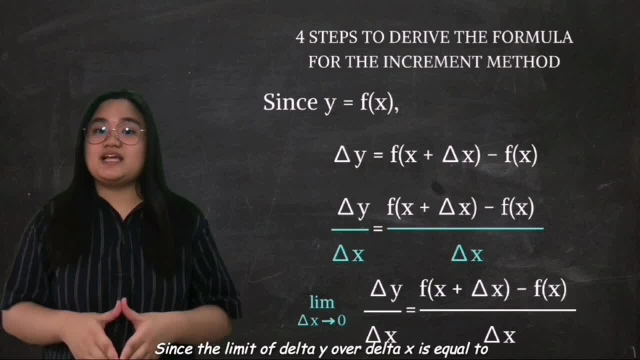 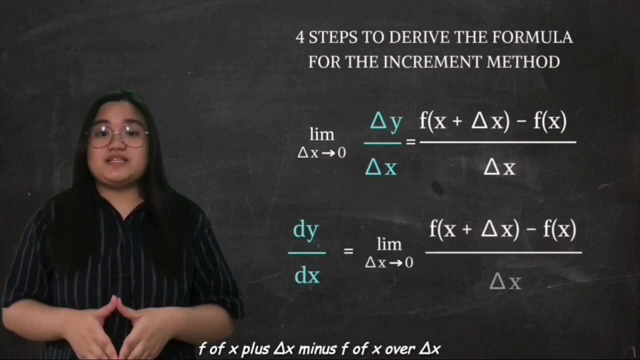 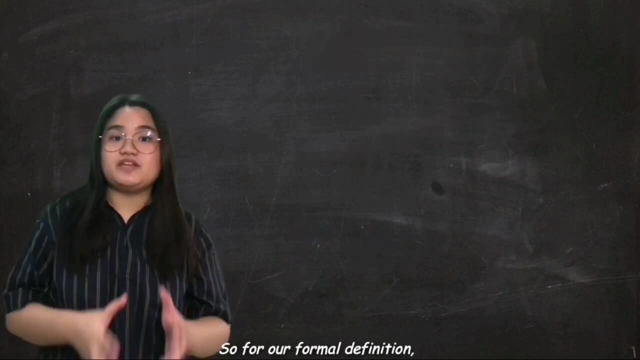 zero. Since the limit of delta y over delta x is equal to dy over dx, we can say that dy over dx is equal to the limit of f of x plus delta x minus f of x over delta x, as delta x approaches zero. So for a formal definition, the 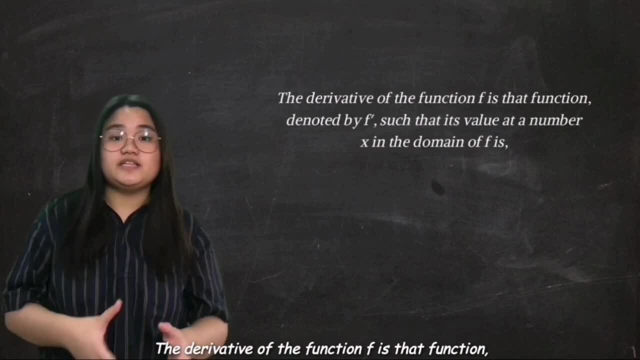 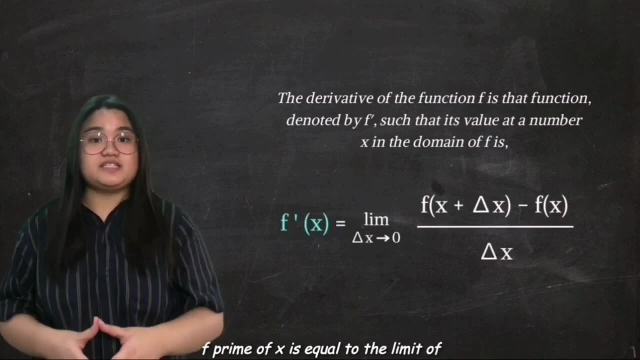 derivative of the function f is that function denoted by f prime, such that its value at the number x in the domain of f is f. prime of x is equal to the limit of f of x plus delta x minus f of x over delta x as delta x approaches. 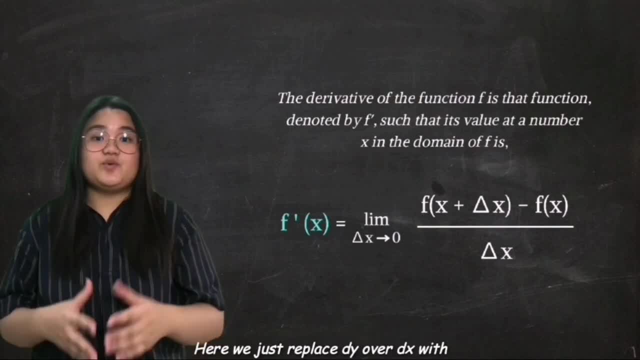 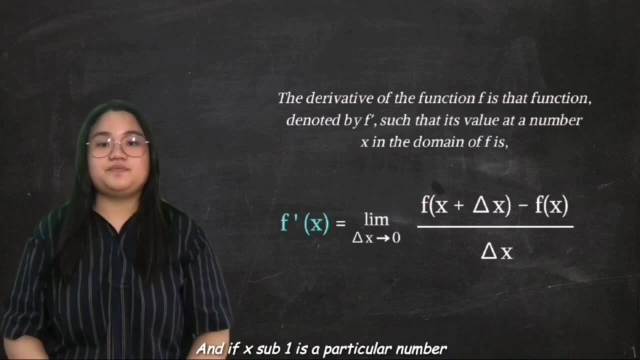 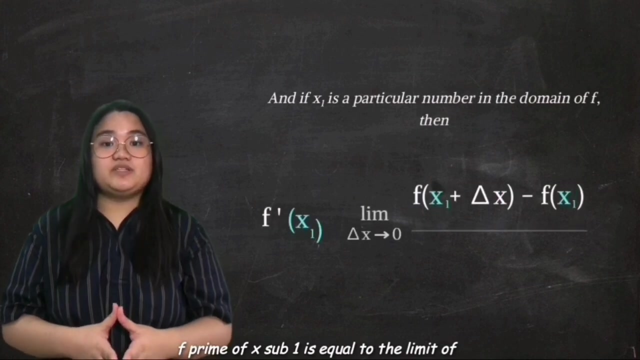 zero. if this limit exists. Here we just replace dy over dx with f prime x, since both are forgetting the derivatives. And if X1 is a particular number in the domain of f, then f prime of X1 is equal to the limit of f of X1 plus delta x, minus f of X1 over delta x. 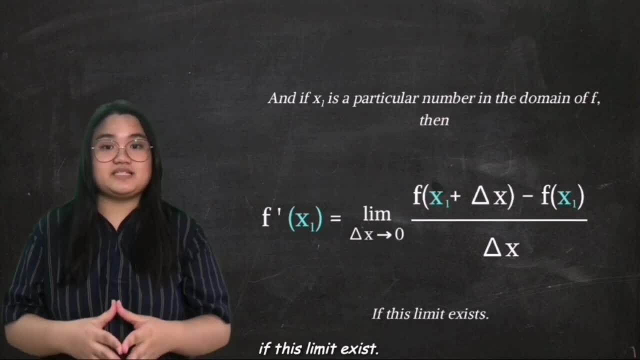 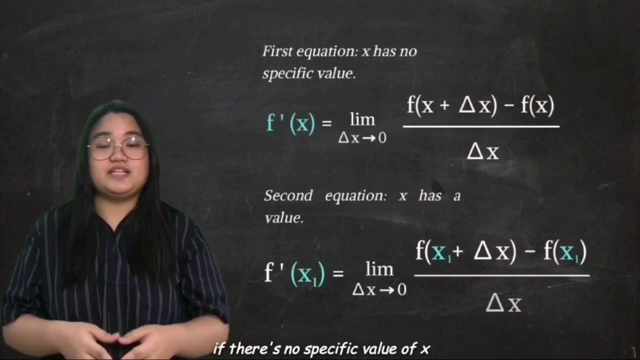 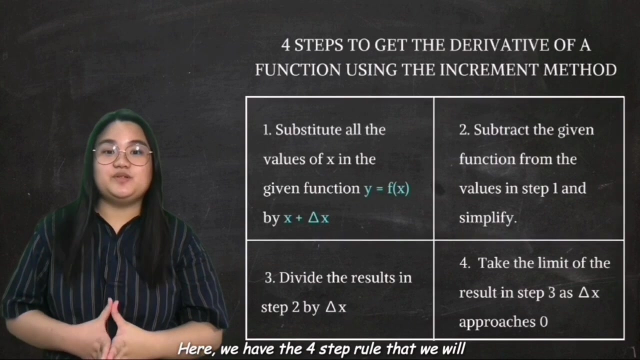 or x over delta x, as delta x approaches zero if this limit exists. the difference of these two equations are simple: the first equation is used if there is no specific value of x, while the second equation is used if there is a value of x. here we have a four step rule that we will follow in order to get the 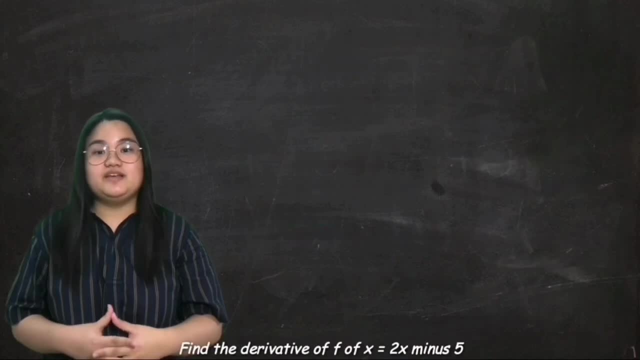 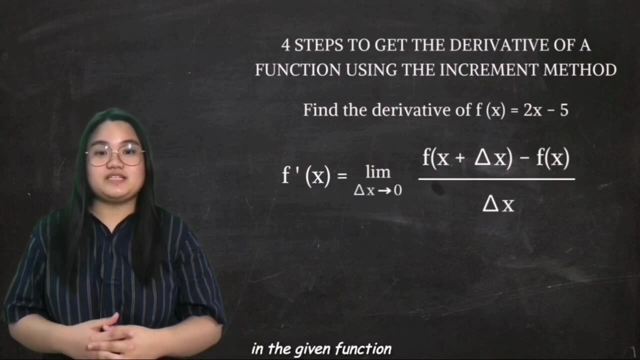 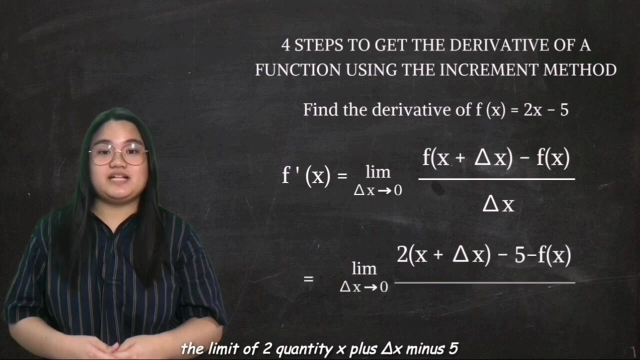 derivative of a function. using the increment method, find the derivative of f of x equals 2x minus 5.. we will first substitute all the values of x in the given function by x plus delta x, so we will obtain the limit of two quantity: x plus delta x minus five, minus f of x over delta x. 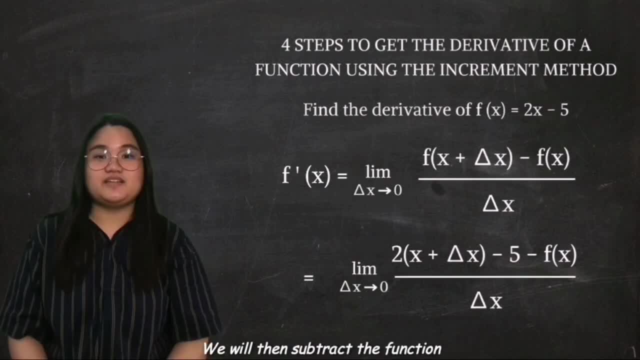 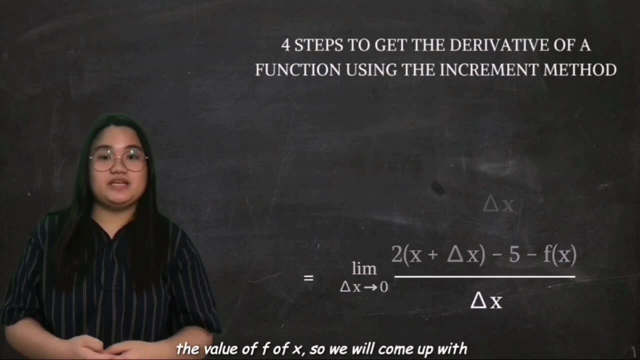 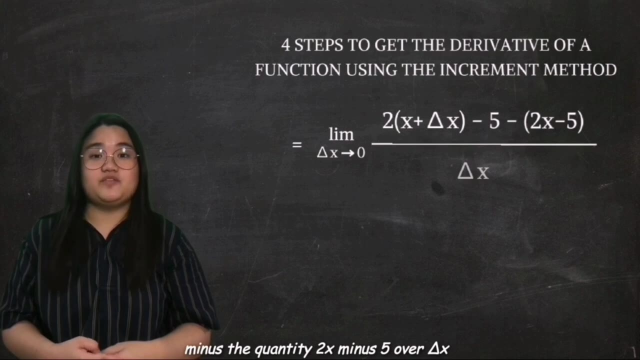 as delta x approaches zero. we will then subtract the function from the given values. that basically means that we will substitute the value of f of x, so we will come up with the limit of two: quantity x plus delta x minus 5, minus quantity 2x minus 5 over delta x as delta x approaches zero. after that, 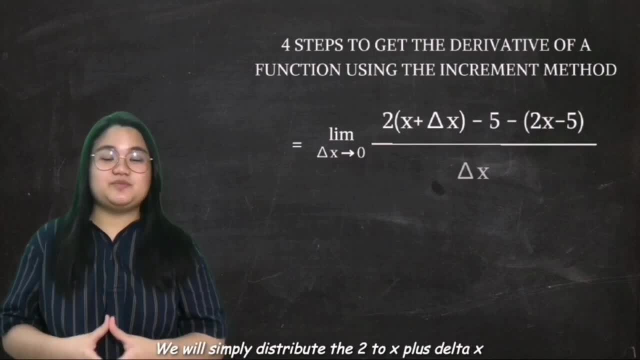 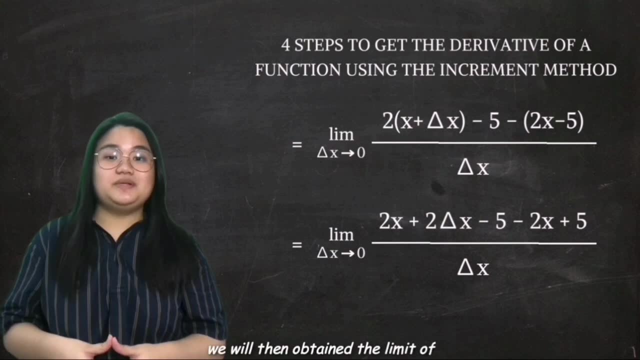 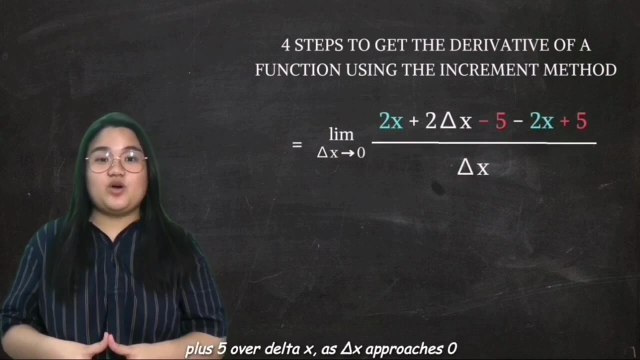 we can simplify the equation. we will simply distribute 2 to x plus delta x and the negative sign, or negative 1 to 2x minus 5.. we will then obtain the limit of 2x plus 2, delta x minus 5 minus 2x plus 5 over delta x as delta x approaches zero. 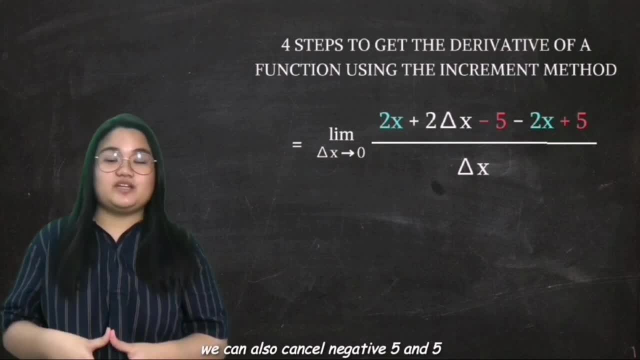 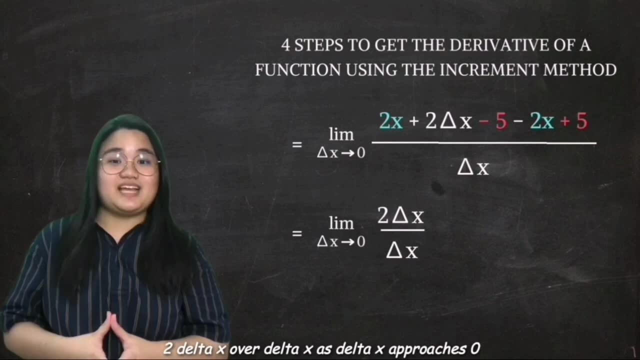 here we can cancel 2x and negative 2x. we can also cancel negative 5 and 5.. so we will obtain the limit of 2 delta x over delta x as delta x approaches 0.. we will then divide the result by: 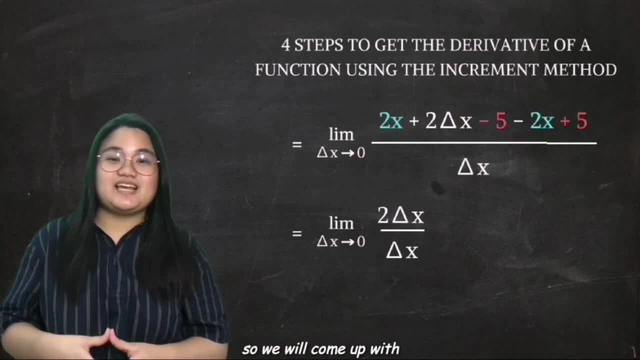 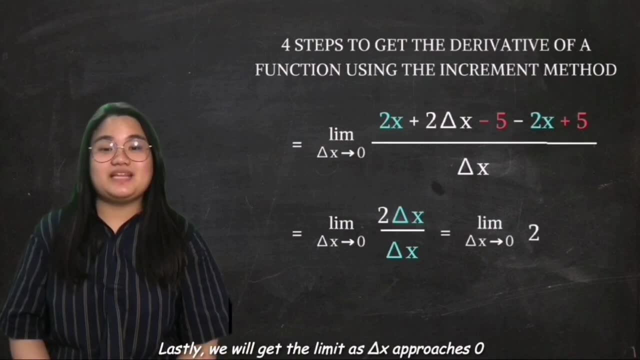 delta x over here. we can cancel delta x, so we will come up with the limit of 2 as delta x approaches 0.. lastly, we will get the limit as delta x approaches 0 and by the limit theorem 2 or the limit of a constant, the limit of 2 is equal to 2 as delta x approaches 0, so we will obtain a final. 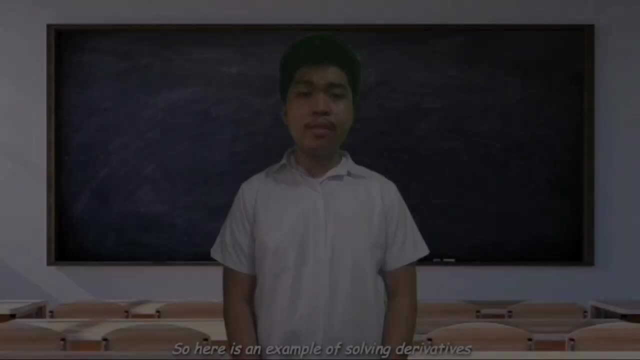 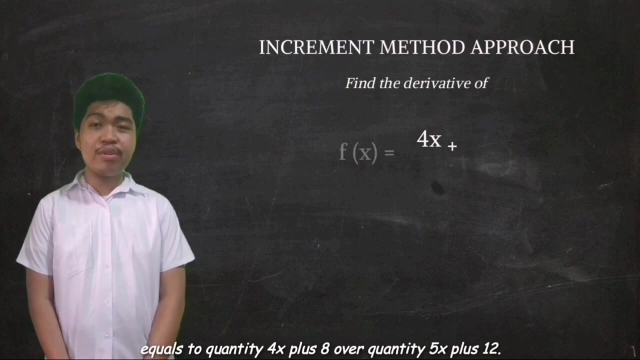 answer of f, prime of x is equal to 2.. so here is an example of solving derivatives using increment method. find the derivative of f of x equal to quantity 4x plus 8 over 5x plus 12.. keep in mind. 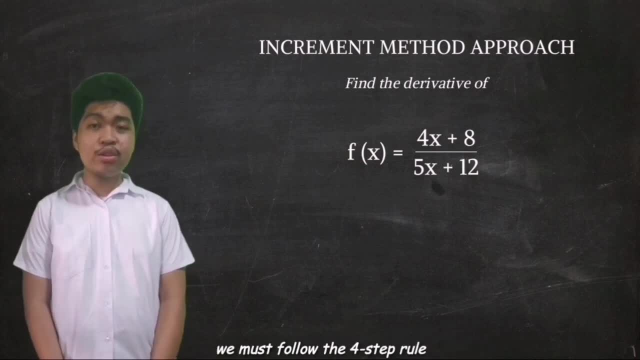 that when using the increment method to solve the derivative of a function, we must follow the 4 step rule and we will use the 4 step rule to solve the derivative of a function. last part is: we will use the魚's Masters method and we must use the follow 4 step rule and we will use the steady sort method. you can apply this formula. thanks, 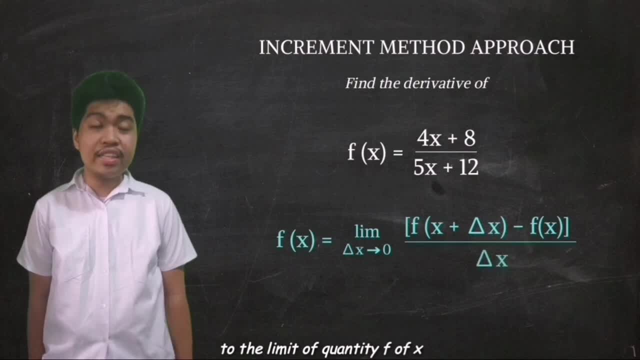 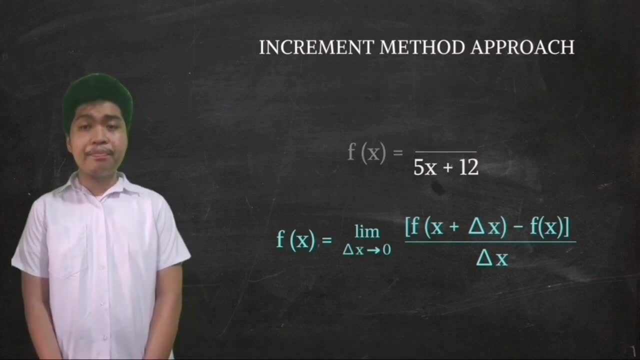 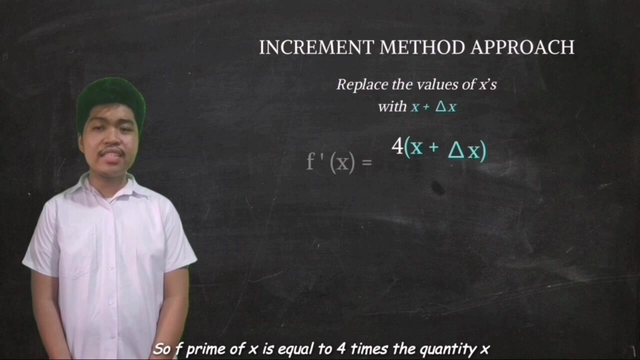 formula f prime of x is equal to the limit of quantity f of x plus delta x, minus f of x, all over delta x as delta x approaches to zero. First replace the values of x's with x plus delta x in the given equation. So f prime of x is equal to 4 times the quantity. 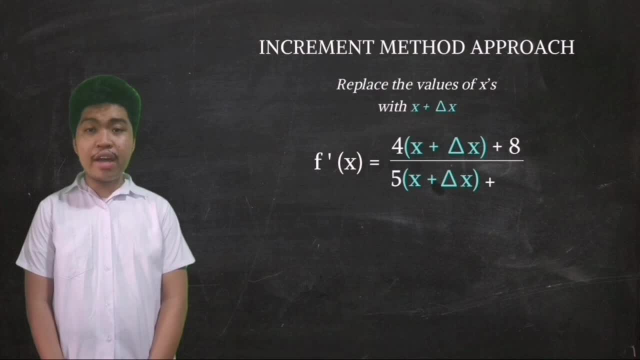 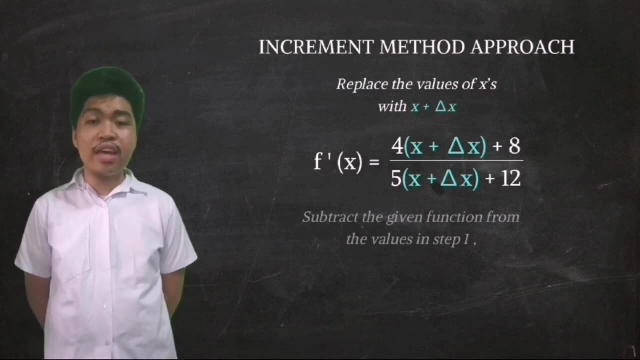 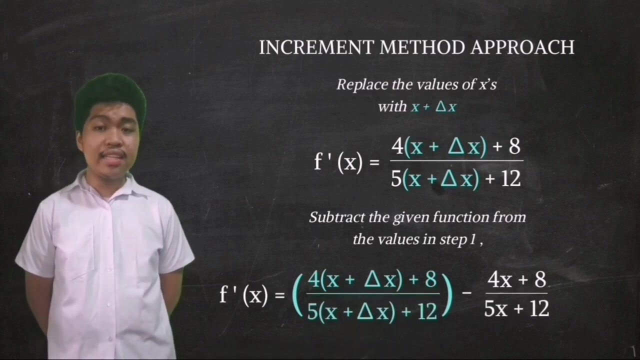 of x plus delta, x plus 8, all over 5 times the quantity of x plus delta, x plus 12.. For the second rule, we must subtract f of x to the equation we formed. f prime of x is equal to quantity: 4 times the quantity of x plus delta, x plus 8, all over 5 times the. 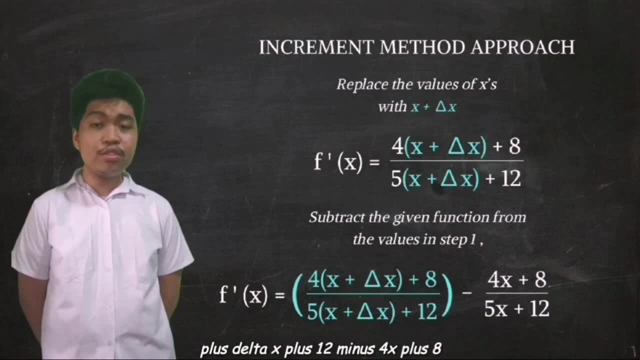 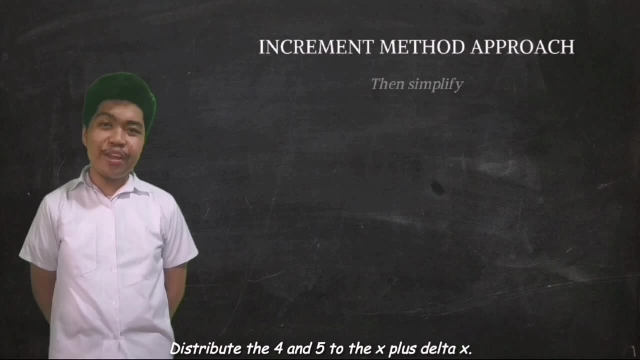 quantity of x plus delta x plus 12 minus 4x plus 8 over quantity 5x plus 12.. Then just simplify: Distribute the 4 and 5 to the x plus delta x. f prime of x is equal to quantity. 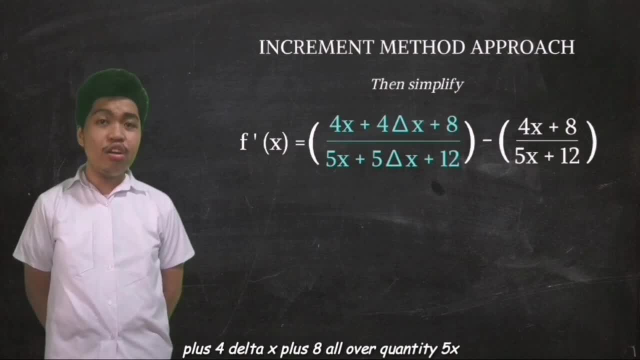 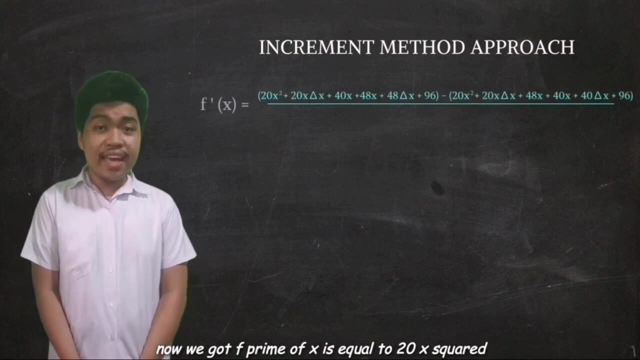 4x plus 4, delta x plus 8.. All over, quantity 5x plus 5. delta x plus 12, minus quantity 4x plus 8 over quantity 5x plus 12.. Get the LCD and then simplify. Now we got f. prime of x is equal to 20x squared. 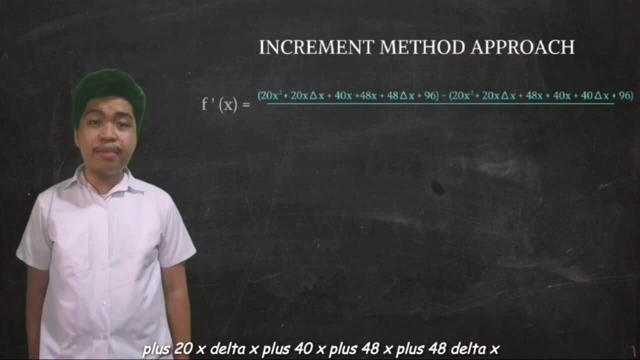 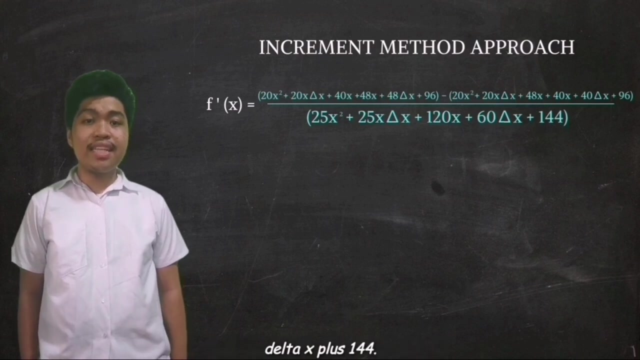 plus 20x delta x plus 40x plus 48x plus 48 delta x plus 96, minus quantity: 20x squared plus 20x delta x plus 40x plus 48x plus 96.. All over the quantity of 25x squared plus 25x delta x plus 120x plus 60x delta x plus. 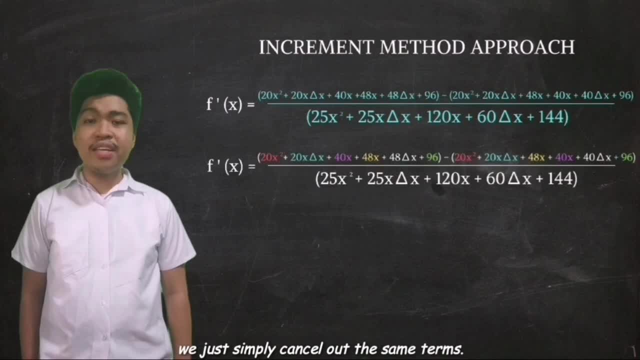 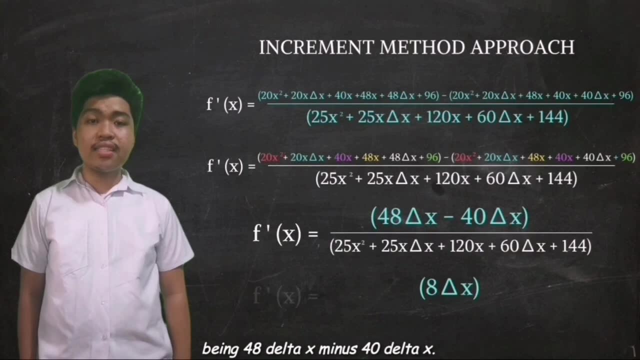 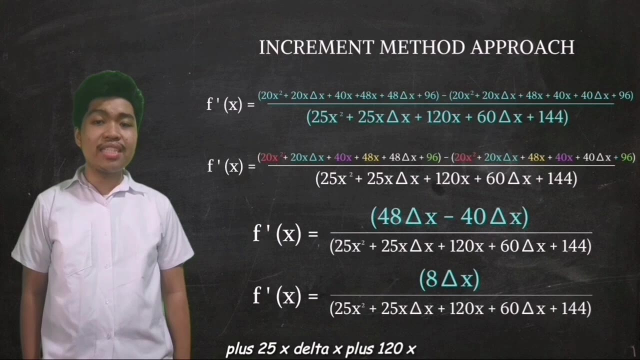 144.. Following that, we just simply cancel out the same terms. This will result the numerator being 40x delta x minus 40x delta x. Simplify and now we got 8x delta x, all over the quantity of 25x squared plus 25x delta. 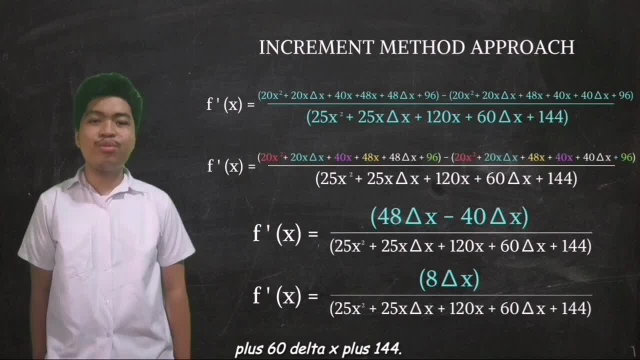 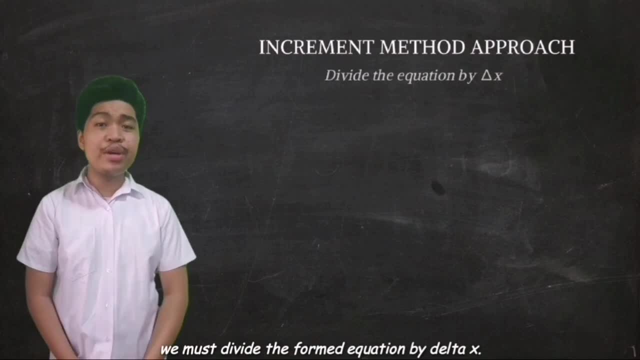 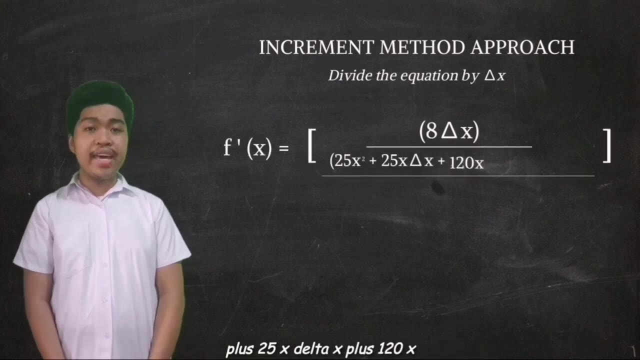 x. For the second to the last rule, in increment method we must divide the form equation by delta x, So 8x delta x, all over the quantity of 25x squared plus 25x. delta x plus 120x plus 60x. 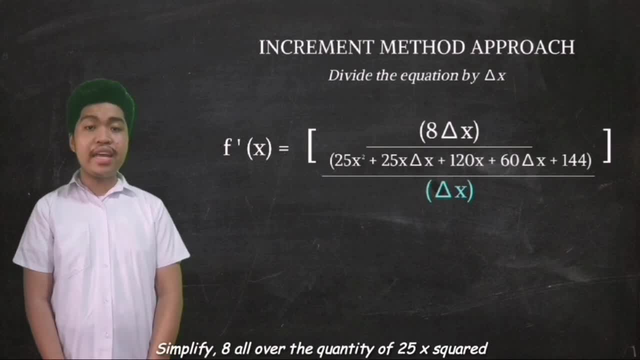 delta x plus 144x divided by delta x. Simplify 8 all over the quantity of 25x squared plus 25x delta x plus 130x divided by delta x. Then just simplify About the total quantity of 25x squared plus 120x plus 60x delta x plus. 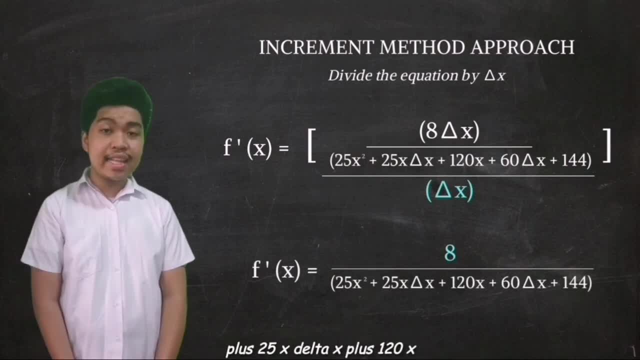 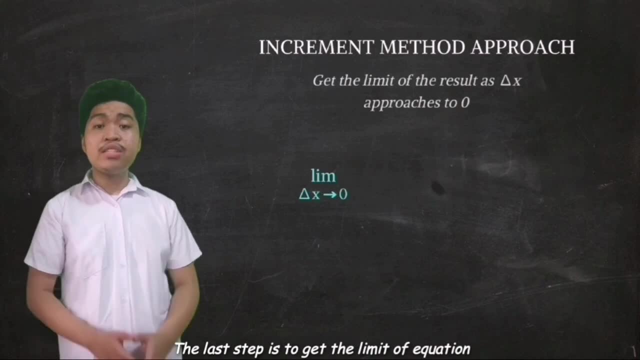 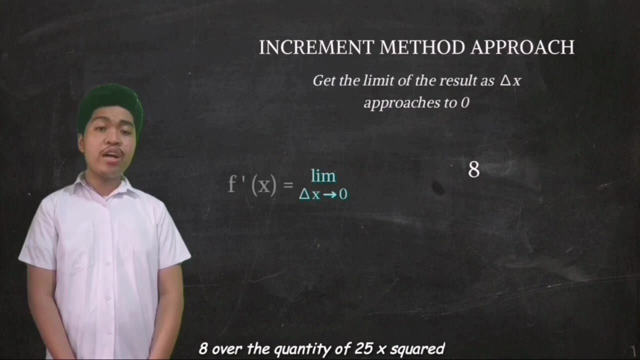 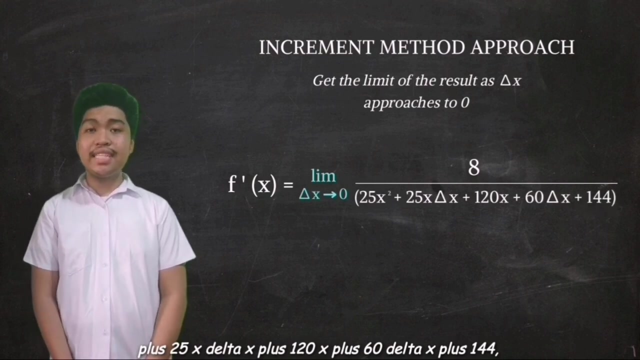 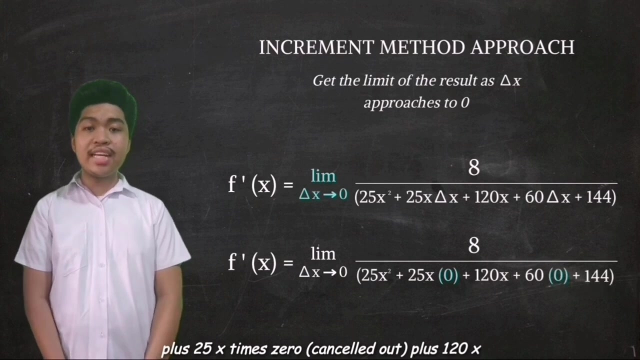 5x plus 1.. 25x squared plus 25x delta x plus 120x, plus 60 delta x plus 144.. The last step is to get the limit of the equation as delta x approaches to 0.. The limit of the equation- 8 over the quantity of 25x squared plus 25x delta x plus 120x, plus 60 delta x plus 144 as delta x approaches to 0- is 8 all over the quantity of 25x squared plus 25x times 0 cancelled out, plus 120x, plus 60 times 0 cancelled out, again plus 144.. 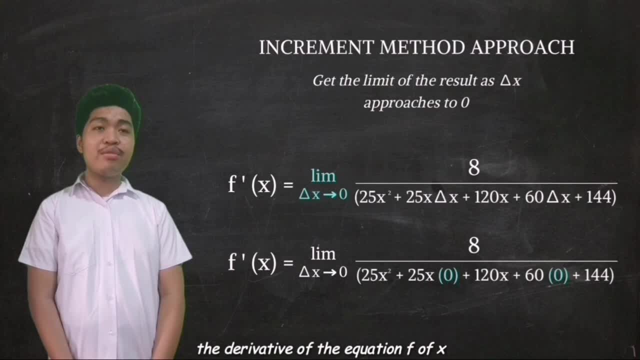 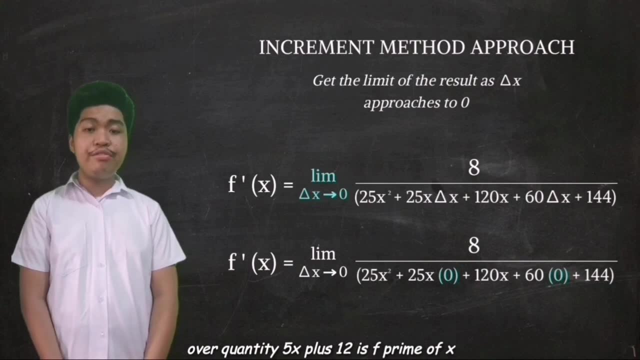 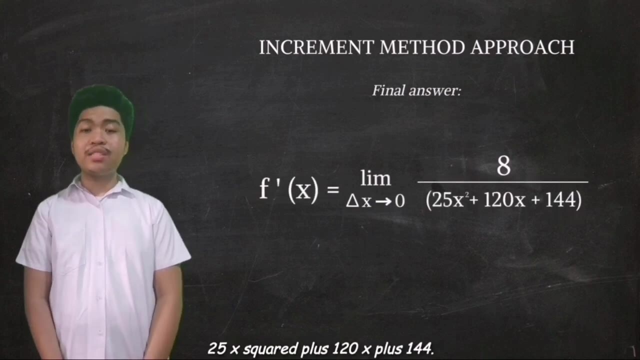 So this is the limit of the equation. So for our final answer, the derivative of the equation f of x equal to quantity 4x plus 8 over quantity 5x plus 12, is f prime of x equal to 8 all over the quantity of 25x squared plus 120x plus 144.. 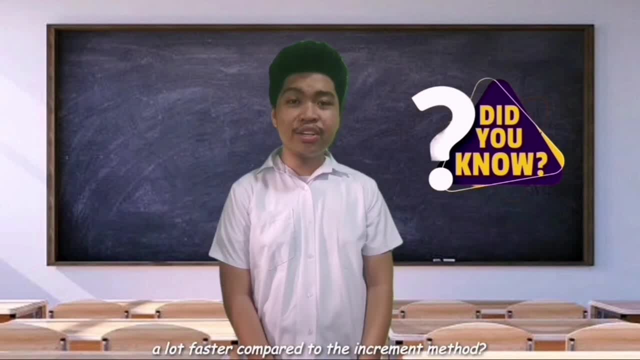 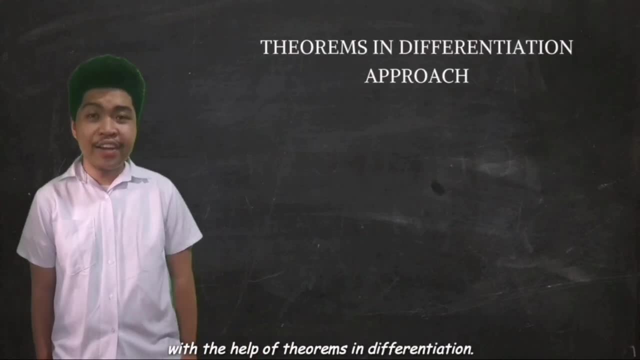 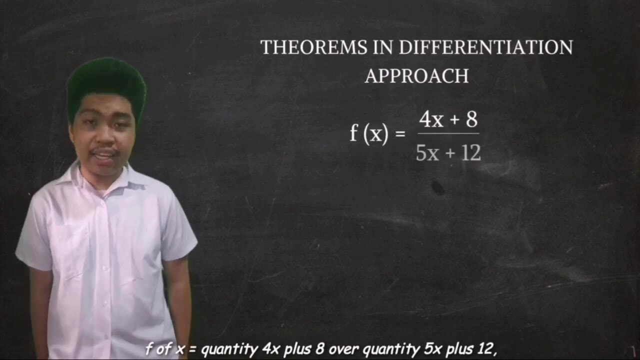 But wait, did you know that we can solve this equation a lot faster compared to the increment method? We can save a lot more time than the increment method With the help of theorem in differentiation. So now we will find the derivative of the equation f of x equal to quantity 4x plus 8 over quantity 5x plus 12.. 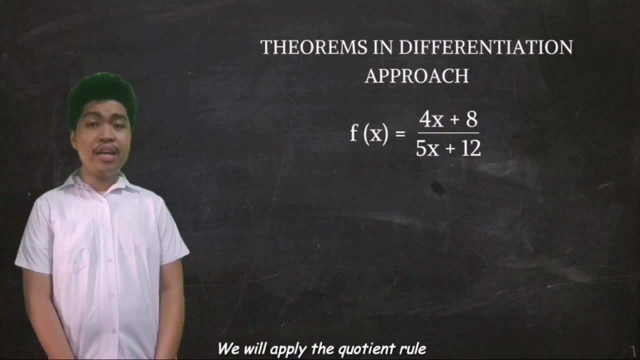 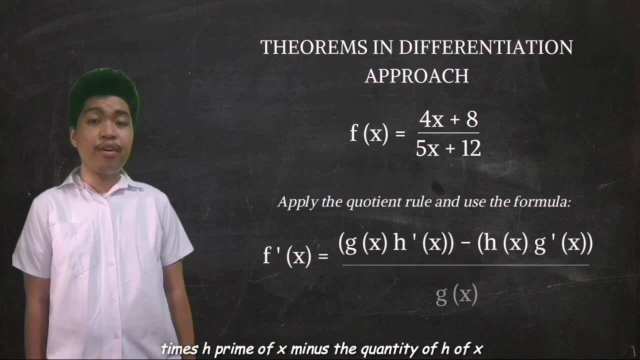 But the theorem. in differentiation approach, We will apply the quotient rule and use the formula: f prime of x is equal to quantity of g of x times h prime of x minus the quantity of h of x times g prime of x all over g of x squared. 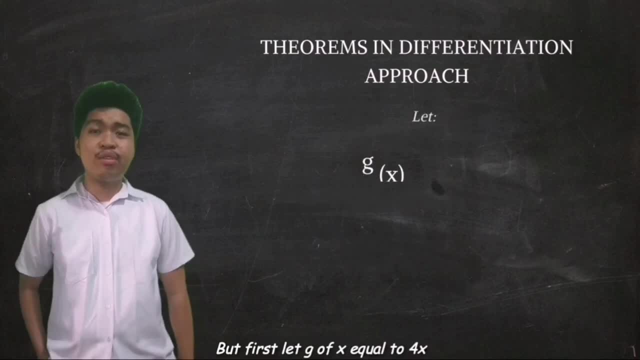 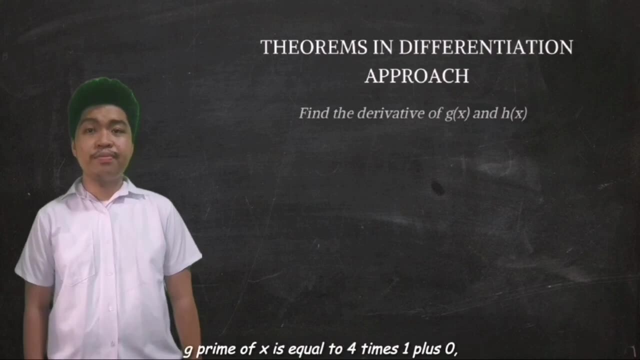 But first let g of x equal to 4x plus 8 and h of x equal to 5x plus 12.. Then find the derivative of the 2. g prime of x is equal to 4 times 1 plus 0.. 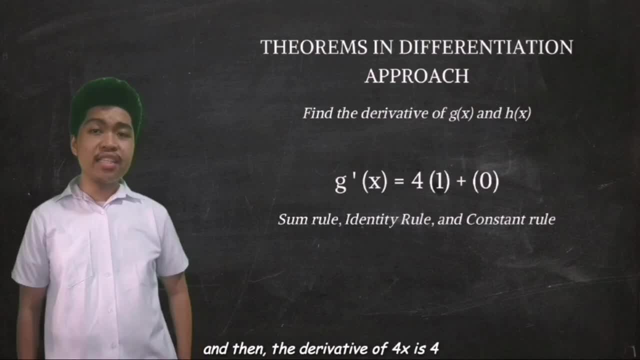 We applied the sum rule and then the derivative of 4x is 4, since we all know that, according to the identity rule, the derivative of x is 1.. And the 8 becomes 0 because of the constant rule. So g. prime of x. 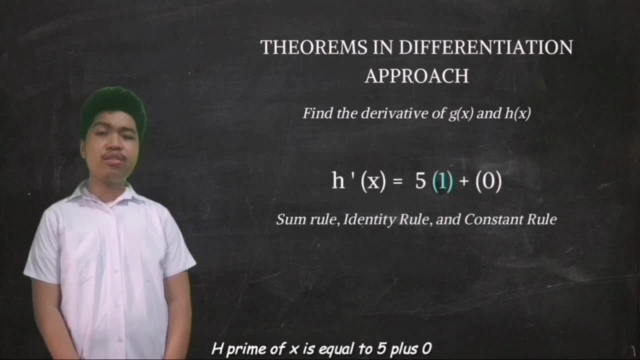 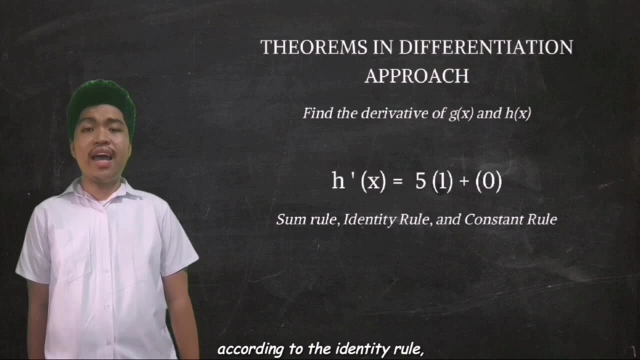 g prime of x is equal to 5 times 1 plus 0.. We applied the sum rule and, just like what I said earlier, according to the identity rule, the derivative of 5x is 5, since the derivative of x is 1.. 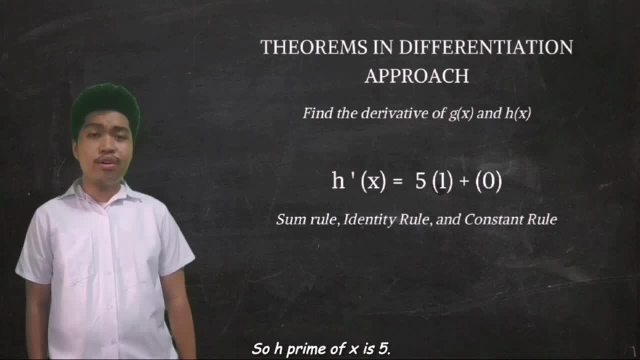 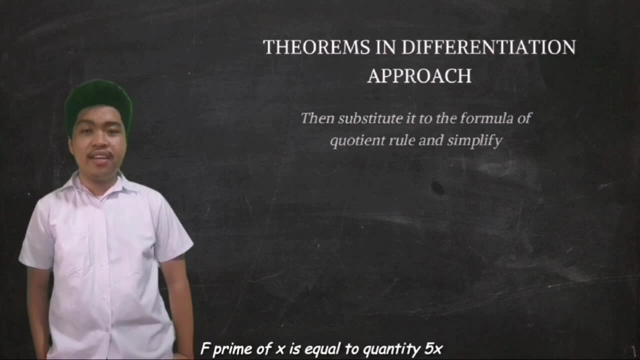 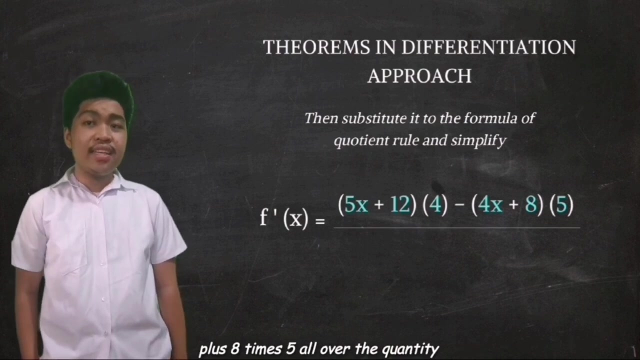 And the 12 becomes 0 due to the constant rule. So h prime of x is 5.. After that we will just substitute the values we got and then simplify. f prime of x is equal to quantity 5x Well times 4 minus quantity 4x plus 8 times 5, all over the quantity of 5x plus 12 squared. 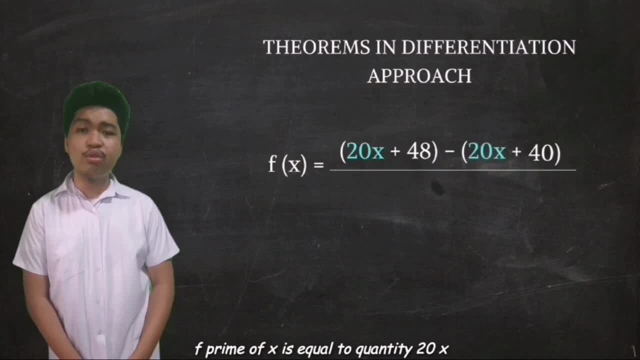 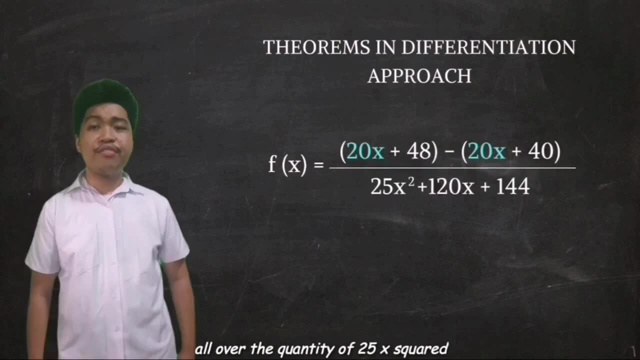 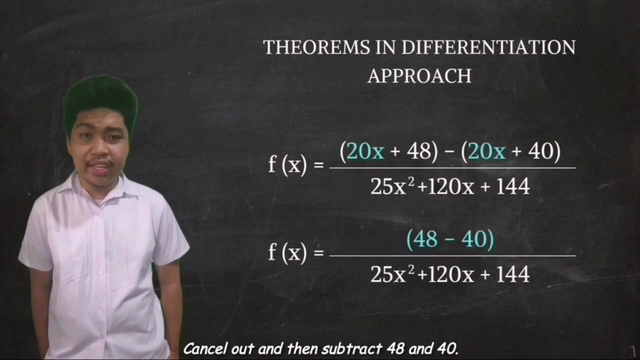 By further simplifying f. prime of x is equal to quantity 20x plus 48, minus quantity 20x plus 40, all over the quantity of 25x squared plus 120x plus 144.. Cancel out and then subtract 48 and 40.. 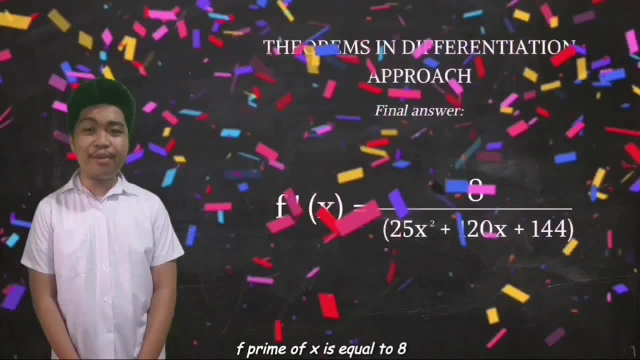 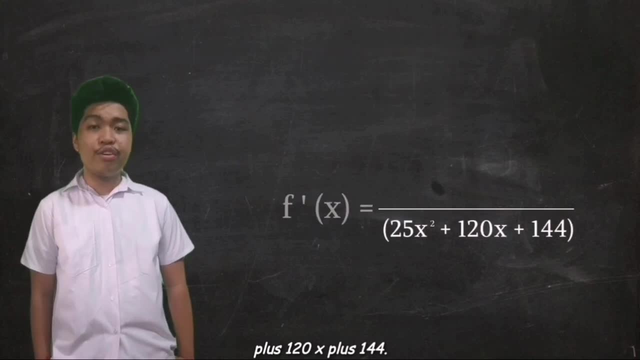 And ta-da, Here's our final Answer: f prime of x is equal to 8, all over the quantity of 25x squared plus 120x plus 144.. As you can see, using differentiation theorems is much faster than using the increment method. 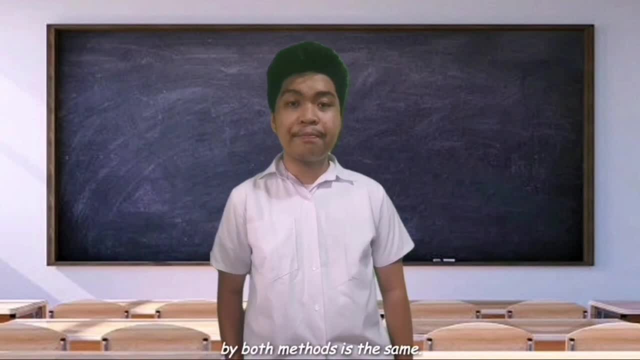 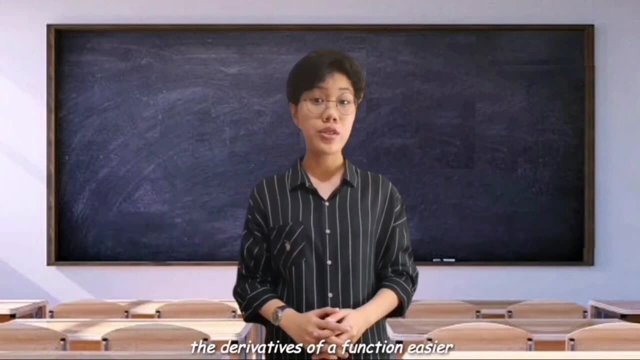 And still the derivative obtained by both methods is the same. The theorems on differentiation are the rules that allow us to find the derivatives of a function easier than when we use the definition of a derivative, which makes even the simplest of functions longer to solve. 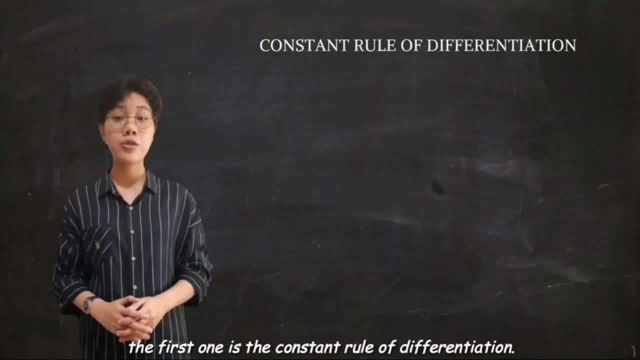 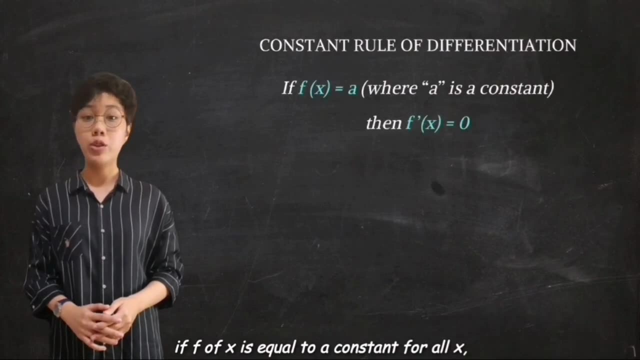 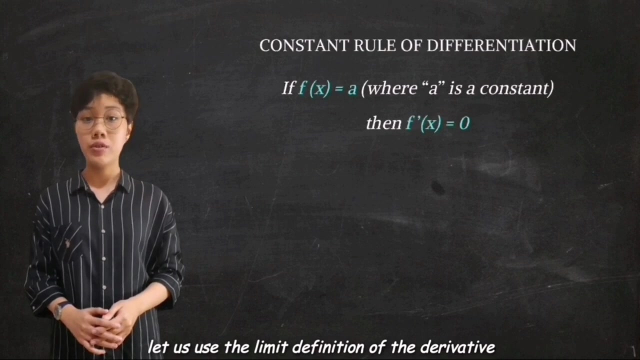 There are seven given differentiation rules. The first one is the constant rule of differentiation. In this theorem it is stated that if f of x is equal to a constant for all x, then f prime of x is equal to 0.. To prove this, let us use the limit definition of the derivative as a function of x. 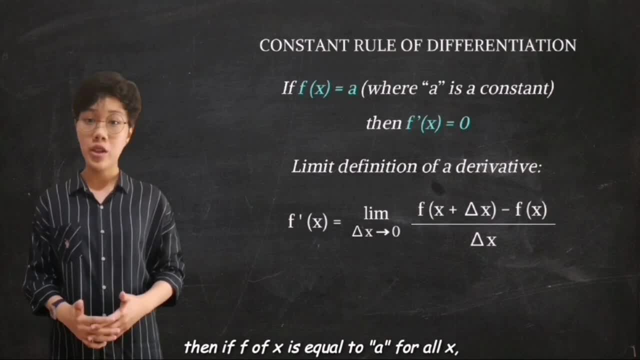 If we use a as our constant, then if f of x is equal to a for all x, f prime of x is the limit of f of x plus delta x, and f prime of x is the limit of f of x plus delta x. 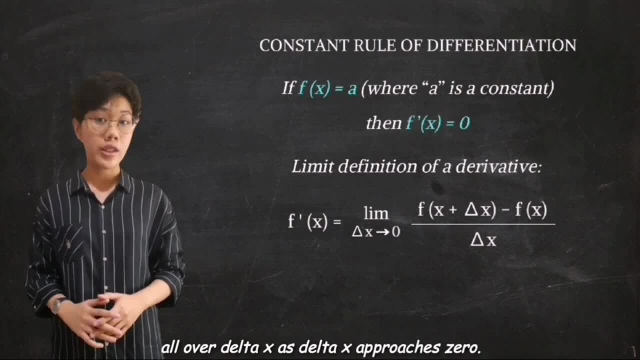 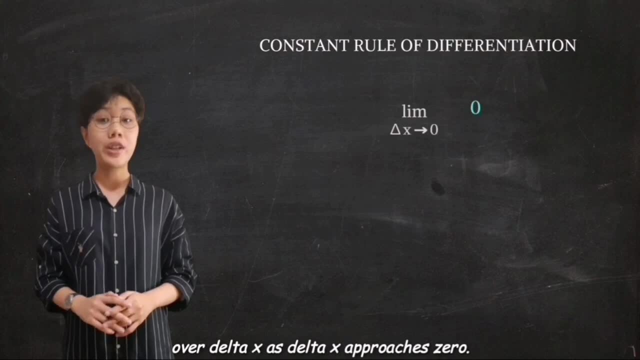 minus f of x all over delta x as delta x approaches 0.. a minus a is equal to 0.. We will then have the limit of 0 over delta x as delta x approaches 0.. By simplifying this, we will have: f of x is equal to 0. 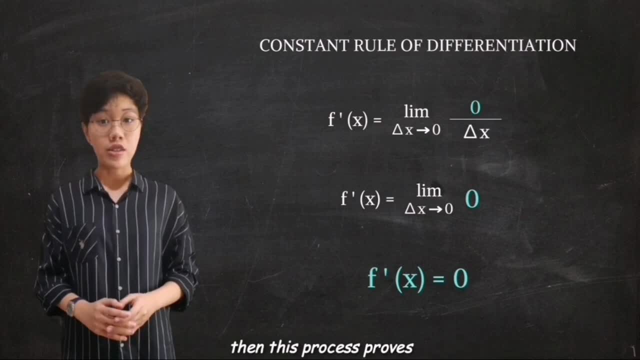 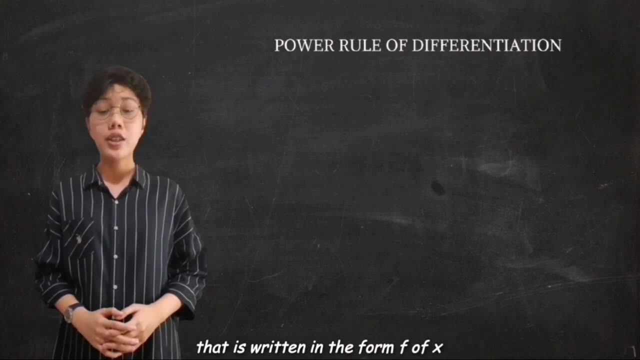 And since the derivative of any constant is equal to 0,, then this process proves the constant rule of differentiation. The second theorem is the power rule of differentiation. that is written in the form: f of x is equal to x raised to n, where n is a constant and a natural number. 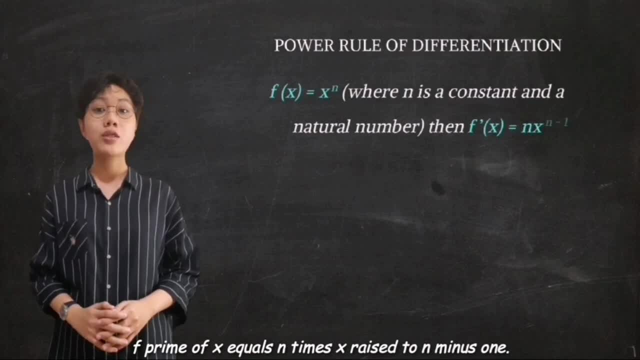 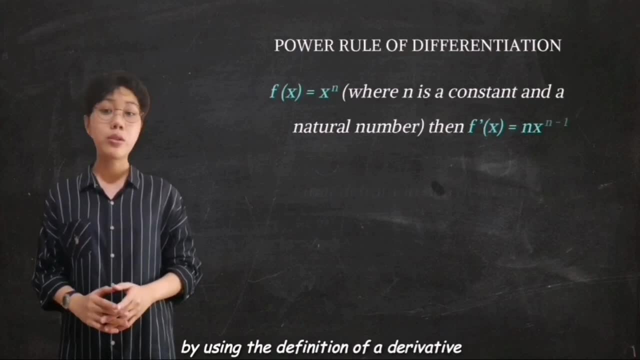 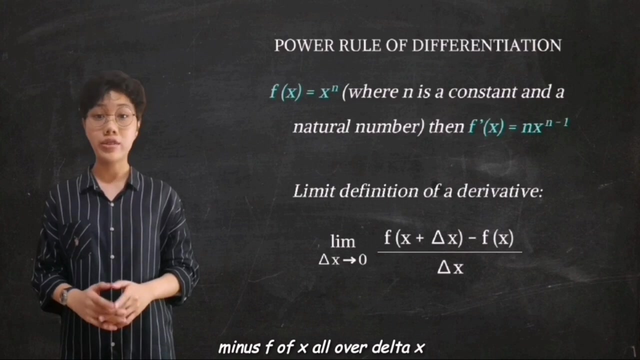 then its derivative will be: f prime of x equals n times x raised to n minus 1.. We need to show that the first derivative is n times x raised to n minus 1 by using the definition of a derivative in the form: the limit of f of x plus delta x minus f of x, all over delta x as delta x approaches 0.. 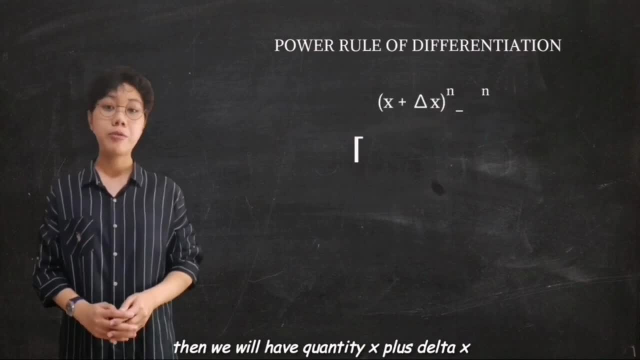 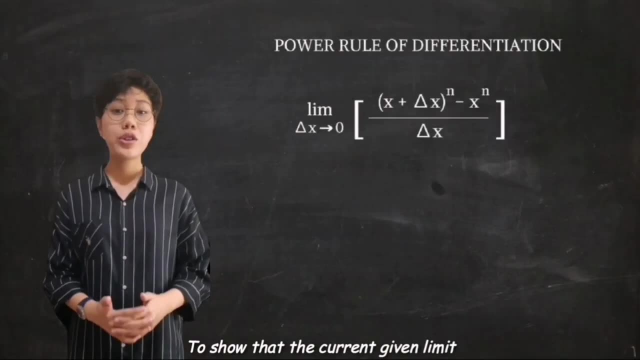 Since f of x is equal to x raised to n, then we will have quantity x plus delta x raised to n minus x raised to n, all over delta x, To show that the current given limit is equal to n times x raised to n minus 1,. 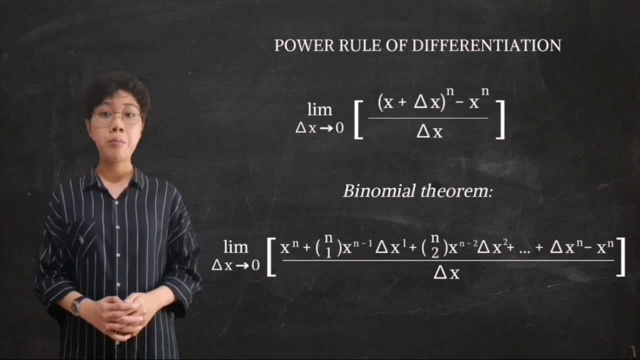 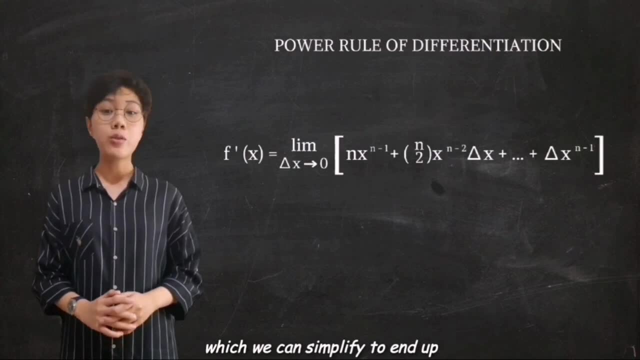 we will use the binomial theorem Now. we will let n be in the set of natural numbers, and by doing that we will be left with this form of the binomial theorem, which we can simplify to end up with n times x, raised to n minus 1.. 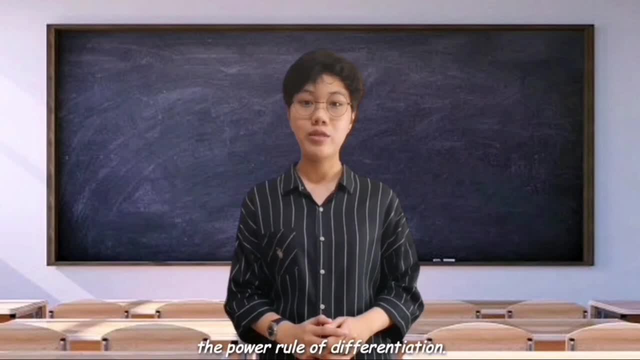 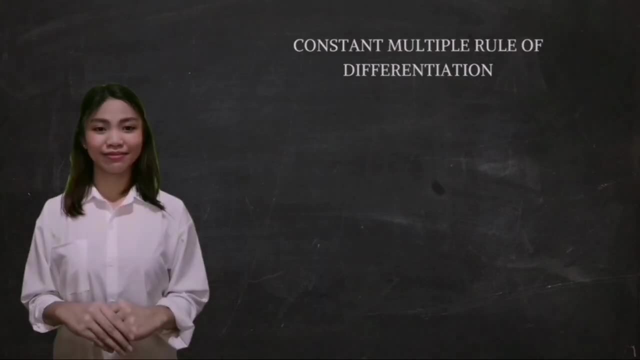 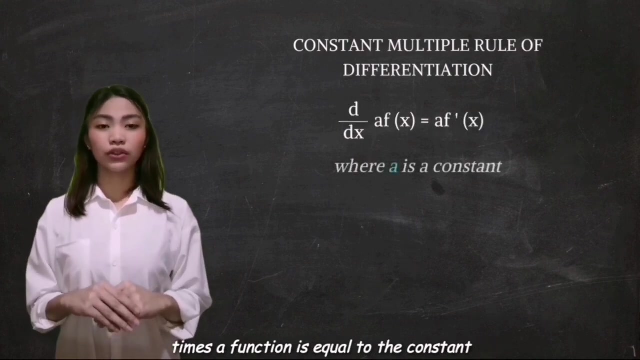 This proves the limited form of the power rule of differentiation For the third theorem, the constant multiple rule of differentiation. This rule states that the derivative of a constant times a function is equal to the constant times, the derivative of a function, By using the definition of the derivative in the given form. 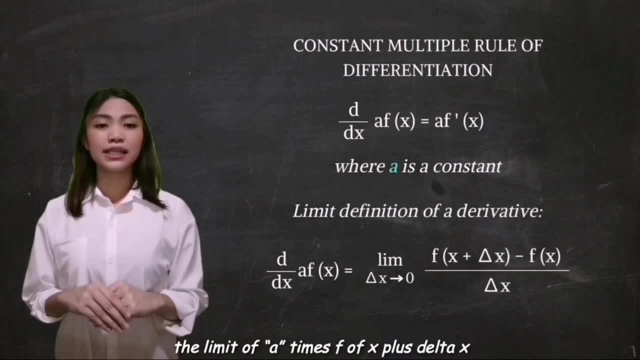 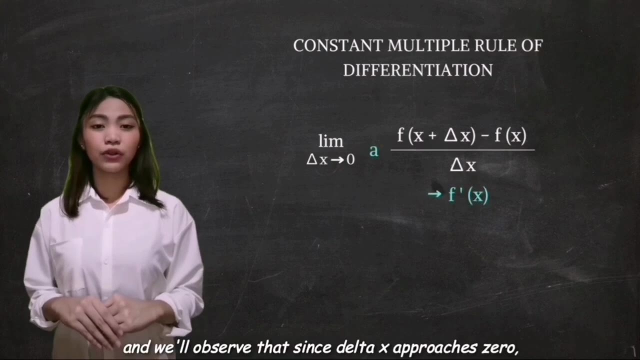 the limit of a times f of x plus delta x, minus a times f of x, all over delta x, as delta x approaches to 0.. Now we will factor out our constant from the yantar fraction and we will observe that since delta x approaches 0,. 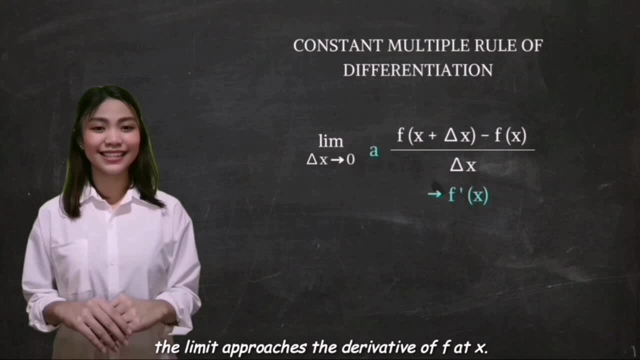 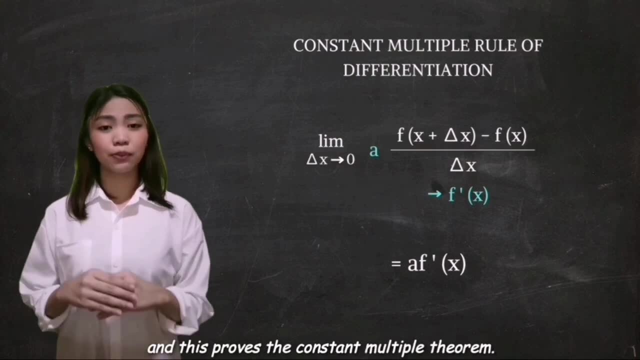 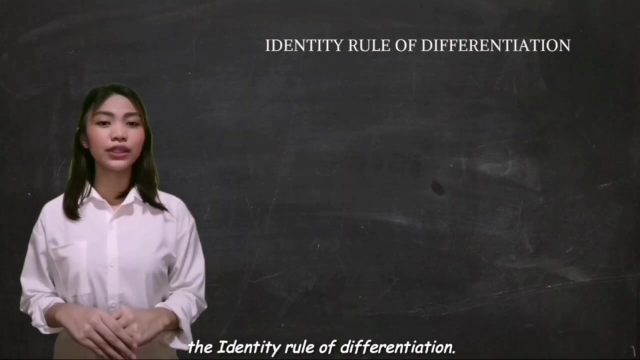 the limit approaches the derivative of f at x, And now we are left with our constant a times f prime of x, and this proves the constant multiple theorem. The fourth theorem is the identification of a constant times a function. The third theorem is the identity rule of differentiation. 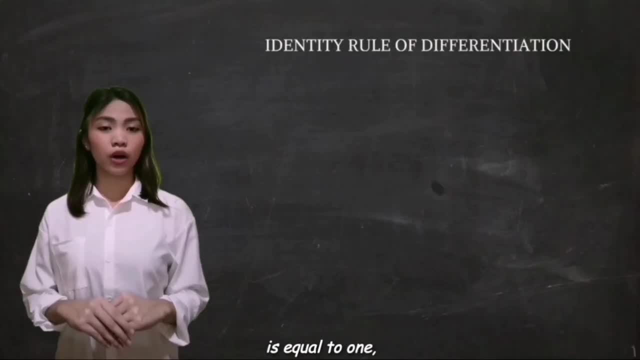 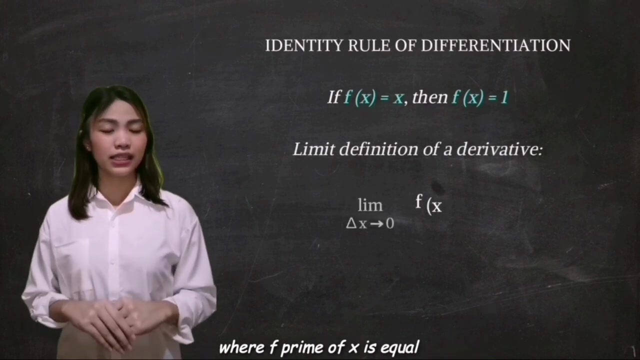 This means that the derivative of a function is equal to 1.. So if we have a function with x as an input, we should also have it as its output. To prove this, we will be using the definition of derivative, where f prime of x is equal to the limit of f of x plus delta x minus f of x. 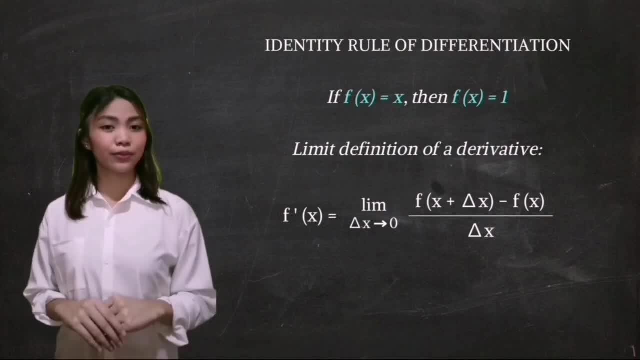 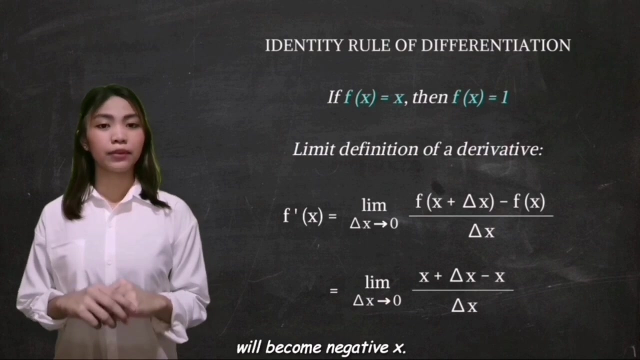 all over delta x as delta x approaches to 0. Again, the input of a function is the same as the output. Therefore, the f of x plus delta x will become x plus delta x, and negative f of x will become negative x. 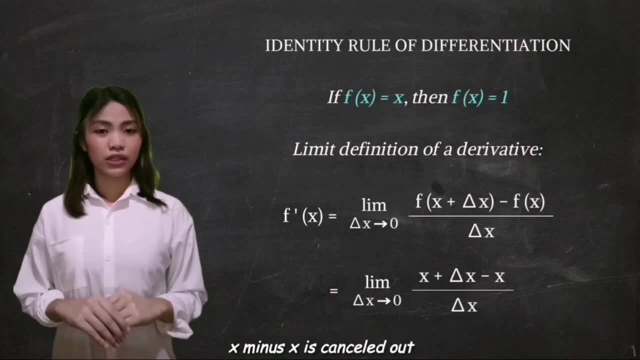 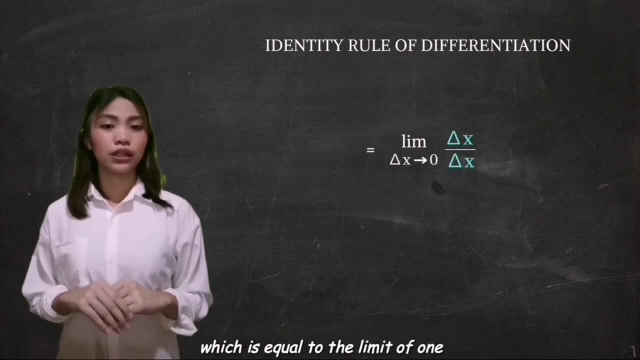 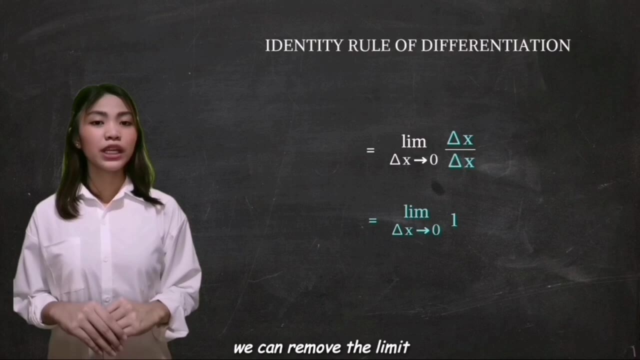 By simplifying this, x minus x is cancelled out and we are left with delta x divided by delta x, which is equal to the limit of 1, as delta x approaches 0.. Since delta x became 1, we can now remove the limit. 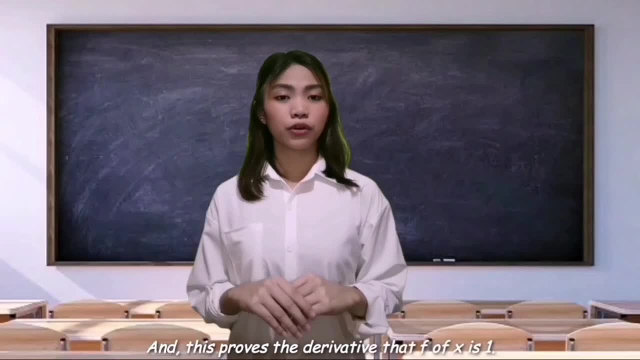 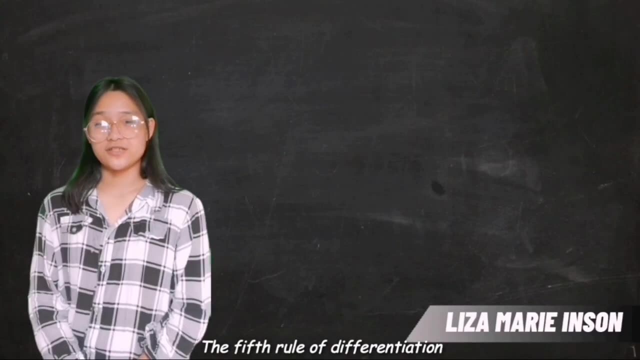 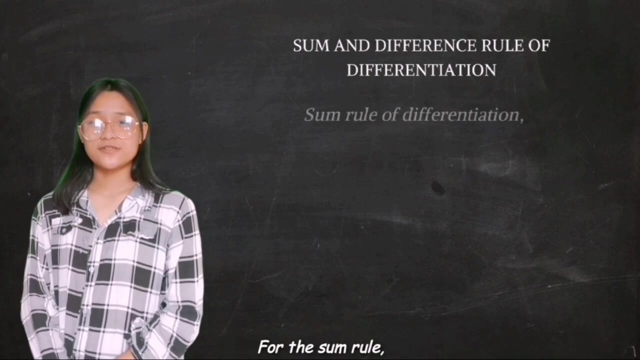 and so our final answer is 1.. And this proves that the derivative that f of x is 1.. The fifth rule of differentiation is the sum and difference rule. The first one is the sum rule of differentiation, For the sum rule, the derivative of the sum of the two functions. 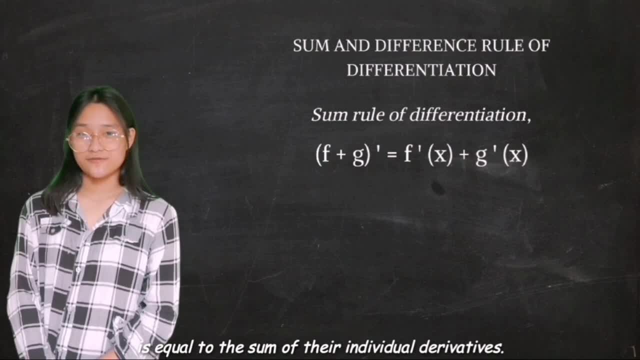 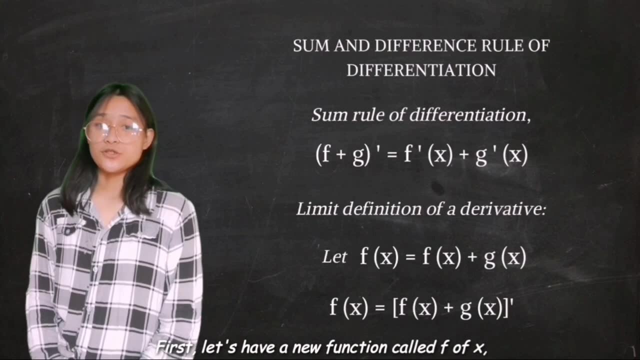 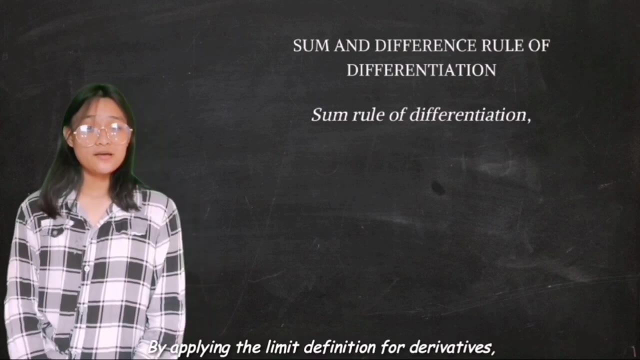 is equal to the sum of their individual derivatives. We can prove this by using the limit definition for derivatives. First, let's have a new function called the f of x, which is equal to the sum of the given individual functions. Second, by applying the limit definition for derivatives. 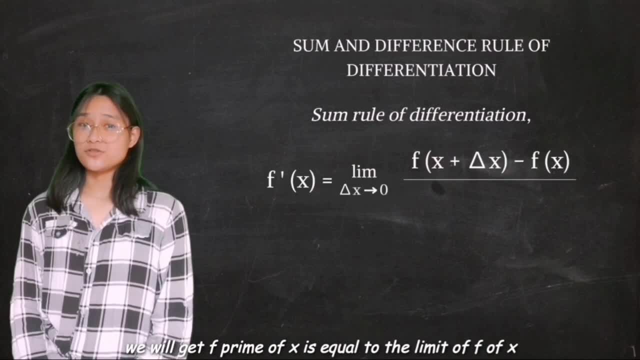 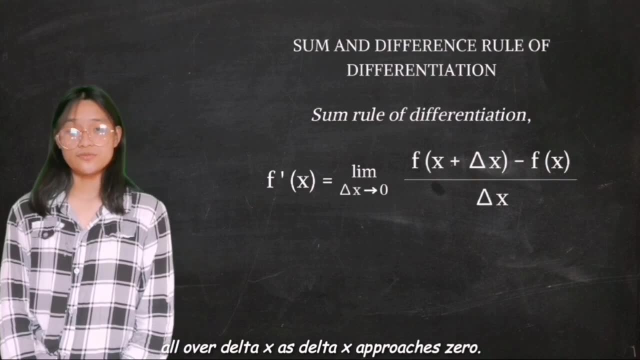 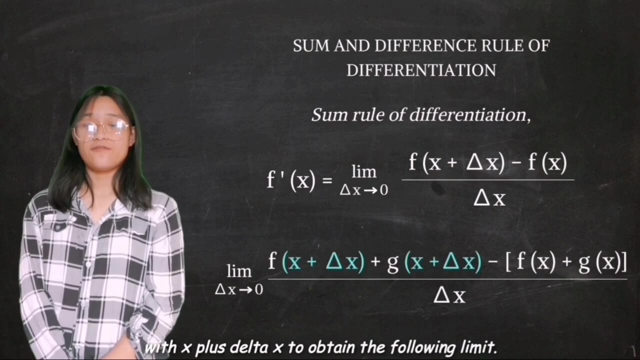 we will get f. prime of x equals to the limit of f of x plus delta x, minus f of x, all over delta x as delta x approaches to 0.. Third, we will simply replace x with x plus delta x to obtain the following limit: 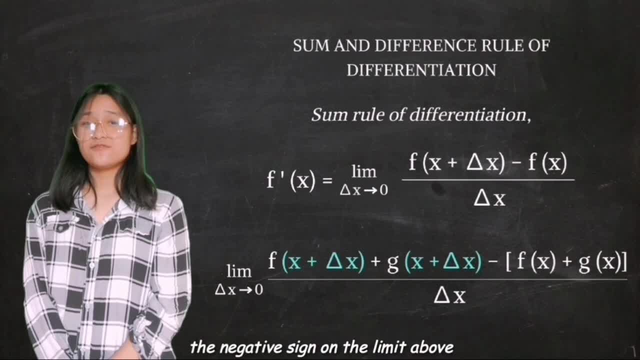 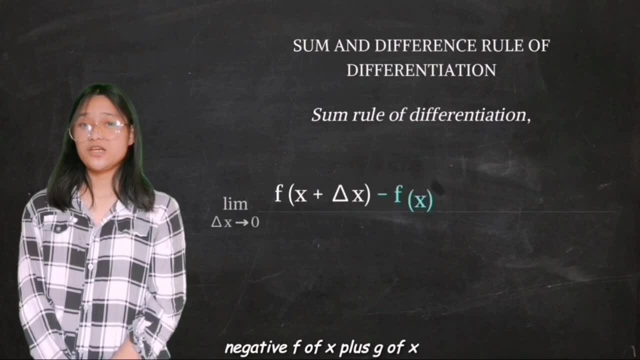 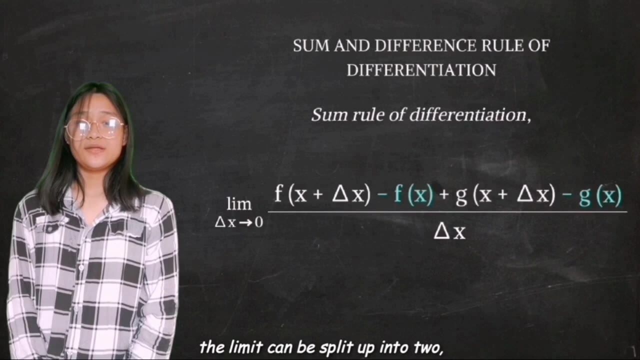 For the fourth step, the negative sign on the limit of all will be applied on both terms, and so negative f of x plus g of x will become negative f of x and negative g of x. Lastly, as you can observe, the limit can be split up into two. 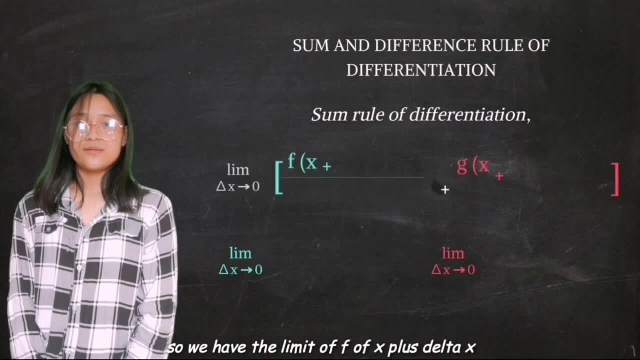 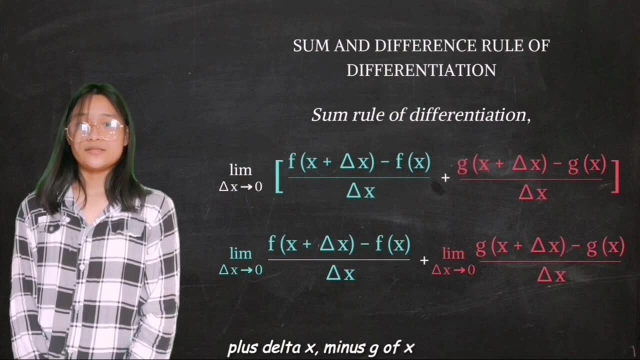 So we have the limit of f of x plus g of x, the limit of f of x plus delta x, minus f of x, all over delta x, as delta x approaches to 0, plus g of x plus delta x, minus g of x, all over delta x as delta x approaches to 0. 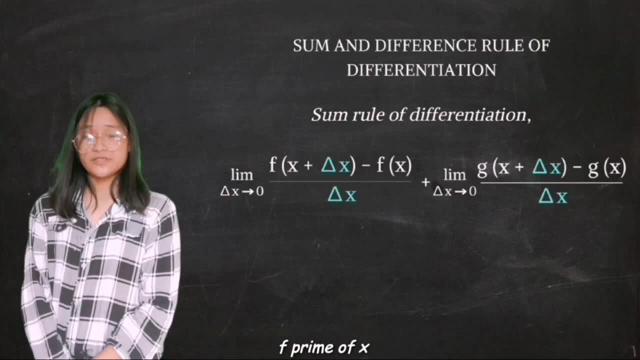 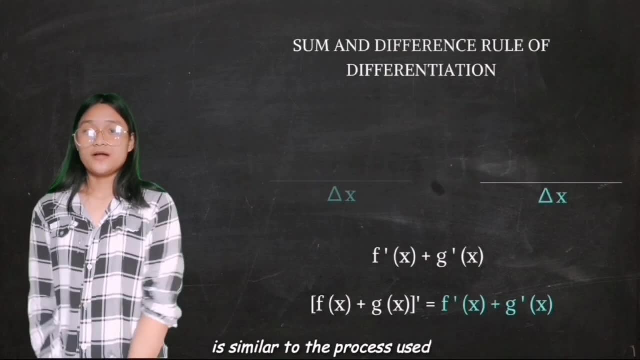 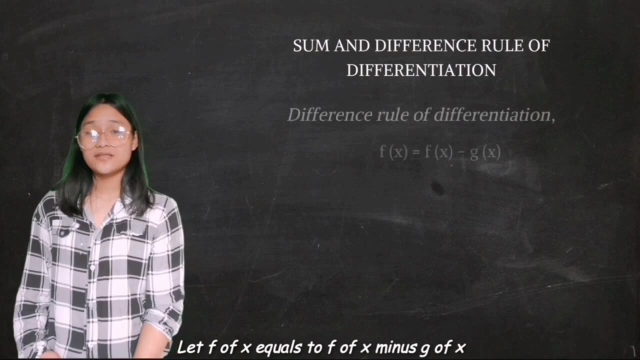 Simplify the limit of f and g: f prime of x plus g prime of x, and that's the sum of the derivative. The process of proving the sum rule is similar to the process used in proving the difference rule. Let f of x equal to f of x minus g of x. 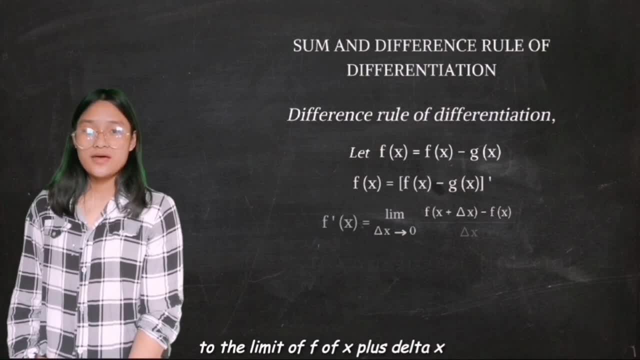 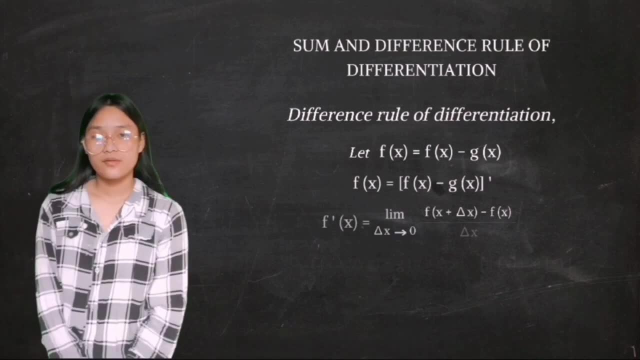 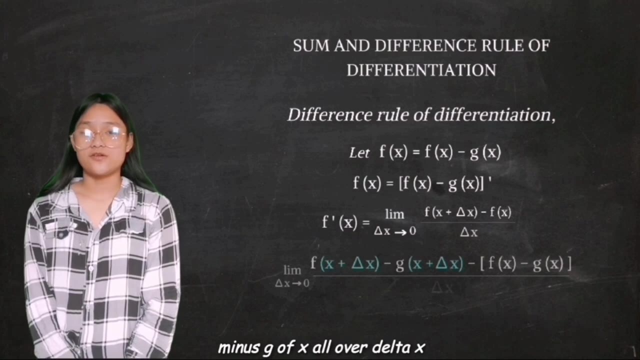 Therefore, f prime of x is equal to limit of f of x plus delta x minus f of x all over delta x as delta x approaches to 0.. The limit of f of x minus g of x plus delta x minus f of x minus g of x all over delta x as delta x approaches to 0. 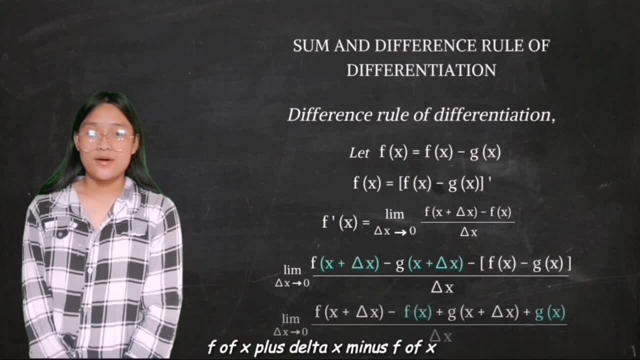 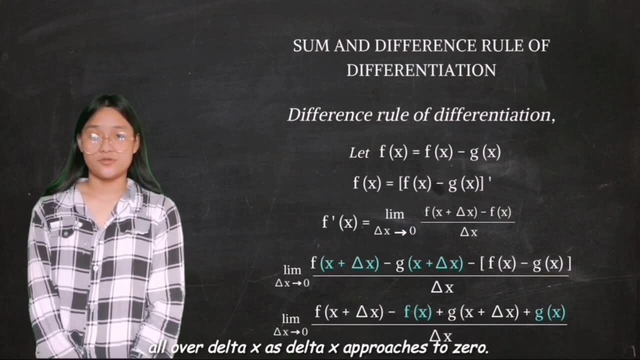 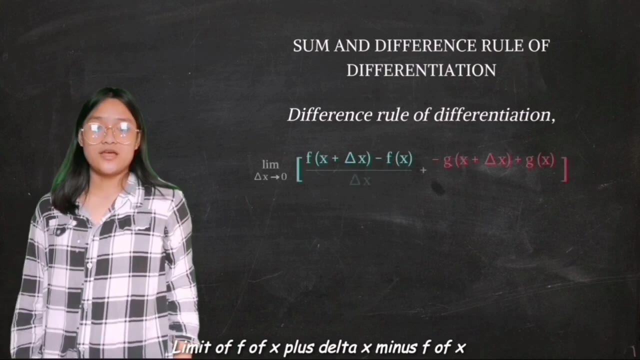 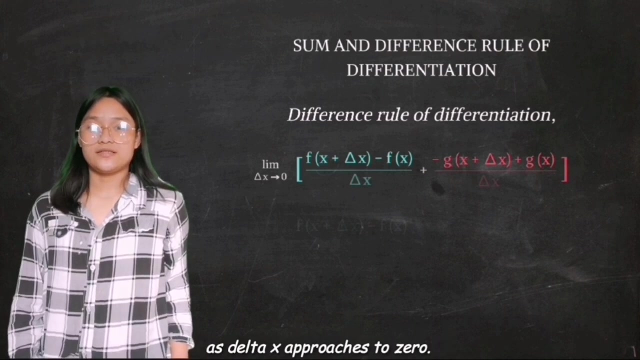 can be written as limit of f of x plus delta x minus f of x plus g of x plus delta x plus g of x all over delta x, as delta x approaches to 0.. It can be written as limit of f of x plus delta x minus f of x all over delta x minus g of x plus delta x plus g of x all over delta x, as delta x approaches to 0. 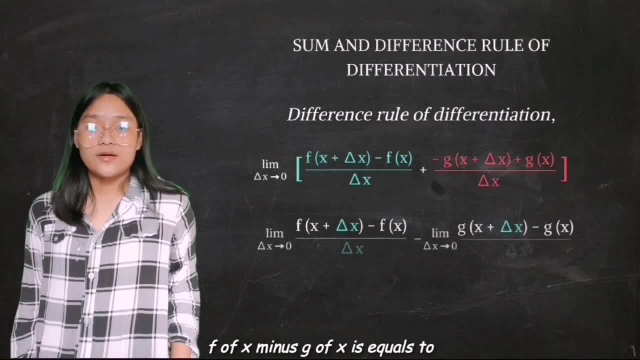 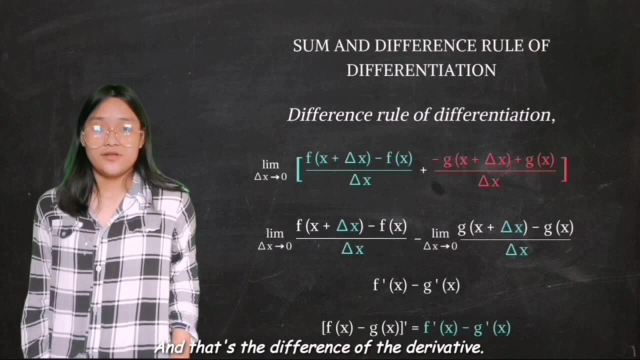 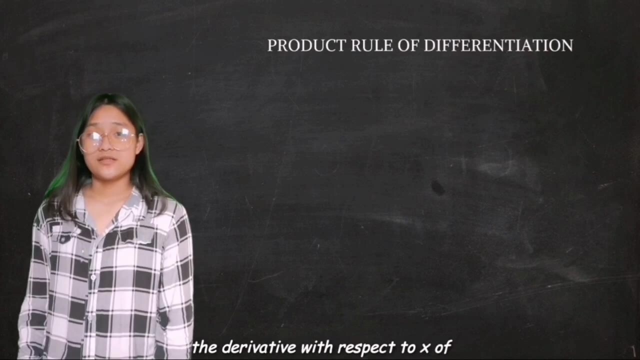 We can simplify it and we can get: f of x minus g of x is equal to f prime of x minus g prime of x, and that's the difference of the derivatives. The product rule is the sixth theorem of differentiation that sets the derivative, with respect to x, of the product of two functions. 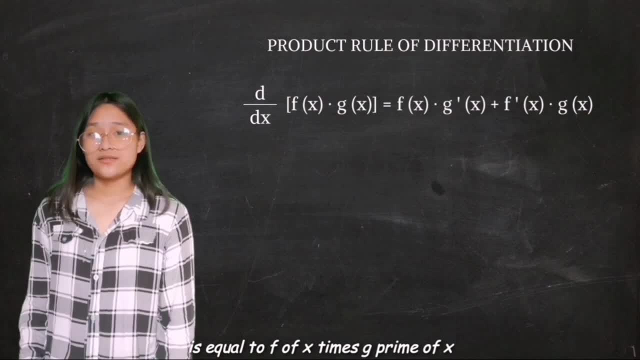 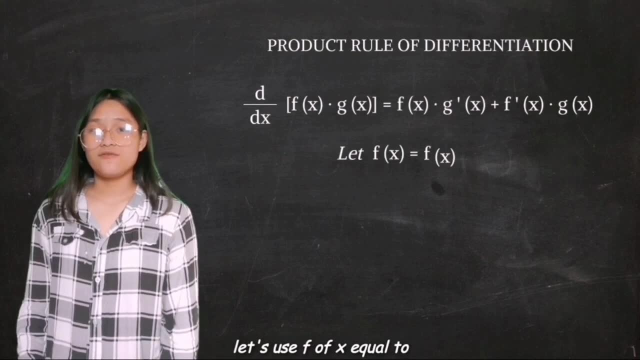 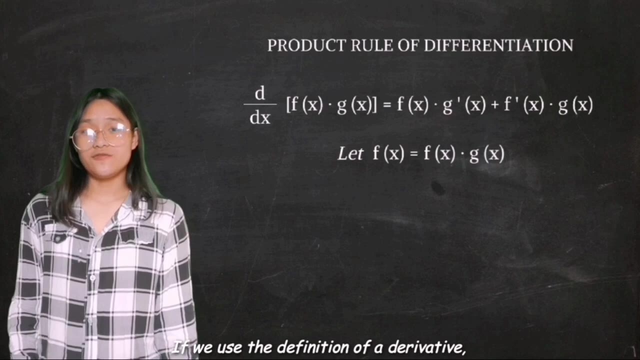 f of x times g of x is equal to f of x times g prime of x, plus prime of x times g of x. To prove this, let's use: f of x equals to the product of f of x times g of x If we use the definition of a derivative. 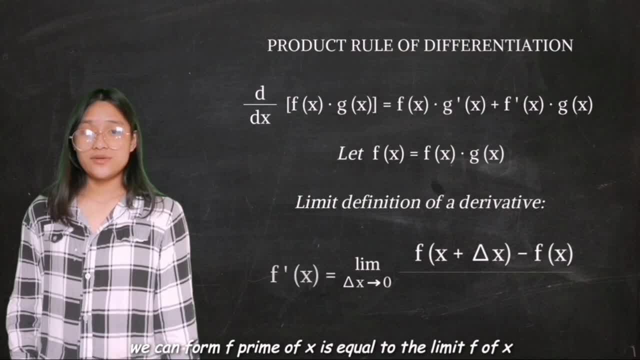 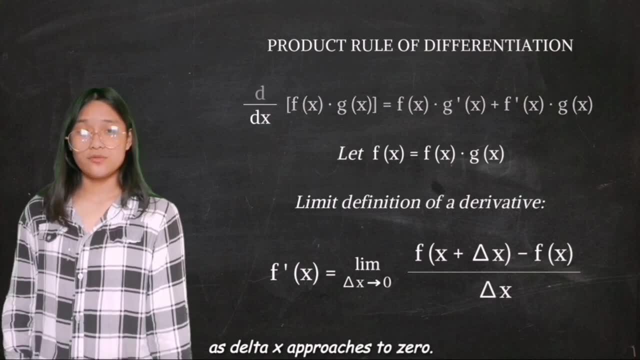 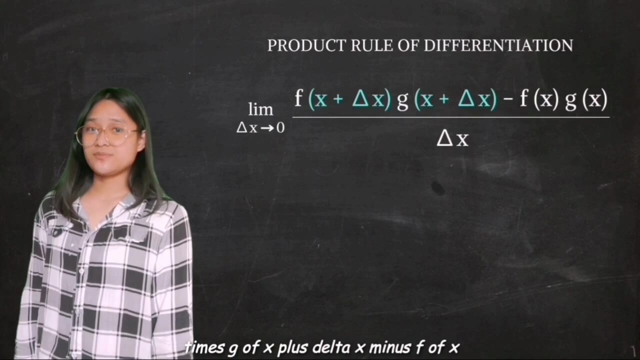 we can form f prime of x is equal to the limit of f of x plus delta x minus f of x, all over delta x as delta x approaches to 0.. We can replace the f of x function to get the limit of f of x plus delta x times g of x plus delta x minus f of x times g of x. 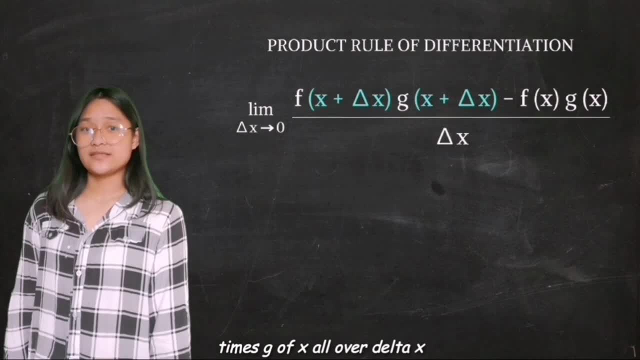 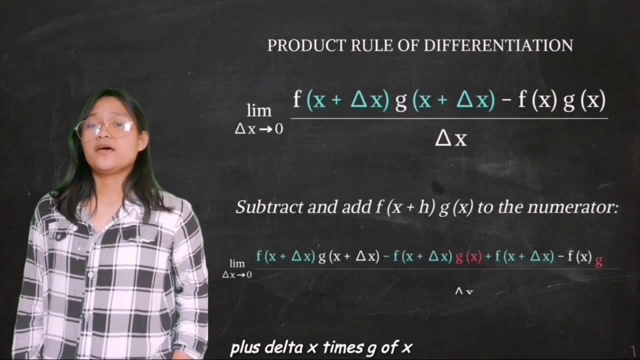 delta x minus f of x times g of x all over delta x as delta x approaches to zero. For the next step, we're going to subtract and add the term f of x plus delta x times g of x to the numerator, which will give us the following limit: 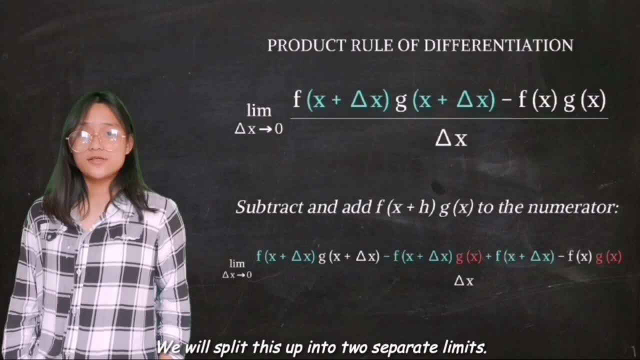 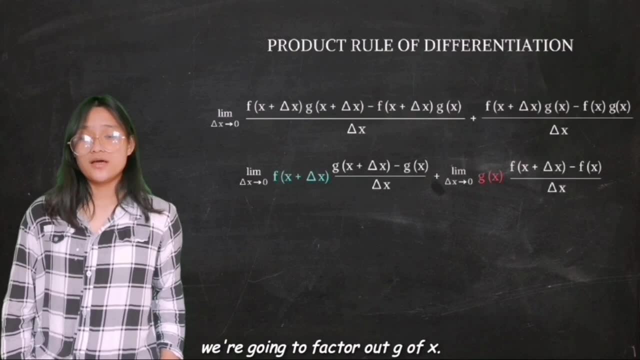 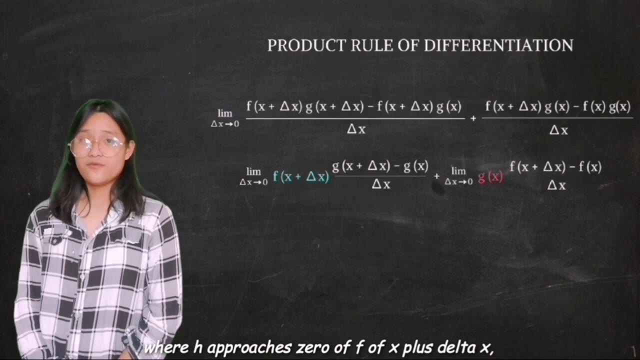 We will split this up into two separate limits. In the first limit we're going to factor out f of x plus delta x, and for the second limit, we're going to factor out g of x. Let's note that in the first limit, where h approaches zero of f of x plus delta x. 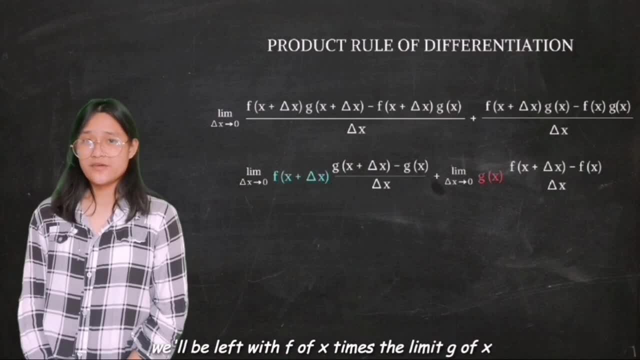 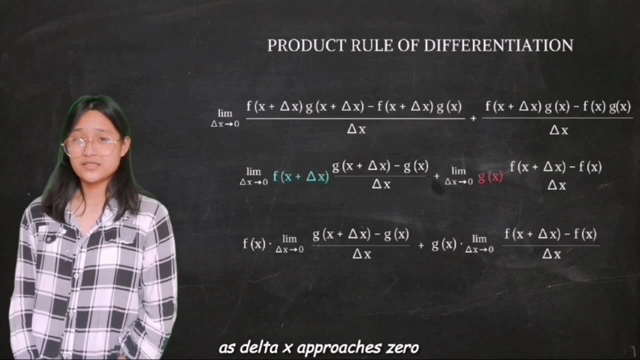 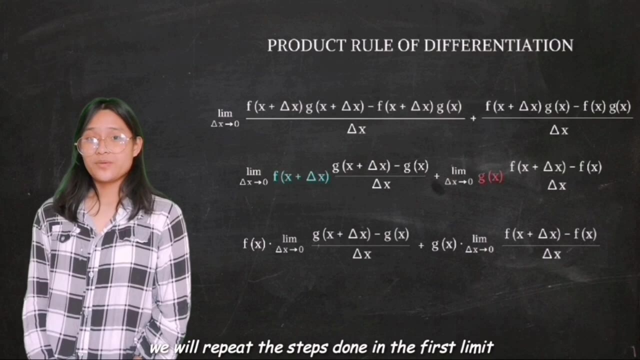 if we substitute in delta x equals zero, we'll be left with f of x, times limit of g of x plus delta x minus g of x, all over delta x as delta x approaches to zero. And for the second limit, where delta x approaches to zero of g of x, we will repeat the steps. 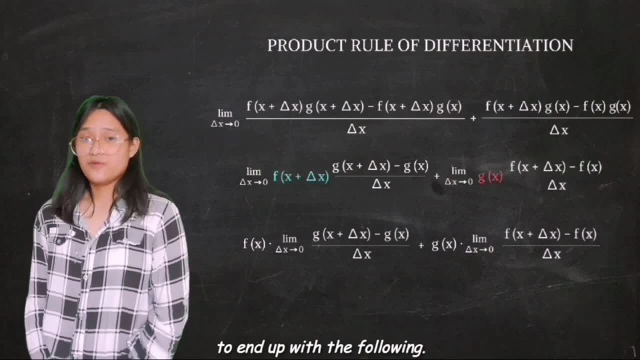 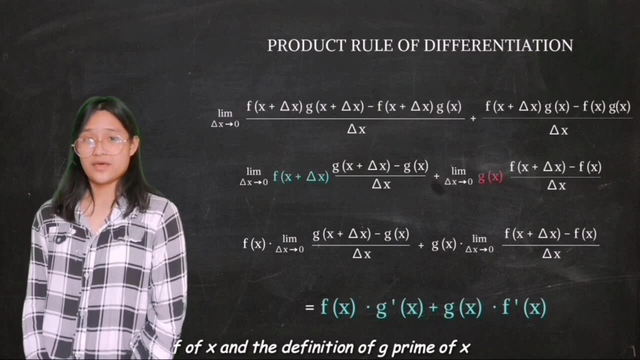 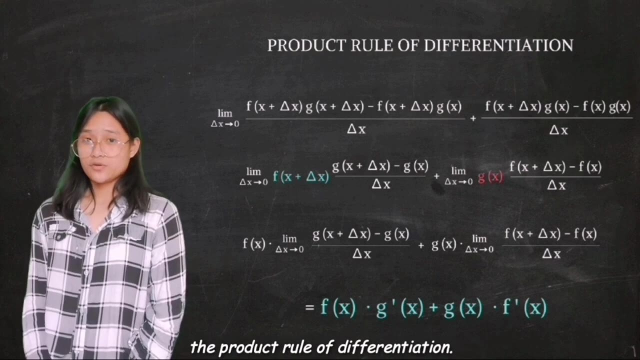 done in the first limit to end up with the following: If we simplify this, we'll get the following: We will get f of x and the definition of g prime of x, plus g of x and the definition of f prime of x, which completes the proof of the product rule of differentiation. 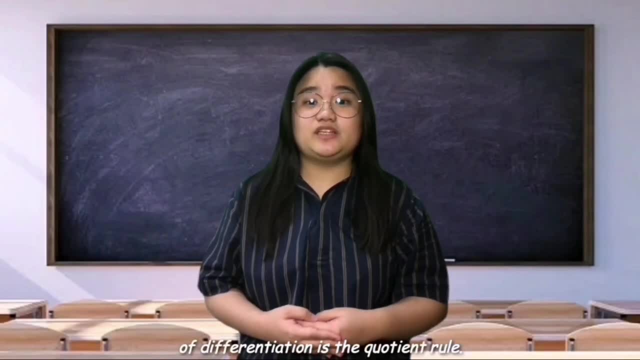 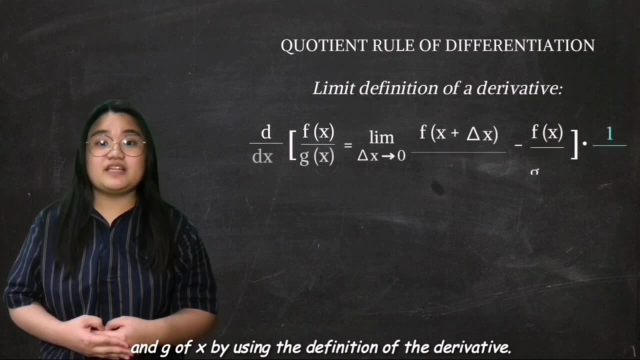 The seventh and last theorem of differentiation is the quotient rule. To prove this theorem, we find the derivative of the quotient between f of x and g of x by using the definition of the derivative. Instead of dividing this limit by delta x, we multiply it by the derivative of delta. 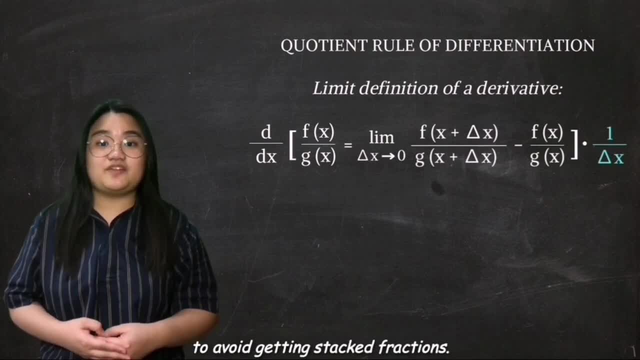 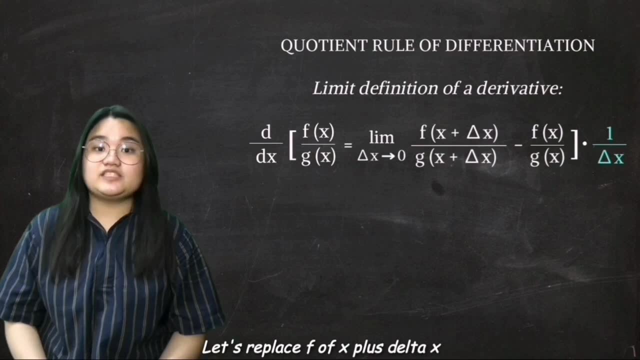 x. We can simply multiply this by one over delta x to avoid getting stacked fractions. After this, we will follow a step similar to how we prove the product rule. Let's replace f of x plus delta x by the value of the function at x plus the appropriate. 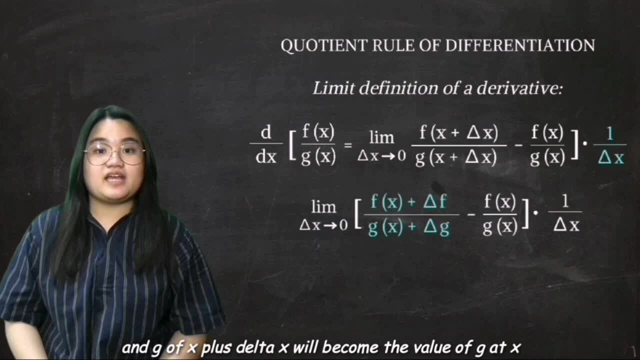 change in the function And g of x plus delta. x will become the value of g at x plus the appropriate change in the function g. In the next step we will be cross multiplying to combine the separated fractions. After this we will follow a step similar to how we proved the product rule. 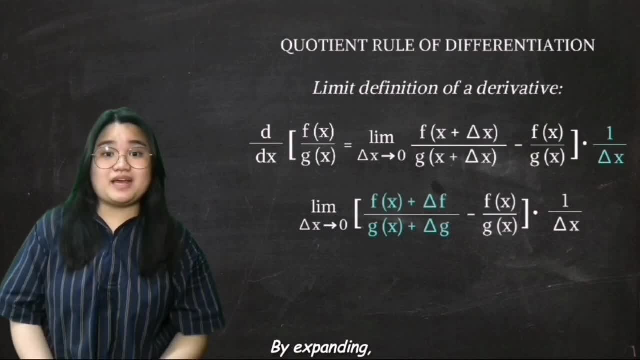 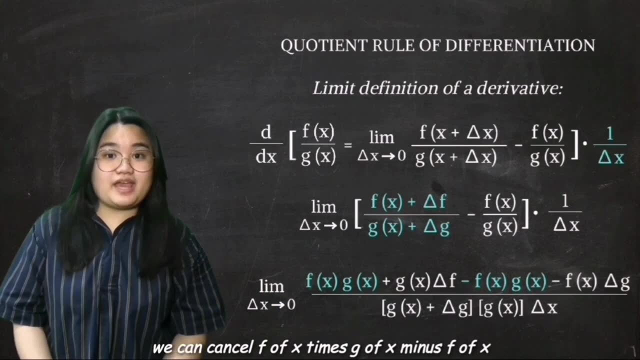 As a result, we will have the values of f of x plus delta x plus the value of the function g. By expanding we will obtain the following: If we observe the numerator, we can cancel f of x times g of x, minus f of x times g of x. then we will be left. 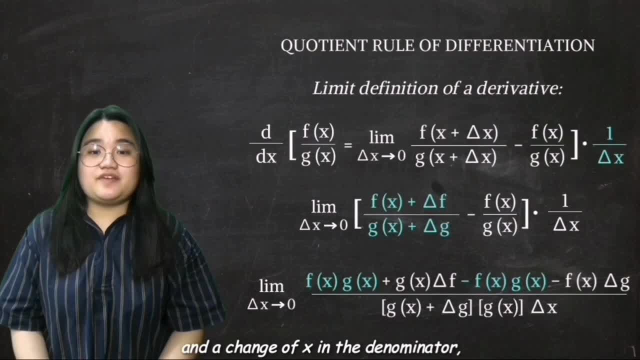 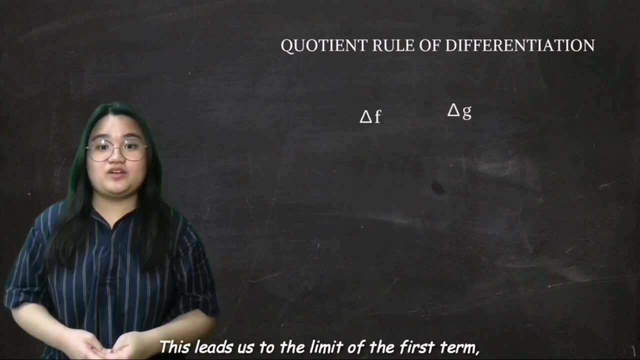 with a change of f and g in the numerator and a change of x in the denominator, which we can pair with delta x and factor out. This leads us to the limit of the first term, g of x times delta f over delta x minus the second. 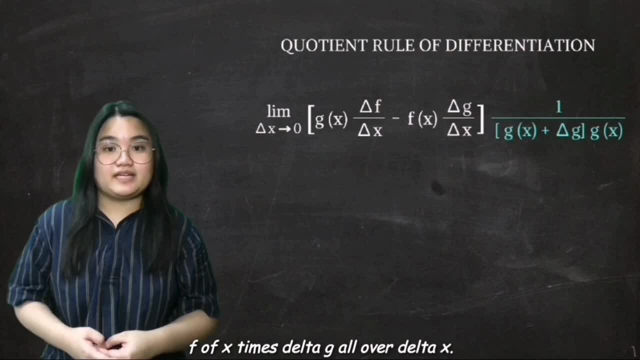 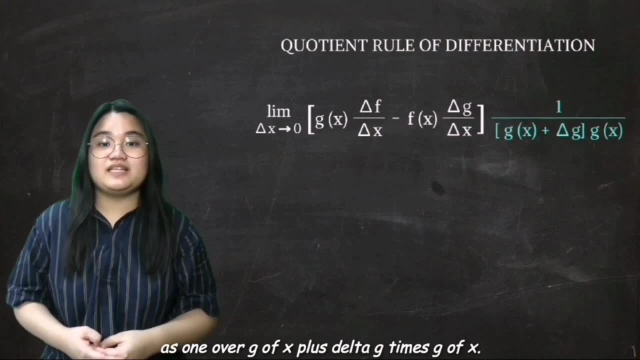 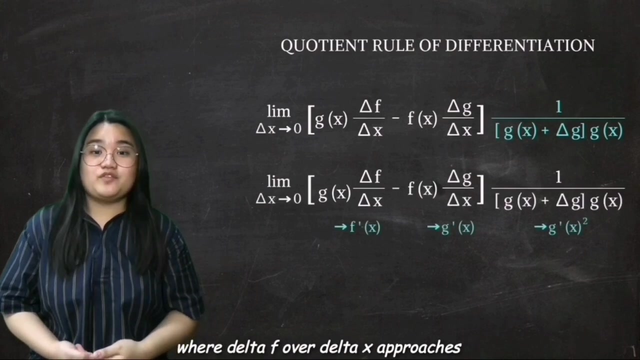 term f of x times delta g all over delta x. We'll also include the two terms left in the denominator and factor them out as 1 over g of x, plus delta g times g of x. By doing this, delta x can approach 0. where delta f over delta x. 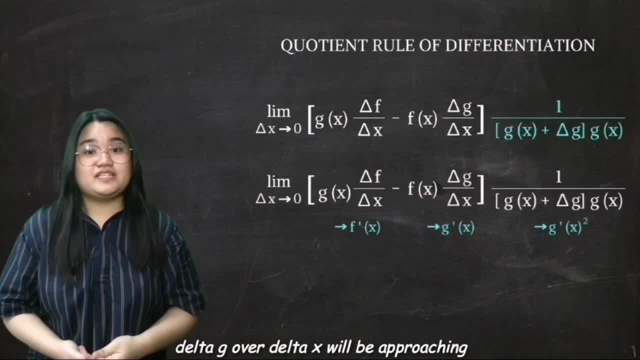 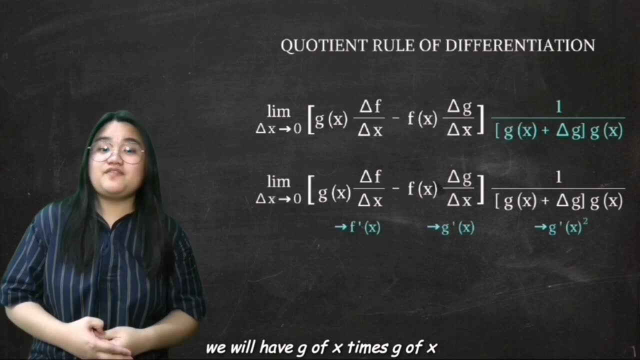 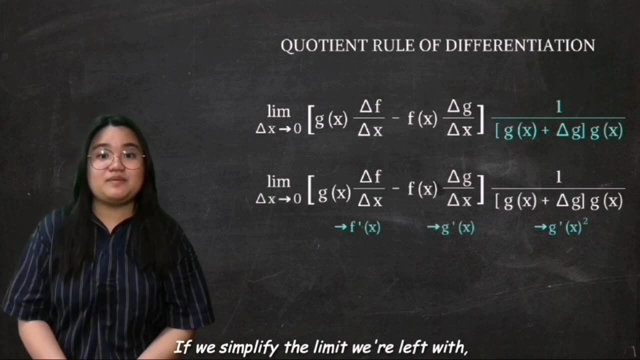 approaches the derivative of f at x, delta g over delta x will be approaching the derivative of g at x, and since delta g approaches 0, we will have g of x times g of x x. therefore, we have g of x squared. if we simplify the limit we're left with, we will obtain f prime. 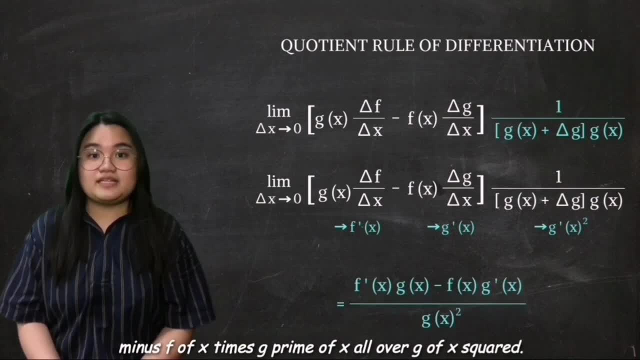 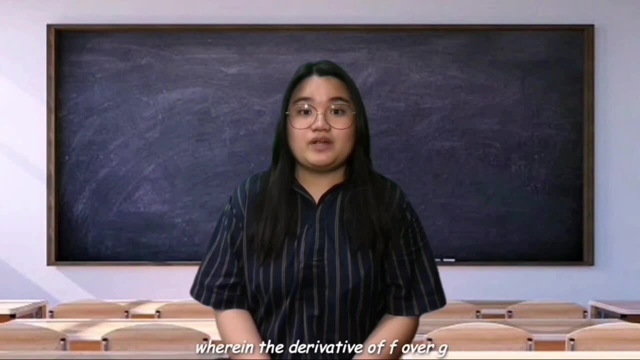 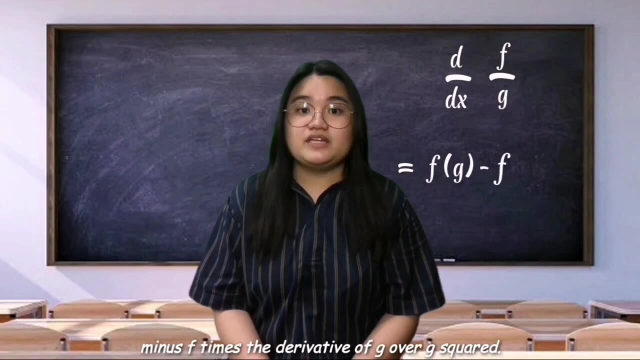 of x times g of x minus f, of x times g, prime of x all over g of x squared. this proves the quotient rule of differentiation, wherein the derivative of f over g is the derivative of f times g minus f times the derivative of g over g squared. one application of derivatives in real life is: 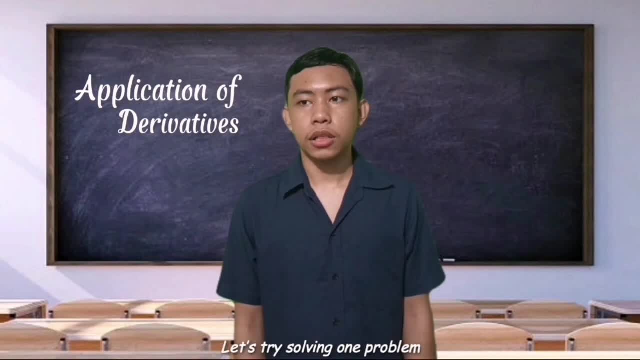 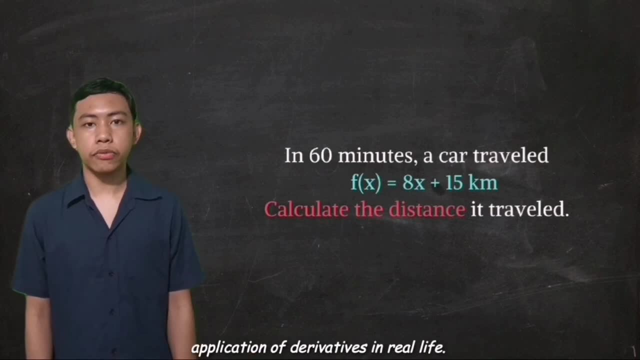 determining the speed or distance covered. let's try solving one problem including this application. so here's a sample problem providing an application of derivatives in real life. in 60 minutes, a car traveled f of x is equal to 8x plus 15 kilometers. calculate the distance. 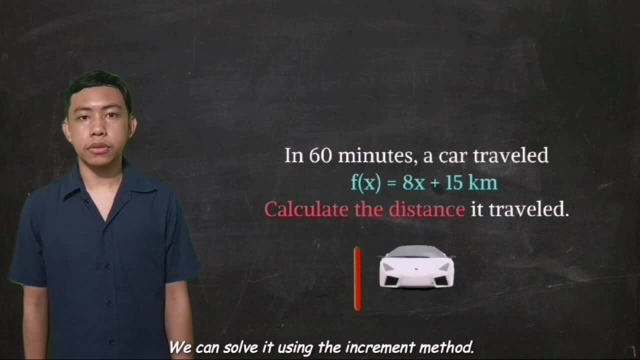 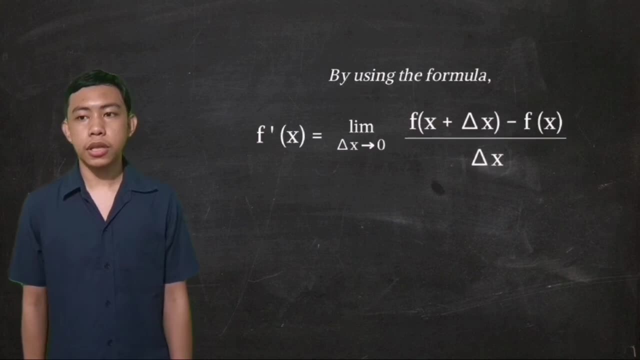 it traveled. we can solve it using the increment method by using formula 3: f prime of x is equal to the limit of f of x plus delta x minus f of x, all over delta x, as delta x approaches to 0.. let's now substitute x plus delta x in the x of the equation. 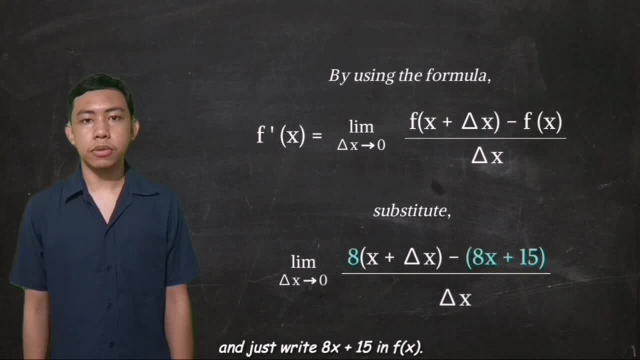 8x plus 15 and just write 8x plus 15 in f of x, we will have limit of 8 times the quantity x plus delta x plus 15, or 1 minus the quantity 8x plus 15, all over delta x as delta x approaches to 0.. 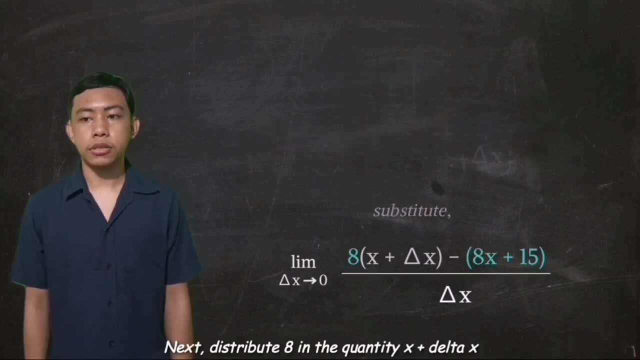 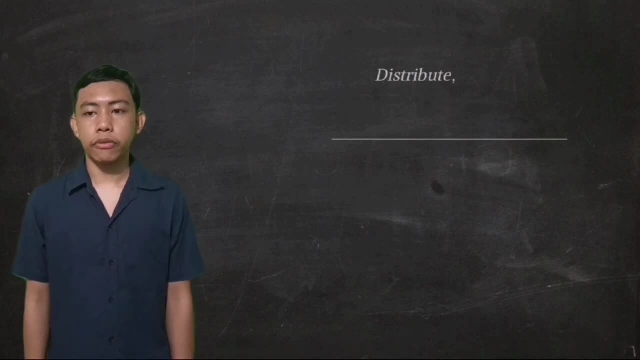 Next, distribute 8 in the quantity x plus delta x and distribute the negative sign in the quantity 8x plus 15.. We will have limit of 8x plus 8, delta x plus 15 minus 8x minus 15, all over delta x as. 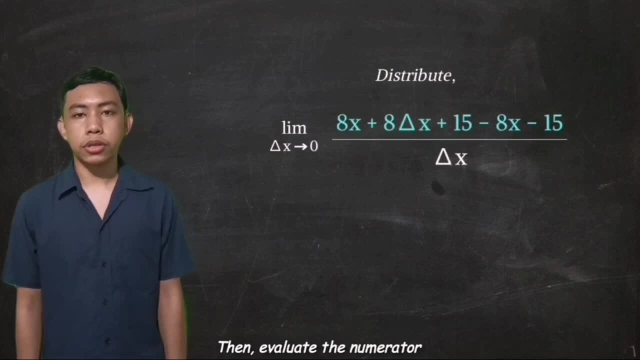 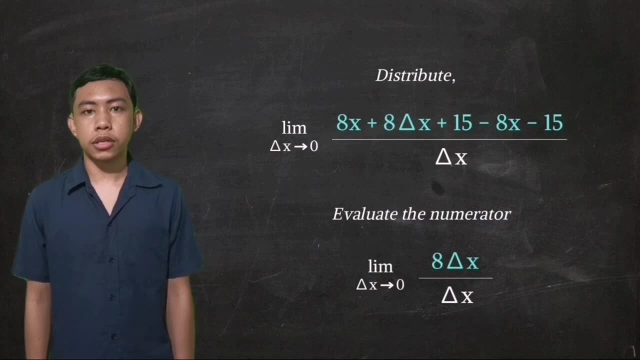 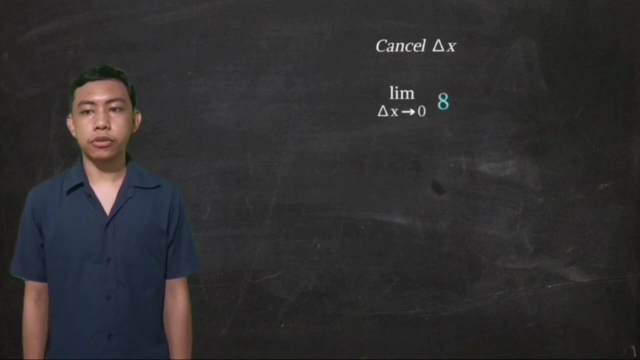 delta x approaches to 0.. Then evaluate the numerator. We will have limit of 8 delta x over delta x as delta x approaches to 0.. Cancel out delta x. We will have limit of 8 as delta x approaches to 0.. By limit theorem 2, we will have the answer. f. prime of x is equal to 8.. 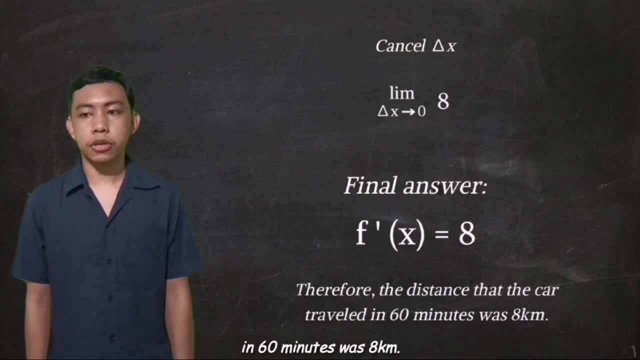 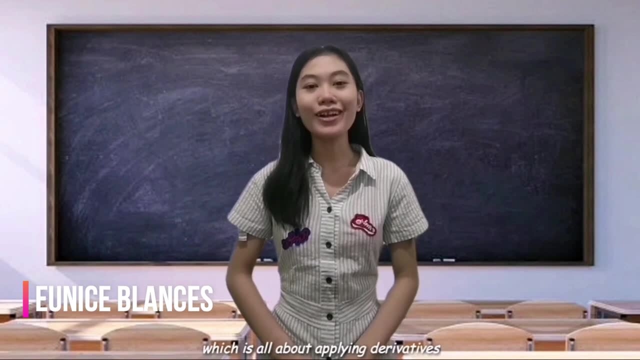 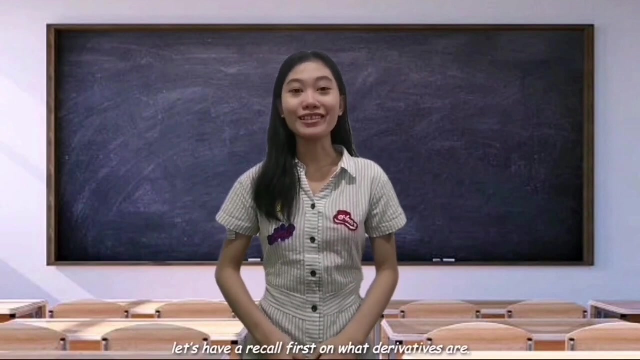 Therefore, the distance that the car traveled in 60 minutes was 8.. Hi, Welcome to this part of the video which is all about applying derivatives in real life, and I hope you enjoy it. Nevertheless, let's have a look at first on what derivatives are. 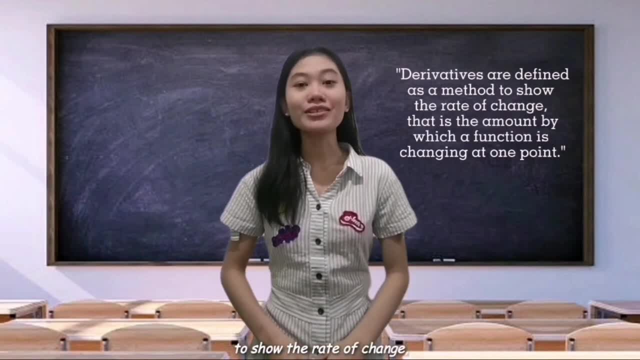 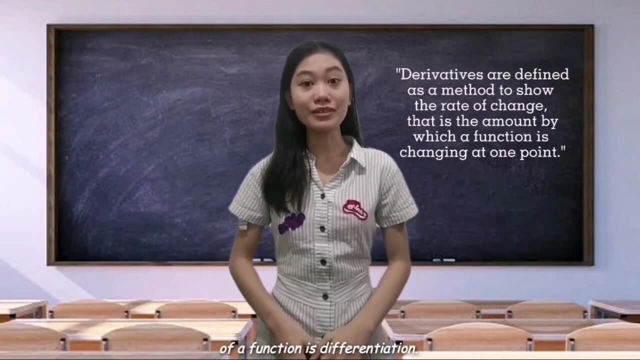 In mathematics, derivatives are defined as a method to show the rate of change, that is, the amount by which a function is changing at one point. The process of finding the derivative of a function is called differentiation. Nowadays, various applications of derivatives are used to define the rate of change. For example, the rate of change is: 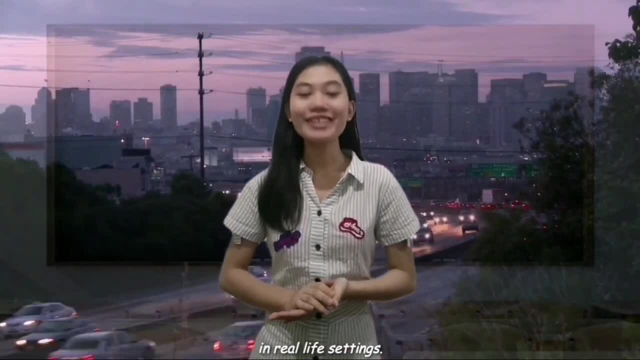 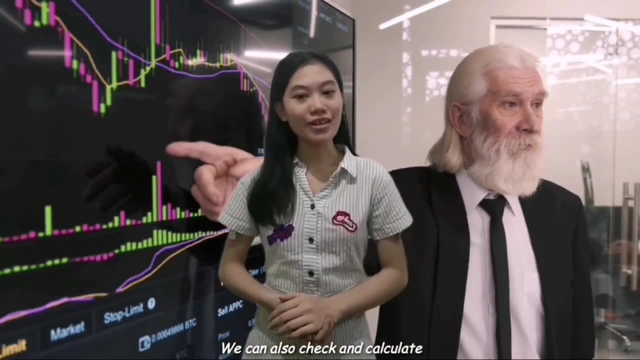 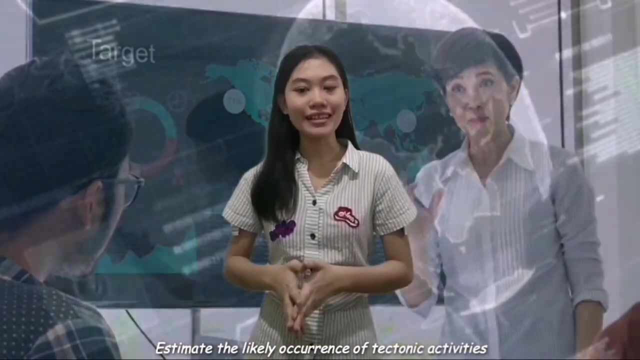 not only applied in mathematics, it also extends everywhere in real life settings. For instance, derivatives are applicable in measuring the rate of increase and drop in the distance. We can also check and calculate temperature variation and which days or months are the hottest and coldest, Estimate the likely occurrence of tectonic activities and 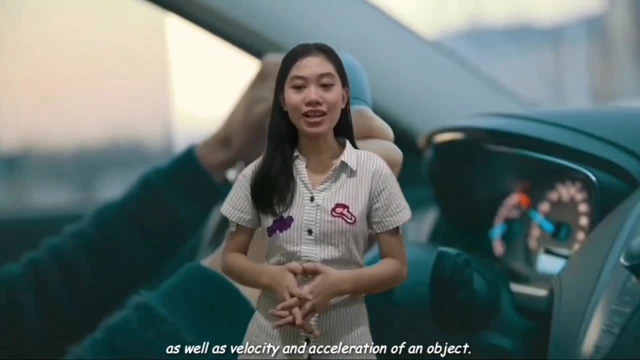 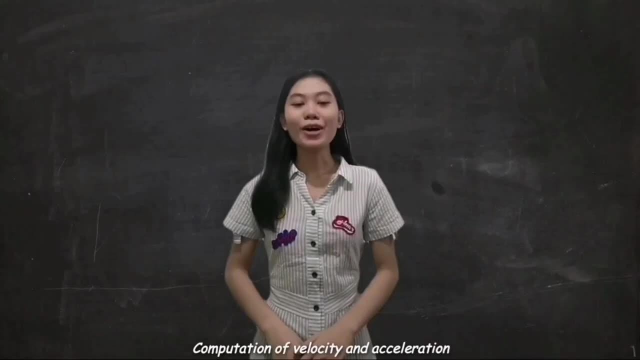 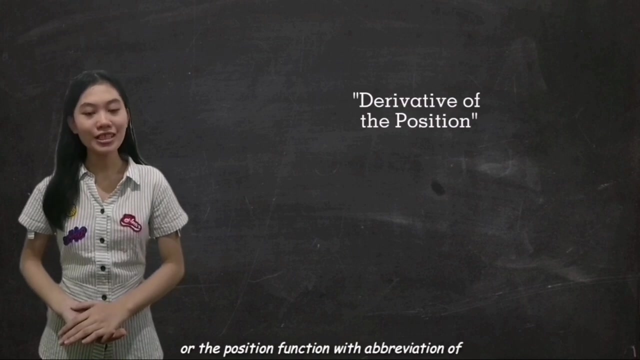 to determine the speed and distance covered, as well as velocity and acceleration of an object. Now let's head out with our examples. Computation of velocity and acceleration of an object is the most applicable plot because the derivative of the position or the position function with abbreviation of s will give you a new function that describes velocity. 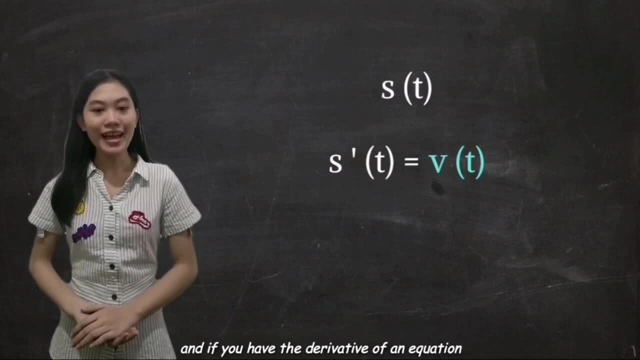 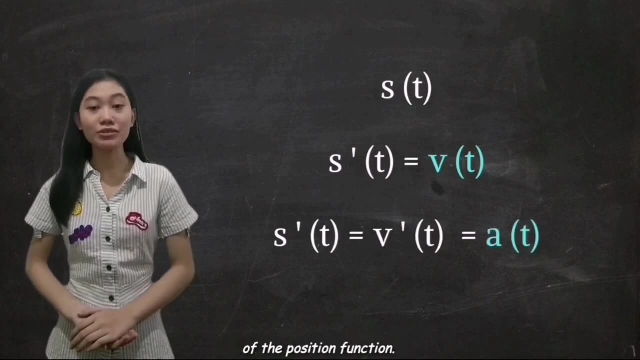 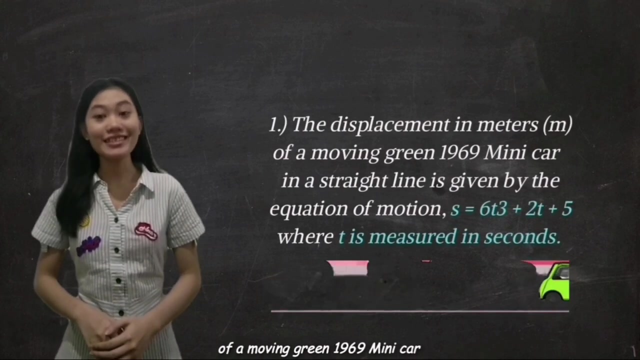 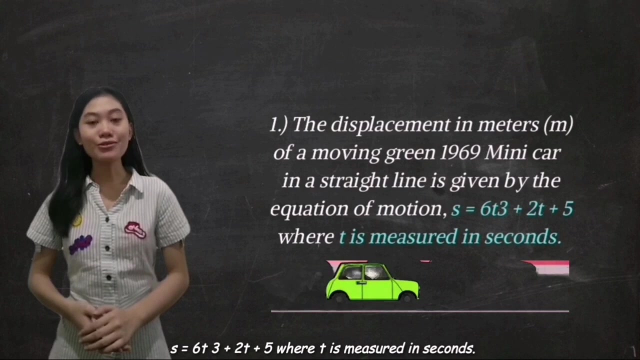 where velocity can be positive or negative in sign and if you have the derivative of an equation that describes the velocity you will get the acceleration. the second derivative of the position function, For example, number 1,, the displacement in meters of a moving green 1969 minicar in a straight line is given by the equation of motion: s is equal to 6t cube plus 2t plus 5, where t is measured in seconds. 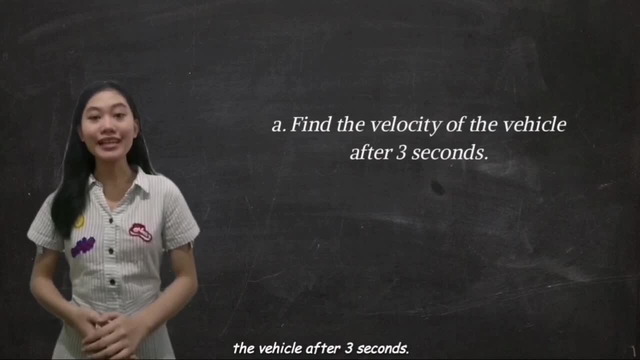 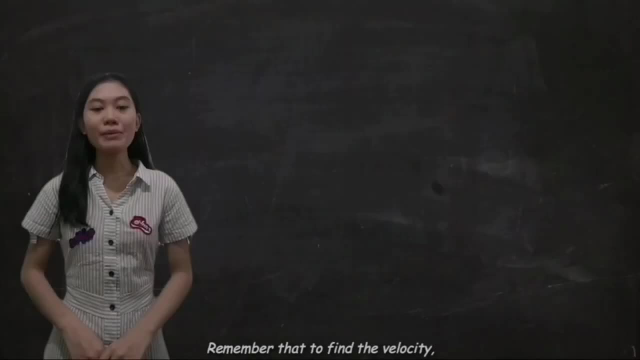 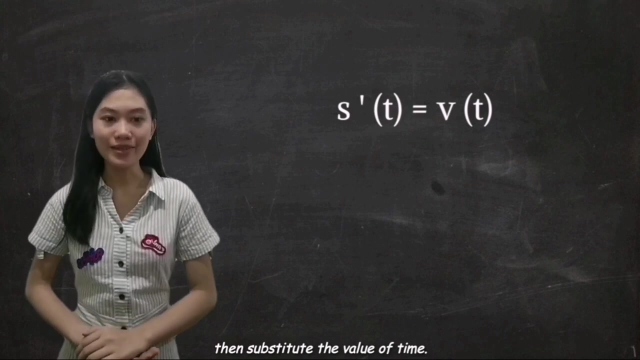 We have to find out: a- find the velocity of the vehicle after 3 seconds, and b- find the acceleration of the vehicle after 3 seconds. Remember that to find the velocity we must find the derivative of s. To find the derivative of the position function, then substitute the value of time. 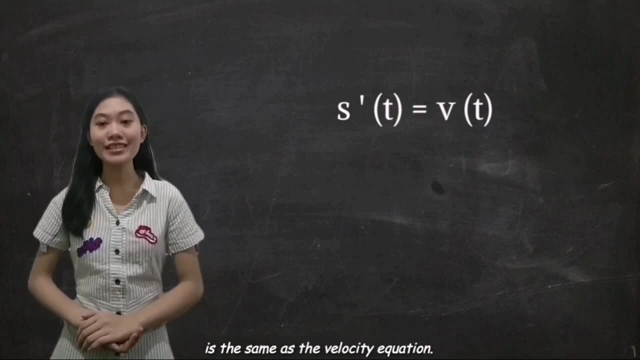 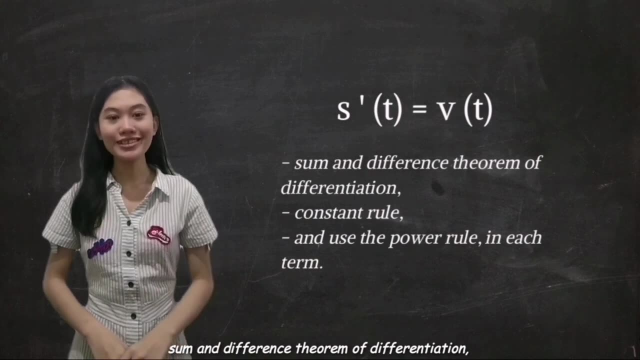 So the derivative of the position function is the same as the velocity equation. We have a polynomial and to do this we will apply the sum and difference theorem of differentiation, constant rule and the use of power rule in H3, where the power of x gets subtracted by 1.. 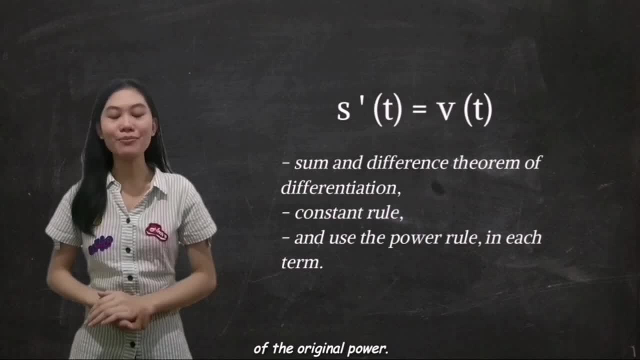 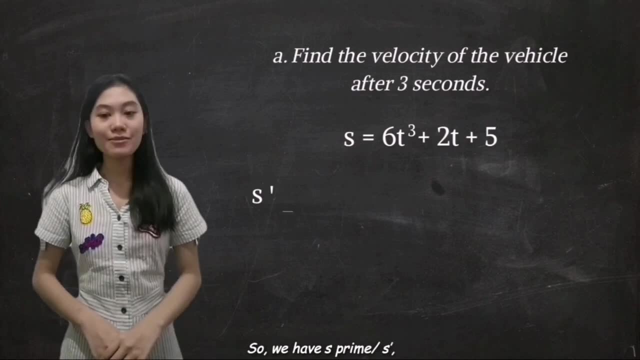 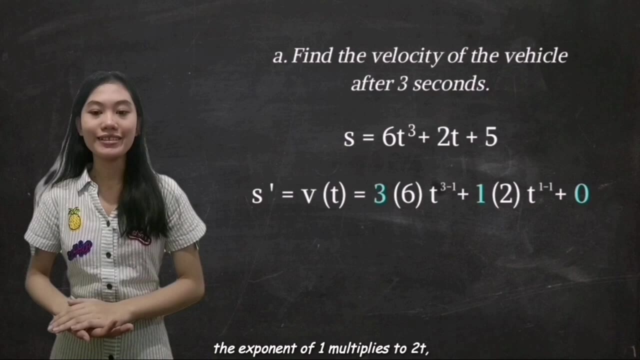 Afterwards, the entire function is multiplied by the value of the original power. a find the velocity of the vehicle after 3 seconds. So we have s prime equals 3 times 6t, raised to 3 minus 1.. For the next term, the exponent of 1 multiplied to 2t, raised to 1 minus 1.. 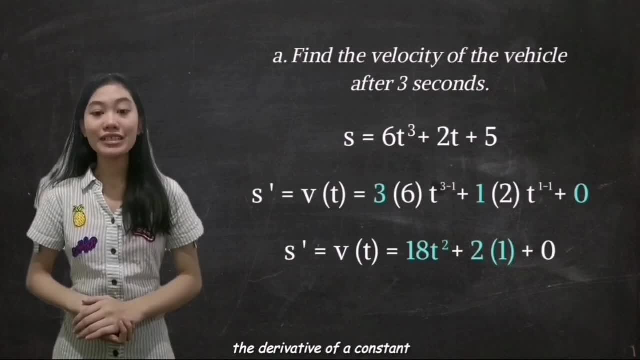 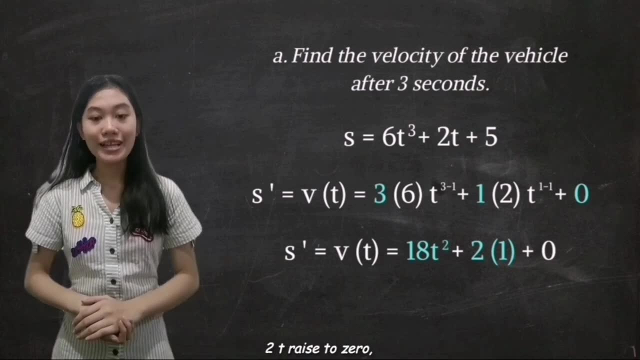 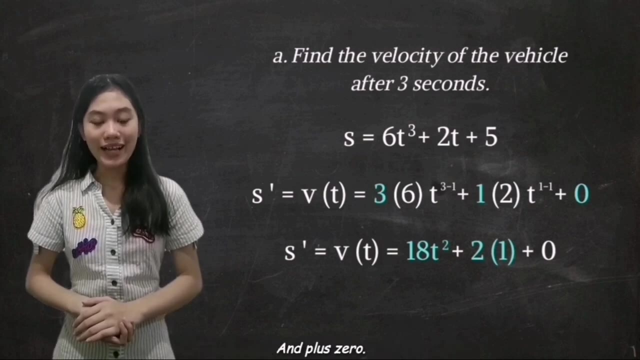 For the last term. since we have a constant, the derivative of a constant is always 0. Then simplify: we have 8t squared plus the second term, 2t, raised to 0. In this part, t raised to 0 is equals to 1. only we have 2 multiplied to 1 and plus 0.. 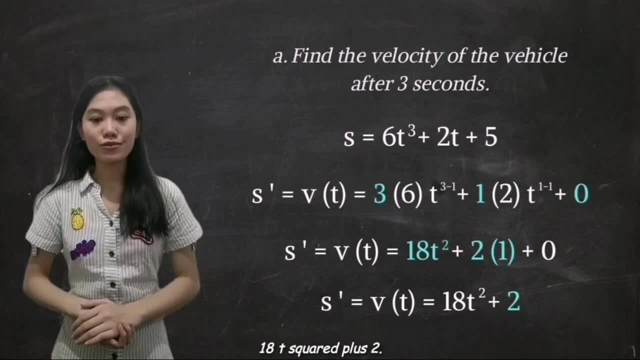 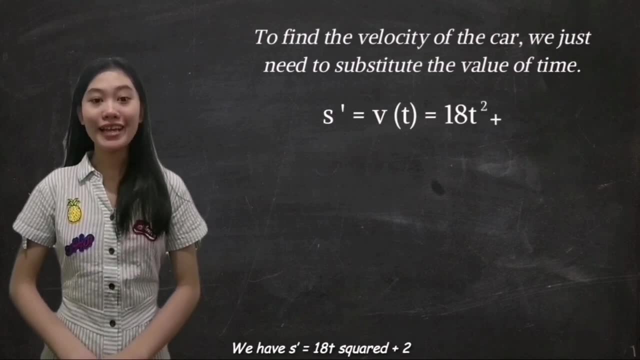 We will have an answer here: 18t squared plus 2.. To find the velocity of the car, we just need to substitute the value of time We have s prime is equals to 18t squared plus 2.. Then it will become 18 times 3 squared plus 2.. 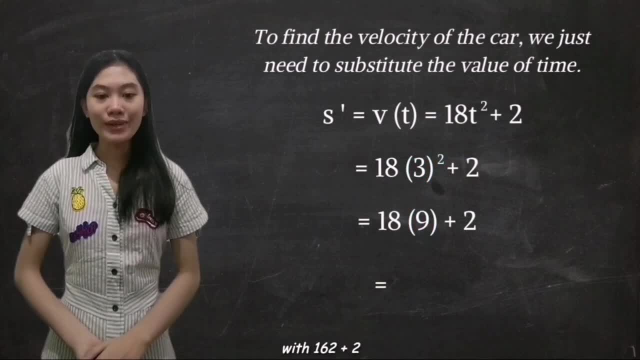 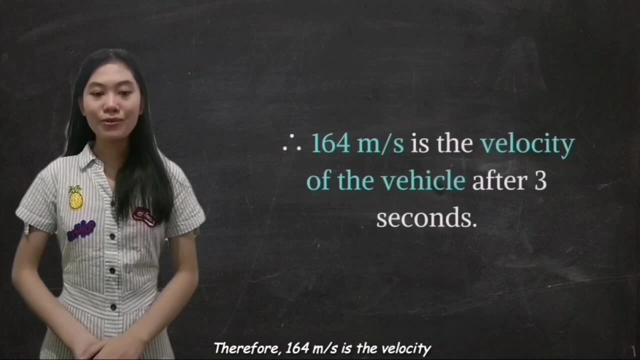 It will come up with 18 times 9 plus 2, with 162 plus 2, with the final answer of 164 meter per second. Therefore, 164 meter per second is the velocity of the vehicle after 3 seconds. Secondly, we need to find the acceleration function. 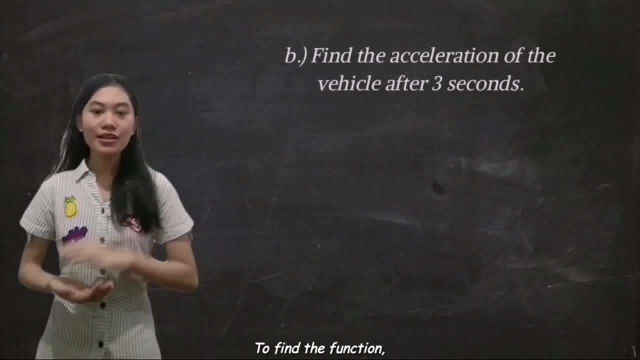 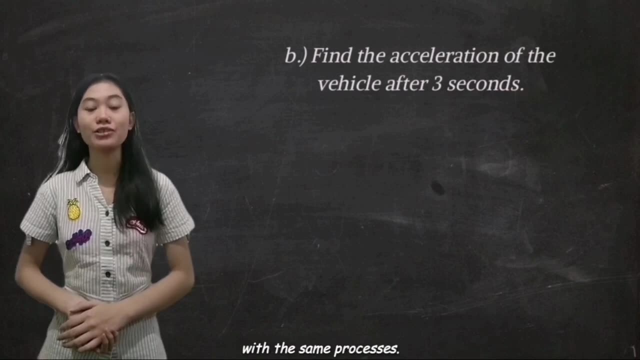 To find the function we need to solve: the derivative of the velocity function or the derivative of the derivative of the position function. with the same process, We have 18t squared plus 2.. Apply power rule, Constant rule and sum and difference rule. 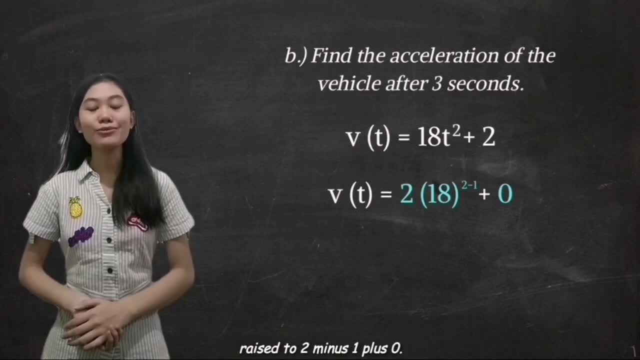 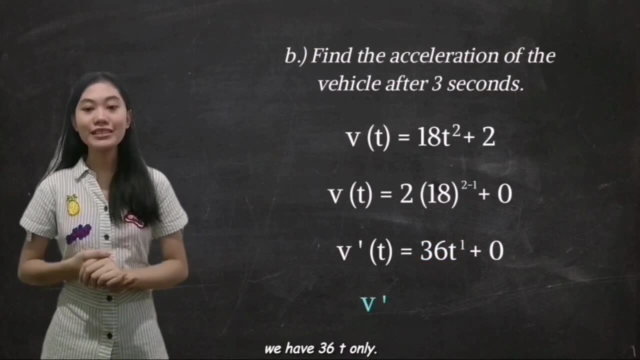 We will come up with 2 times 18t raised to 2 minus 1 plus 0., Then 36t raised to 1 plus 0.. Further simplify, We have 36t. only To find the acceleration of the car, we need to substitute the value of time. 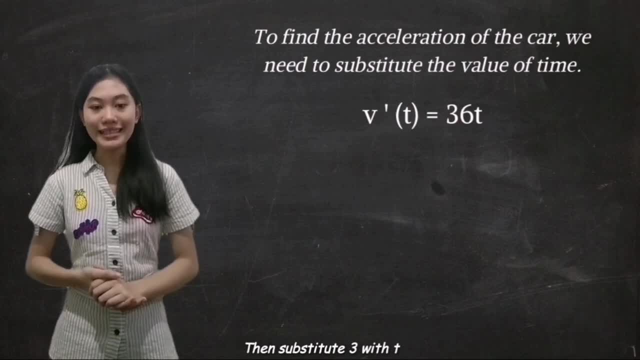 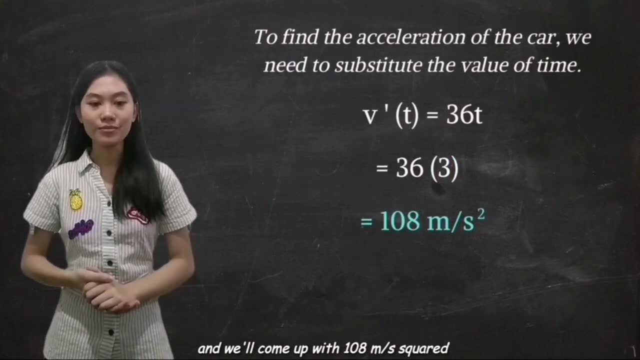 We have 36t. Then substitute 3 with t. We will have 36 times 3 and will come up with 108 meter per second squared. Therefore, 108 meter per second squared is the acceleration of the vehicle after 3 seconds. 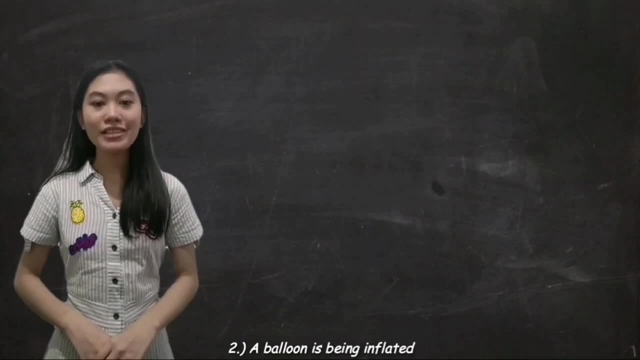 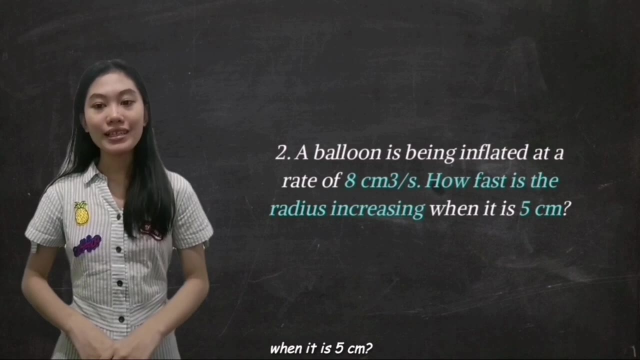 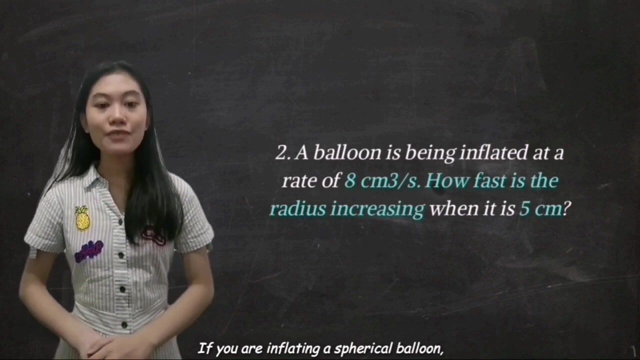 For our next example, number 2.. A balloon is being inflated at a rate of 8 cubic meters. How fast is the radius increasing when it is 5 centimeters? In this case, there is a rate of change. If you are inflating a spherical balloon, the volume expands with respect to radius. 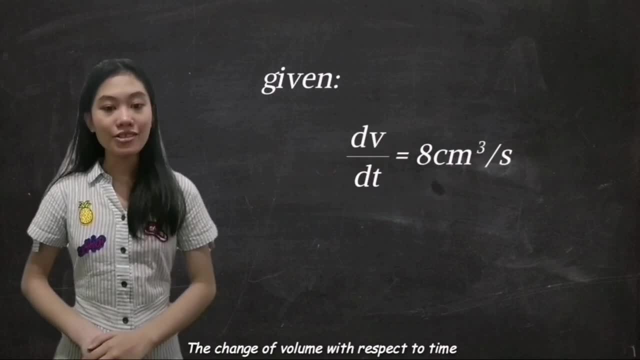 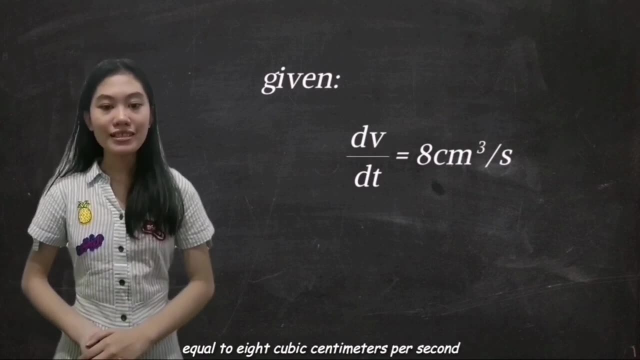 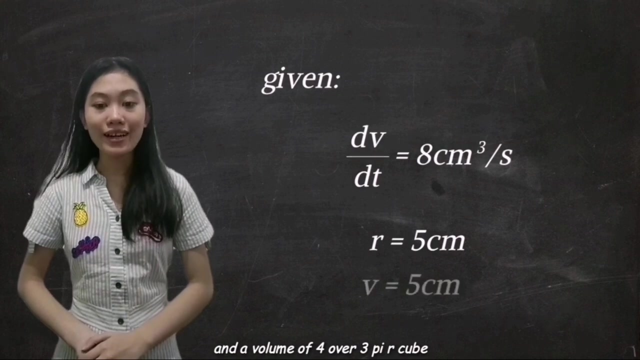 Let's start our computation with the given values of The change of volume with respect to time. is represented as dv over dt, equal to 8 cubic centimeters per second, Our radius of 5 centimeters and the volume of 4 over 3 pi r cubed. 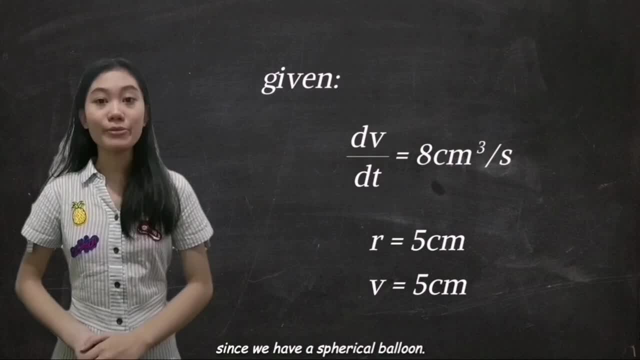 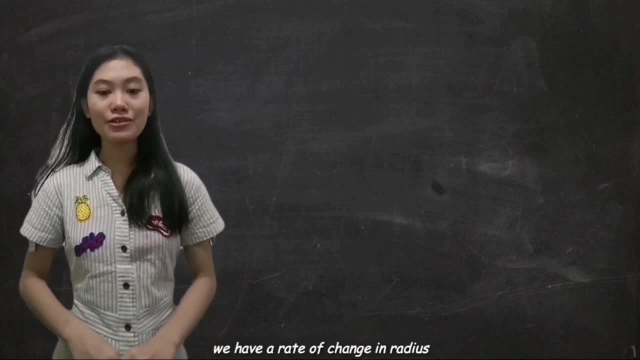 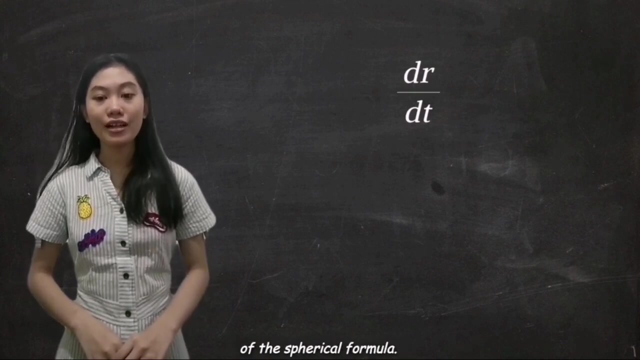 is a constant formula for spheres. since we have a spherical balloon, Since we have to find the rate of change in radius as it increases, we have a rate of change in radius with respect to time: dr over dt. To get the values of dr over dt, we have to get the derivative of the spherical formula. 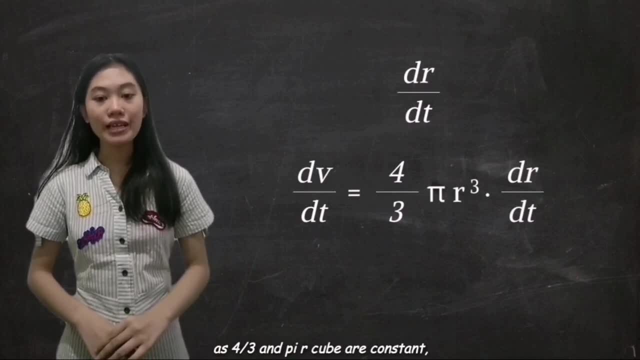 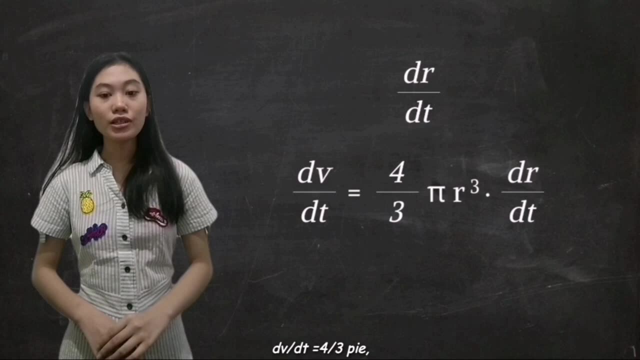 We have dv over dt and 4 over 3 and pi r cubed are constant. We will only get the derivative of radius. Then we will now have dv over dt is equal to 4 over 3. pi Apply power. 3 multiplied to r, then raised to 3 minus 1, equals 2.. 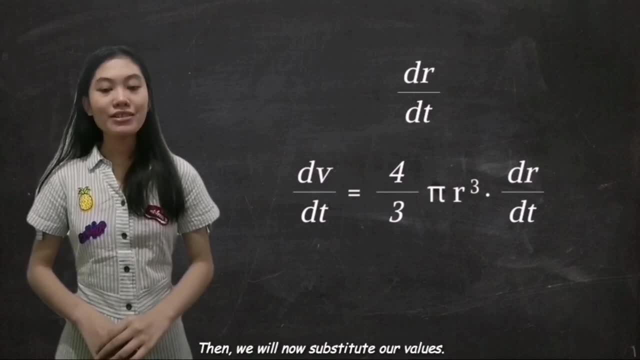 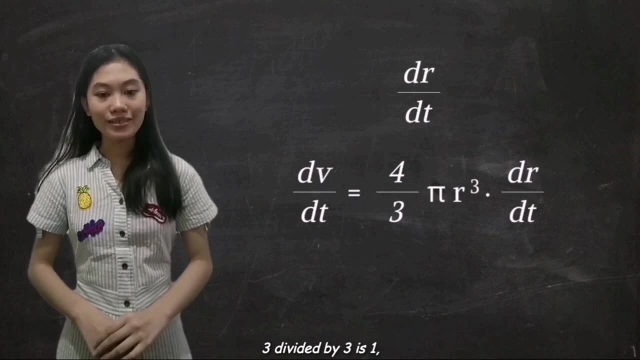 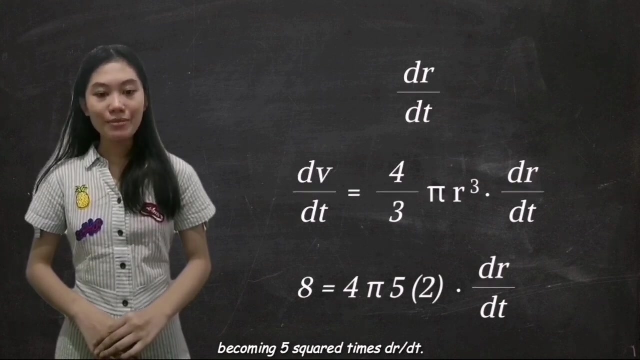 Then multiply it with dr over dt. Then we will now substitute our values: dv over dt is 8.. We can apply division: 3 divided by 3 is 1. We will only have 4 pi only. We have a radius of 5, becoming 5 squared times dr over dt. 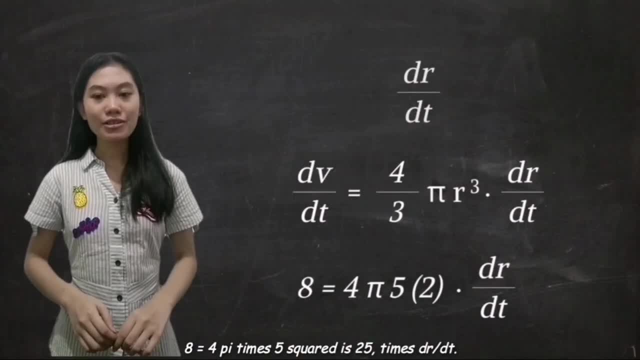 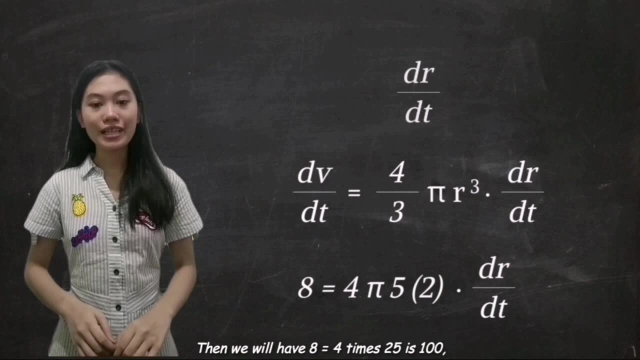 Further perform the operation. 8 is equal to 4 pi times 5. squared is 25 times dr over dt. Then we have: 8 is equal to 4 times 25 is 100.. We have 100 pi times dr over dt. 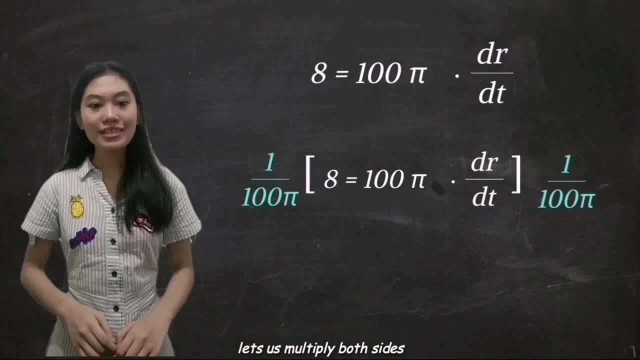 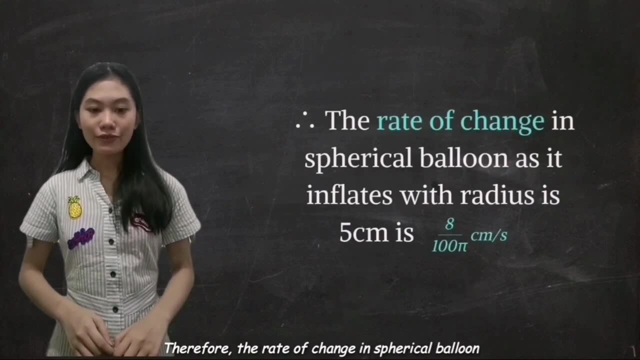 We remove 100 pi and get the value of dr over dt. Then let's multiply both sides with 1 over 100 pi. It will now become 8 over 100 pi. Therefore the rate of change in spherical balloon as it inflates with radius of 5 centimeters. 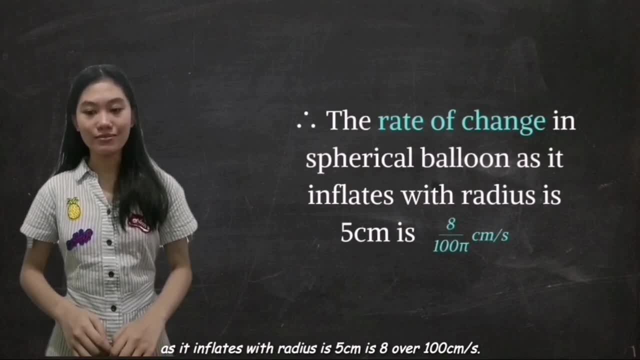 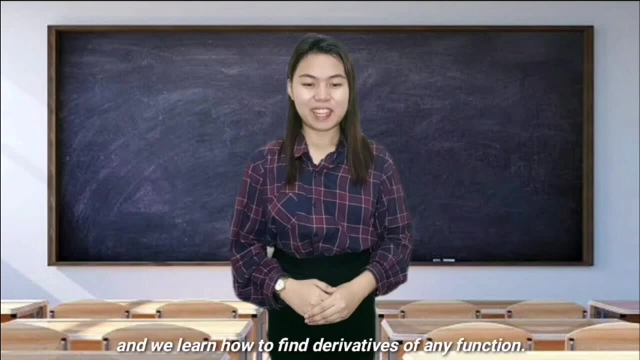 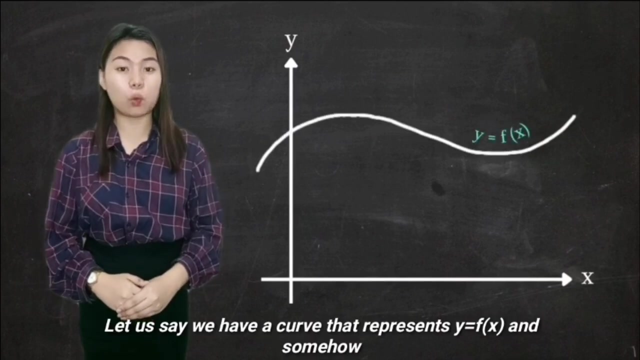 is 8 over 100 pi centimeters per square. From our previous video we already know what is derivatives And we learned how to find derivatives of any function. And now I'll discuss about integral calculus. Let's say we have a curve that represents y is equal to f of x. 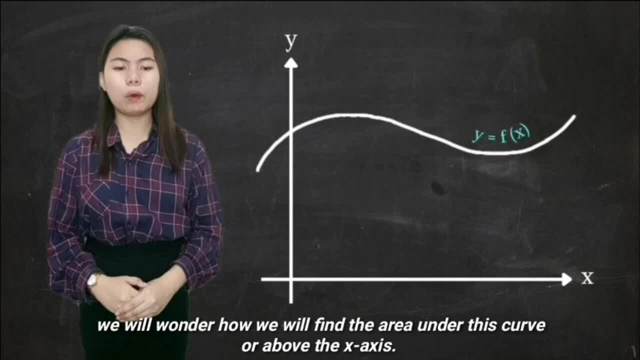 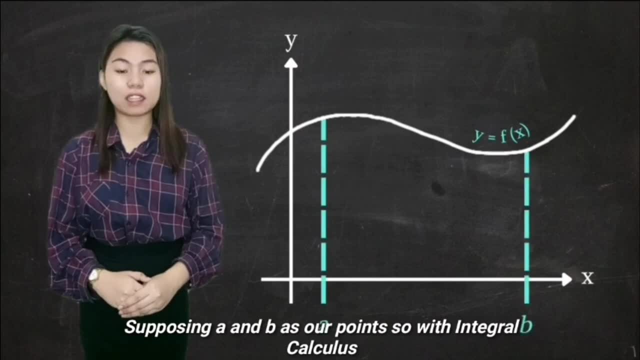 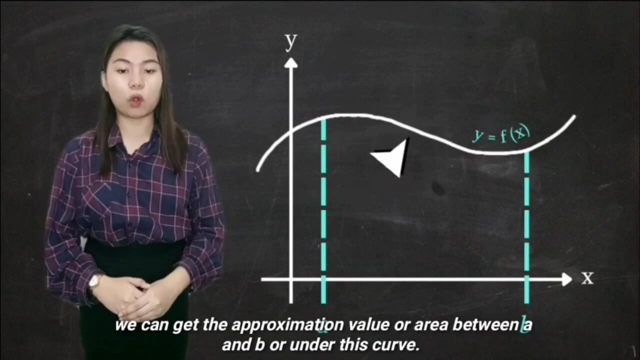 And somehow we will wonder how we will find the area under this curve or above the x-axis, Supposing a and b as our points. So with integral calculus we can get the approximation value or area between a and b or under this curve. 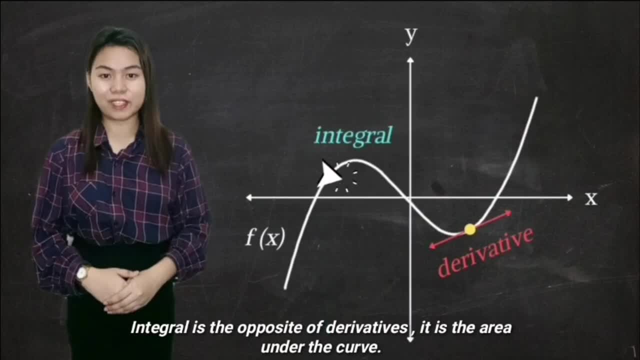 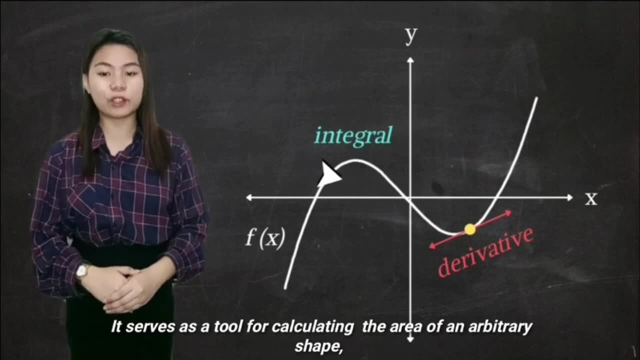 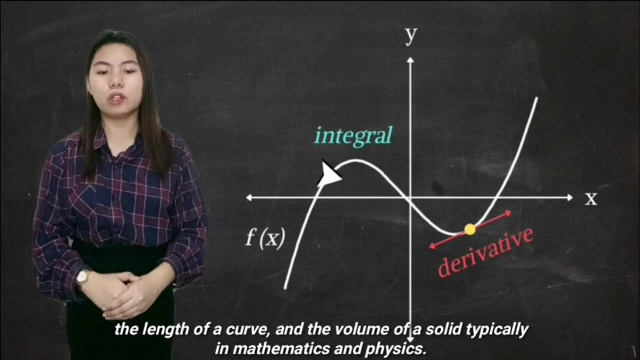 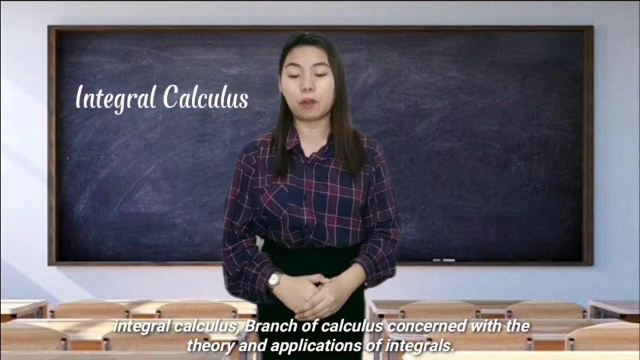 Integral is the opposite of derivatives. It is the area under the curve. It serves as a tool for calculating the area of an arbitrary shape, the length of a curve and the volume of a solid. typically, in mathematics and physics, Integral calculus is a branch of calculus. 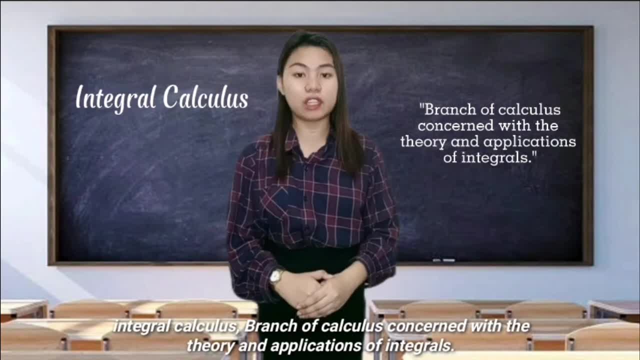 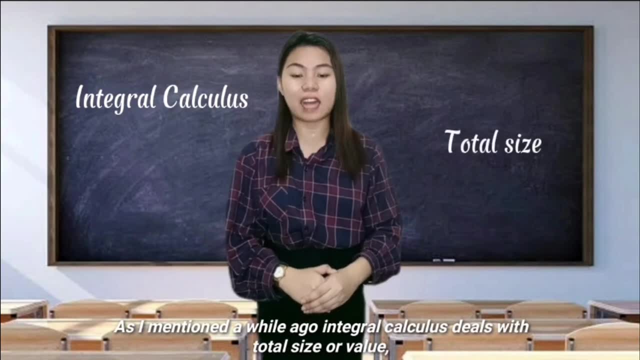 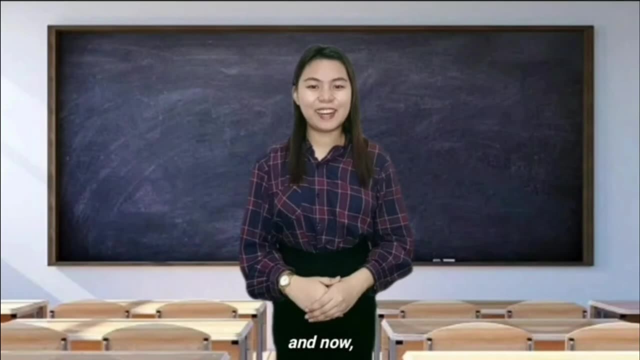 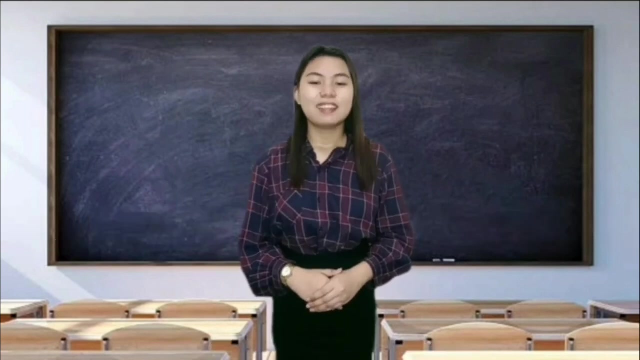 concerned with the theory and applications of integrals. As I mentioned a while ago, integral calculus deals with the total size or value, such as length, area and volumes. And now let's proceed with the difference of differentiation and anti-differentiation. 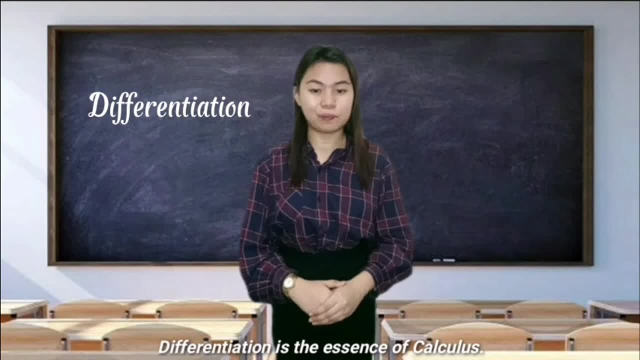 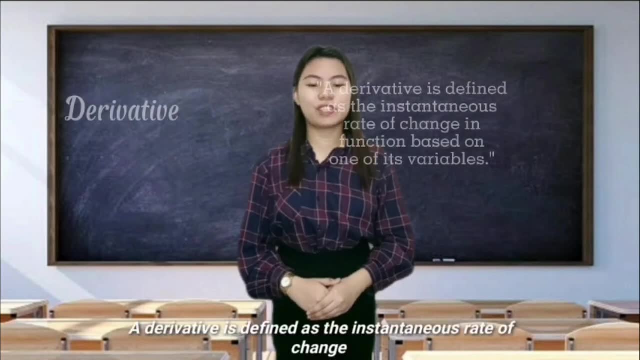 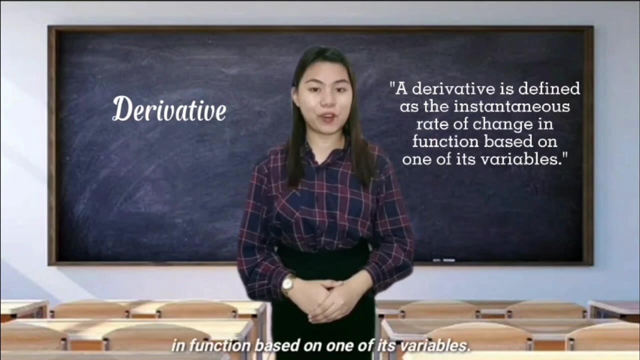 Differentiation is the essence of calculus. Differentiation is a method of finding the derivative of a function. A derivative is defined as the instantaneous rate of change in a function based on one of its variable. It is similar to finding the slope of a tangent to the function at a point. 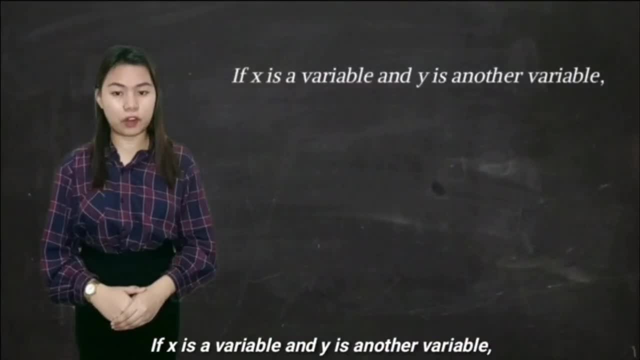 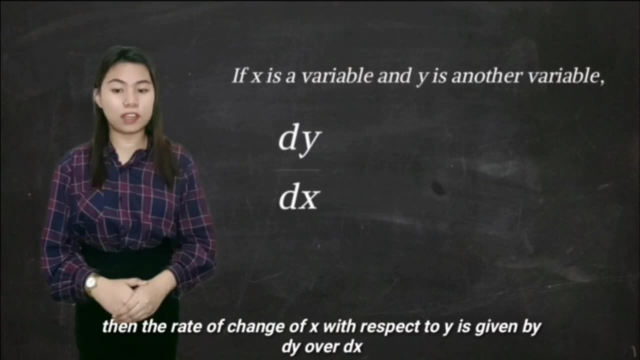 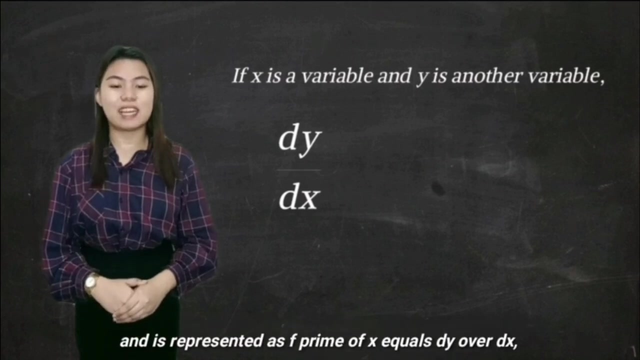 If x is a variable and y is another variable, then the rate of change of x with respect to y is given by dy over dx. This is the general expression of the derivative of a function and it is represented as f' Where y is equal to f is any function. 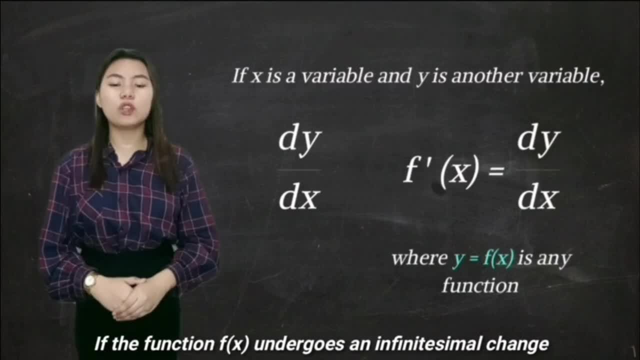 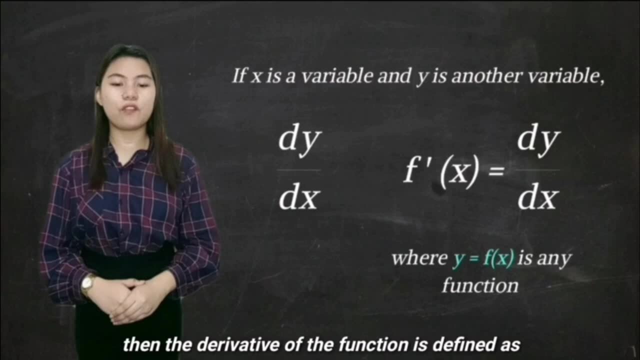 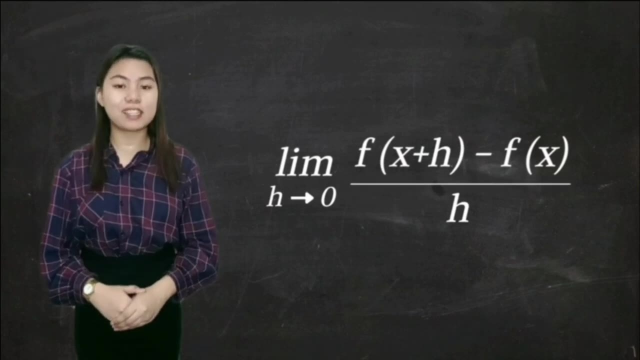 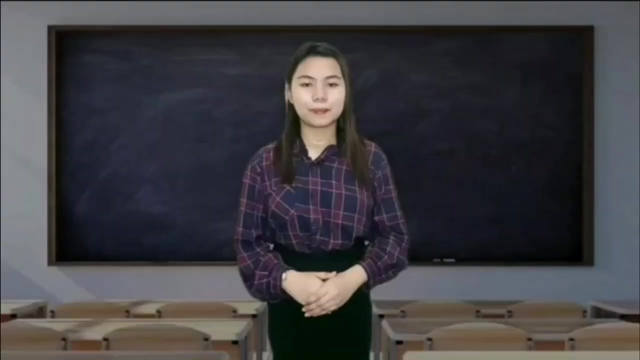 if the function f undergoes an infinite similar change of delta x near to any point x, then the derivative of the function is defined as the limit of f plus delta x minus f, all over delta x. as delta x approaches to zero, The anti-derivative, also referred to as an integral, 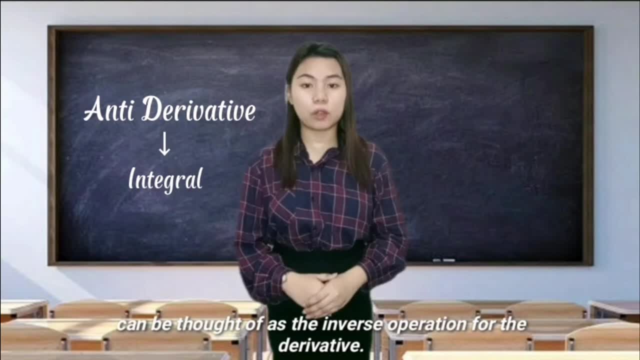 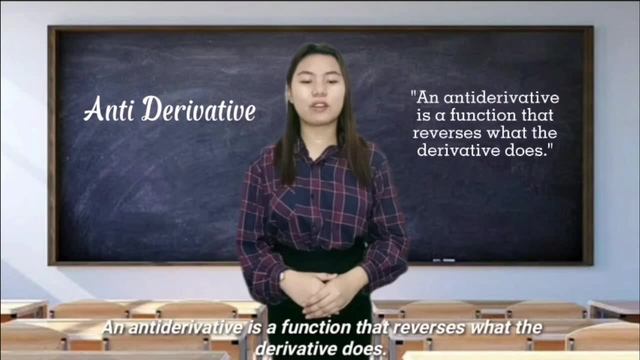 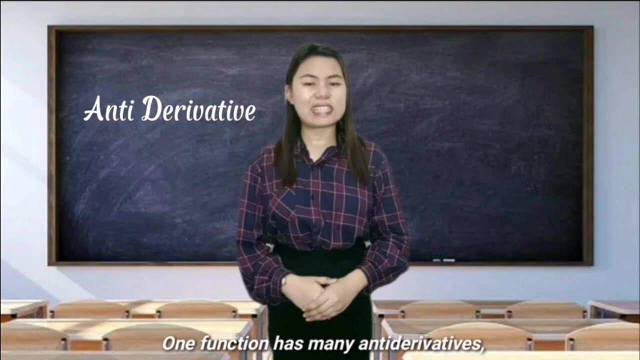 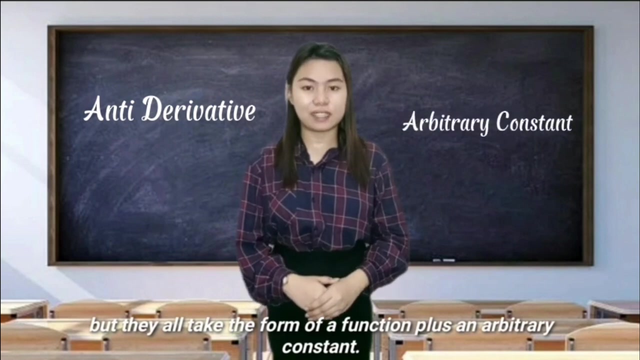 can be thought of as the inverse operation for the derivative. In other words, it is the opposite of a derivative. An anti-derivative is a function that reverses what the derivative does. One function has many anti-derivatives, but they all take the form of a function plus an arbitrary constant. 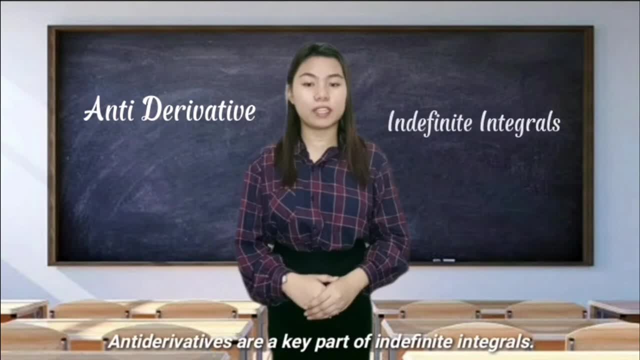 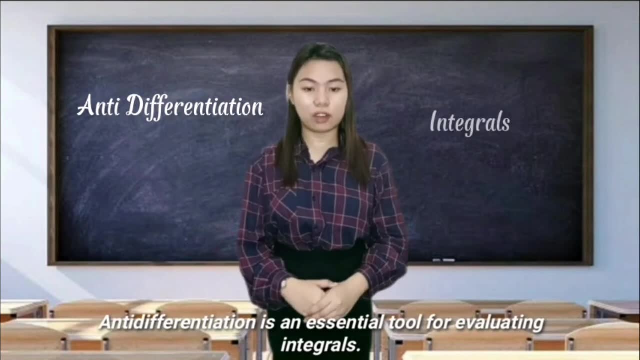 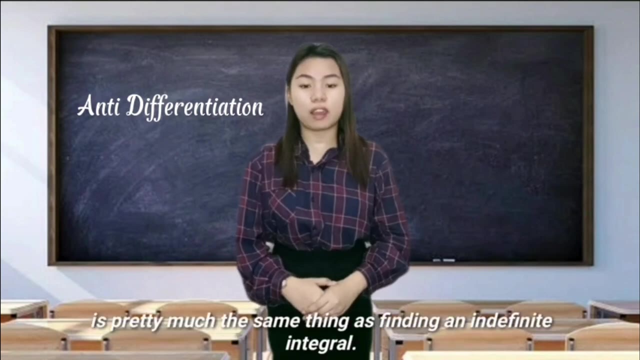 Anti-derivatives are a key part of indefinite integrals. Anti-differentiation is an essential tool for evaluating integrals. In fact, you might say that anti-differentiation is pretty much the same thing as finding an indefinite integral When we anti-differentiate a function. 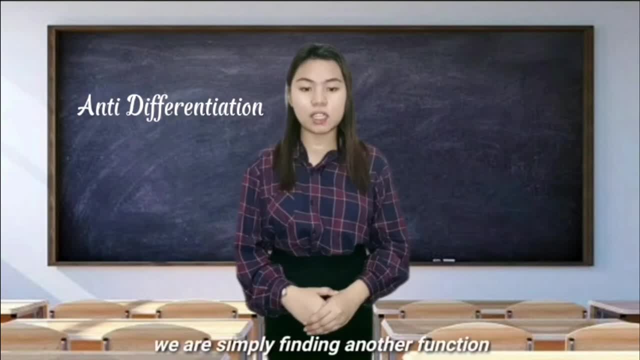 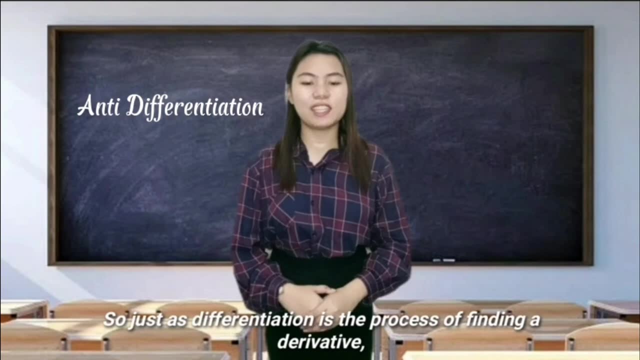 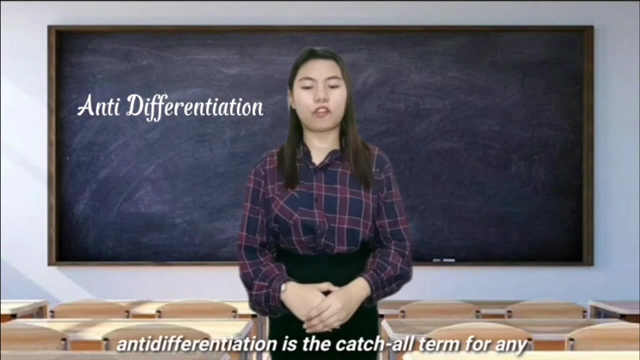 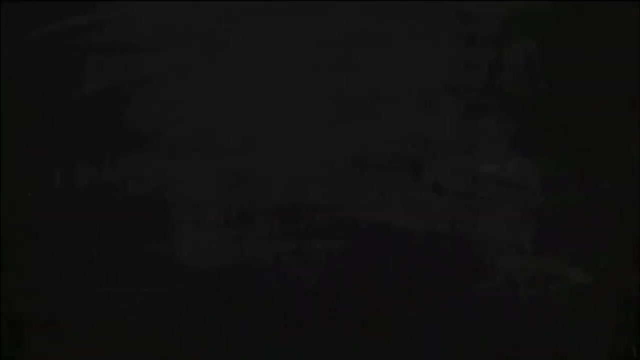 we are simply finding another function whose derivative is equal to the one we started with. So, just as differentiation is the process of finding a derivative, anti-differentiation is the catch-all term for any formula, technique or method of finding an anti-derivative. 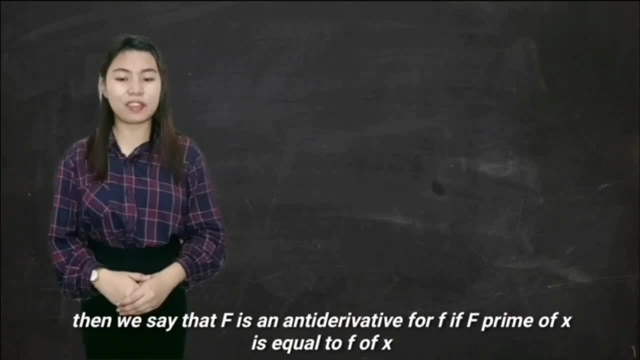 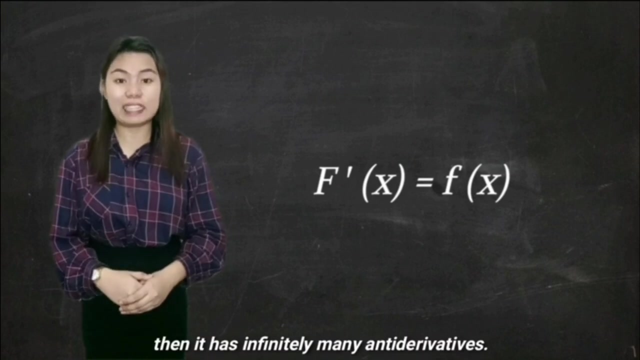 If f is a function, then we can say that f is an anti-derivative for f. if f' is equal to f, If a function has one anti-derivative, then it has infinitely many anti-derivatives. This is because the derivative of any constant is 0.. 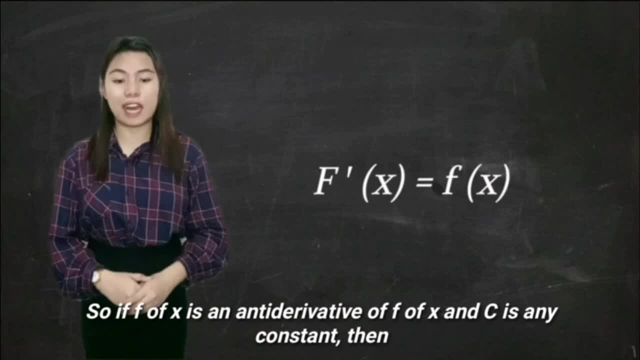 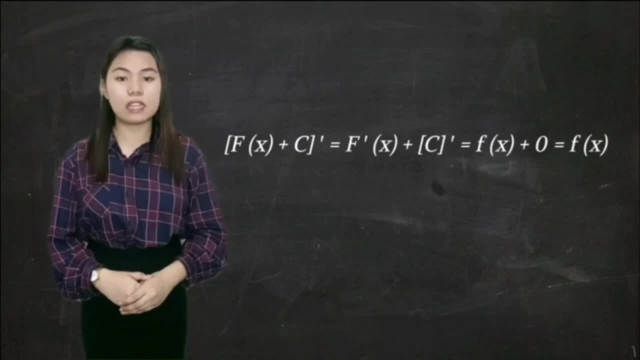 So if f is anti-derivative of f and c is any constant, then f plus the constant of integration is equal to f' plus constant integration is equal to f plus 0 is equal to f. Therefore, f plus c is also an anti-derivative for f. 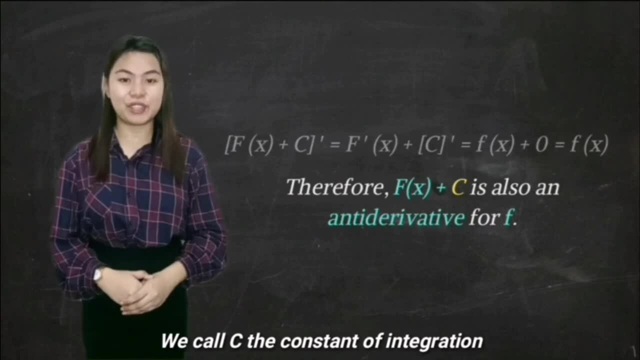 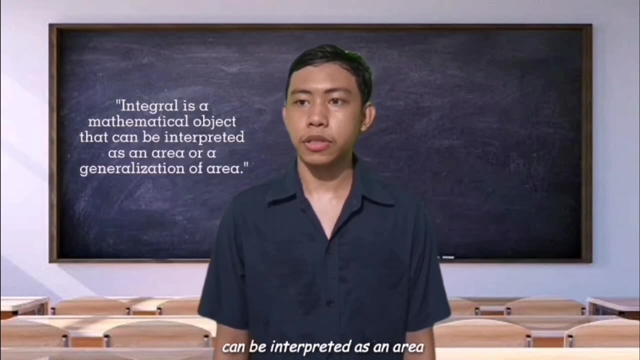 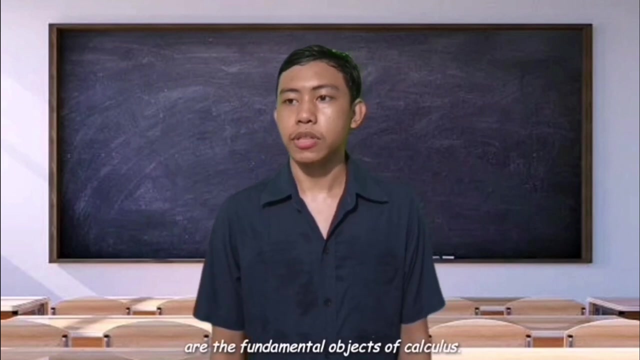 We call c the constant of integration Integrals. In calculus, an integral is a mathematical object that can be interpreted as an area of a generalization of area. Integrals, together with derivatives, are the fundamental objects of calculus. Other words for integral include anti-derivative and derivative. 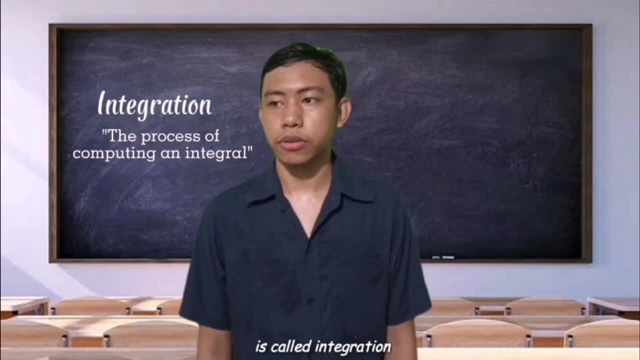 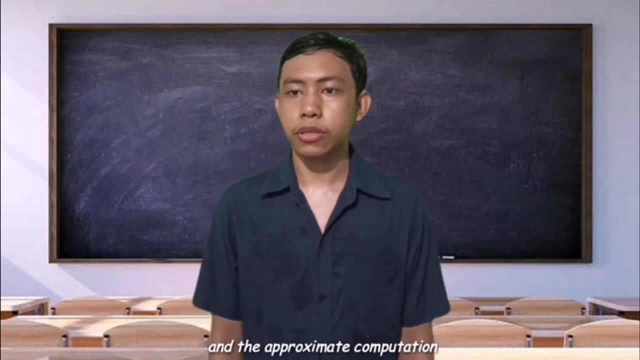 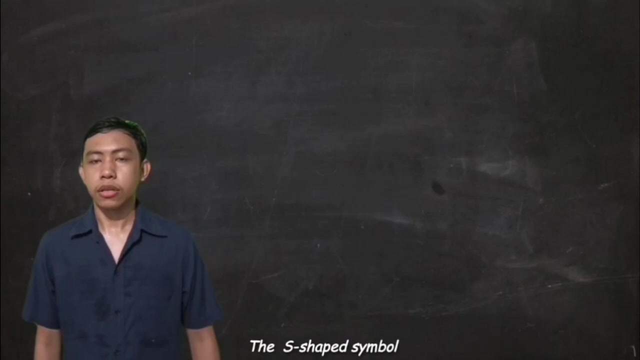 The process of computing an integral is called integration. A more archaic term for integration is quadratic. The appropriate computation of an integral is termed numerical integration. Integral notation: An s-shaped symbol is called an integral sign. The function f of x is a function. 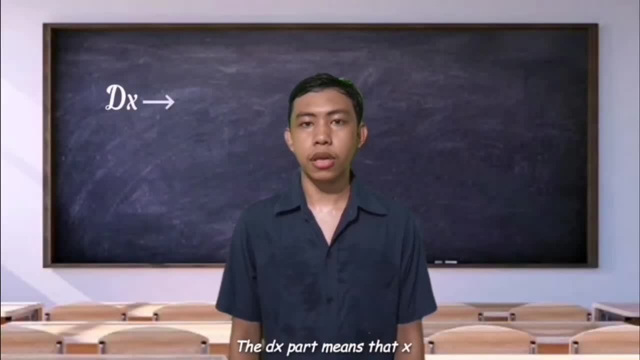 that determines a change in the number of point of contact and is used to tell the increase in mimicry between two points of changing and spiteALIZE. The following point is a value of dimension of the interval. We have two variables to count. that determines theאש. 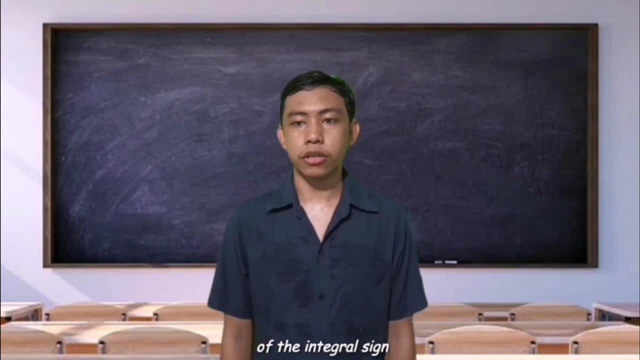 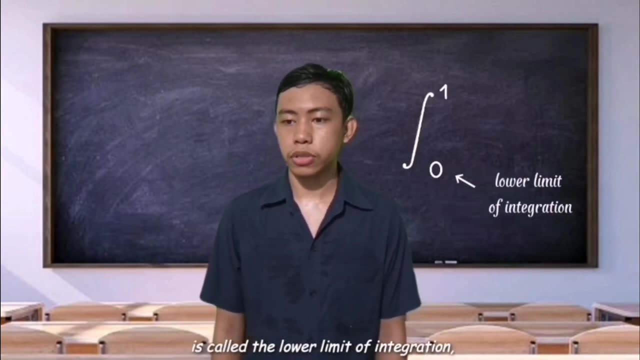 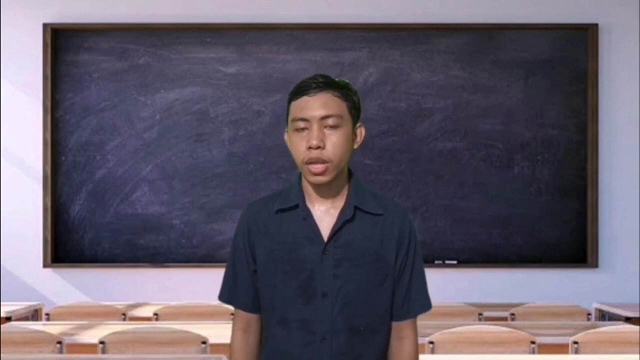 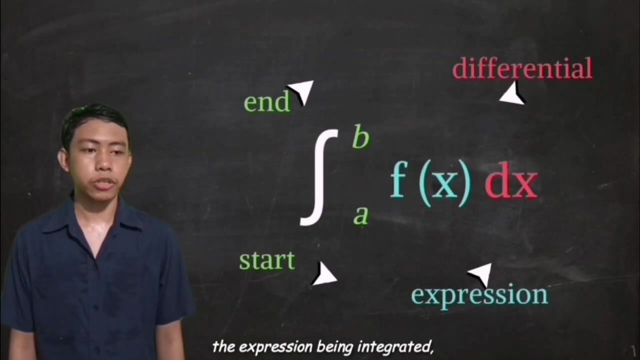 u. we are taking into account. We just need to find out what we are yielding for. 0 as 0.. f is represented by the integral symbol and has four parts: The expression being integrated, the differential, a start value and an end value, Typically the operator. 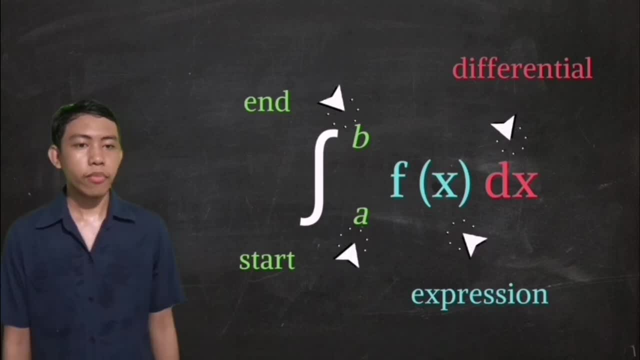 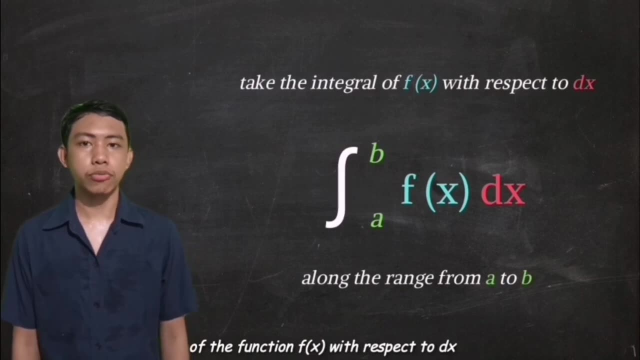 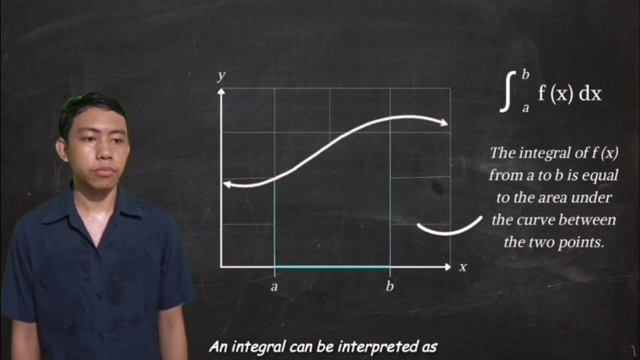 appears in an expression like this. In plain language, this means that take the integral of the function f with respect to dx along range from a to b. Importantly, the differential dx expresses which variable is being integrated. An integral can be interpreted as the area under the curve of a function. 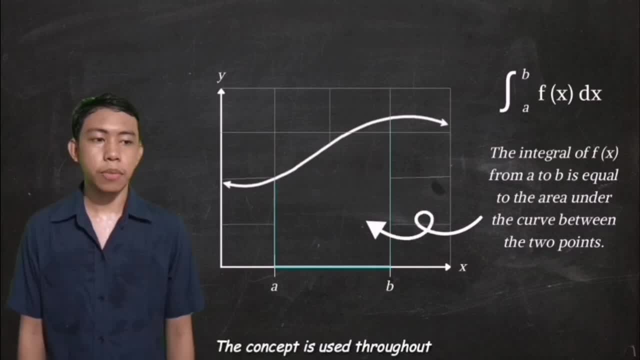 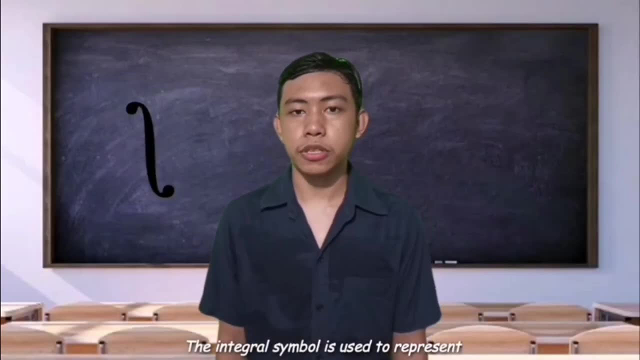 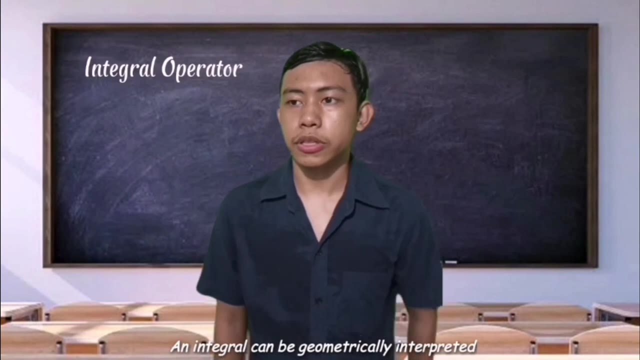 between the points a and b. The concept is used throughout physics and higher level mathematics. The integral sign is used to represent the integral operator in calculus. The integral operator is an integral that can be geometrically interpreted as the area under the curve of a function between the points a and b. 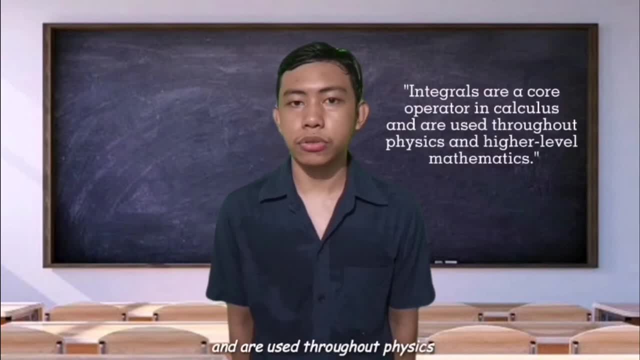 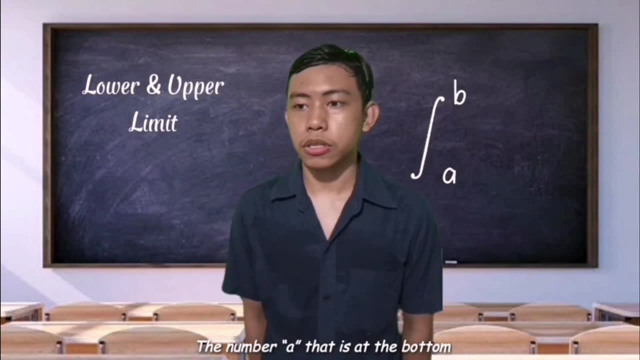 Integrals are a core operator in calculus and are used throughout physics and higher level mathematics. The lower and upper limit, The number a that is at the bottom of the integral sign, is called the lower limit of the integral, with the number b at the top of the integral sign, is called the upper limit of the integral. 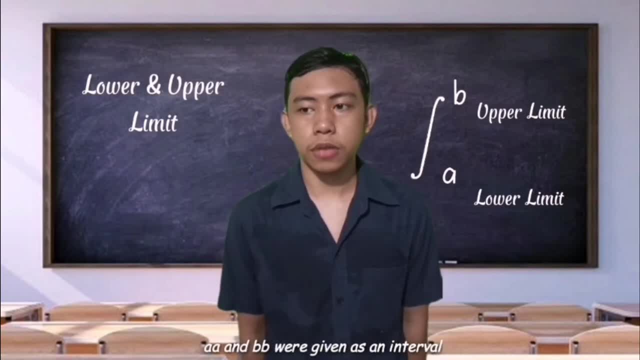 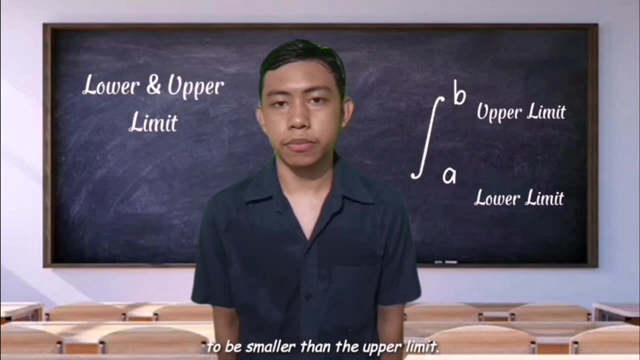 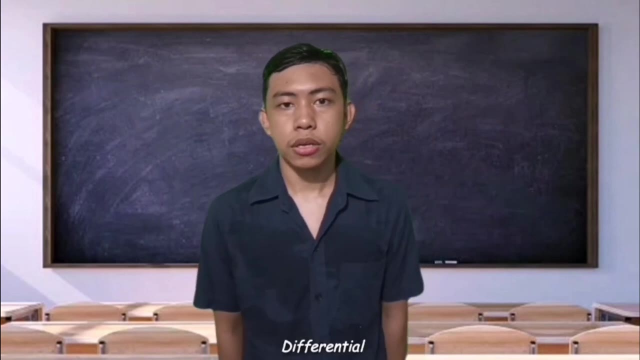 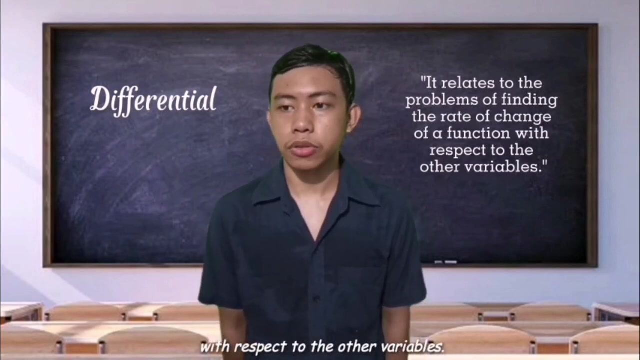 Also, despite the fact that a and b were given As an interval, the lower limit does not necessarily need to be smaller than the upper limit. Relatively, we'll often call A and B as the interval of integration Differential. It relates to the problems of finding the rate of change of a function with respect to the other variables. 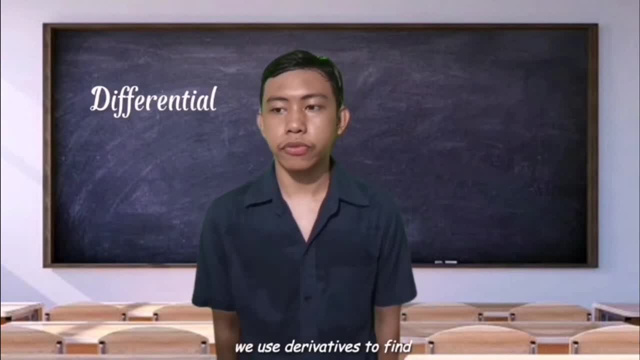 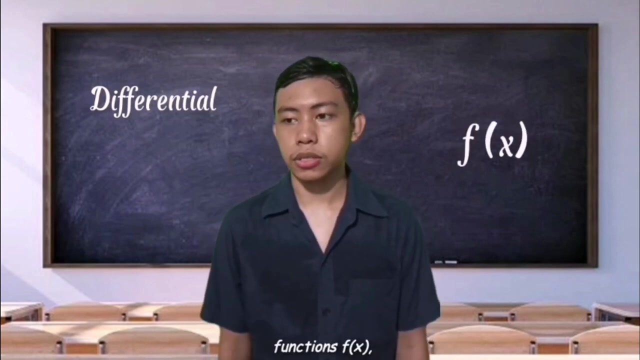 Moreover, to get the ideal solution, we use derivatives to find the maxima and minima values of a function. In addition, it arises from the study of the limit of a quotient. Furthermore, it deals with the variables, such as x and y, functions f of x and the consequent changes in the variables x and y. 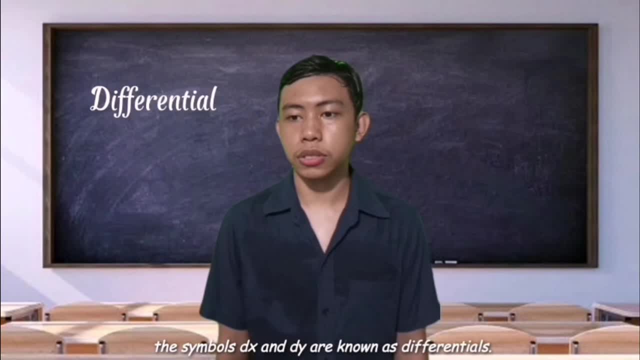 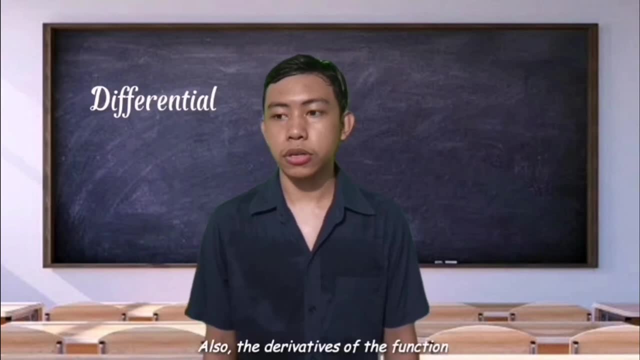 Besides, the symbols dx and dy are known as differentials. Moreover, the process of finding derivatives is what we call differentiation. Also, the derivatives of the function are represented by dy over y. This means that the function is the derivative of y with respect to the variable x. 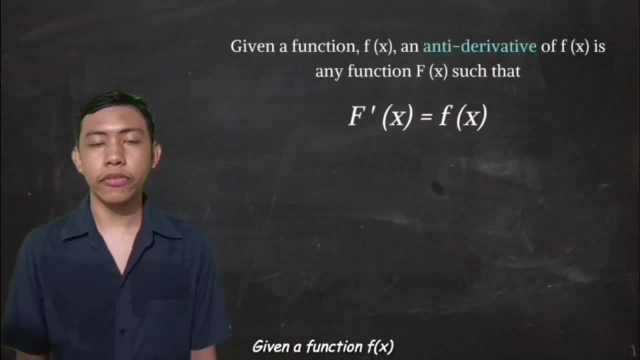 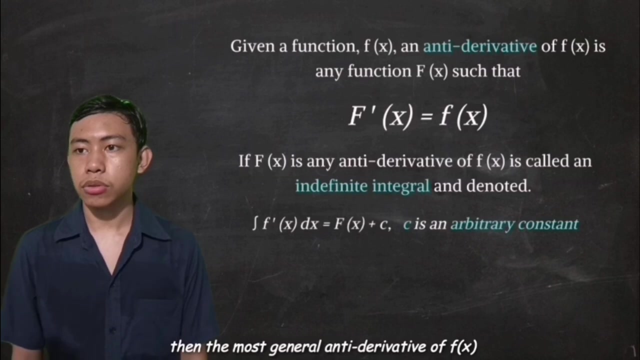 The letter C constant Given a function f of x. an antiderivative of f of x is any function f of x, such that f prime of x is equal to f of x. If f of x is any antiderivative of f of x, then the most general antiderivative of f of x is called an indefinite integral. 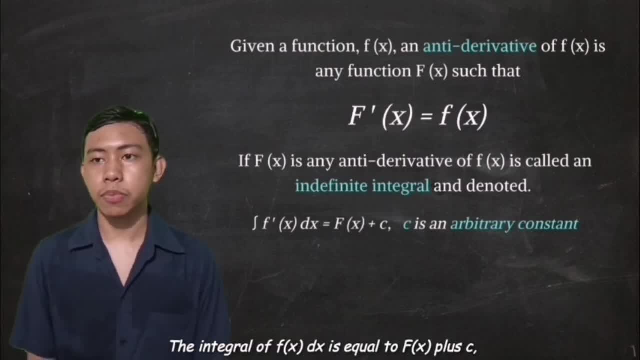 And they know that the integral of f of x with respect to dx is equal to f of x plus c, where c is any arbitrary constant. In this definition, the s-shaped symbol is called the integral symbol, f of x is called the integranon. 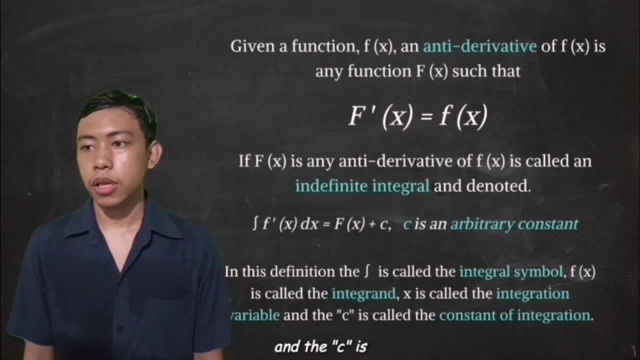 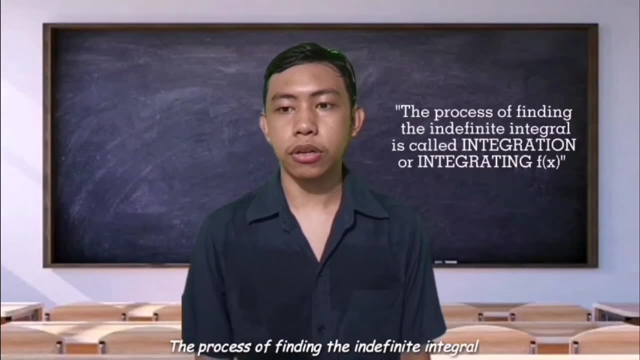 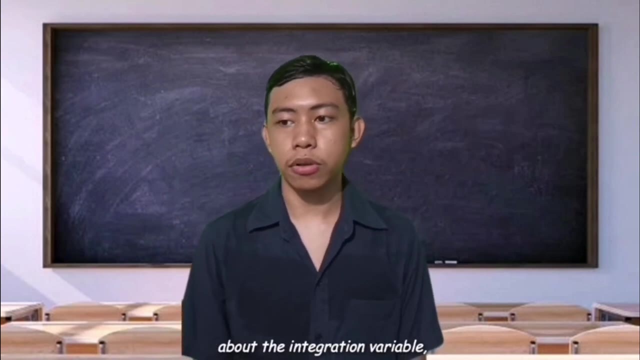 x is called the integration variable and the c is called the constant of integration. The process of finding the indefinite integral is called integration or integration of eingres crumplard f of x. If we need to be specific about the integration variable, we will say that we. 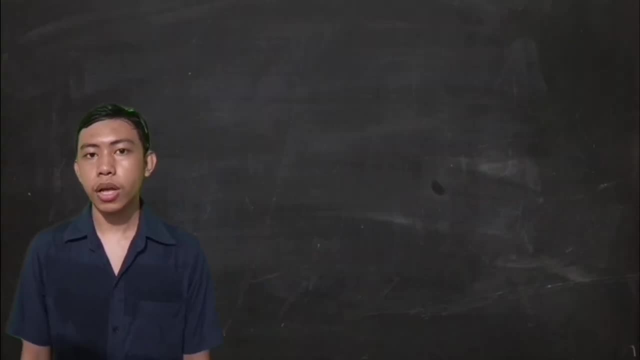 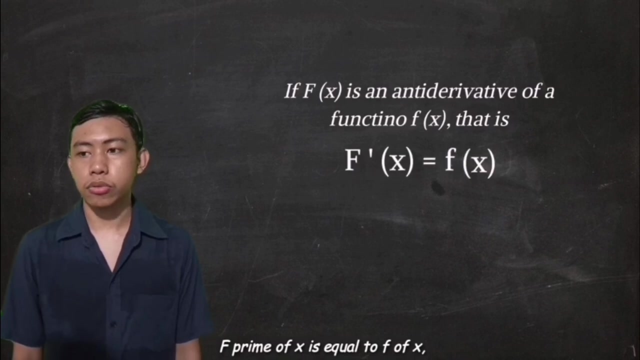 are integrating f of x with respect to x. If f of x is an antiderivative of a function, f of x, that is, f prime of x, is equal to f of x, then g of x is equal to f of x plus. 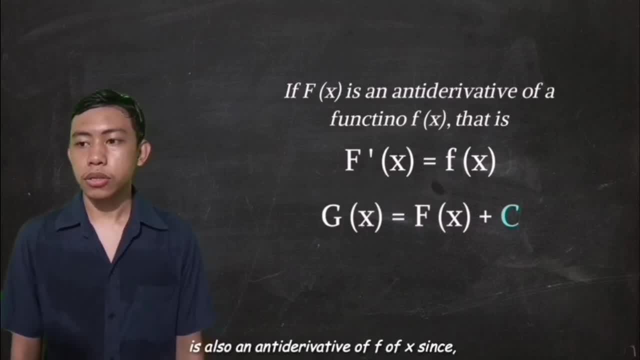 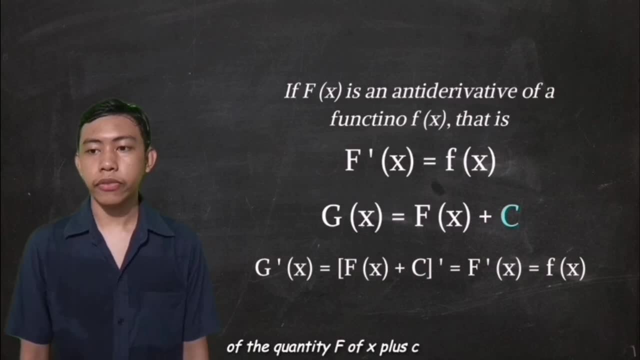 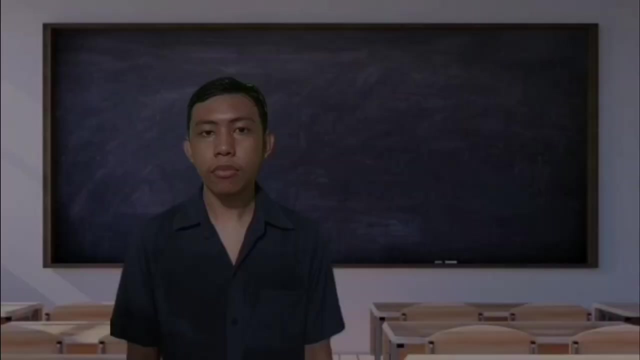 c. where c is any constant, It's also an antiderivative of f of x, since g prime of x is equal to the prime of f of x plus c equals to f of x and equals to f prime of x. Hence there are a. 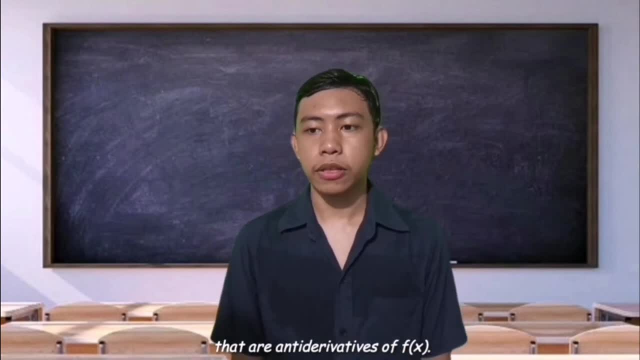 family of functions only differ by a constant that are antiderivatives of f of x. In order to include all antiderivatives of x, the constant f of x is equal to f of x. The constant of integration c is used for indefinite integrals. 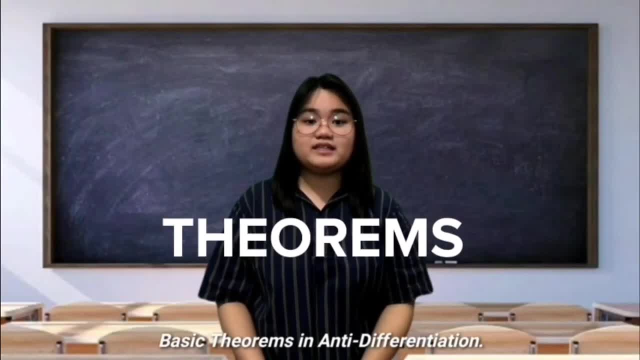 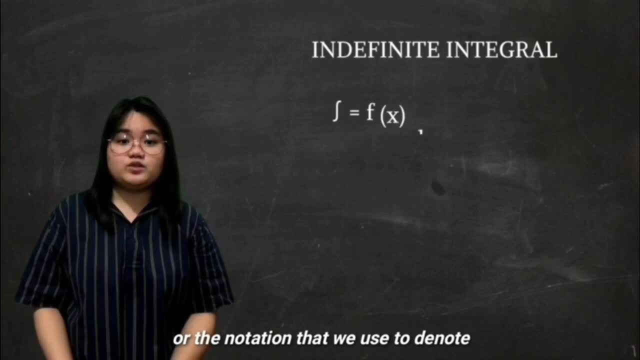 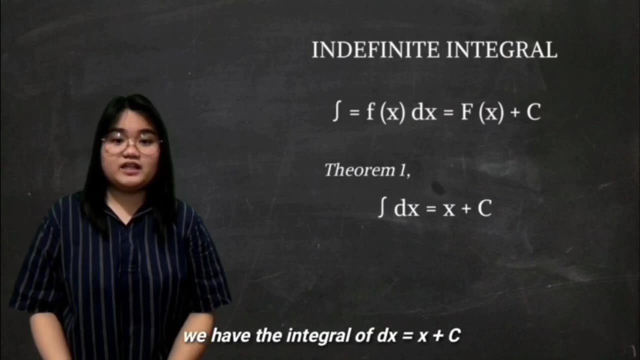 For this portion we will be talking about the basic theorems in antideferential. Over here we have the indefinite integral, or the notation that we use to denote the antiderivatives of a function. Let's begin with the theorems. For theorem 1, we have the integral of dx. 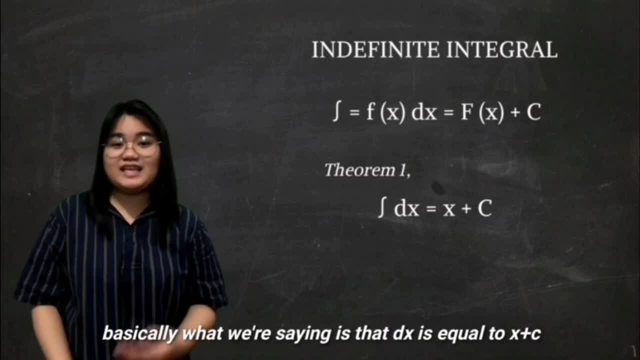 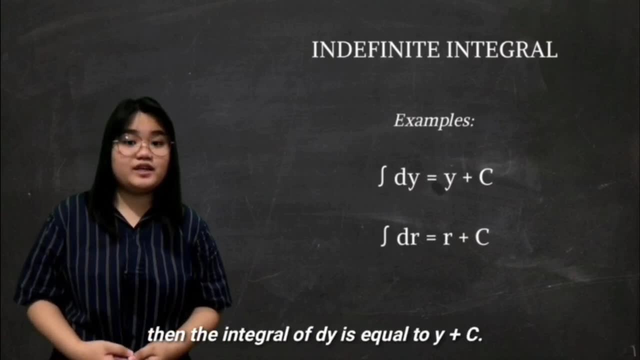 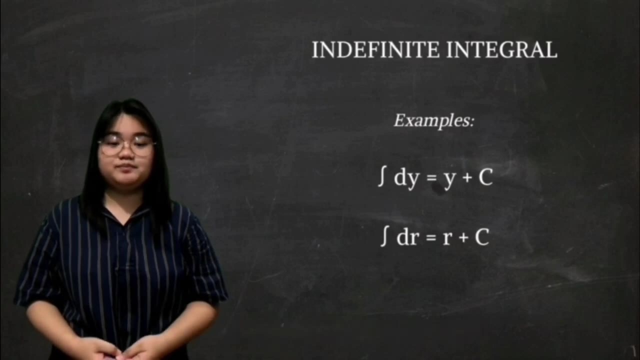 equals x plus c. Basically, what we're saying is that dx is equal to x plus c. For example, if our variable of integration is y, then the integral of dy is equal to y plus c, And if it is R, then the integral of dr is equal to R plus c. Next we have theorem 2 for the 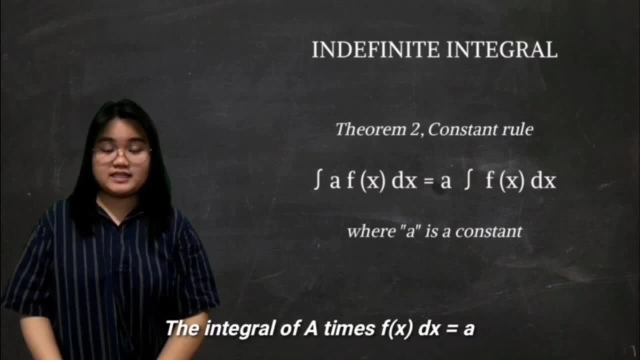 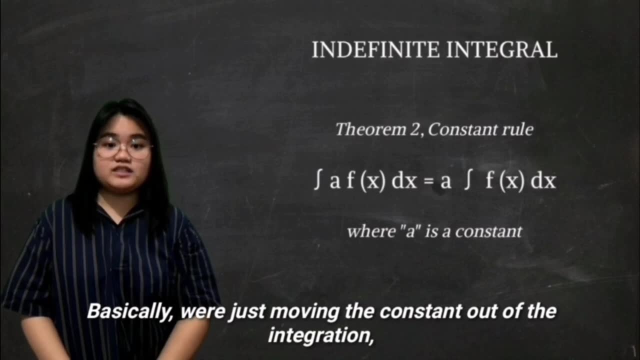 constant rule We have: the integral of a times f of x dx equals a times the integral of f of x? dx, where a is a constant. Basically, we're just moving the constant out of the. For a better understanding, let's move on to the examples. 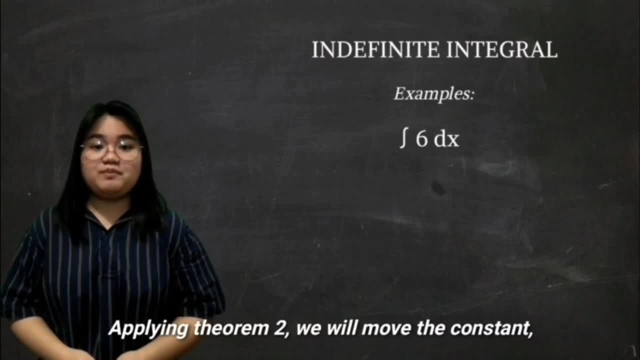 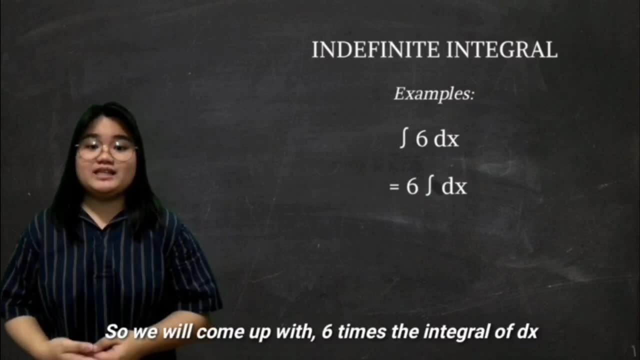 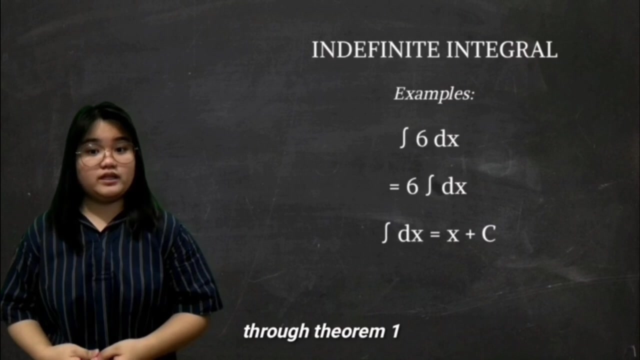 Let us evaluate the integral of 6 dx. Apply theorem 2.. We will move the constant, which is 6, outside of the integration, So we will come up with 6 times the integral of dx. Since the integral of dx is equal to x plus c through theorem 1,. 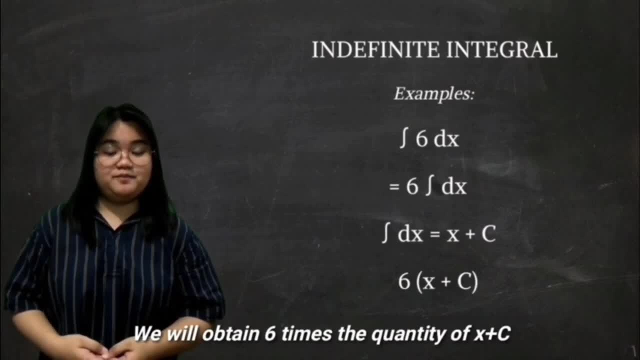 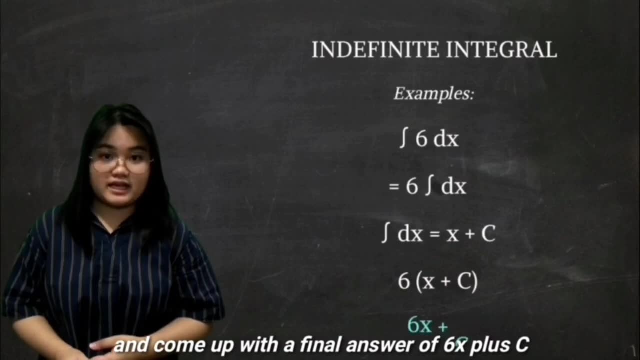 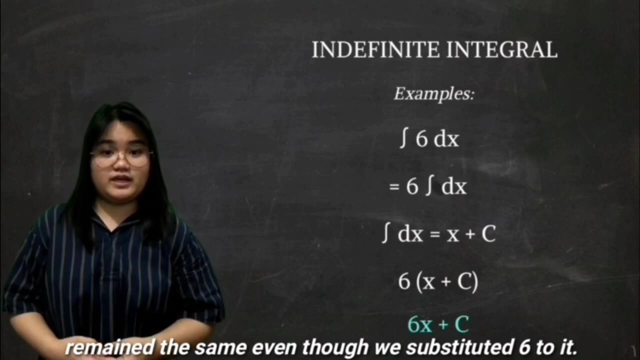 we will obtain 6 times the quantity of x plus c. We can substitute 6 to the quantity of x plus c and come up with the final answer of 6x plus c. We can see that the arbitrary constant remains the same even though we substitute 6 to it. 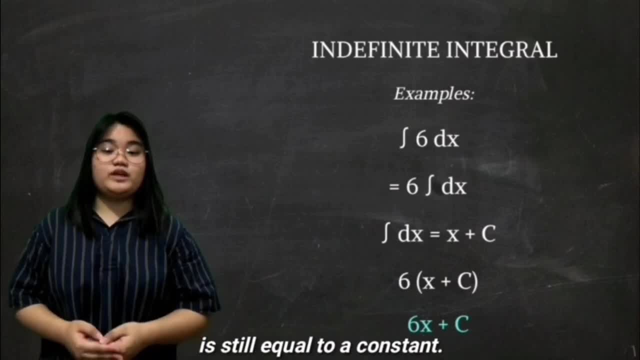 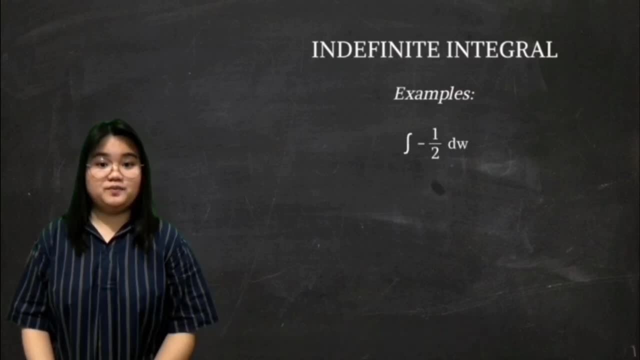 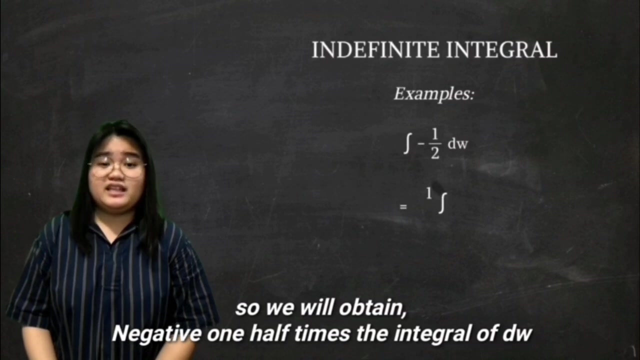 This happened because 6 times c is still equal to the constant. For the next example, we have the integral of negative 1 half dw. Again, by limit theorem 2, we will move negative 1 half out of dx. So we will obtain negative 1 half times the integral of dw. 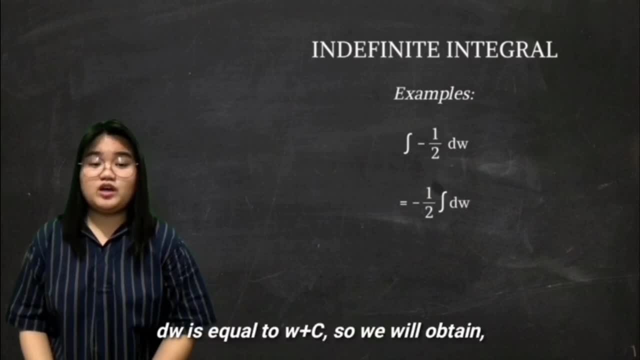 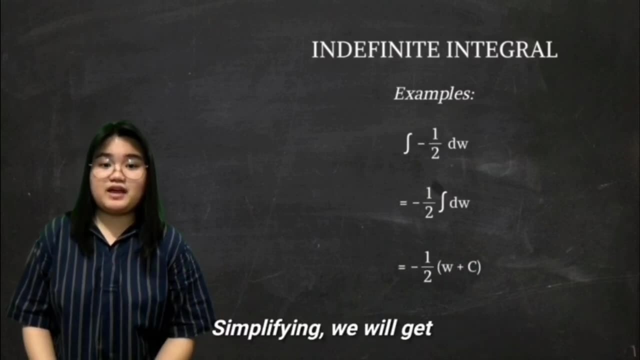 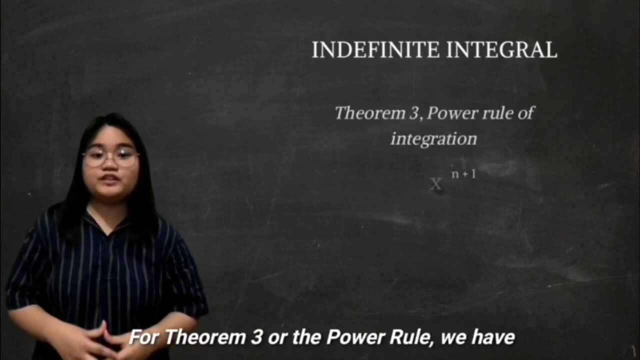 Through limit. theorem 1, dw is equal to w plus c, So we will obtain negative 1 half times the quantity of w plus c. Simplifying, we will get negative 1 half w plus c as our final answer For theorem 3, or the power rule. 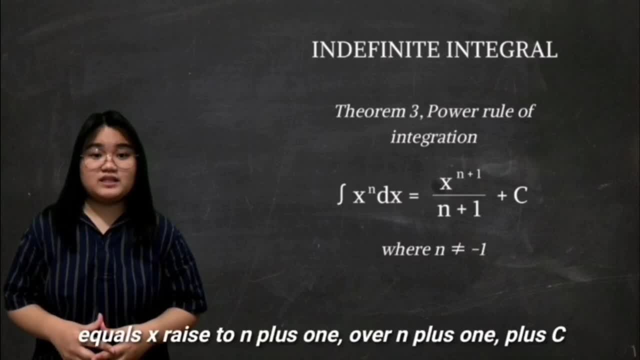 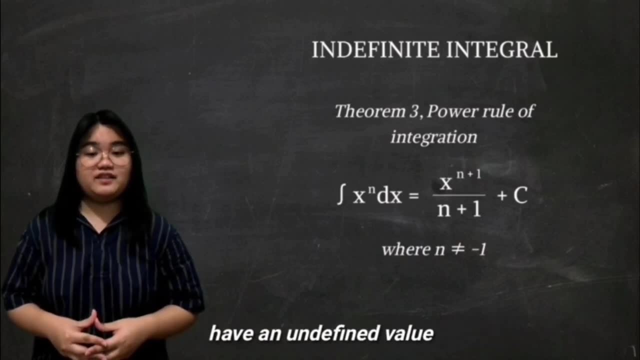 we have the integral of x raised to the n dx equals x raised to the n dx, So we will have n plus 1 over n plus 1 plus c, Where n cannot be equal to negative 1, since we will have an event value. 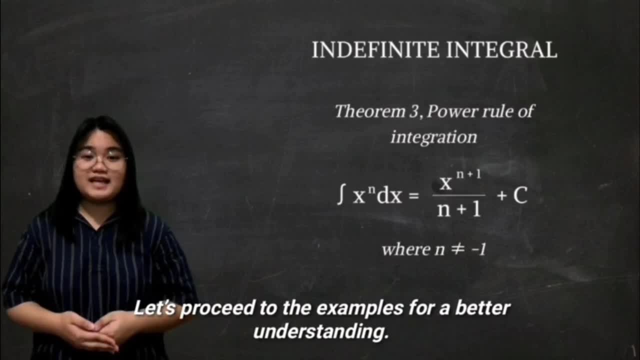 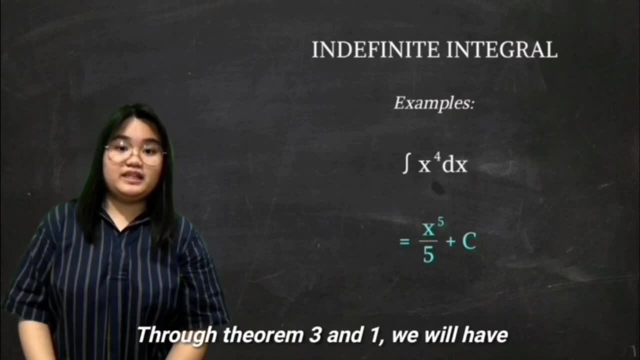 Let's proceed to the examples for a better understanding. So over, here we have the integral of x raised to 4 dx using the power rule in theorem 1.. We will have x raised to 4 plus 1 over 4 plus 1 plus c. 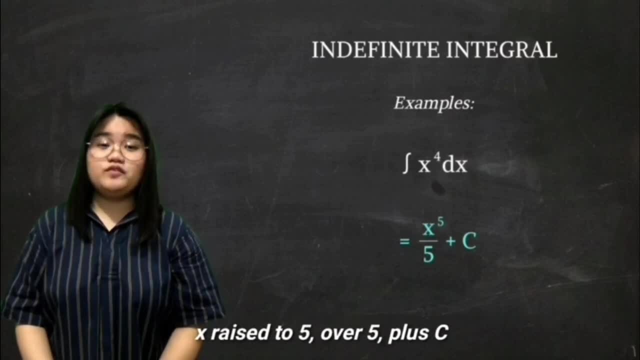 By simplifying, we will get x raised to 5 over 5 plus c. as our final answer For the next example, we have the integral of x raised to 4 plus 1 over 4 plus 1 plus c. We will have x raised to 4 plus 1 over 4 plus 1 plus c. 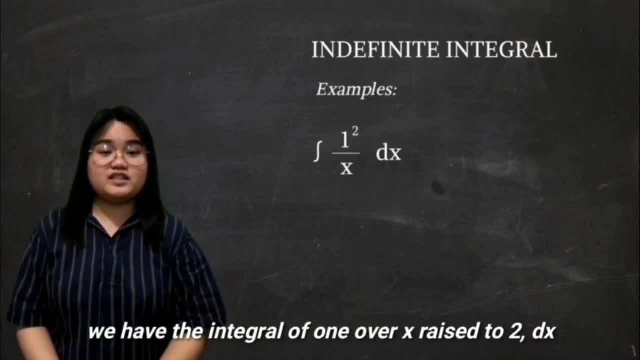 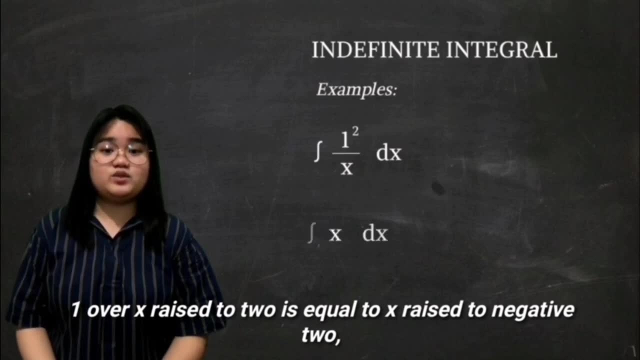 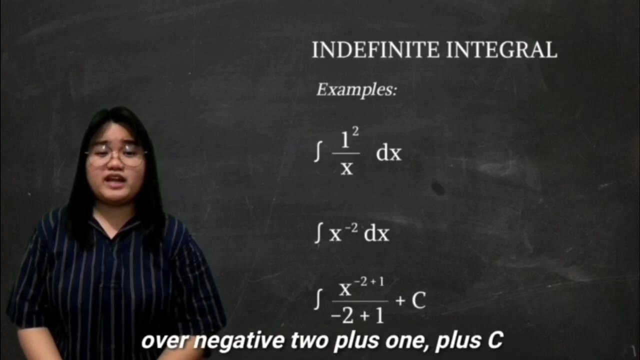 For the next example, we have the integral of 1 over x raised to 2, dx. By the loss of exponent, 1 over x raised to 2 is equal to x raised to negative 2.. By theorem 3 and 4, we will obtain x raised to negative, 2 plus 1 over negative, 2 plus 1 plus c. 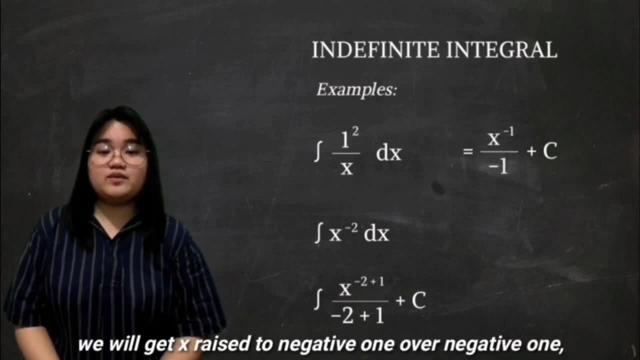 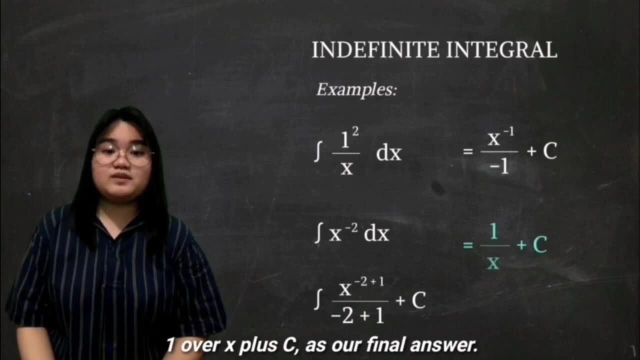 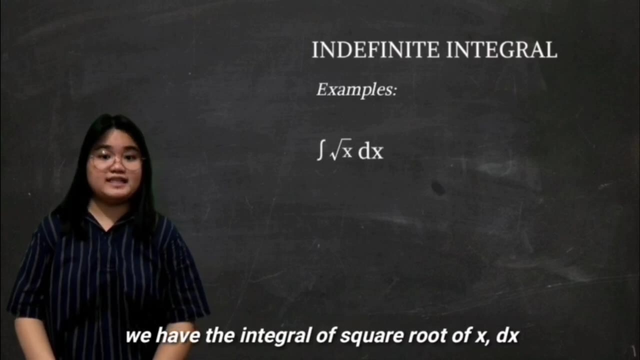 Solving the equation, we will get x raised to negative, 1 over negative, 1 plus c. Again by simplifying, we will obtain 1 over X plus C. as our final answer For the next example, we have the integral of square root of X to X. 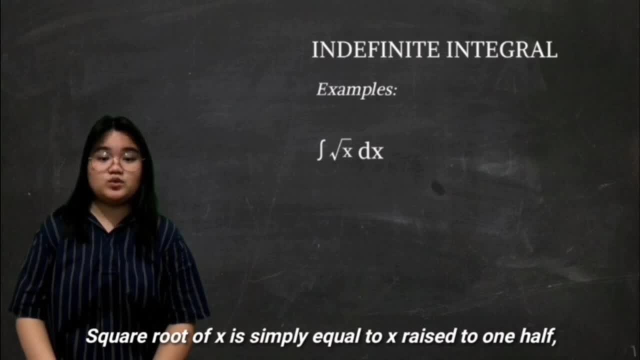 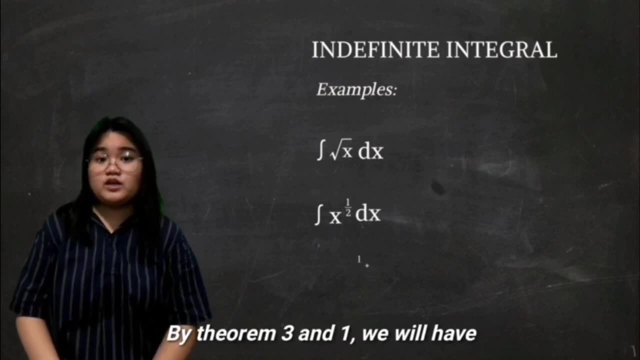 Square root of X is simply equal to X raised to 1 half, so we will have the integral of X raised to 1 half to X By theorem 3 and 1, we will obtain X raised to 1 half plus 1 over 1 half plus 1 to C. 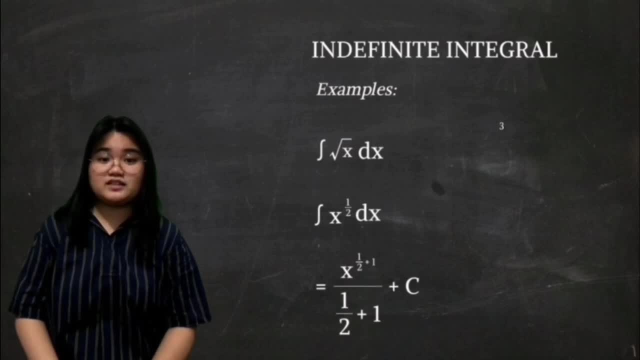 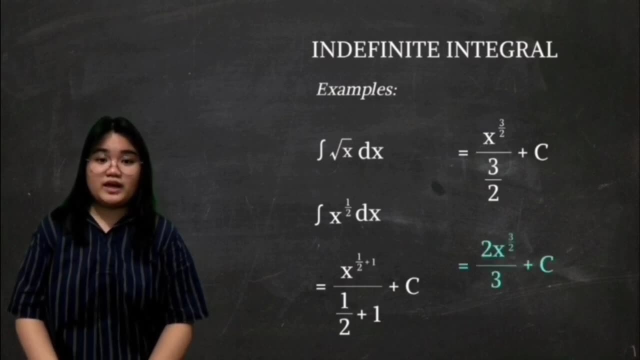 Solving the equation, we will get X raised to 3 over 2 over 3 over 2 plus C. We will then simplify so we will get 2 X raised to 3 over 2 over 3 plus C as our final answer. 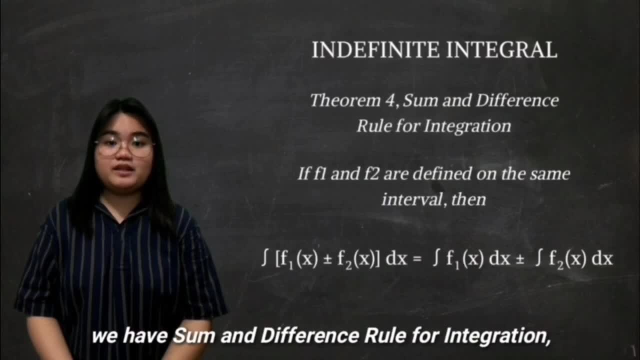 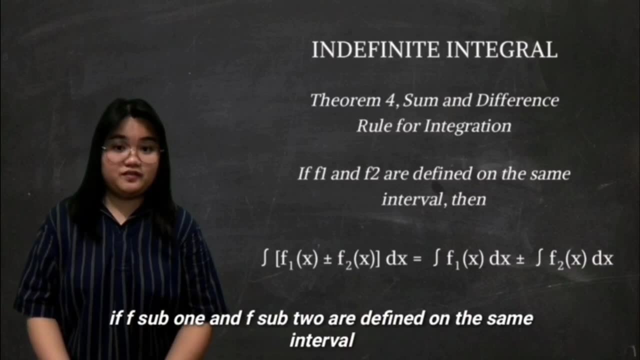 For theorem 4, we have the sum and difference rule for integration. This states that if F sub 1 and F sub 2 are defined in the same interval, then the integral of F sub 1 of X will be equal to X raised to 1 half plus 1 half to X. 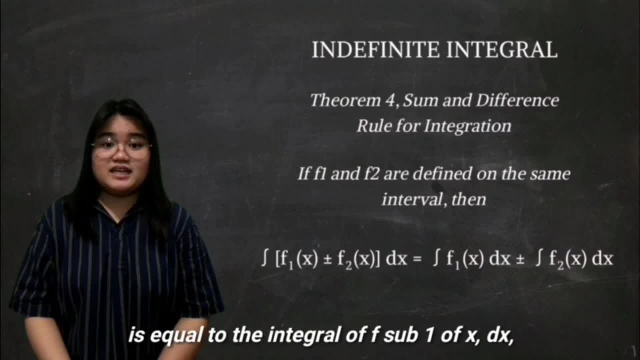 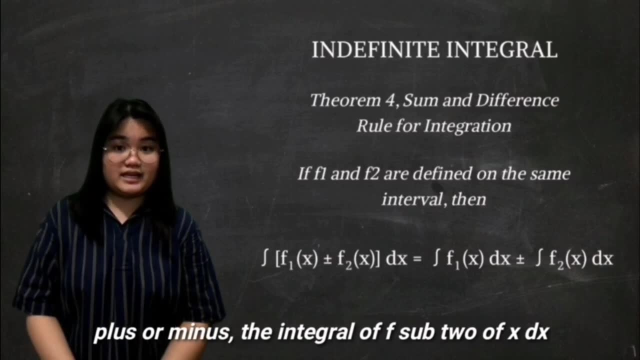 Plus or minus F sub 2 of X to X is equal to the integral of F sub 1 of X to X, plus or minus the integral of F sub 2 of X to X. Basically, we are just distributing the integral to the functions in this equation. 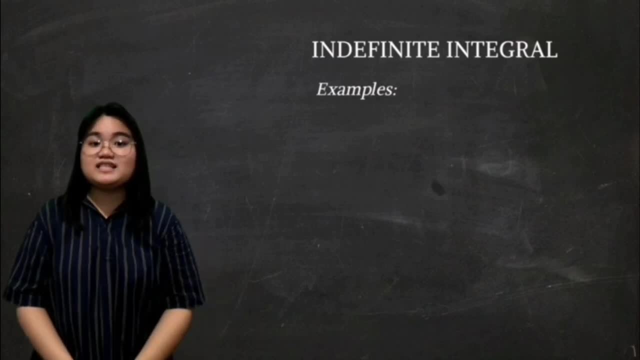 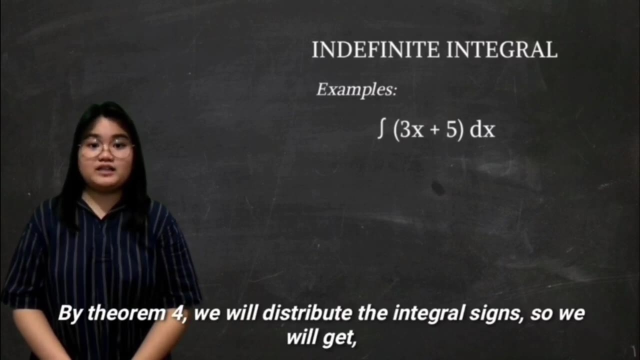 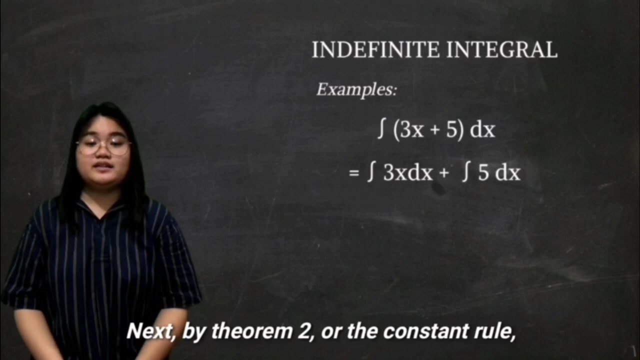 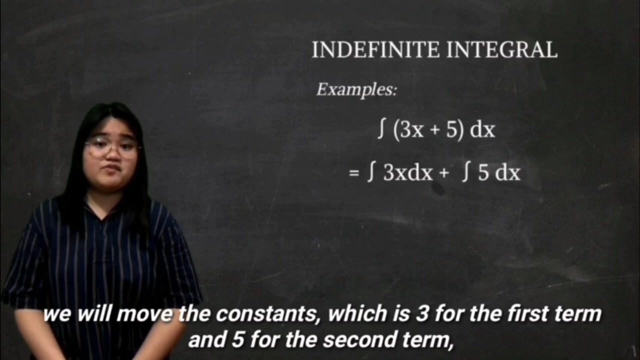 So let us proceed to the examples. Let us evaluate the integral of 3X plus 5 to X By theorem 4, we will distribute the integrals, so we will get the integral of 3X to X. Next, by theorem 2 or the constant rule, we will move the constants, which is 3 for the first term and 5 for the second term, outside of the integration. 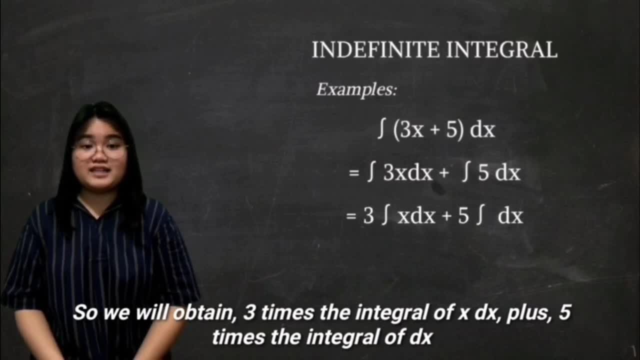 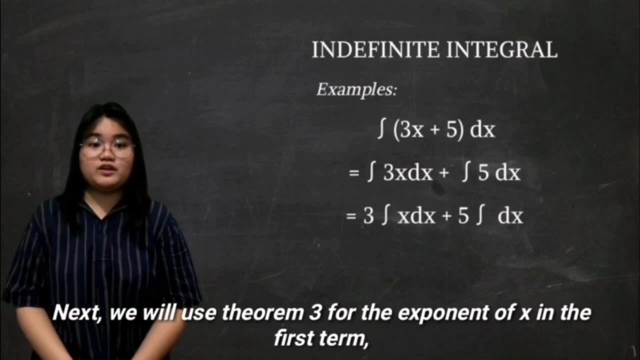 So we will obtain 3 times the integral of X to X plus 5 times the integral of T to X. Next we will use theorem 3 for the exponent of X in the first term. So we will come up with 3 times the integral of X raised to 1 plus 1.. 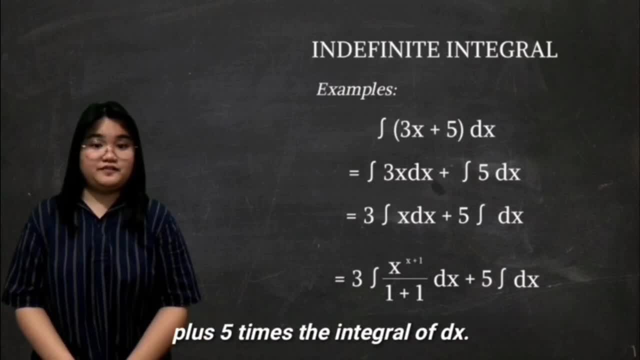 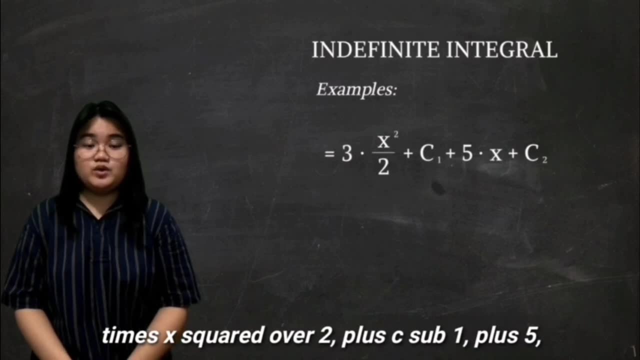 So we will get 3 times the integral of X to X plus 5 times the integral of T to X. By solving and by theorem 1,, we will get 3 times X squared over 2 plus C sub 1, plus 5 times X plus C sub 2.. 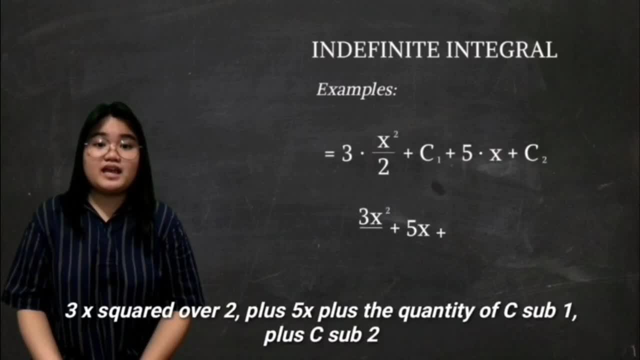 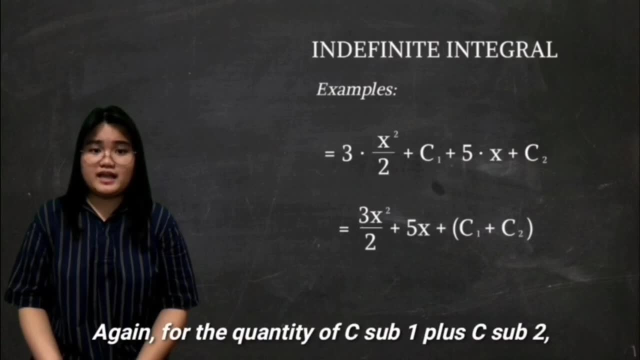 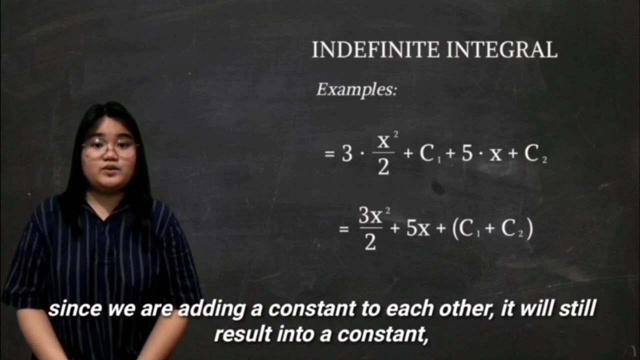 Simplifying and attaching it, we will obtain 3X squared over 2 plus 5X, plus the quantity of C sub 1 plus C sub 2.. Again for the quantity of C sub 1 plus C sub 2.. Since we are adding a constant to each other, it will still result into a constant. 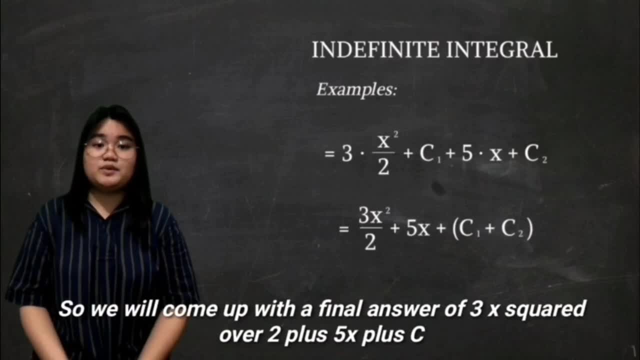 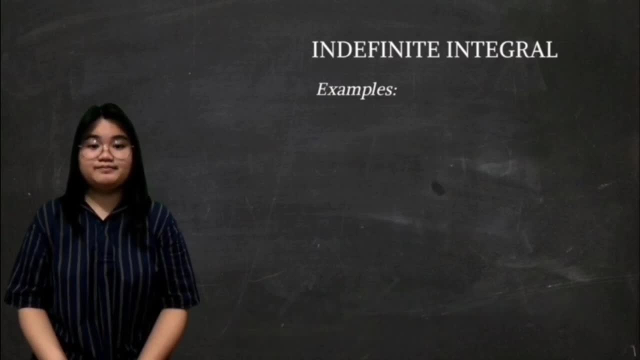 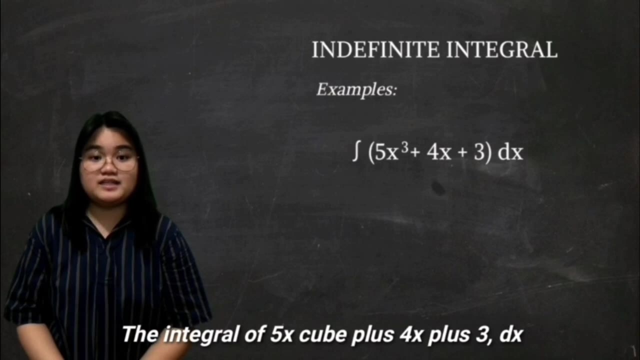 So we can just denote it as C. So we will come up with a final answer of 3X squared over 2 plus 5X plus C. For our final example, we have the integral of 5X cubed plus 4X plus 3DX. 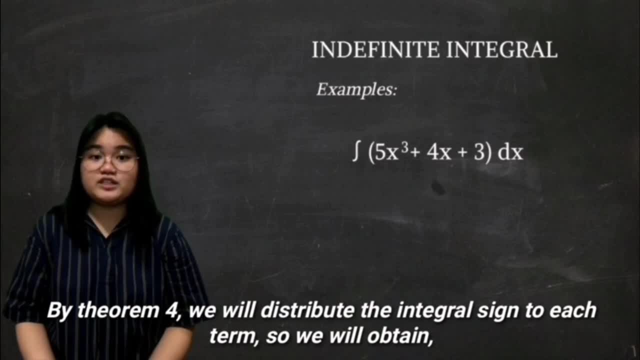 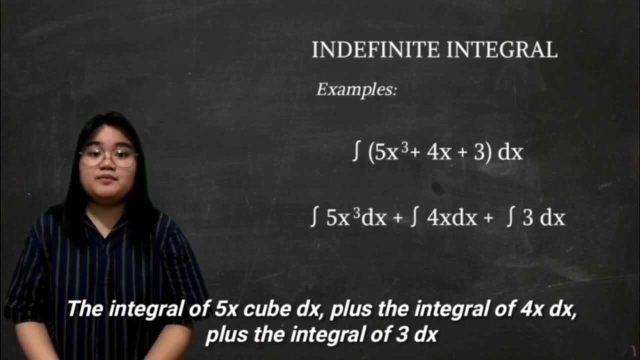 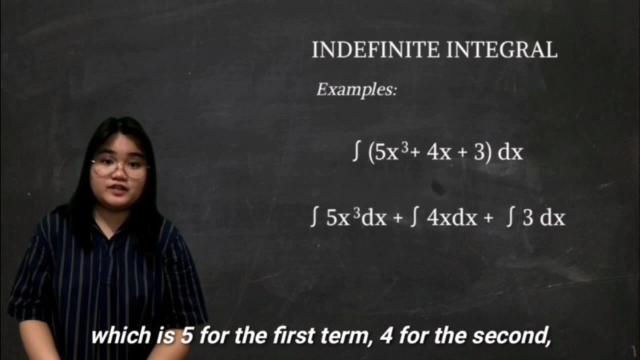 By theorem 4, we will distribute the integral side to each term. We will obtain the integral of 5X cubed plus the integral of 4X cubed plus the integral of 3DX. Next, by theorem 2, we will move the constants, which is 5 for the first term, 4 for the second term and 3 for the third term, out of the equation. 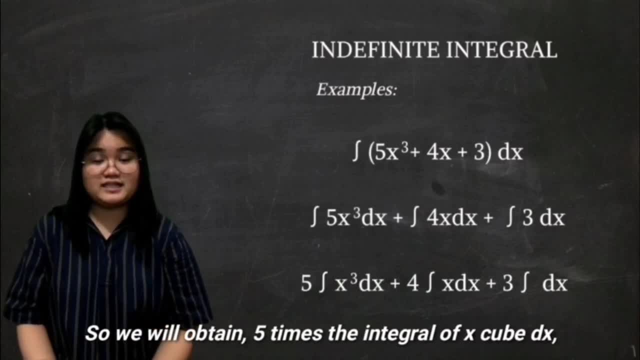 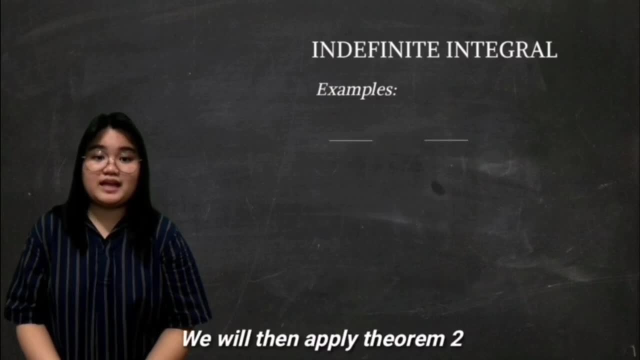 So we will obtain 5 times the integral of X cubed, plus 4 times the integral of XDX, plus 3 times the integral of DX. We will then apply theorem 2.. And by solving and at the same time applying theorem 1,. 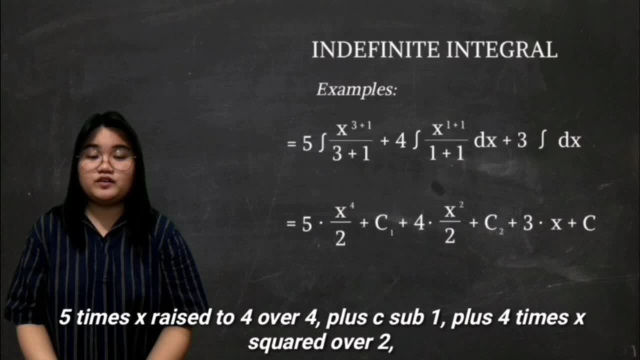 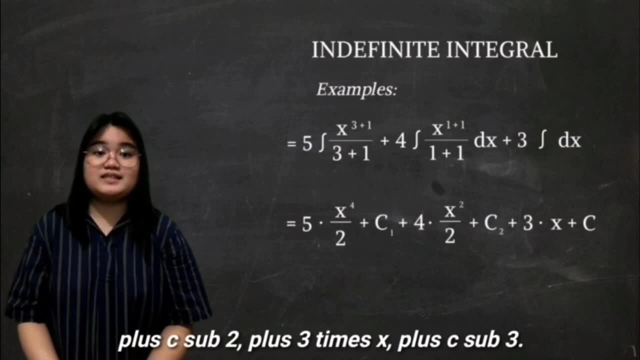 we will obtain 5 times X raised to 4 over 4 plus C sub 1, plus 4 times X squared over 2 plus C sub 2, plus 3 times X plus C sub 3.. Simplifying and rearranging the equation: 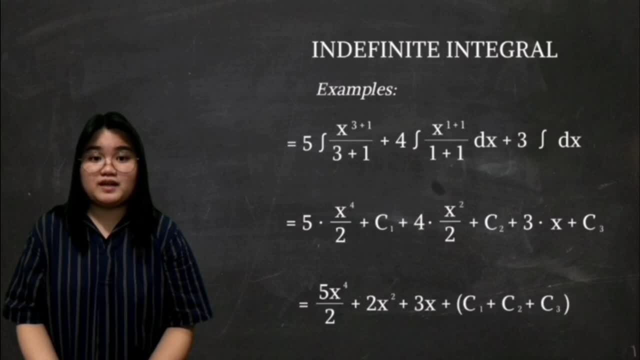 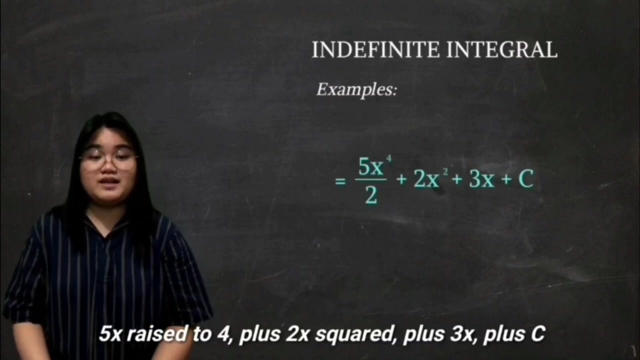 we will obtain 5X raised to 4 over 4 plus 2X, squared plus 3X, plus the quantity of C sub 1 plus C sub 2 plus C sub 3.. For the final answer, we have 5X raised to 4 over 4 plus 2X, squared plus 3X plus C. 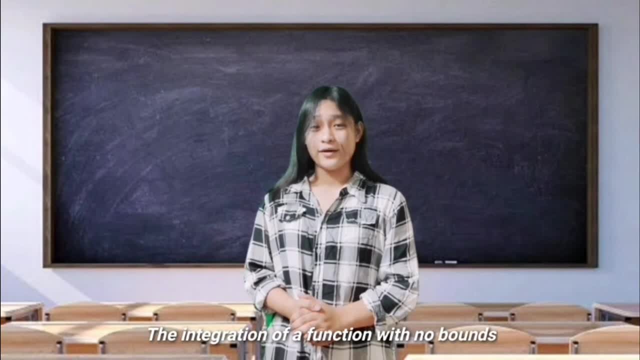 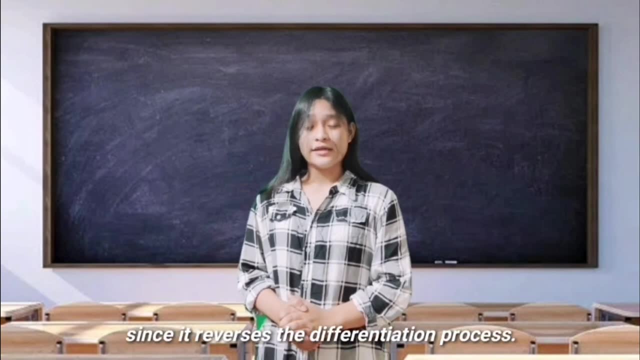 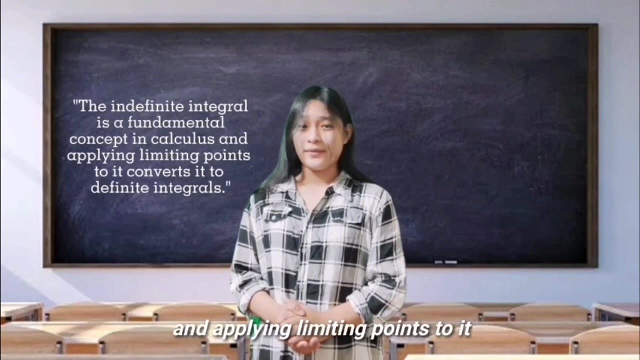 The integration of a function with no bounds is known as an indefinite integral. Integration is the antiderivative of a function, since it reverses the differentiation process. The indefinite integral is a fundamental concept in calculus. In applying limiting functions and applying limiting points to it, converts it to definite integral. 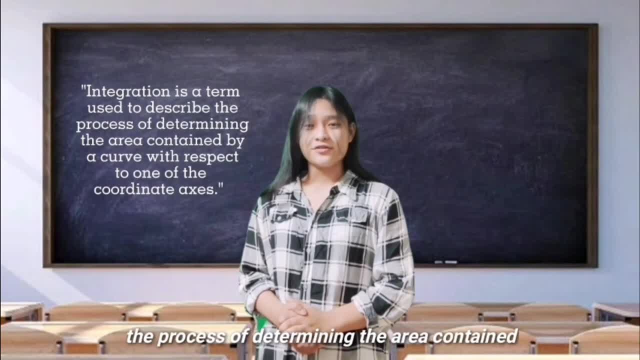 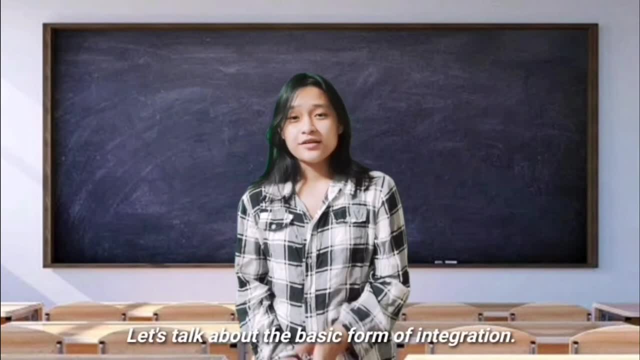 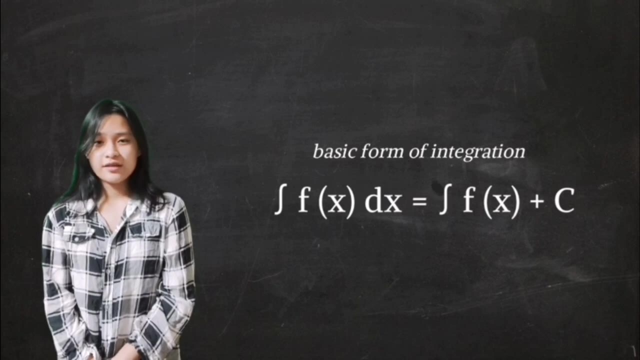 Integration is a term used to describe the process of determining the area contained by a curve with respect to one of the coordinate axes. Let's talk about the basic form of integration, The indefinite integral of F. with respect to X, We have F. DX is equal to the antiderivative of F plus the arbitrary constant C. 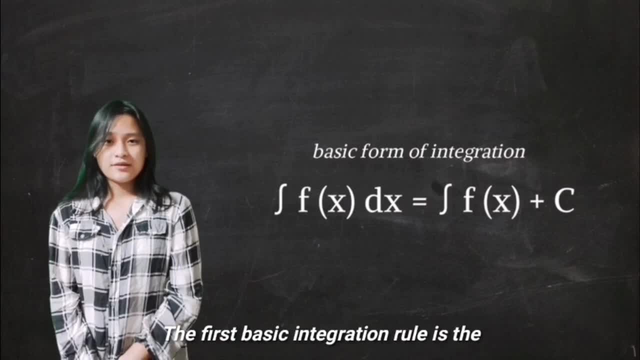 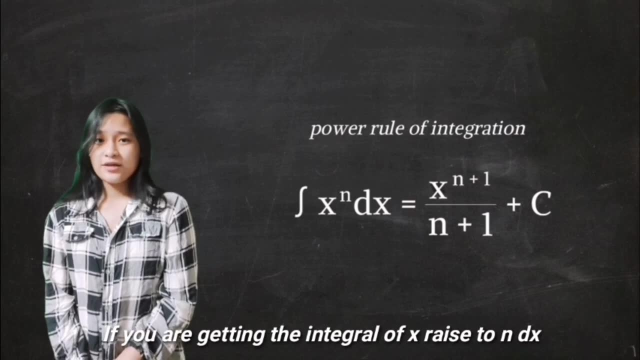 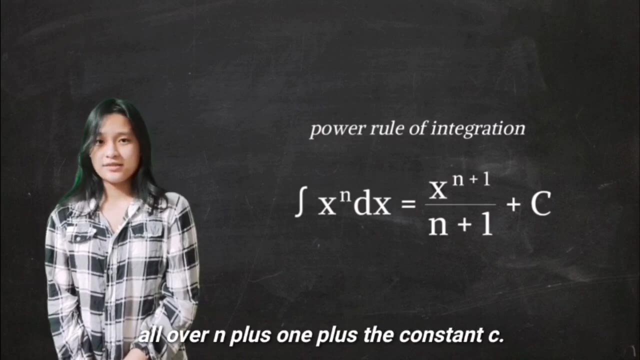 The first basic integration rule is the power rule of integration. If you are getting the integral of X raised to N DX, it is just equal to X raised to N plus 1. all over N plus 1 plus the constant C, For example, we have the integral of X raised to 7 DX. 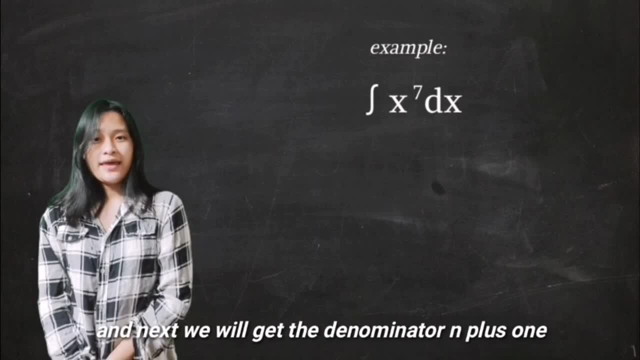 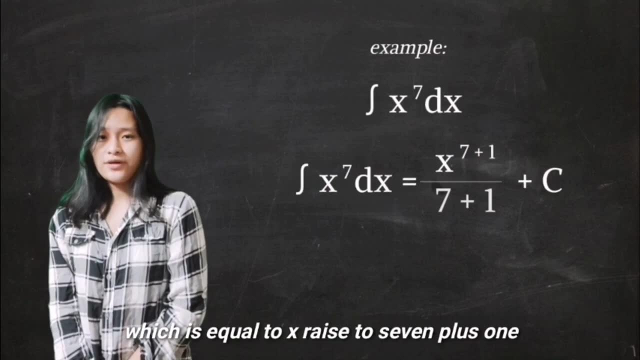 So first we will get the X raised to N plus 1 and the denominator N plus 1.. And then the constant C, Which is equal to X raised to 7 plus 1, all over 7 plus 1 plus the constant C. 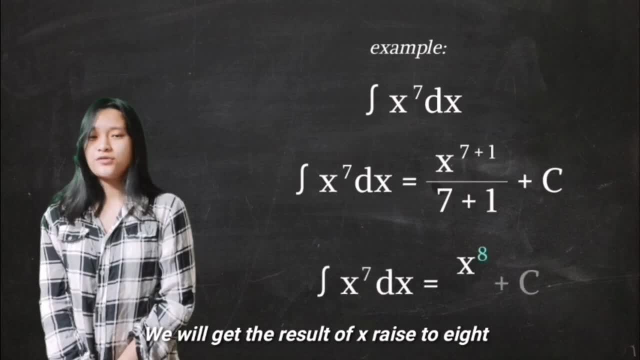 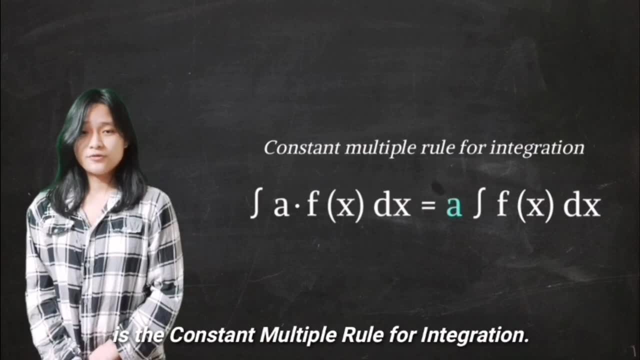 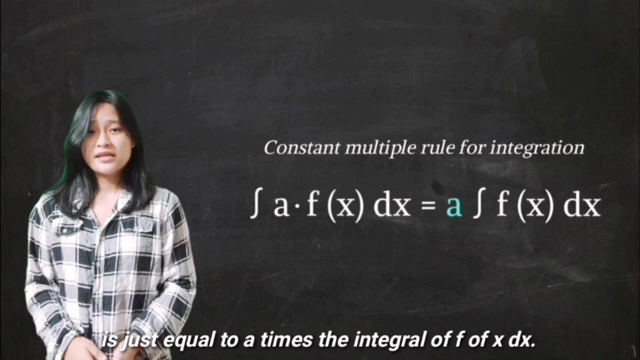 We will get the result of X raised to 8, all over 8 plus the constant C. The next rule of integration is the constant multiple rule for integration. The integration of A multiplied to F- DX is just equal to A times the integral of X- DX. 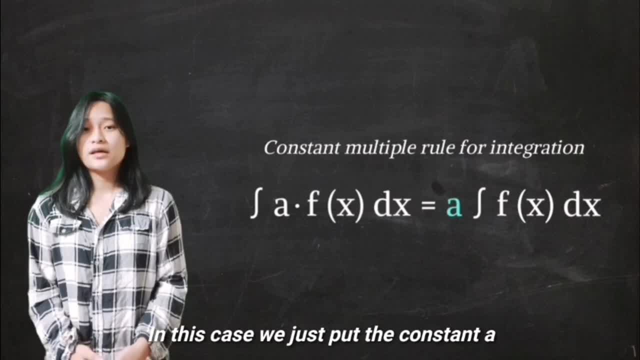 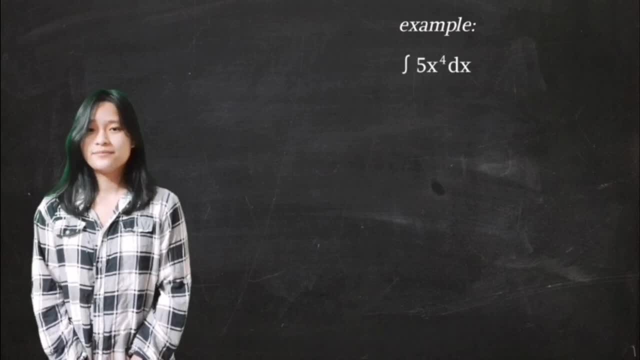 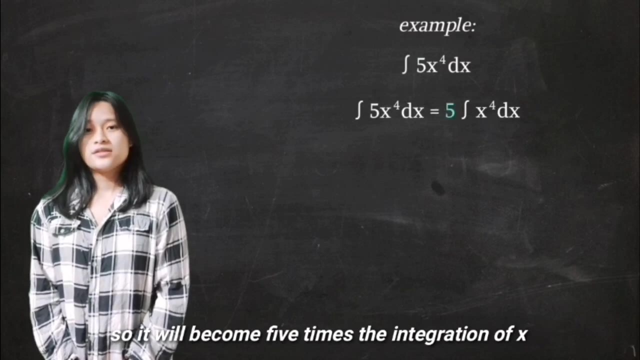 In this case we just put the constant A outside the integration. For example, we have the integral of 5X raised to 4 DX. First we will put the constant outside the integration, So it will become 5 times the integration of X raised to 4 DX. 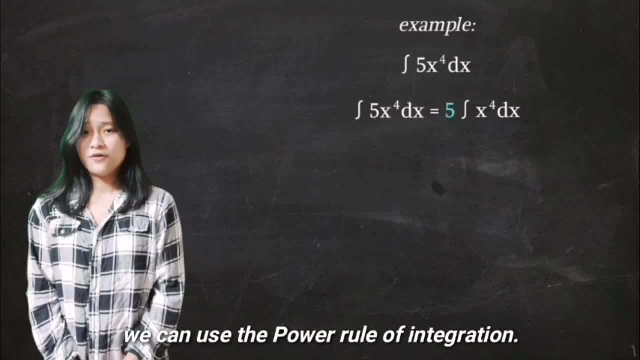 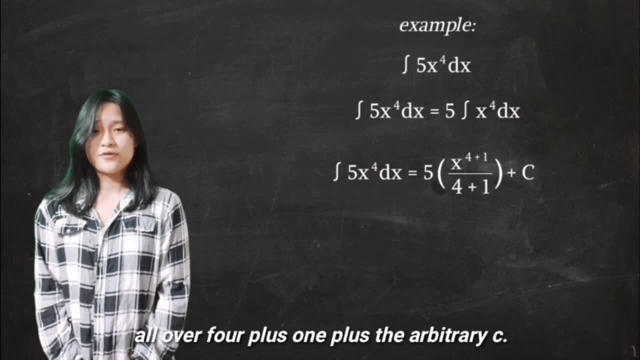 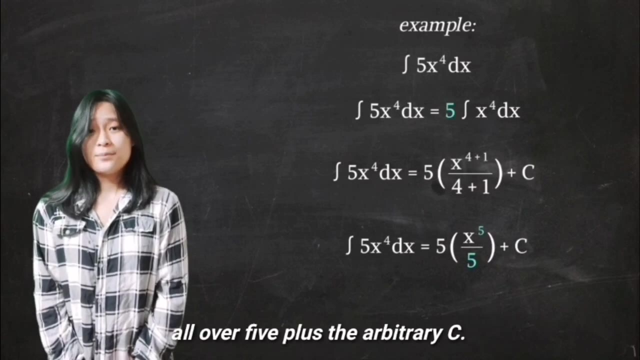 In this case we can use the power rule of integration. It will become 5 times the X raised to 4 plus 1 DX. All over 4 plus 1 plus the arbitrary C, We will get 5 times X raised to 5. all over 5 plus the arbitrary C. 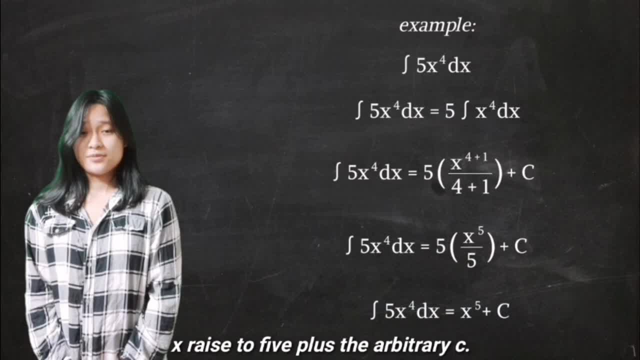 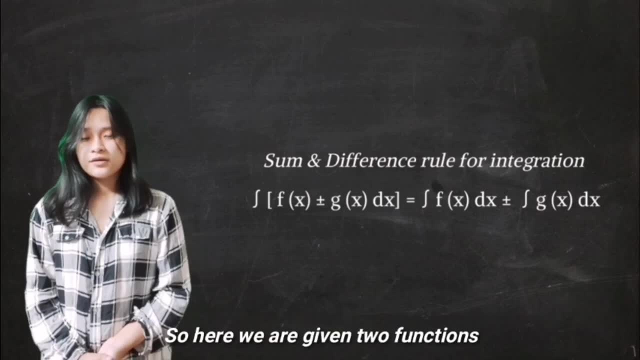 If we simplify it, we can get X raised to 5 plus the arbitrary C. The next rule is the sum and difference rule for integration. So here we are given two functions, Which is the F of X and the G of X. 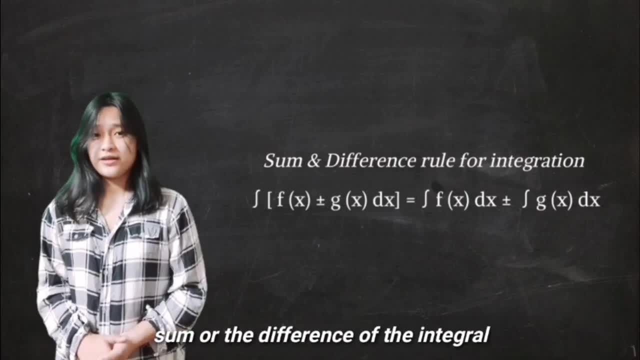 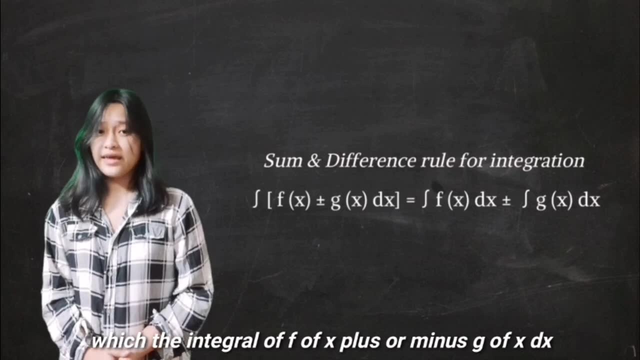 From the name itself, we will get the sum or difference of the integral, Which, the integral of F of X plus or minus G of X- DX, is just equal to the integral of F of X- DX, plus or minus the integral of G of X- DX. 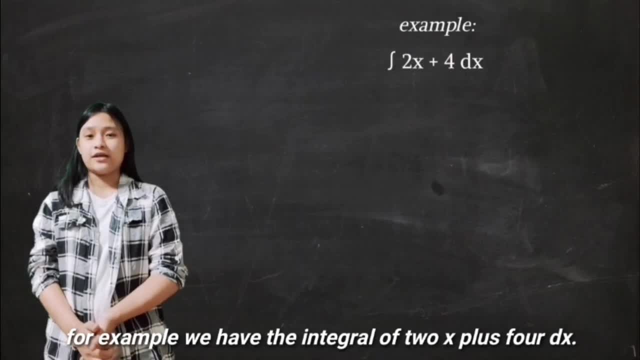 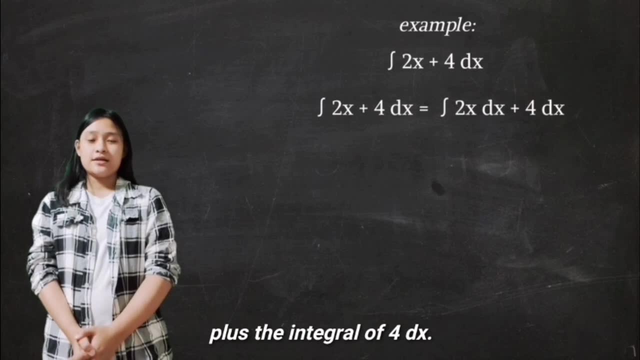 For example, we have the integral of 2X plus 4 DX. First we will separate them, Which will be equal to the integral of 2X DX plus the integral of 4 DX. Second, we can apply the equation. 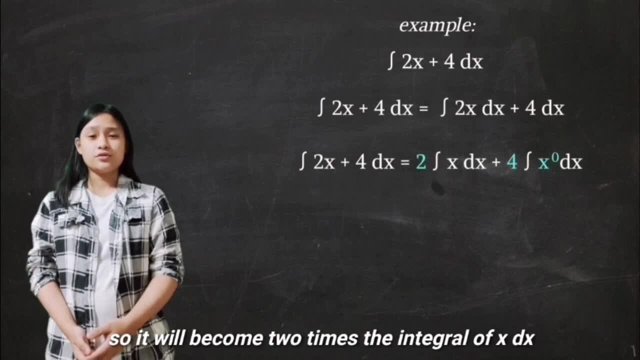 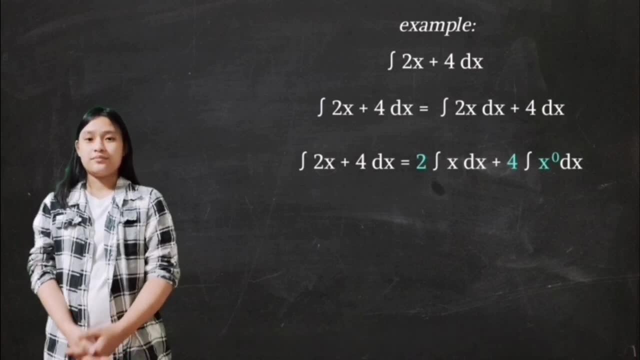 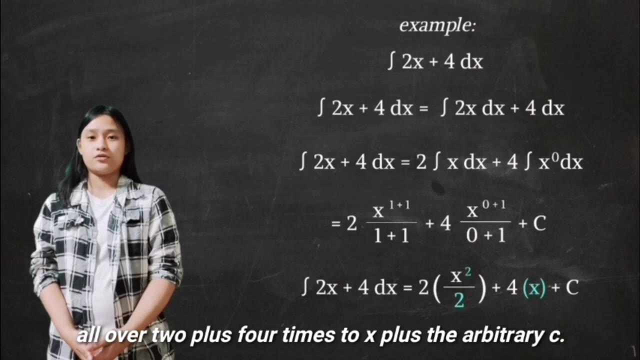 The constant multiple rule. So it will become 2 times the integral of X, DX, plus 4 times the integral of X raised to 0, DX. Now we can perform the power rule. It will become 2 times X raised to 2, all over 2 plus 4 times X plus the arbitrary C. 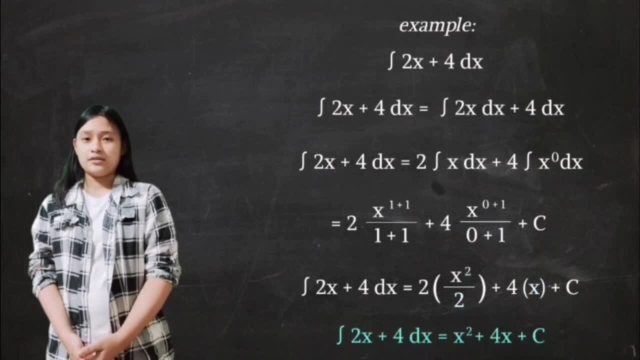 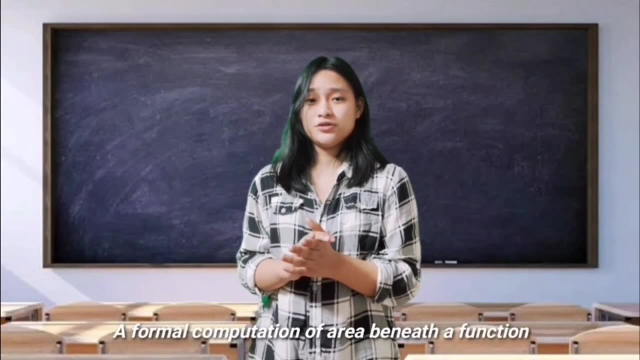 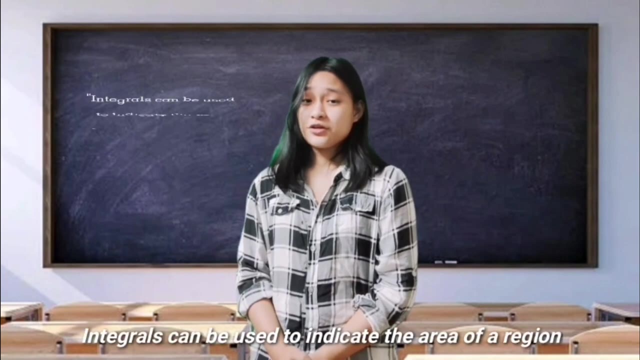 And we will get the result of X squared plus 4X plus the arbitrary C. A formal computation of area beneath a function using microscopic slivers or stripes of the region is known as a definite integral. Integrals can be used to indicate the area of the region. 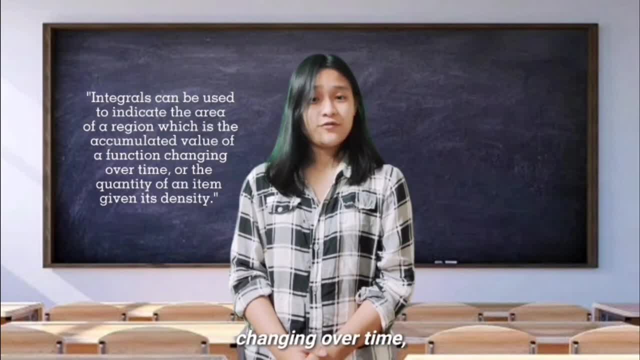 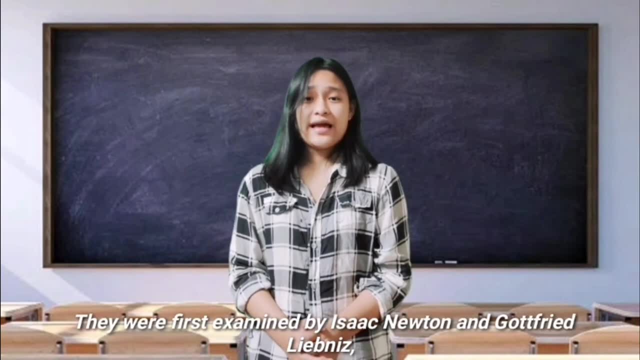 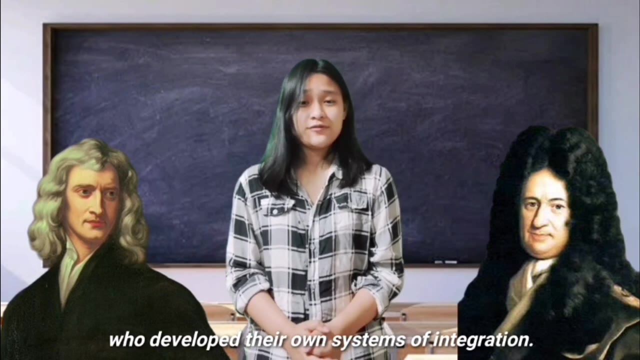 which is the accumulated value of a function changing over time, or the quantity of an item given its density. There were first examined by Isaac Newton and Gaffrey Leibniz, two of the 17th century mathematicians who developed their own systems of integration. 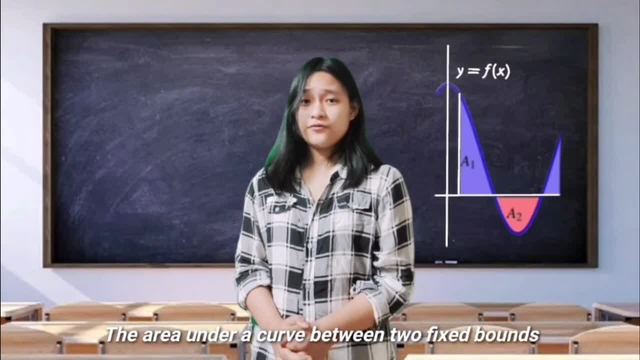 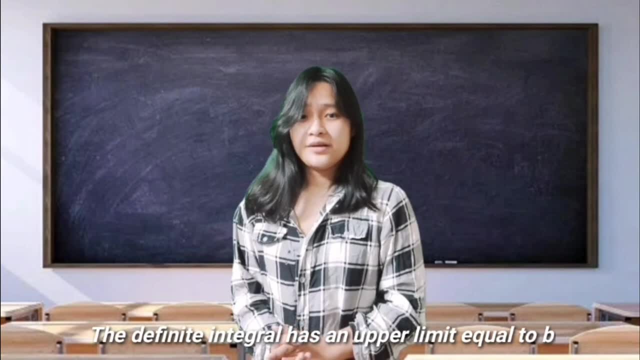 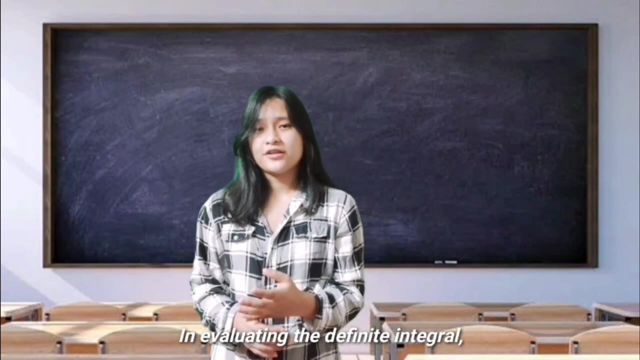 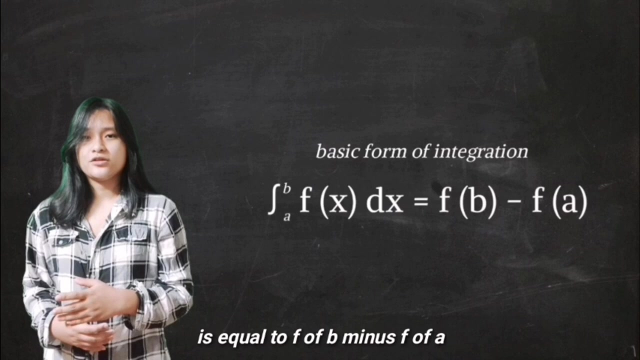 The area under a curve between two fixed bounds is called the definite integral. The definite integral has an upper limit equal to B and a lower limit equal to A. In evaluating the definite integral, we have a form of integral of F of X. DX from A to B is equal to F of B minus F of A. 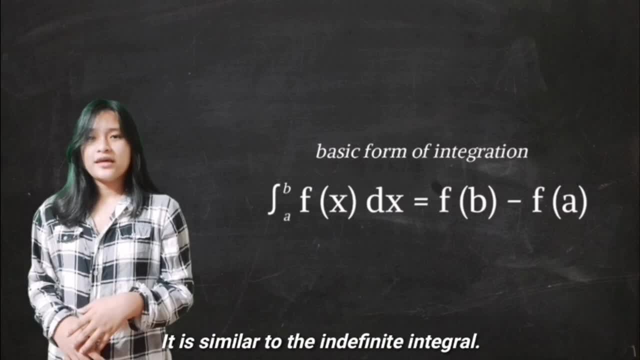 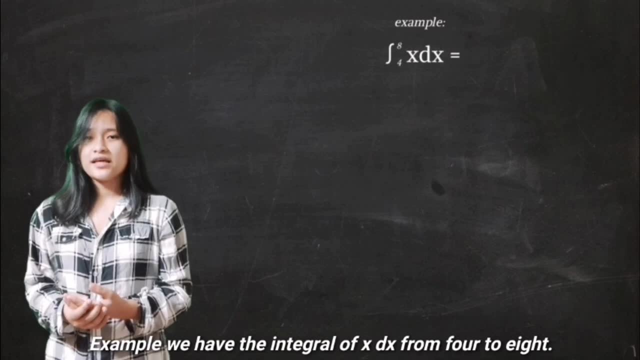 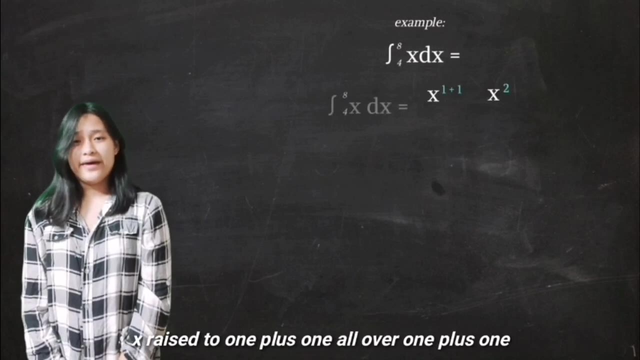 In evaluating the definite integral. it is similar to the indefinite integral. For example, we have the integral of X, DX from 4 to 8.. First we will apply the power rule, So it will become X raised to 1 plus 1, all over 1 plus 1.. 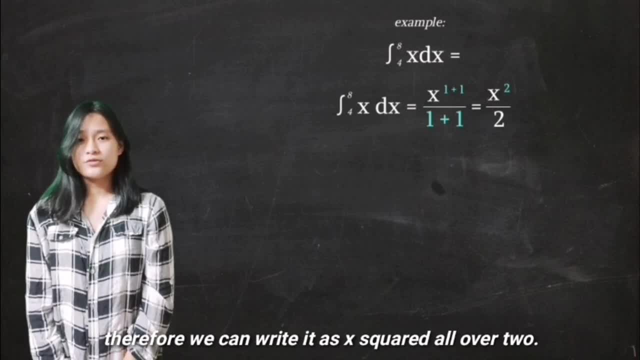 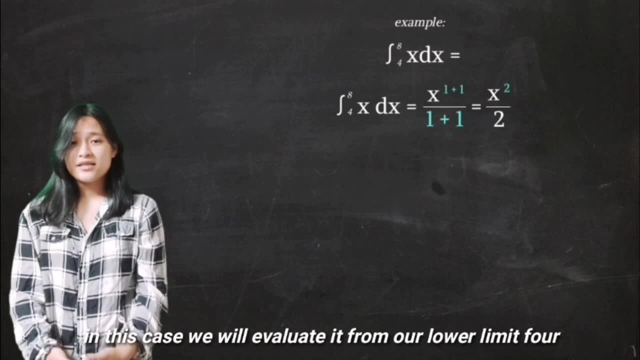 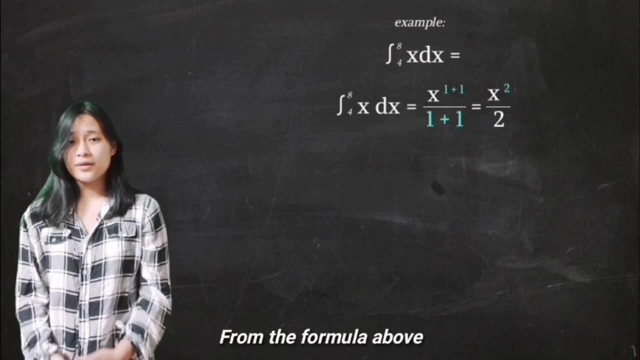 Therefore, we can write it as X squared all over 2.. Since we are in definite integral, we will not write the arbitrary C In this case. we will evaluate it from our lower limit, 4, until the upper limit 8.. From the formula above: 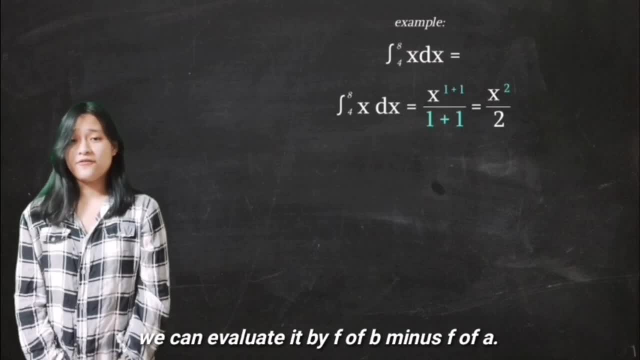 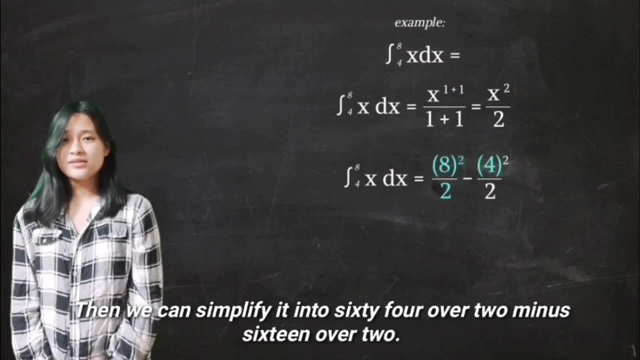 we can evaluate it by F of B minus F of A. It will become 8 squared over 2 minus 4 squared over 2.. Then we can simplify it into 64 over 2 minus 16 over 2.. We can simplify it into 32 minus 8,. 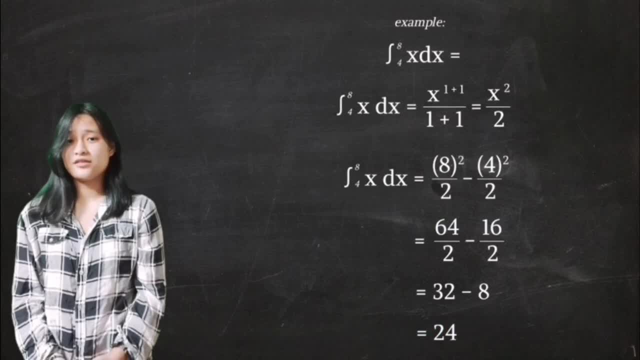 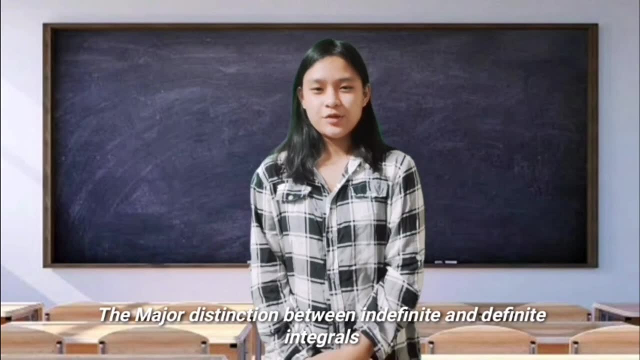 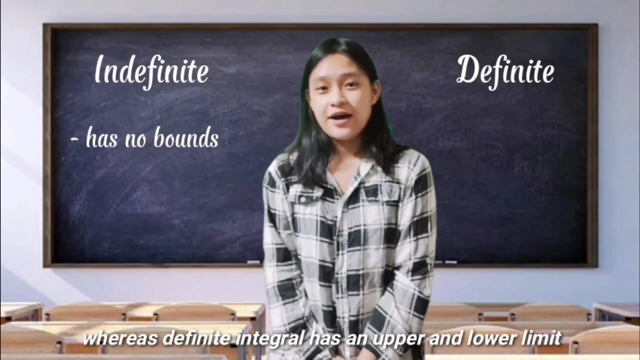 which is equal to 24.. Therefore, the integral of X, DX from 4 to 8 is equal to 24.. The major distinction between indefinite and definite integrals is that indefinite integrals have low bounds, whereas definite integrals have an upper and lower limit. 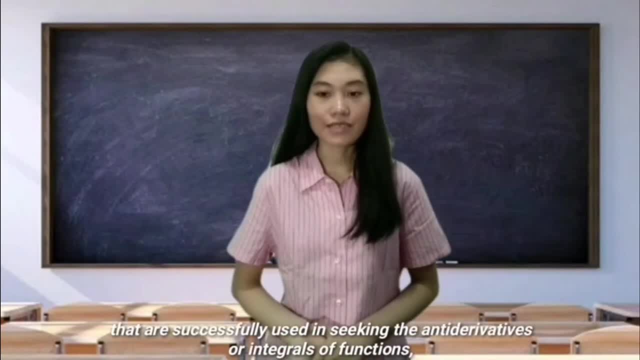 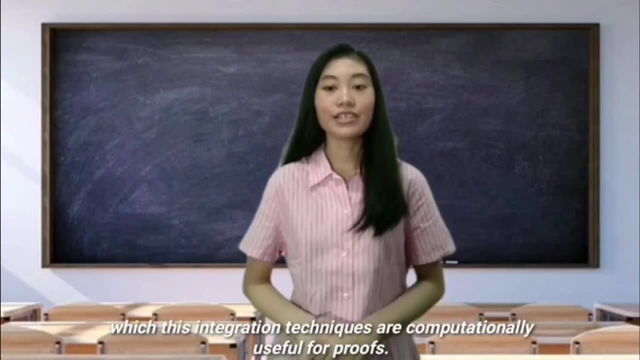 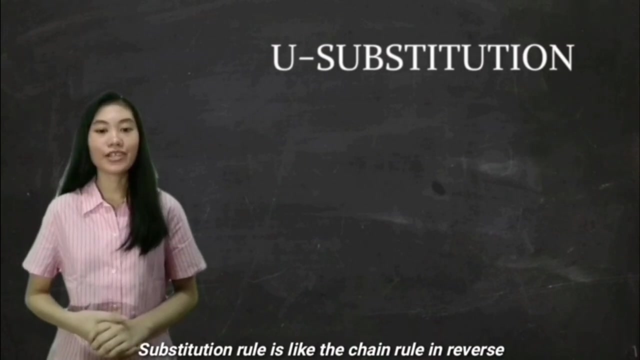 In this part of the video we will provide you some techniques that are successfully used in seeking the antiderivatives or integrals of functions, which these integration techniques are computationally used for proofs. Number 1. U-substitution- Substitution rule is like the chain rule in reverse. 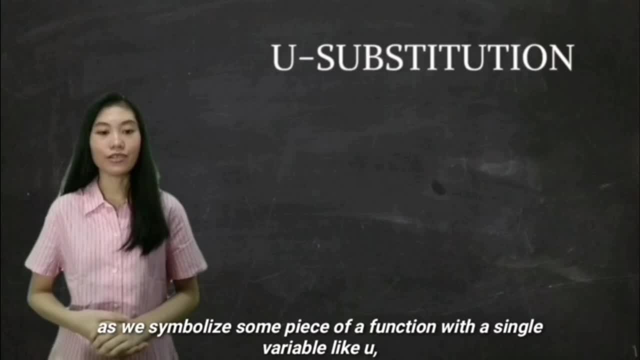 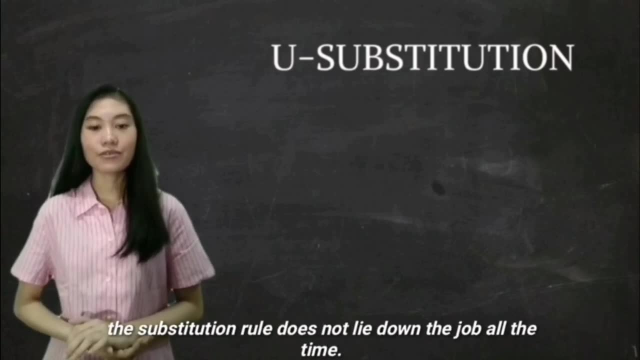 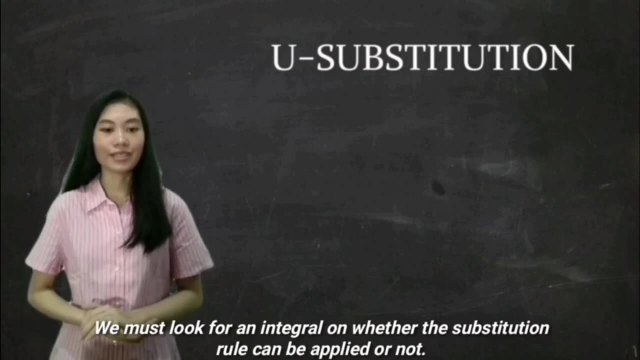 as we symbolize some feasible function with a single variable like U, allowing us to integrate more simply. Take note that while the chain rule will always work, however, the substitution rule does not lie down the job all the time. We must look for an integral on whether the substitution rule can be applied or not. 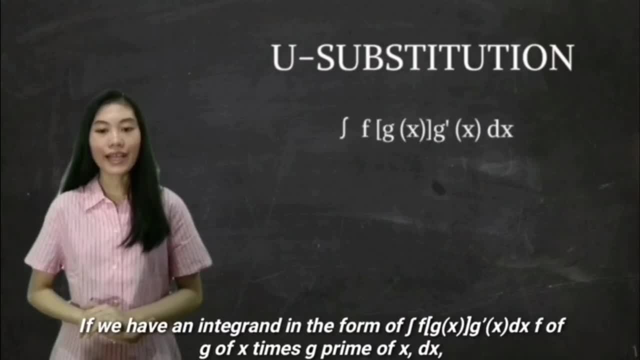 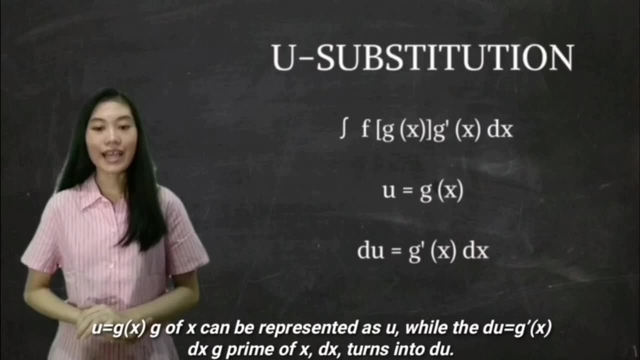 If we have an integral in the form of F of G of X times G frag of X- DX, G of X can be represented as U, while the G prime of X- DX turns into DU. then we end up with F of U- DU. 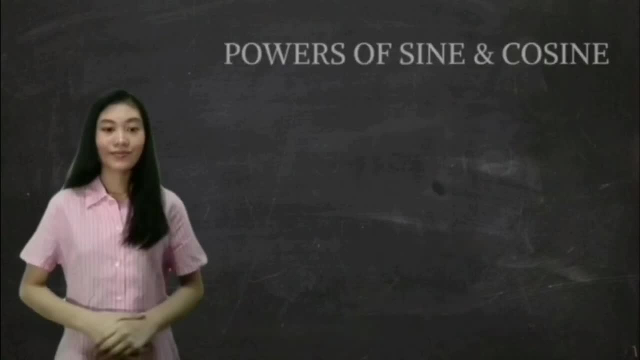 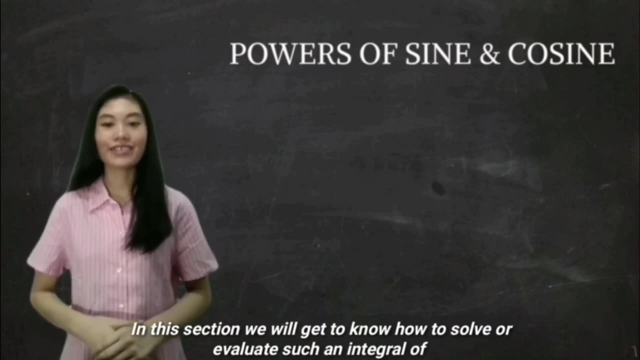 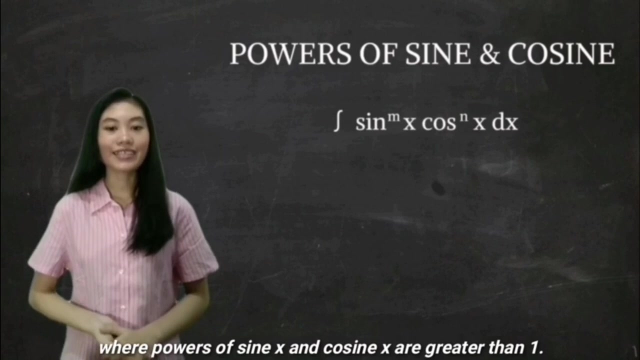 which we can integrate. Number 2. Powers of sine and cosine. In this section we will get to know how to solve or evaluate such an integral of sine raised to F of X, cosine raised to F of X, DX, where power of sine X and cosine X are greater than 1.. 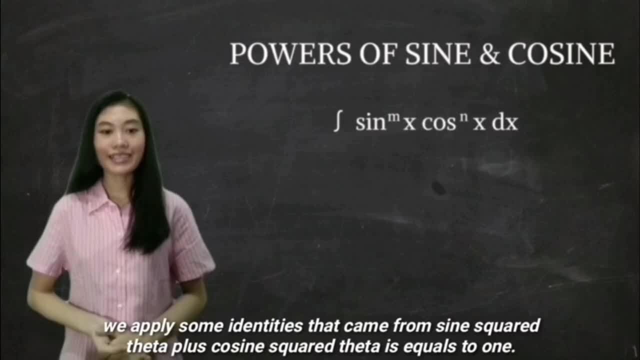 In solving this integral, we apply some identities that came from sine squared theta plus cosine squared theta is equal to 1.. We have two conditions. First condition is, if n is an odd number, split the low factor of cosine X and use the identity. 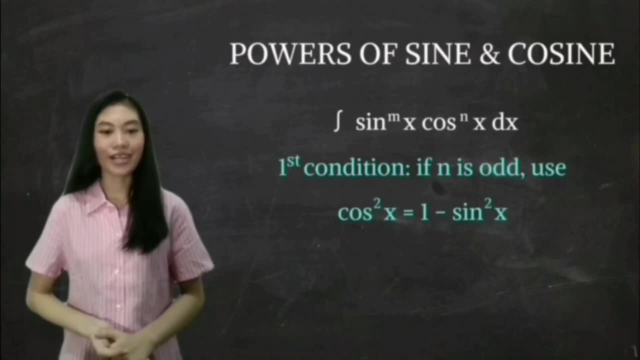 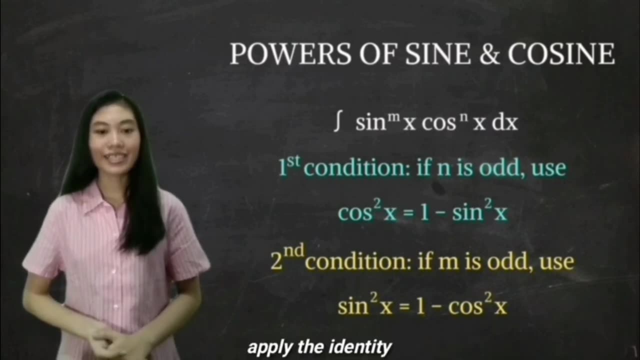 cosine squared X equals to 1 minus sine squared X. On the second case, if n is odd, split the low factor of sine X. apply the identity: sine squared X equals 1 minus cosine squared X. On the third case, if n is an odd number: 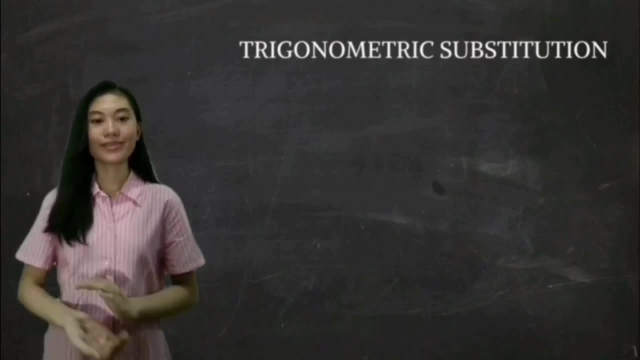 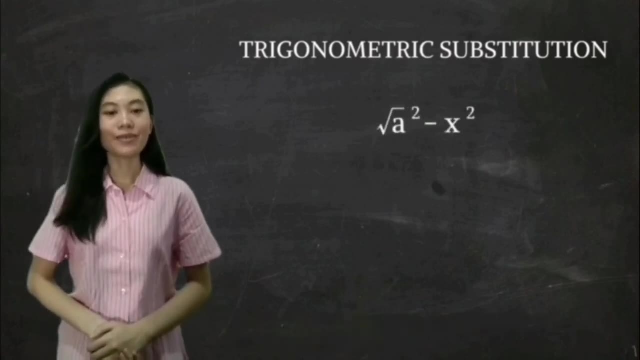 split the low factor of sine X and cosine squared X equals to 1, minus sine squared X. Number 3.. Trigonometric Substitution: This technique works in one of the three specific terms present in the integral. These are: square root of A squared minus X squared. 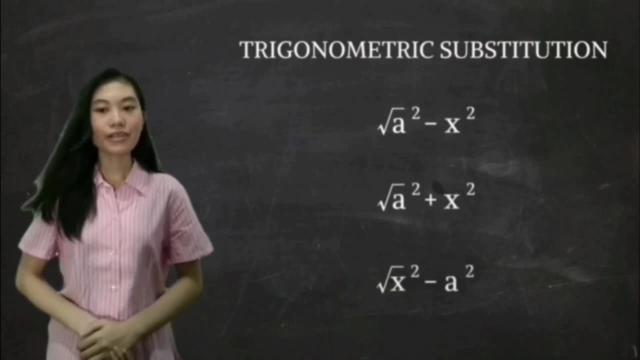 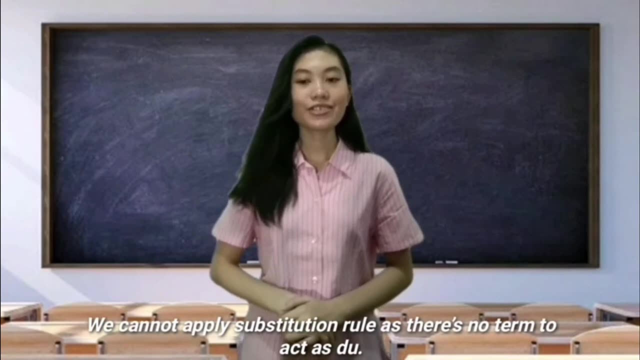 square root of A squared plus X squared, or square root of X squared minus A squared. A can be any positive number. We cannot apply substitution rule, as there is no term to act as DU. However, we can change X into something else that is positive. 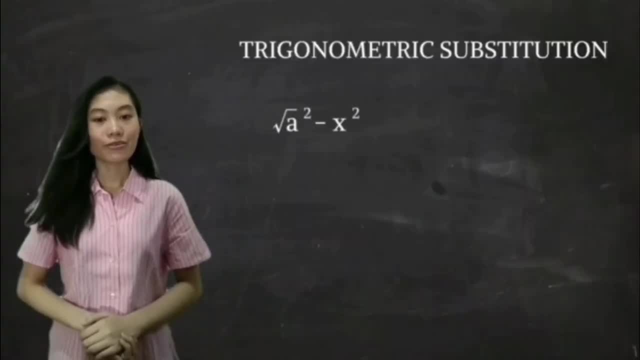 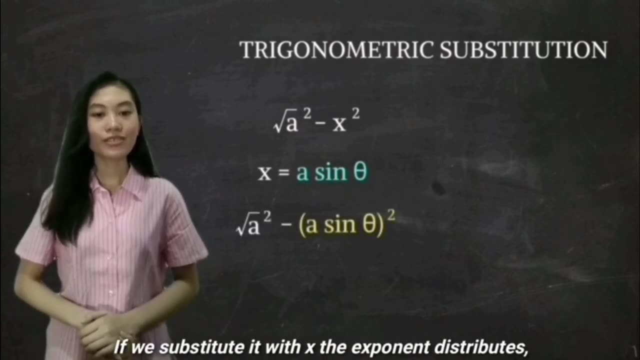 We can change X into something else. that results in getting rid of the radical With square root of A squared minus X squared. let X be sine theta. If we substitute it with X, the exponent distributes. We get A squared minus A squared, sine squared theta. 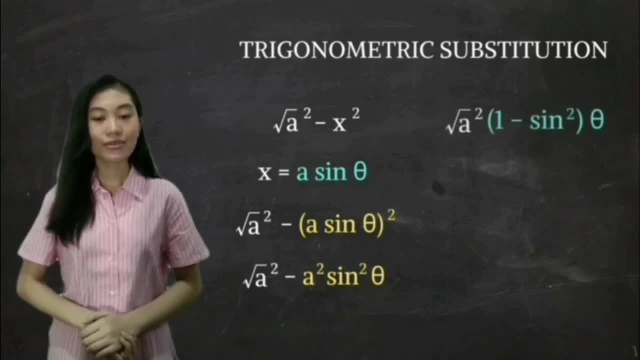 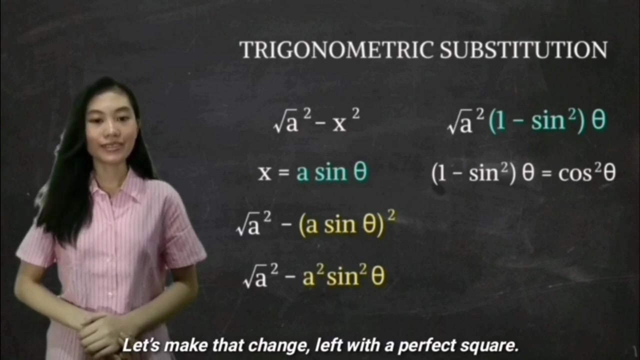 Then factor out A squared to get into A squared quantity: 1 minus sine squared theta. And with agorean identities, 1 minus sine squared theta is equal to cosine squared theta. Let's make the change when we are left with a perfect square. 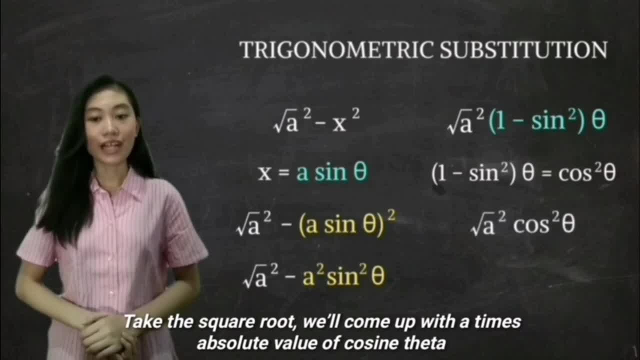 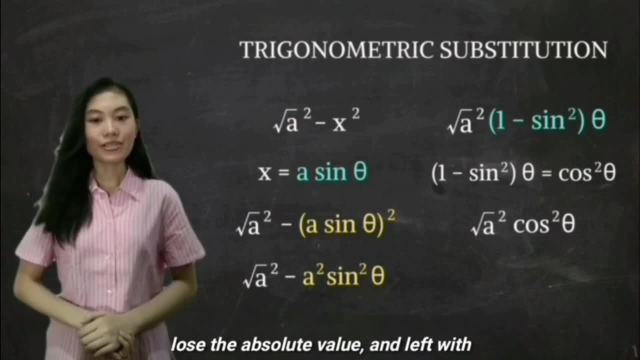 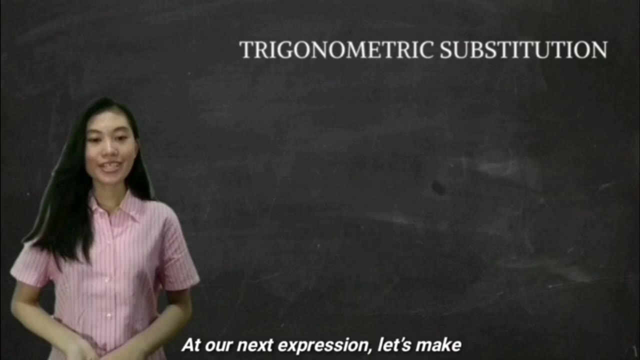 Take the square root, We'll come up with A times absolute value of cosine theta. If we take the interval with theta, cosine theta will be positive, Lose the absolute value and left with A cosine theta. At our second expression, let's make X equal to A tangent theta. 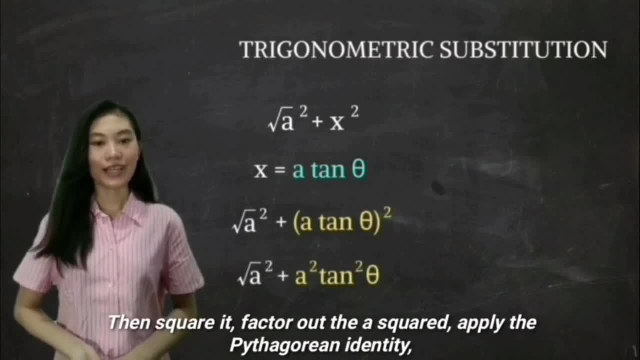 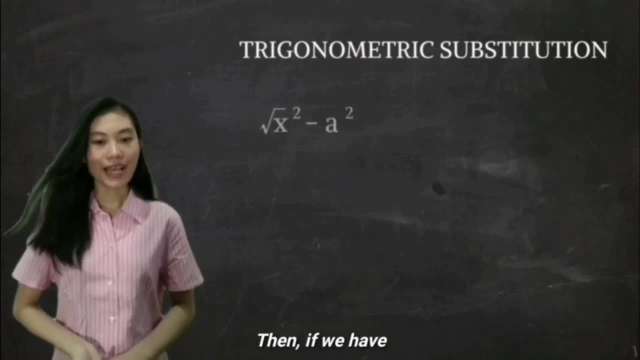 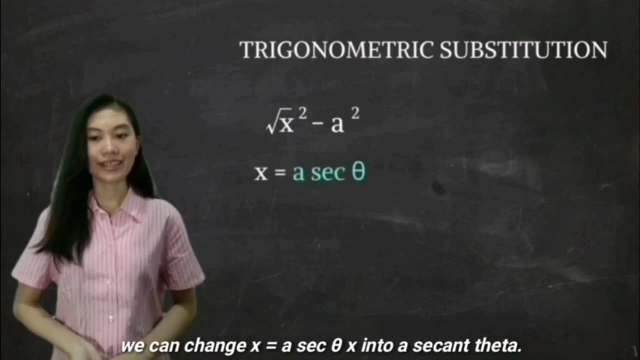 Then square it. Factor out the A squared, Apply the Pythagorean identity, Get rid of the radical to get A second theta. Then we have square root of X squared minus A squared. We can change X into second theta, Then perform the process we have used earlier. 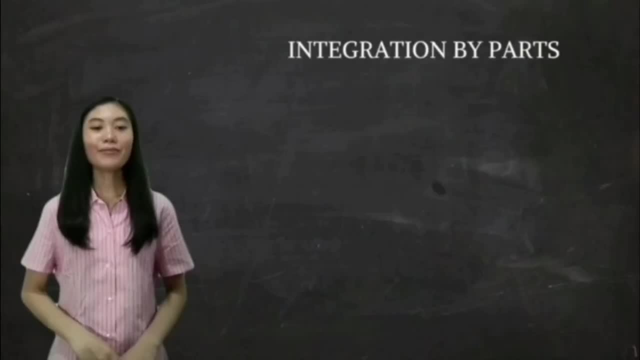 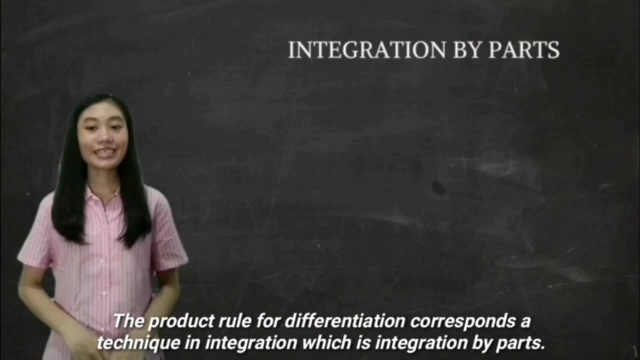 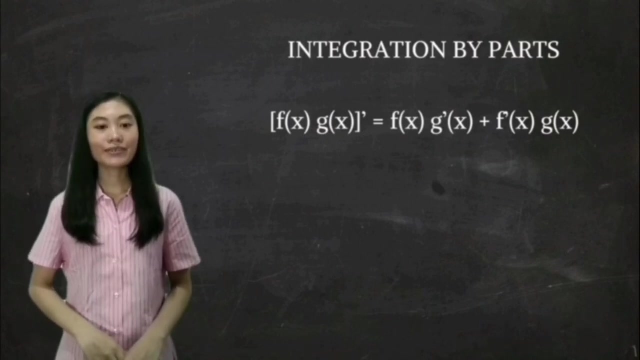 We'll have A tangent theta. Number four: Integration by parts. The product rule for differentiation corresponds to technique in integration, which is integration by parts. The product rule says that the derivative of two functions is equal to the first times the derivative of the second. 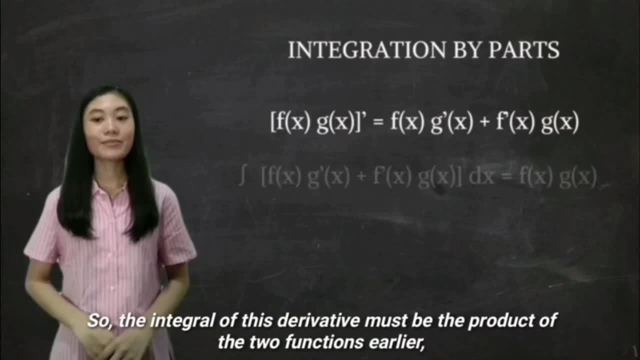 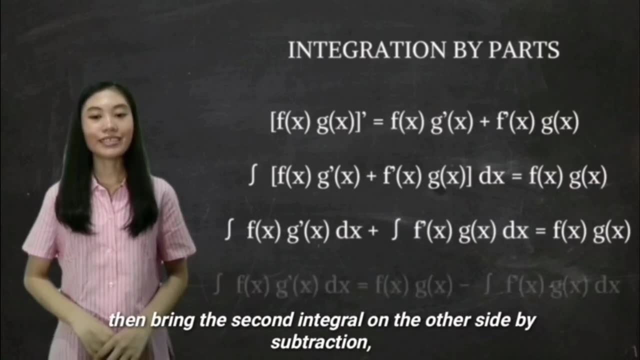 times the derivative of the first times second. So the integral of this derivative must be the product of the two functions. earlier Integral of the sum is equal to the sum of integrals. Then bring the second integral on the other side. by subtraction We'll come up with a formula of integration by parts. 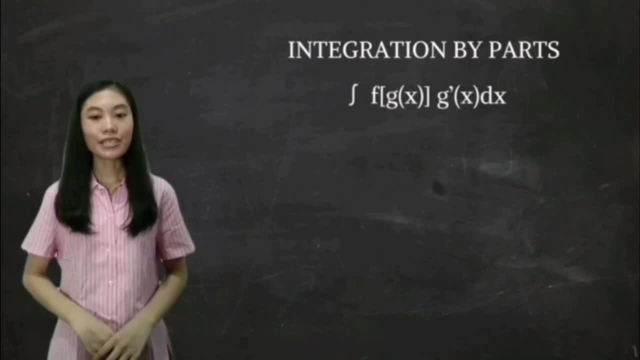 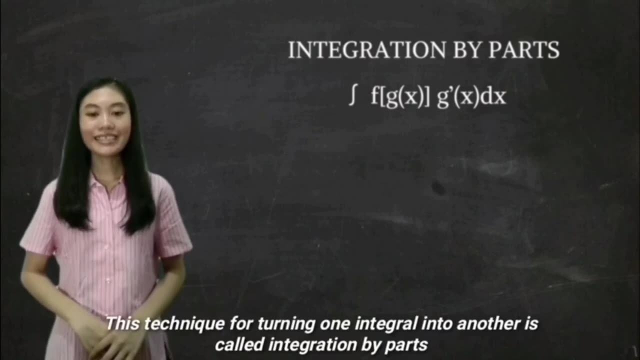 In many cases we have an integral form of f, of g, of x times g, prime, of x, dx, But this form is easier. This technique for turning one integral into another is called integration by parts, and it is usually written in more compact form. 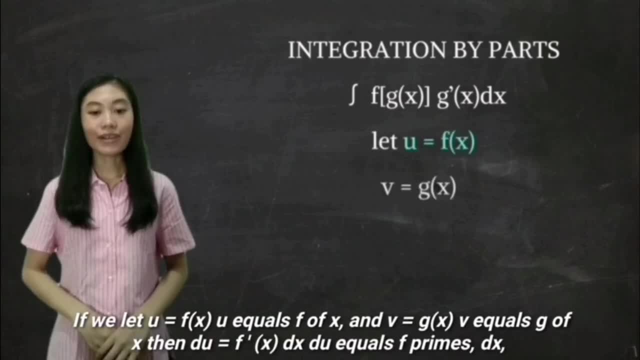 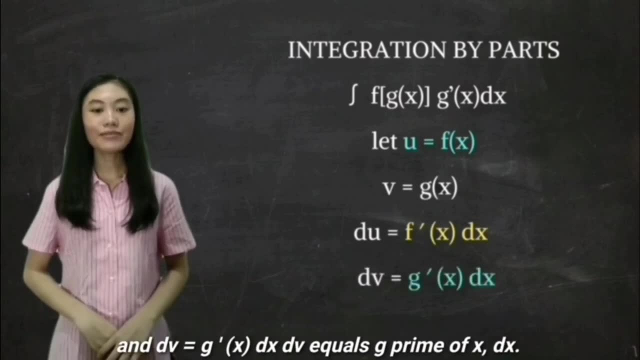 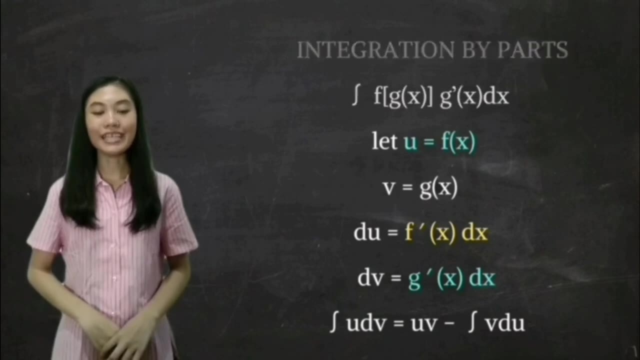 If we let u equals f of x and v equals g of x, then du equals f prime of x dx and v equals g prime of x dx. We'll come up with the integral of u. dv equals uv minus the integral of v, du Number five. 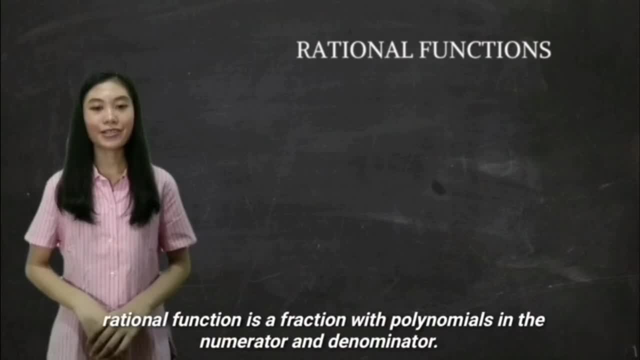 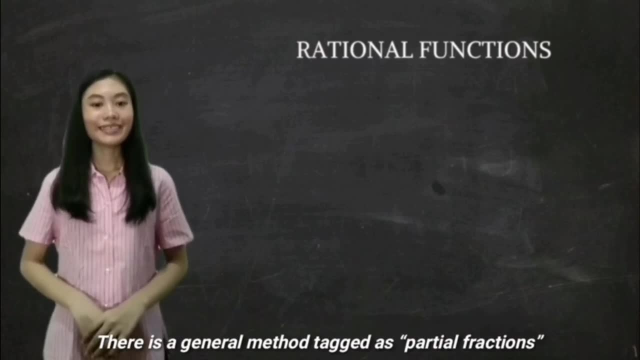 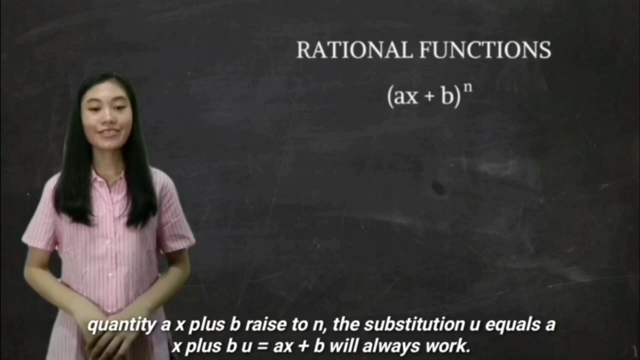 Rational functions. A rational function is a fraction with polynomials in the numerator and denominator. There is a general method, tagged as partial fractions, that allows us to integrate any rational function. If the denominator has the form quantity ax plus v. raised to n, the substitution u equals ax plus v. 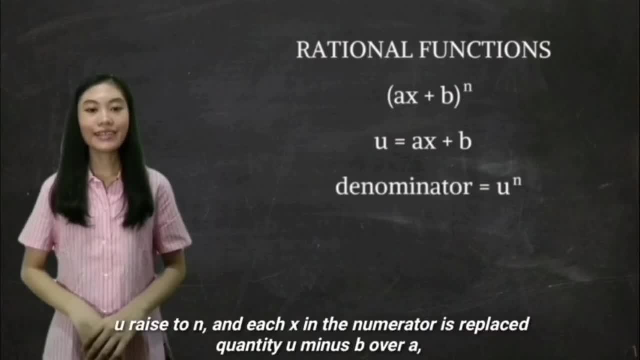 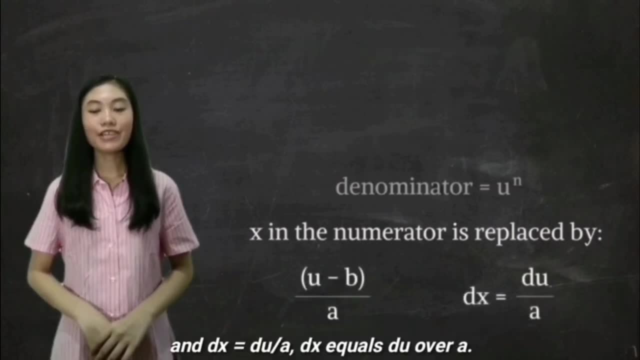 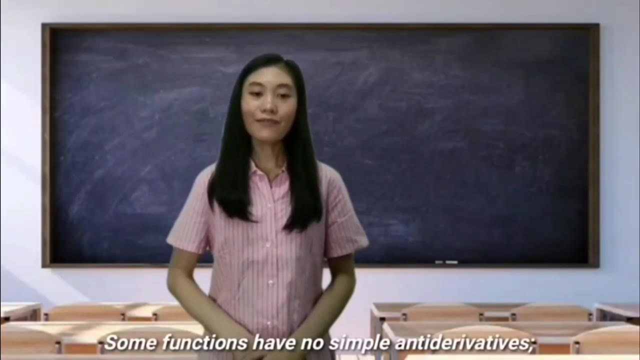 will always work. The denominator becomes u raised to n and each x in the numerator is replaced by quantity u minus v over 8 and dx equals du over 8.. Number six: Numerical integration, Trapezoidal rule. Some functions have no simple integralities. 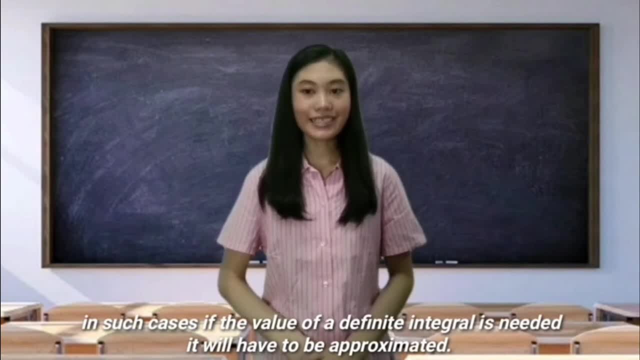 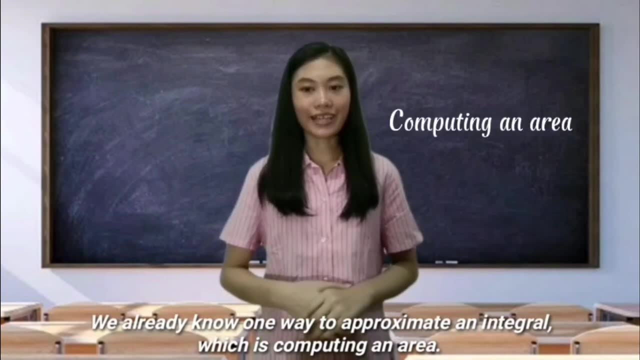 In such cases, if the value of a definite integral is needed, it will have to be approximated. We already know one way to approximate an integral, which is computing an area, An area under a curve approximated by rectangles or by trapezoids. 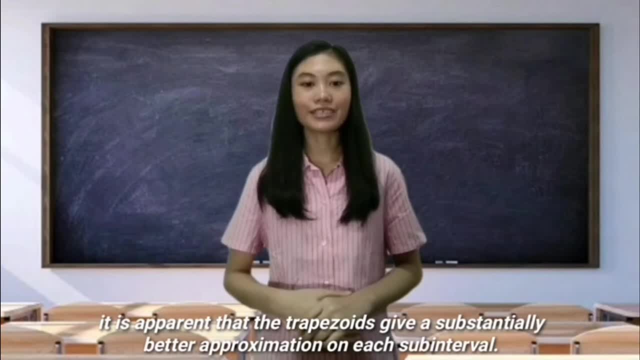 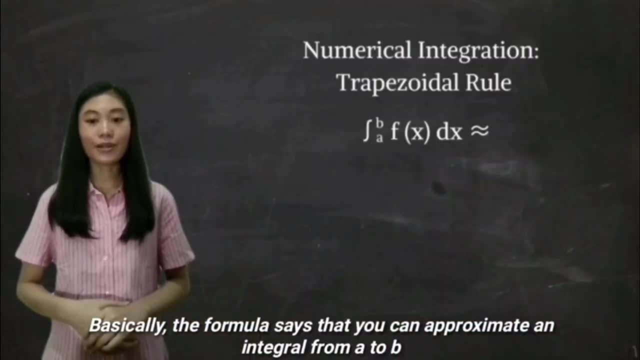 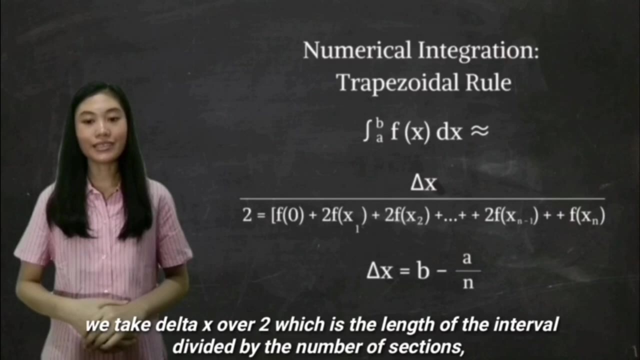 It is apparent that trapezoids give a substantially better approximation on each subinterval. Basically, the form says that you may approximate an integral from a to b, Assume we chop it up into sections. We take delta x over 2, which is the length of the interval. 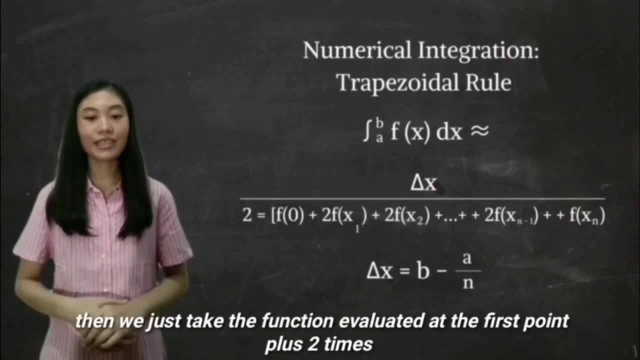 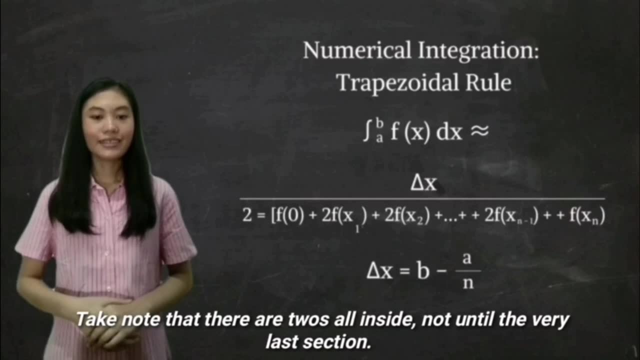 divided by the number of sections. Then we just take the function evaluated at the first point plus 2 times the function evaluated at the next one. Take note that there are 2s all inside, not until the very last section. Then we have x sub i, given the formula. 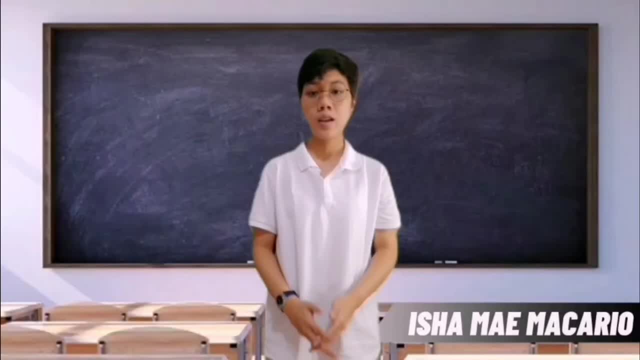 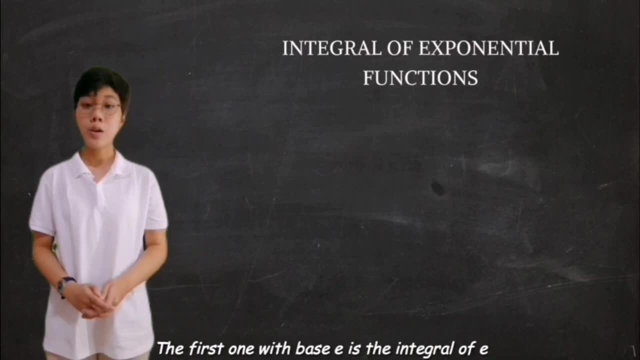 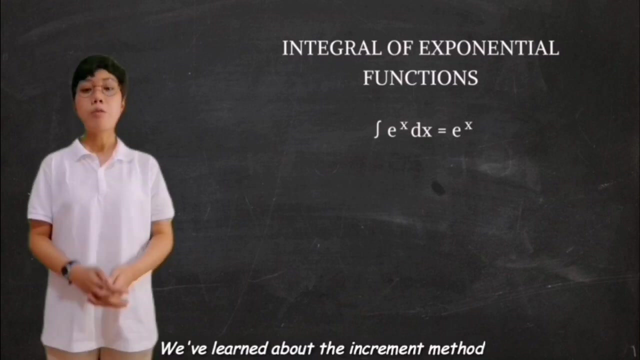 a plus i, delta x. Let's discuss the integration involving exponential functions. There are 2 basic formulas. The first one, base e, is the integral of e to the x dx equal to e raised to x plus c. We've learned about the increment method. 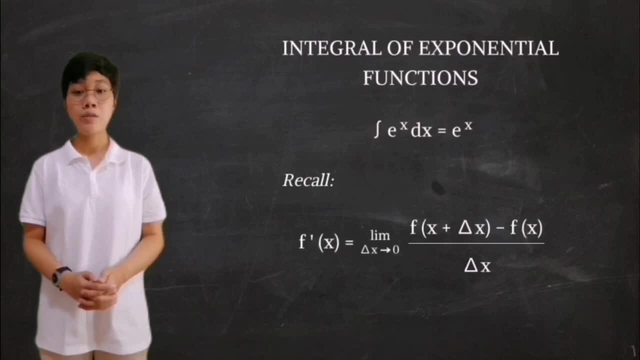 in our lessons in derivatives, And we recall by the formula f prime of x equal to the limit of x plus delta x minus f of x. all over delta x is the change in x equal to 0, we will find the derivative of e raised to x. 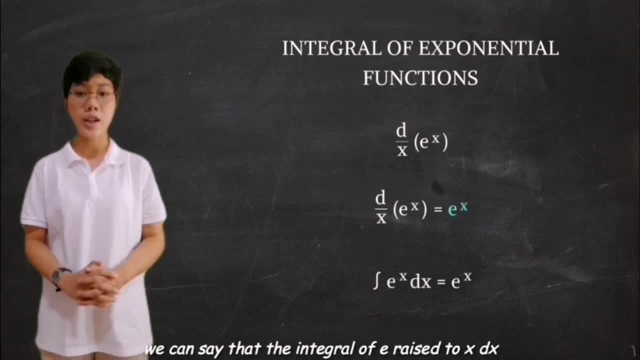 which is also e raised to x, And because of this we can say that the integral of e raised to x, dx is equal to e raised to x. This is the formula for the base e or Euler's number, The second example of integration. 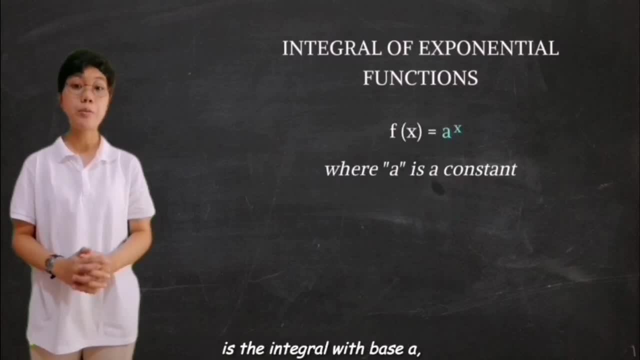 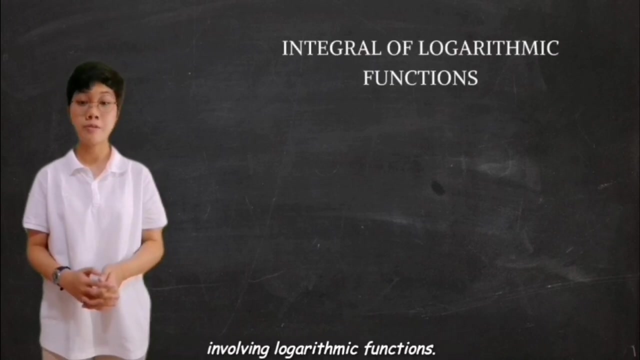 involving exponential functions is the integral of base a, where a is a constant. The integral of a raised to x, dx is equal to a raised to x, all over ln of e plus c. Now let's move on to the integration involving logarithmic functions. 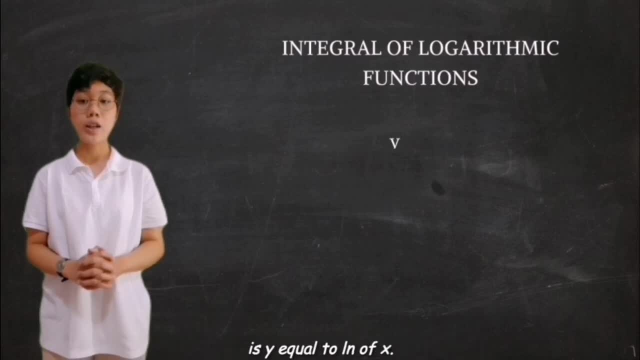 The function of the natural logarithm of x is y equal to ln of x. By exponentiating this function we will get b raised to ln of x is equal to x and is one of the properties of the natural logarithm and Euler's number. 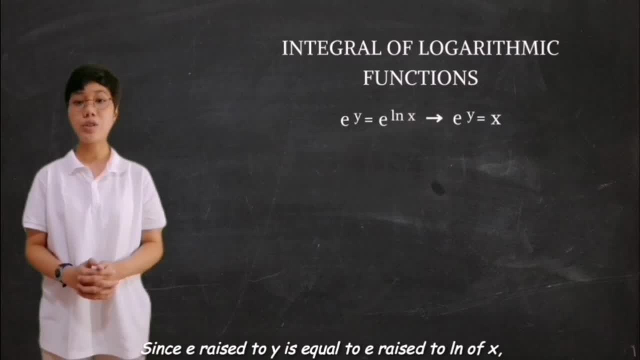 of exponential functions. Since e raised to y is equal to e raised to y to x, then e raised to y is equal to x. If we get the derivative of both sides of this function, we will obtain 1 over ln raised to y. 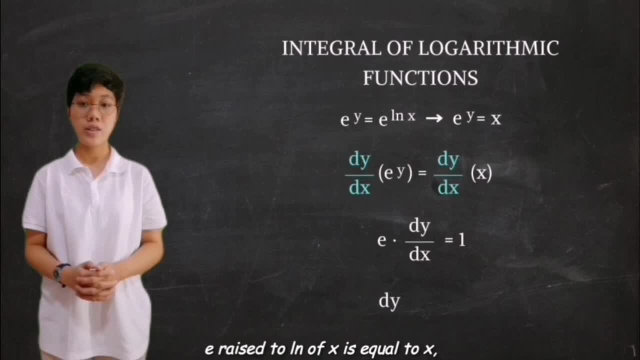 But since y is equal to ln of x and e, raised to ln of x, is equal to x, then we will be left with 1 over x. We will have the derivative of the natural logarithm of x by getting the antiderivative of 1 over x. 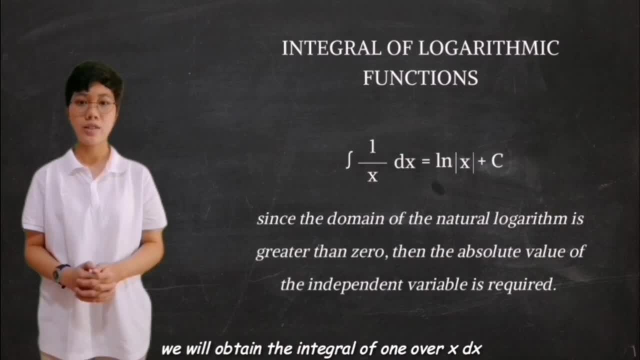 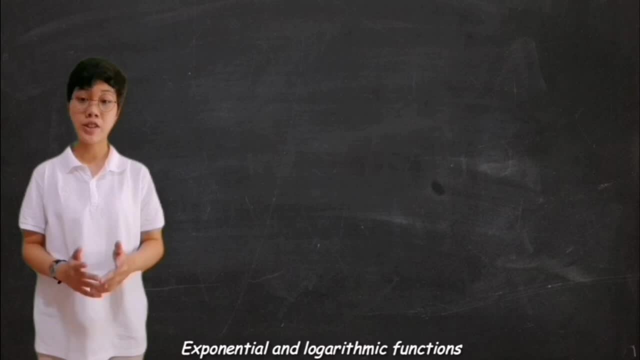 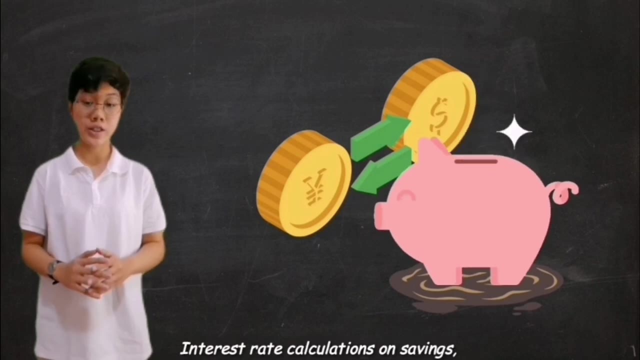 Therefore we will obtain the integral of 1 over x. dx equal to ln, the absolute value of x plus c. Exponential and logarithmic functions have various applications, especially in economics, where these equations are applied in interest rate calculations and biology. 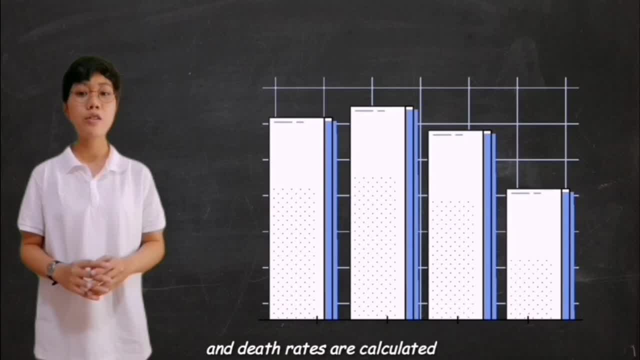 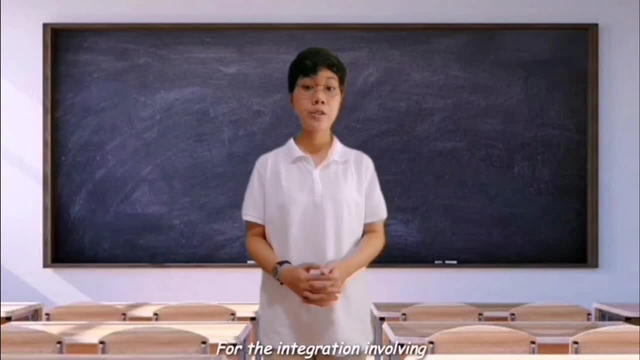 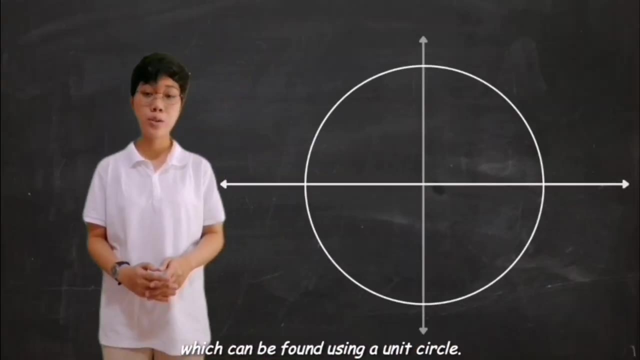 where animal and plant population growth are calculated and predicted using exponential functions. For the integration involving trigonometric functions and integrals, we need to know about the eight trigonometric elements which can be found. using a unit circle, We can form a right triangle. 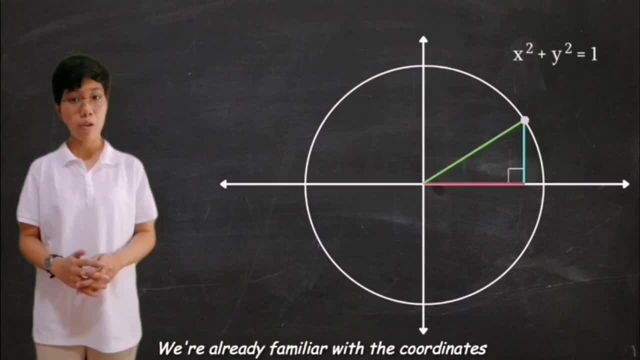 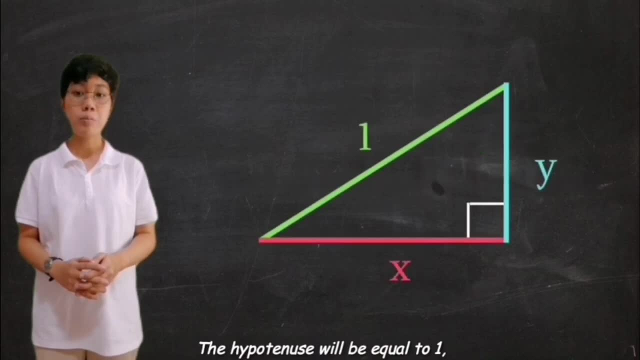 by placing a point on the unit circle. We are already familiar with the coordinates of different signs. If we recall, we know the theorem: The hypotenuse will be equals 1, the adjacent will be equals x and the opposite will be equals y. 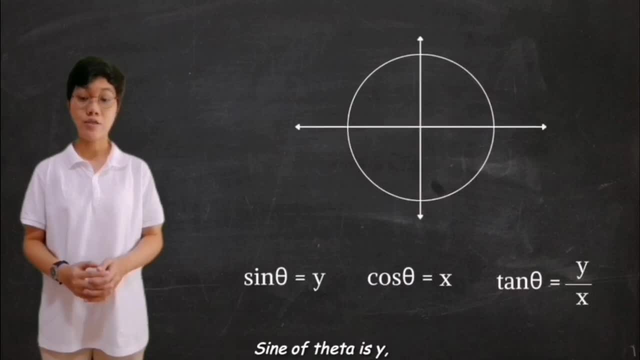 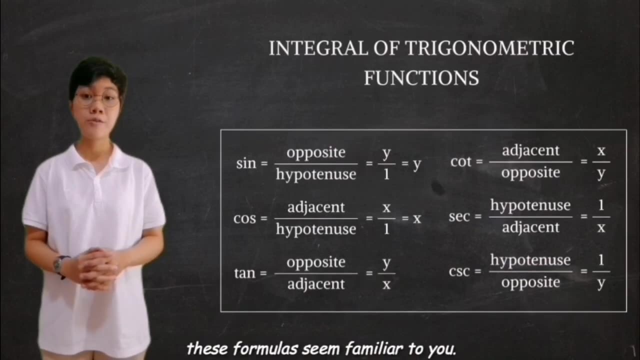 Because of the unit circle. we get formulas like sine of theta is y, cosine of theta is x and tangent of theta is y over x. You might be wondering why these formulas seem familiar to you. As you can see, this reminds us. 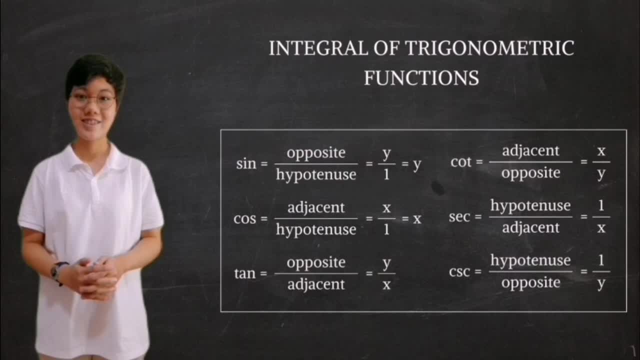 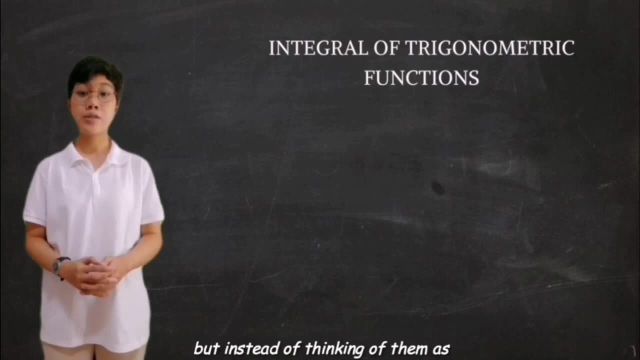 of the six trigonometric functions. Now let's create new definitions for all of these functions, But instead of thinking of them as coordinates of the unit circle, we are going to consider them only as terms of the trigonometric functions. For example, 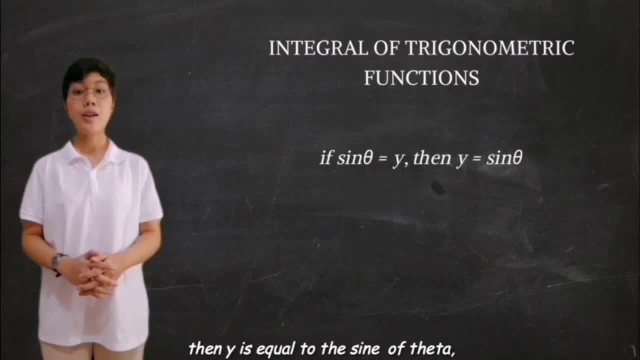 if the sine of theta is equal to y, then y is equal to the sine of theta, And if the cosine of theta is equal to x, then x is equal to the cosine of theta. Or if tangent is equal to y over x. 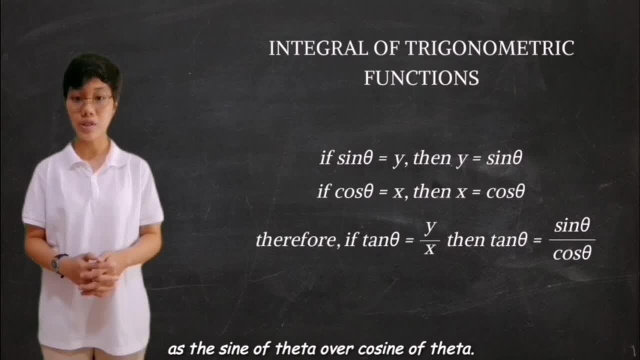 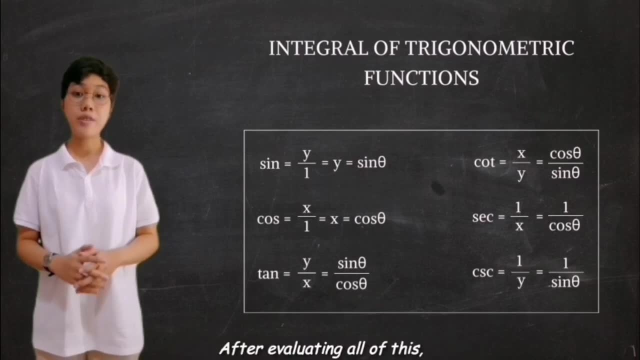 then we can rewrite tangent as the sine of theta over the cosine of theta. We will use the same process to identify the other trigonometric functions. After evaluating all of this, we'll think about what else we can create from our equation. This is where the formula 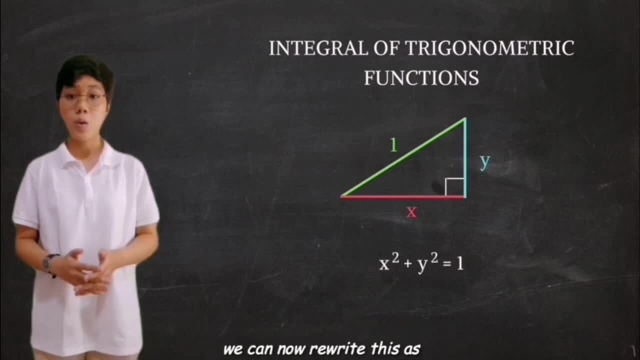 for the Boolean theorem comes in From what we've discussed. we can now rewrite this as: cosine squared of theta plus sine squared of theta equals 1.. This now becomes the first of the trigonometric identities, And if we have two equations, 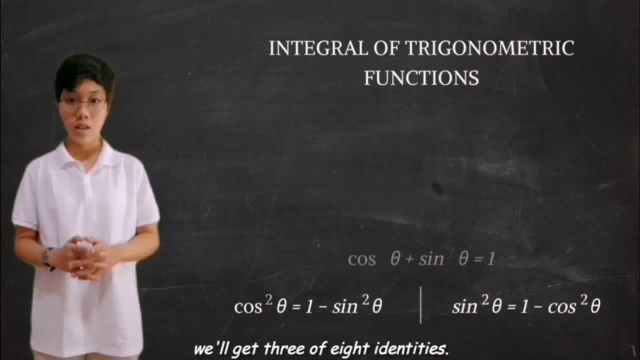 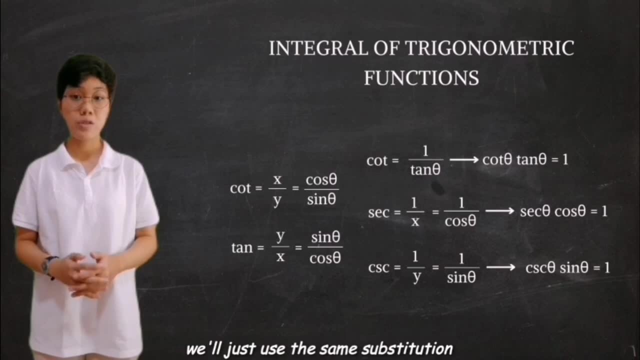 where we transpose sine in the first and cosine in the second, we'll get three of the identities. To get the five other trigonometric identities, we'll just use the same substitution process through when we created a new definition of trigonometric functions. 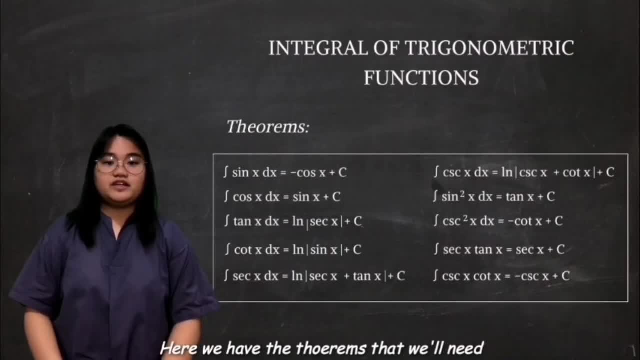 Here we have the theorems that will be used for integrating trigonometric functions. Let's solve a problem by using one of these formulas. For our example, we have to get the integral of g sine x plus sigma squared of x over x. 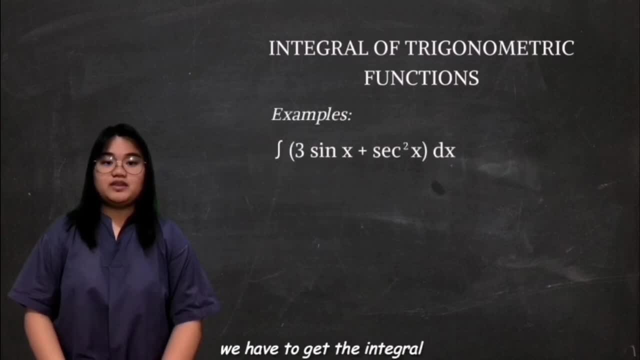 First let's separate g sine x and sigma squared of x by applying the sum of g sine x plus sigma squared of x over x. First let's separate g sine x and sigma squared of x by applying the differential of integration. We already have an answer. 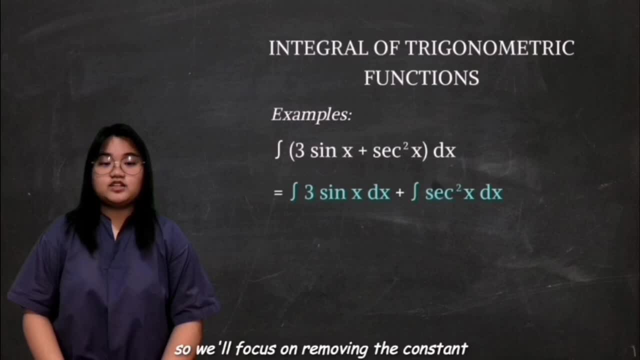 for the integral of sigma squared x over x. so we'll focus on removing the constant, which is three, from the integral of three sine x over x. by applying the constant multiple for integration, The equation will now become three integral of sine of x over x. 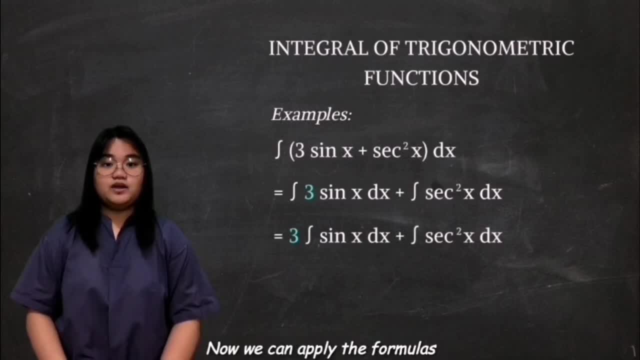 plus integral of sigma squared x over x. Now we can apply the formulas of trigonometric functions. and let's not forget the artificial constant. For the last step, since we still have three, we can simplify this by multiplying it to the negative. 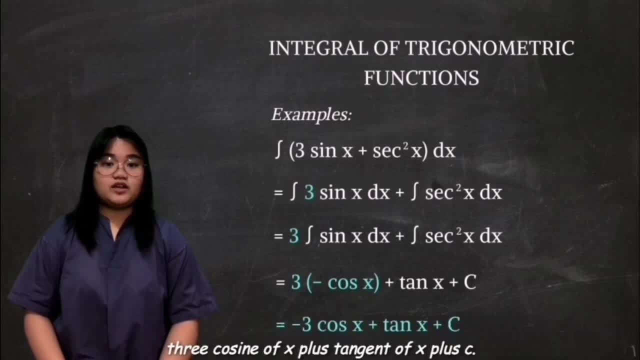 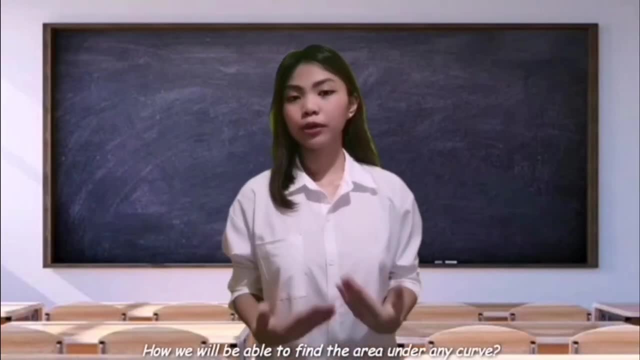 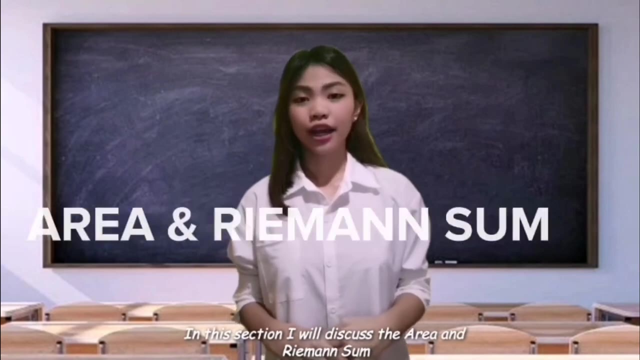 cosine of x. Our final answer is negative. three cosine of x plus tangent of x plus c. Have you ever wondered how we will be able to measure the area under any curve? In this section, I will discuss the area under the Riemann sum. 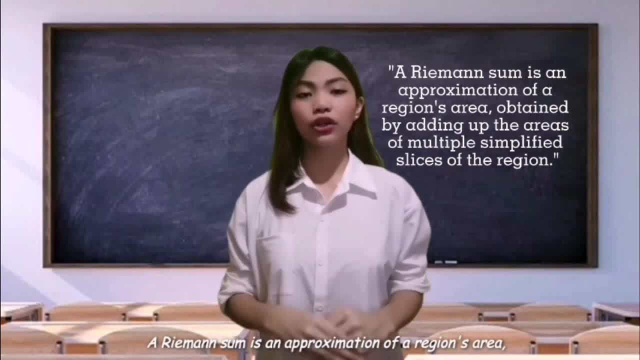 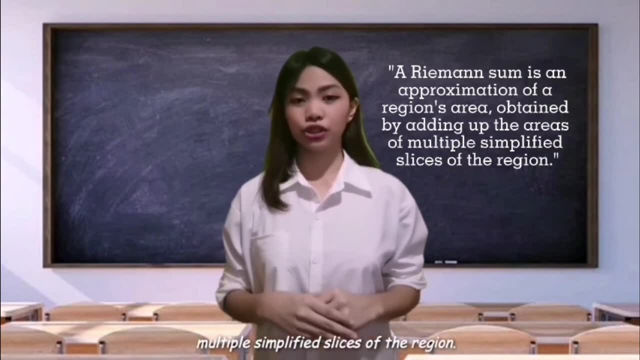 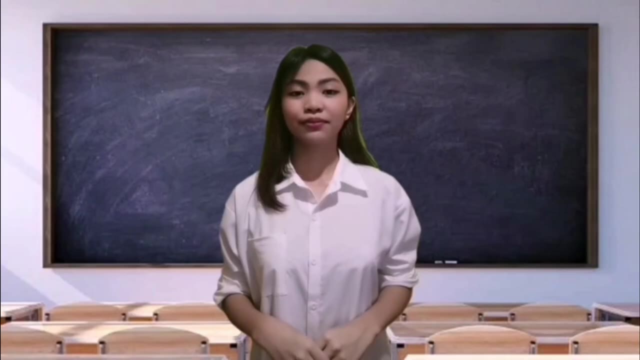 In mathematics, a Riemann sum is an approximation of region's area obtained by adding up the areas of multiple simplified slices of the region. It is named after 19th century German mathematician, Bernhard Riemann. How is Riemann sum? 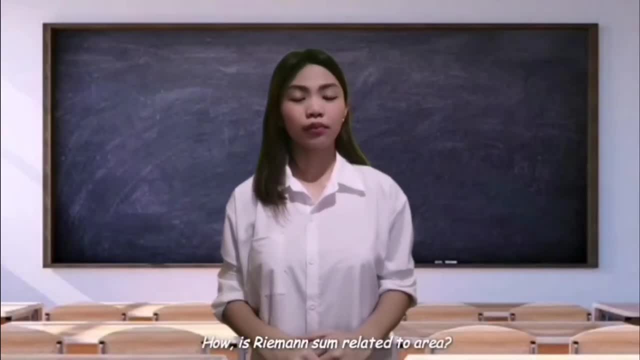 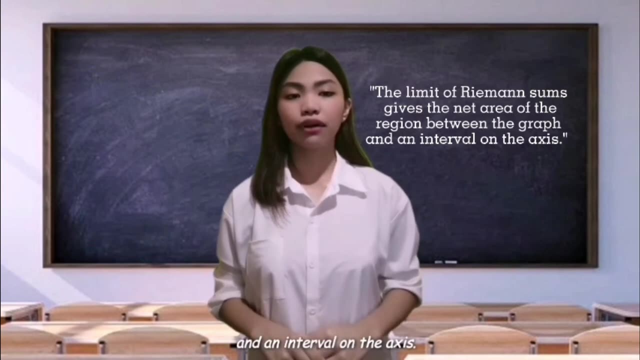 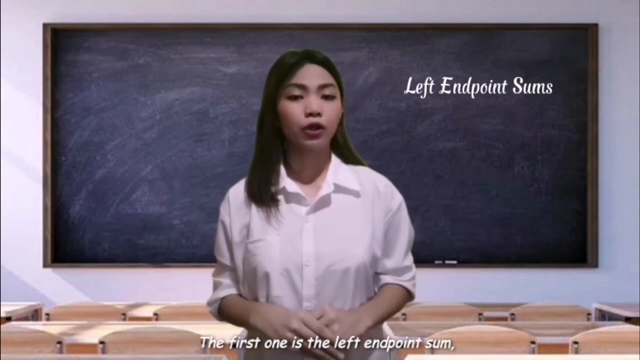 related to area. The limit of Riemann sum gives the net area of the region between the graph and the axis. There are three basic types of Riemann sum. The first one is the left end point sum. The second one is the. 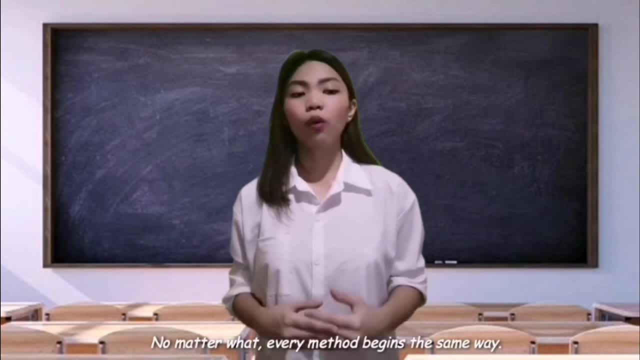 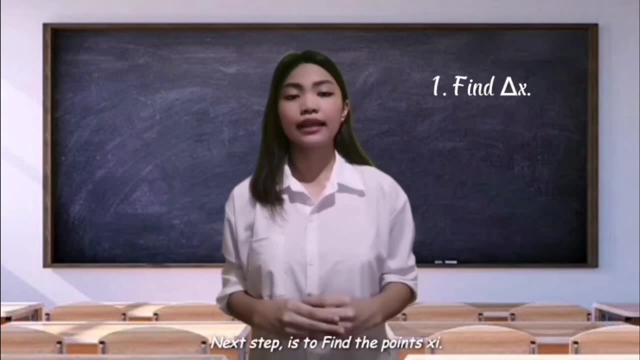 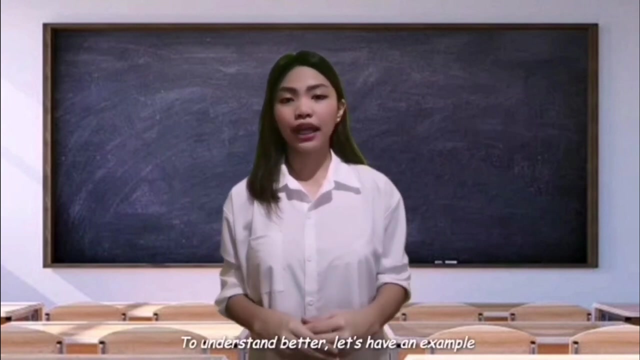 right end point sum. And the third is the midpoint rule. No matter what, every method begins the same way. The first step is to find the delta x. Let's have an example. Suppose that we have a graph, So how can we? 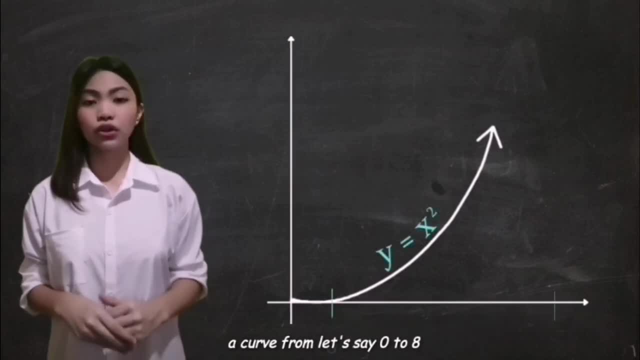 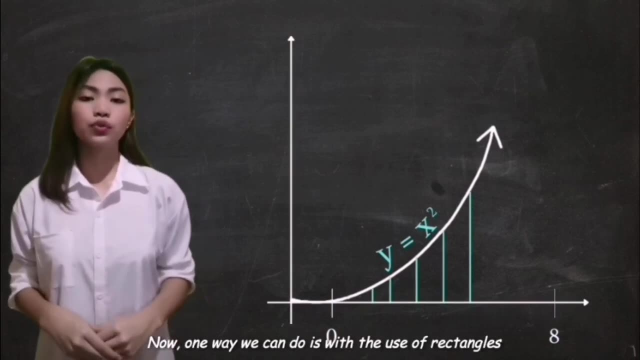 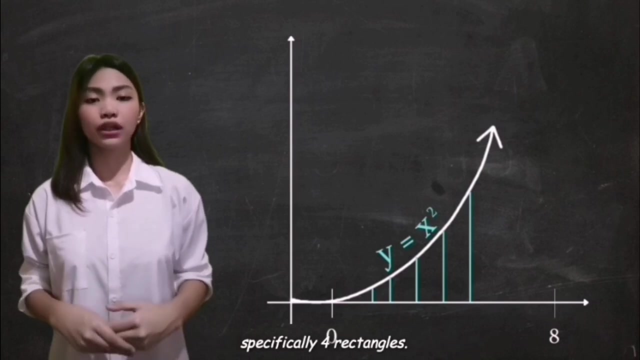 calculate the area under a curve from, let's say, 0 to 8? How can we determine the shaded area? Now, one way we can do is with the use of rectangles. So let's use rectangles to measure the approximate area, and specifically, 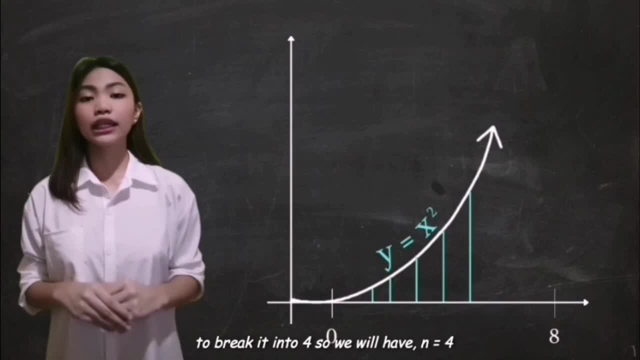 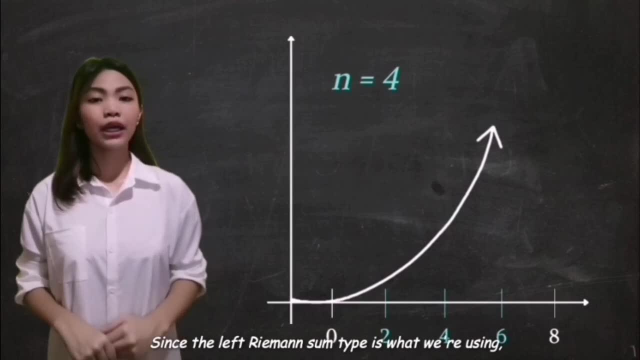 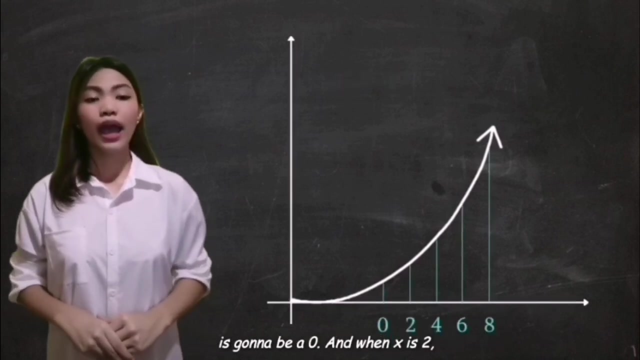 for rectangles And we're going to break it into 4.. So we will have: n is equal to 4.. Since the left Riemann sum type is what we're using, the first rectangle from left end point is gonna be a 0.. 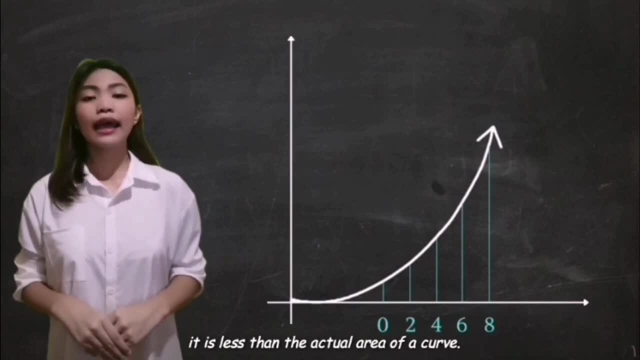 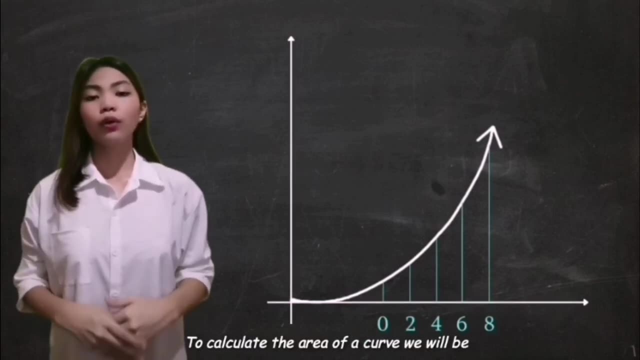 And when x is 2, it is gonna touch the curve, and so we're gonna calculate the area of a curve. To calculate the area of a curve, we will be multiplying the width times the height, And we need to do that in every rectangle. 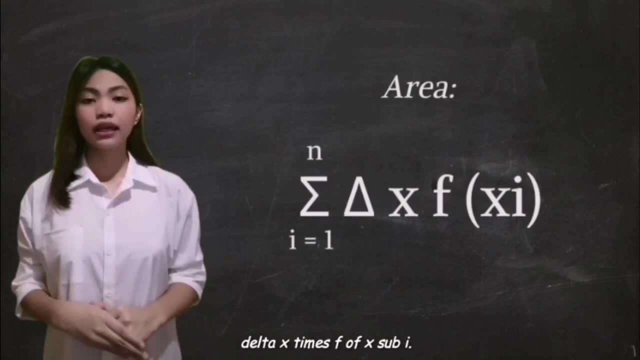 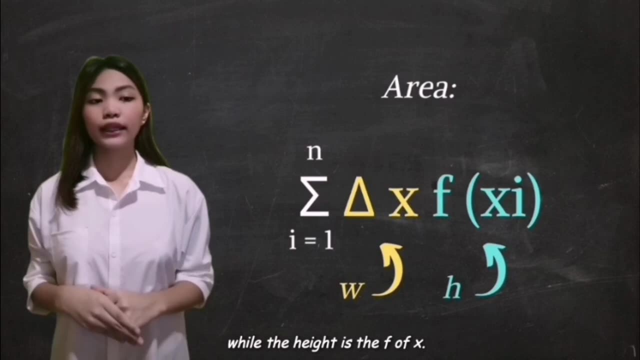 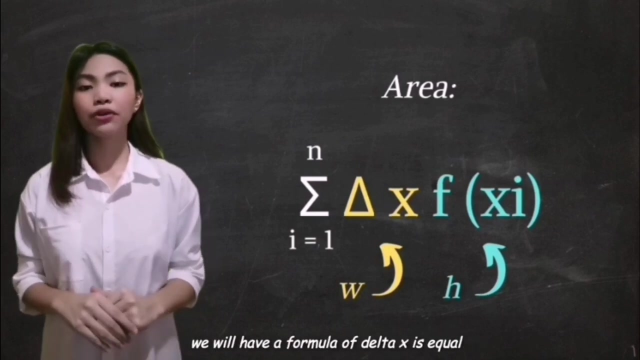 So we will come to the process and formula of the area is equal to the sigma times delta x times f of x of. i Remember that delta x is the value of delta x. We will have a formula of delta x is equal to b. 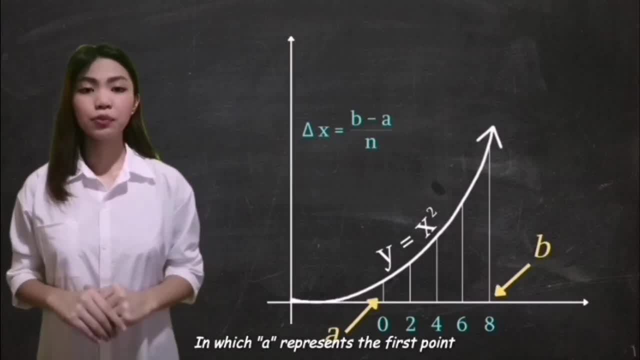 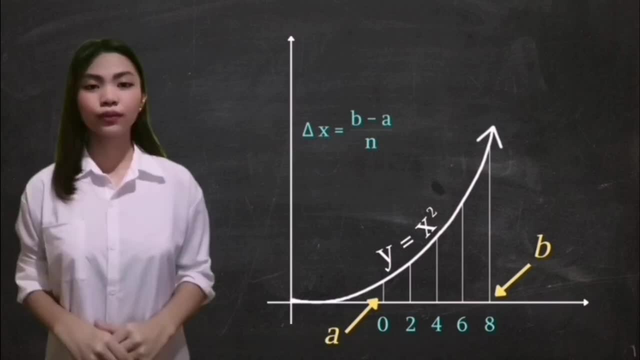 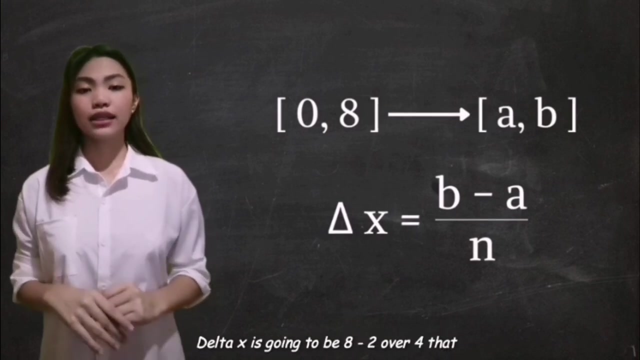 minus 8 over n, in which a represents the first point and b represents the end point, while n represents the rectangles. So we want to calculate the area from 0 to 8, and that is from 8 to the answer of 2.. 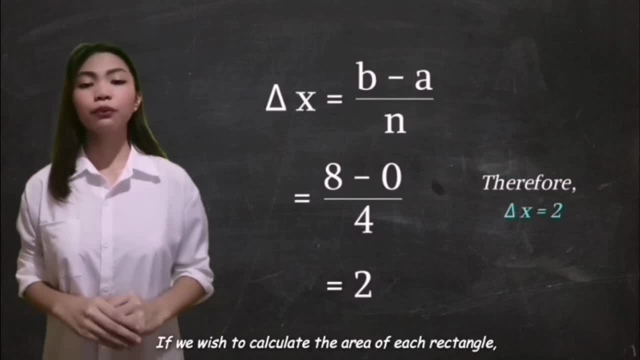 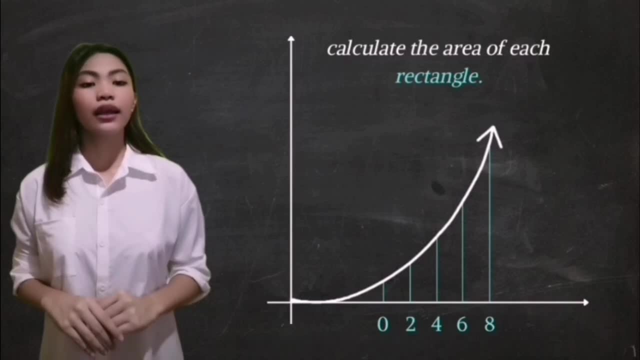 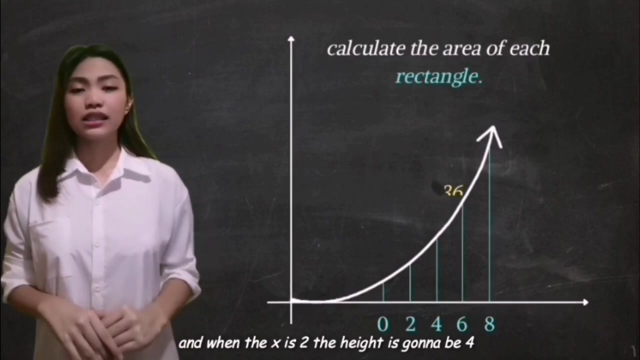 Therefore the delta x is 2.. If we wish to calculate the area of a rectangle using the formula of i, y is equal to x squared. Therefore, when x is 0, so the height is 0.. And when the x. 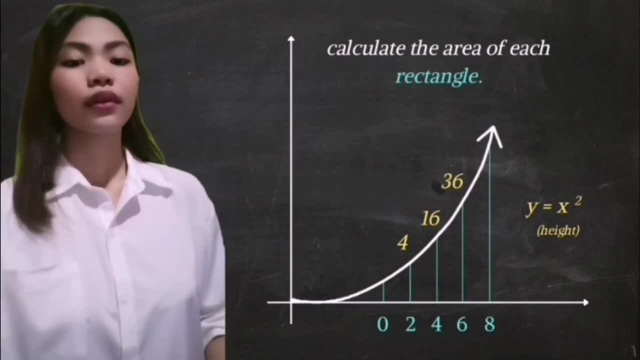 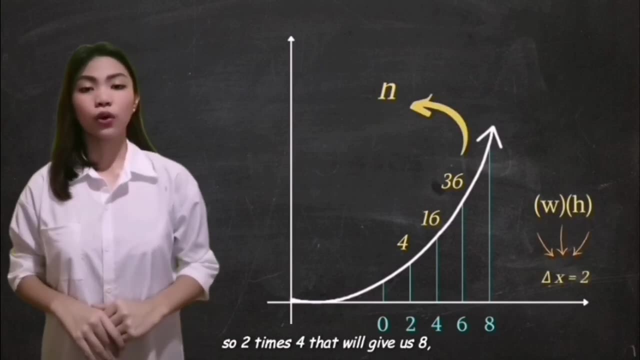 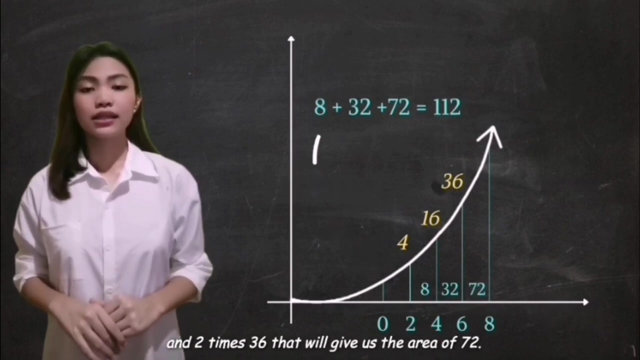 is 2, the height is gonna be 4.. Now we will calculate the area of each rectangle. that is width times the height. So 2 times 4, that will give us 8.. Next, 2 times 16, that will. 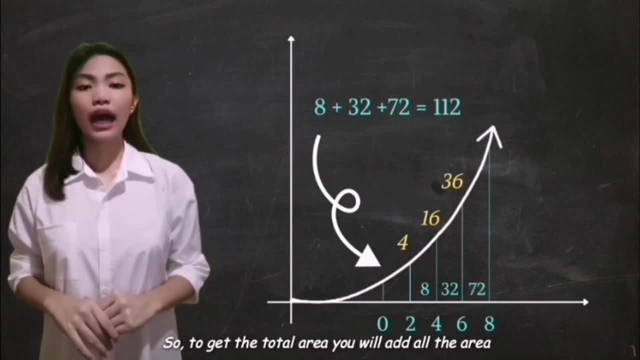 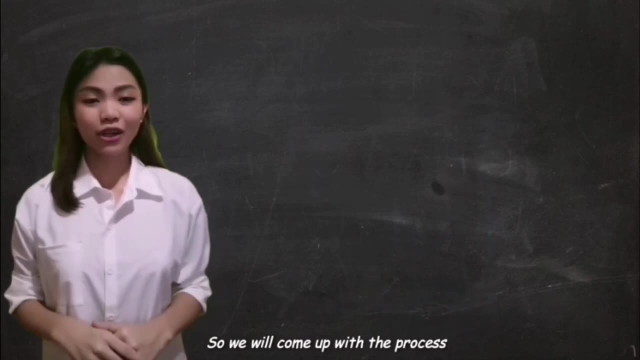 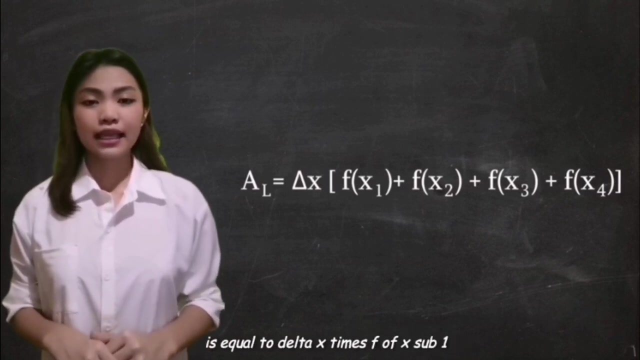 give us 36.. Next, 2 times 36, that will give us the area of 72. So we will come up with a process that will help us better. So we will have the area using the left end point, that is. 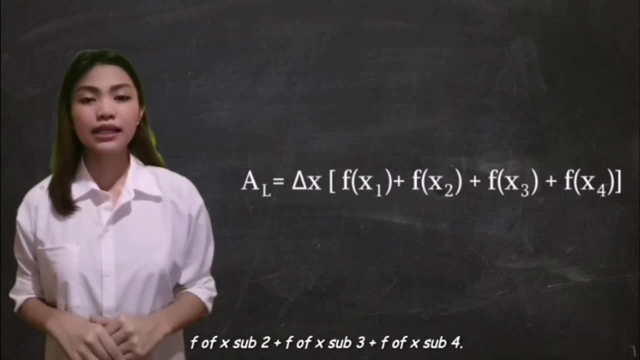 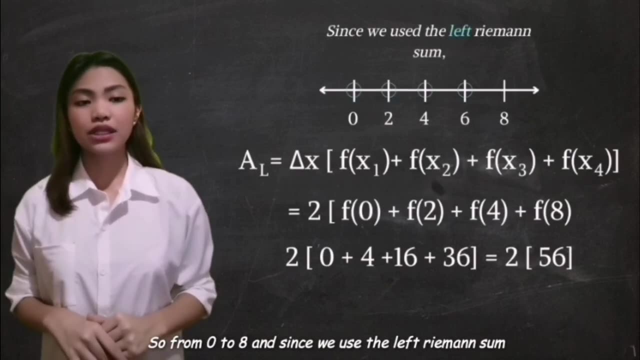 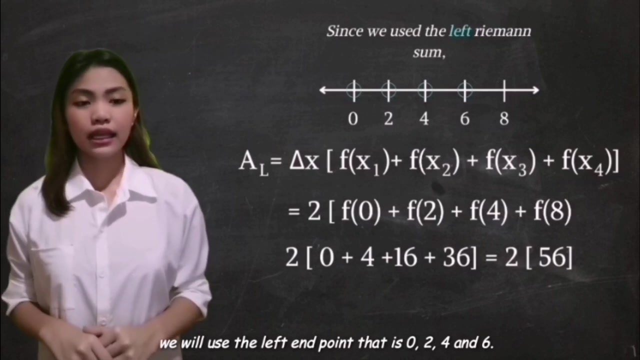 equal to delta x times f of x sub 1 plus f of x sub 2 plus f of x sub 3 plus f of x sub 4.. From the formula we will substitute the given value. that will give us delta x times f. 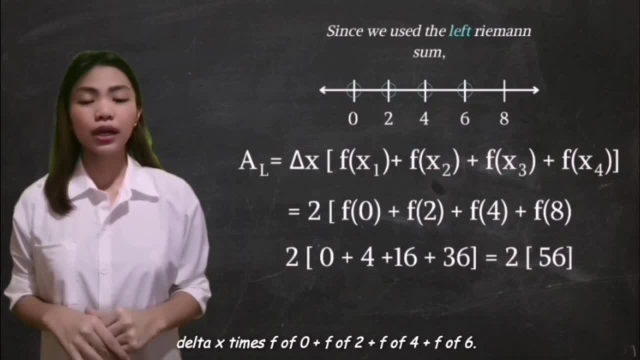 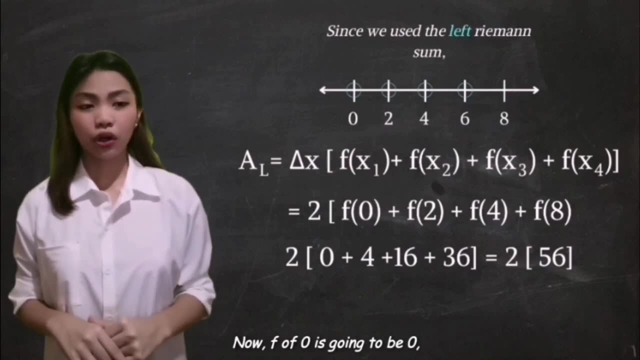 of 0 plus f of 2, plus f of 4 plus f of 6.. Now f of 0 is going to be 0,, f of 2 is going to be 4, f of 4 is going to be 16,. 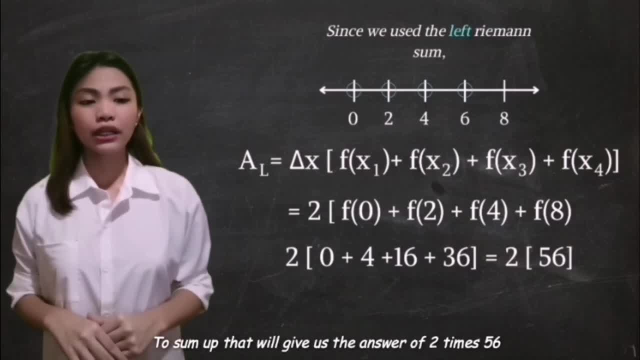 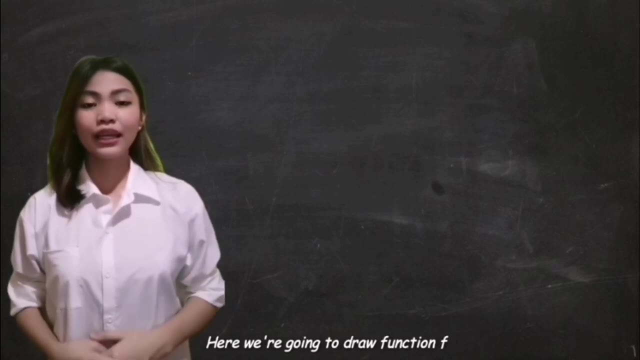 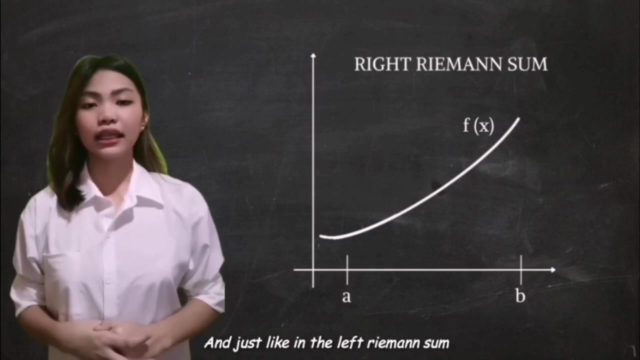 and f of 6 is going to be 36.. So the answer is 2 times 56, which is equal to 112, and that is the approximate area under the curve. The next type is the right Riemann sum Here: 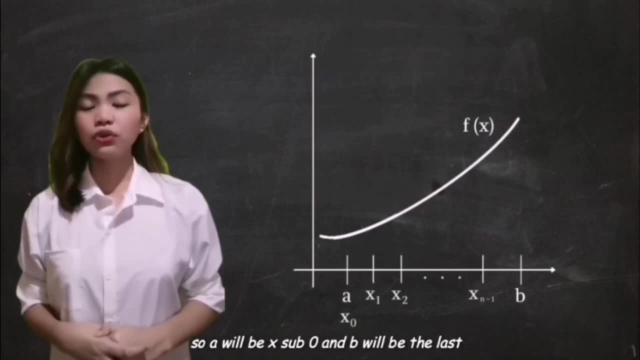 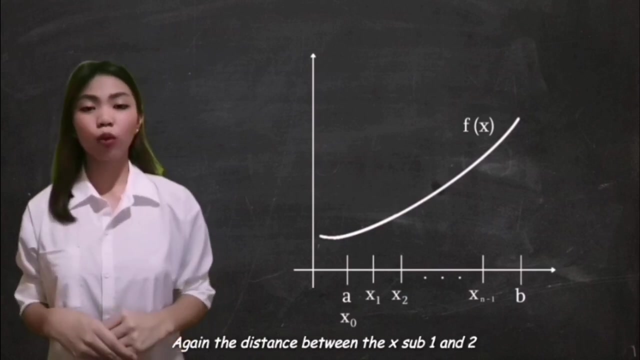 we are going to draw the x of 0 and b will be the last, which is x of f, And we are going to add up from 0 and whatever gonna be the value of x of i is Again the distance between the x of 1. 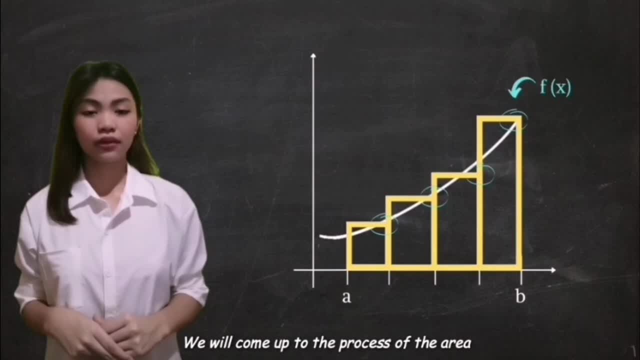 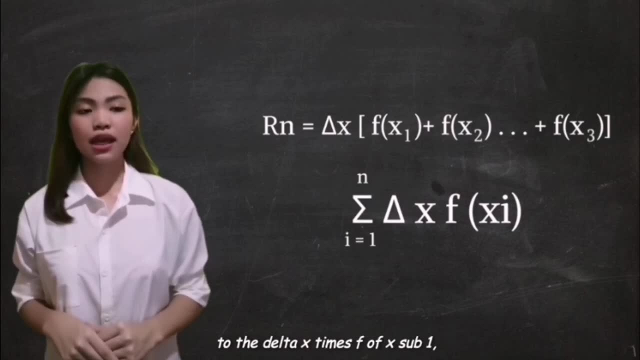 and 2 is the width, which is the delta x, And since we use the right Riemann sum, it's equal to the delta x times f of x of 1 plus f of x of 2, and so on from the last number. 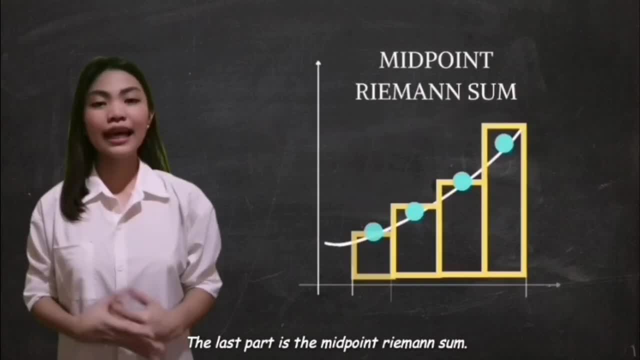 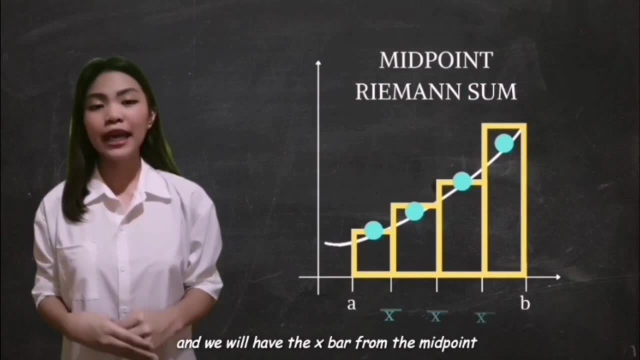 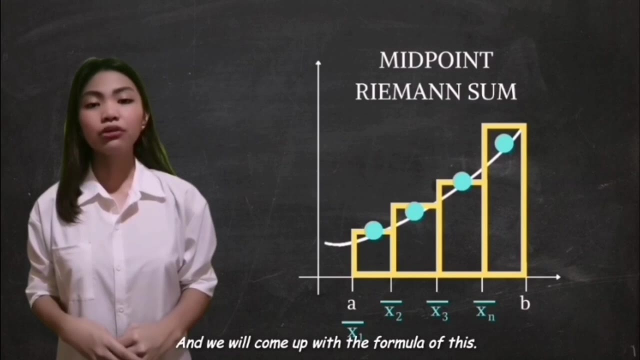 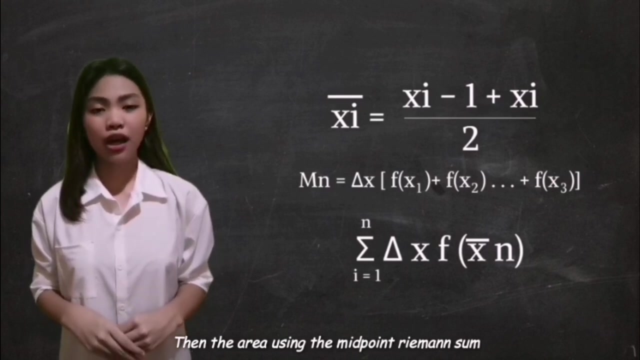 of f of x of n, So we will have the summation of delta x times f of x of i, So the x bar represents the average And we will come up with the formula of this. Then the area using the: 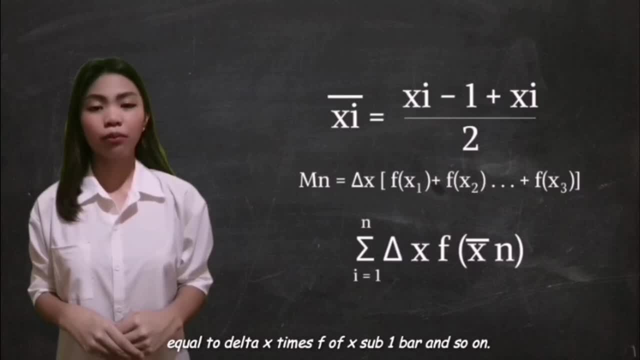 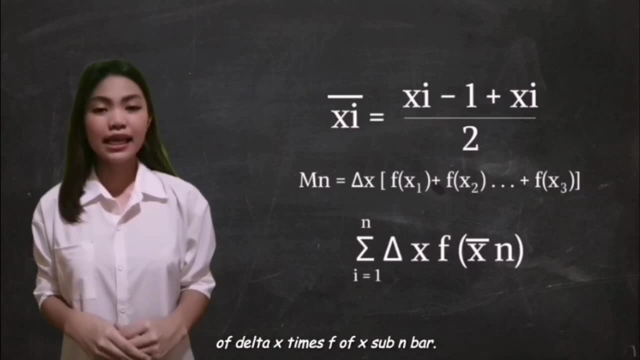 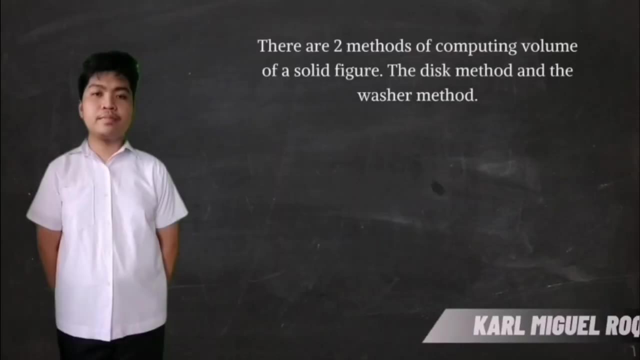 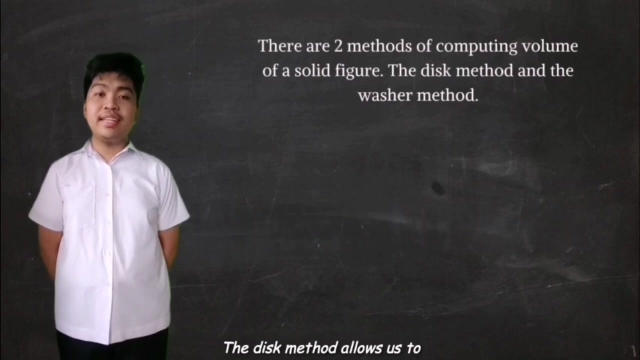 midpoint Riemann sum is equal to delta x times f of x of 1 bar, and so on. Now we will get the formula of the summation of delta x times f of x of n. We have two methods of computing. volume of a. 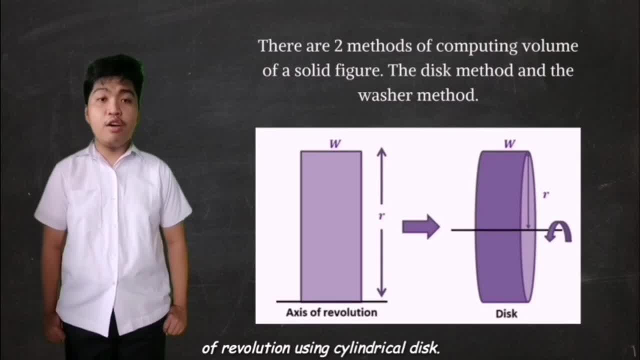 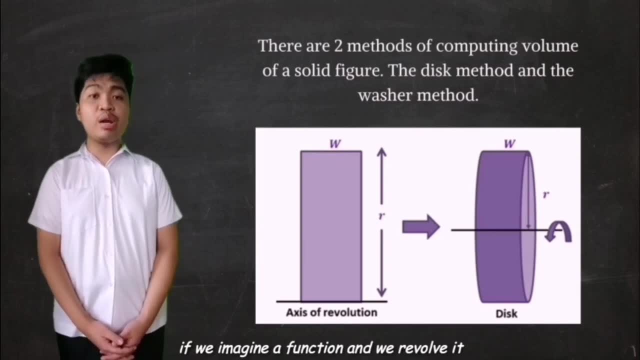 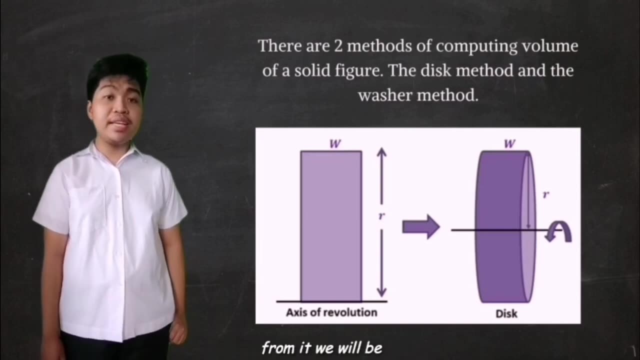 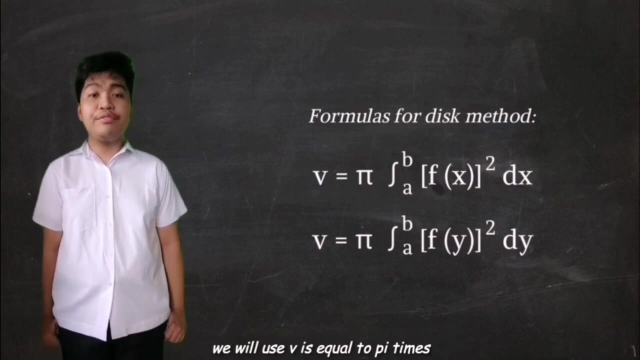 solid here, The disc method and the washer method. The disc method allows us to calculate the volume of solids of revolution using cylindrical disc. It is called method. are these two We will use? v is equal to pi times the integral of f of x squared. 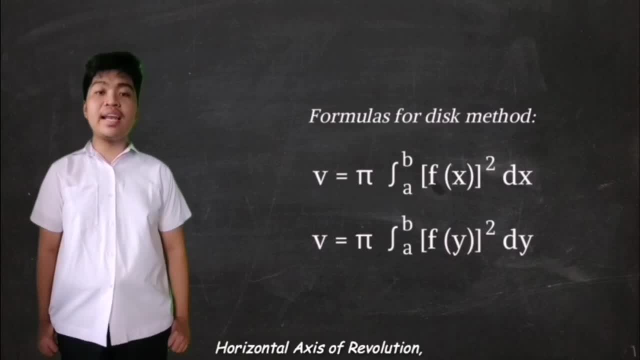 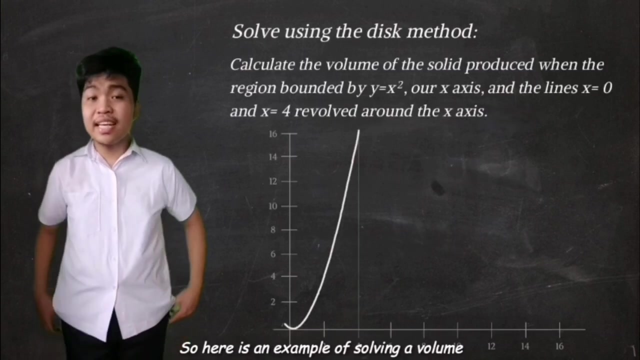 dx from a to b if it is horizontal axis of revolution. On the other hand, we will use: v is equal to pi times the integral of f of y squared dy from a to b if it is vertical axis of revolution. So here is an example of solving a volume of a solid figure using 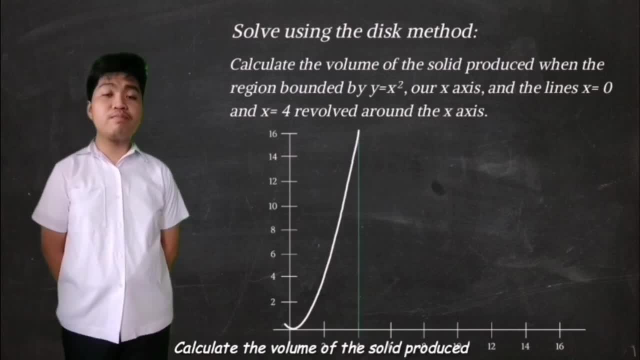 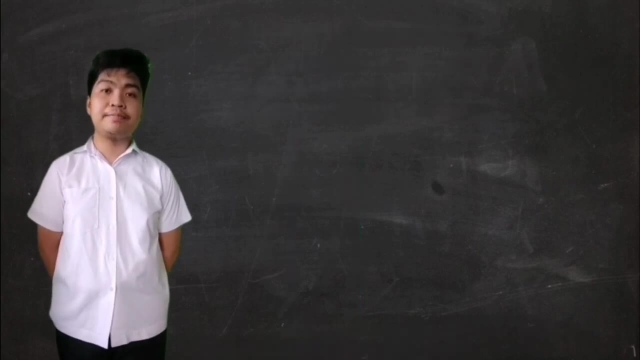 the this method Calculate the volume of the solid produced when the region bounded by y equals x squared. our x-axis and the lines x equals 0 and x equals 4 revolve around the x-axis. Our formula will be: v is equal to pi times the integral of f of x squared dx. 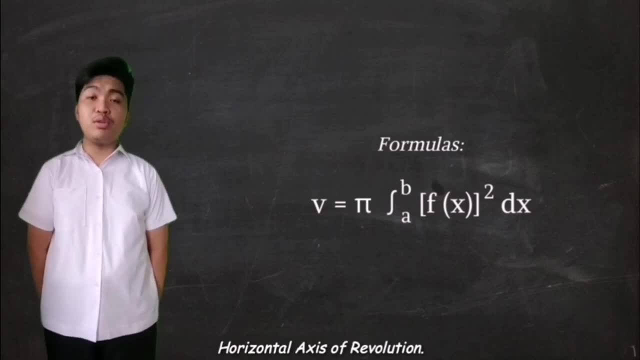 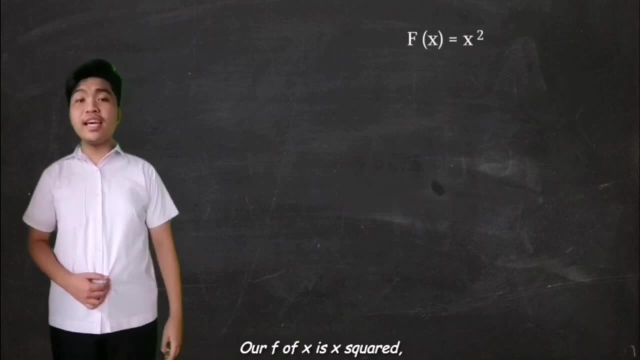 from a to b, since it is horizontal axis of revolution. Now let's identify and calculate the volume of the solid produced when the region bounded by y equals x squared dx from a to b. Then substitute the elements given in the problem. Our f of x is x squared a will be: 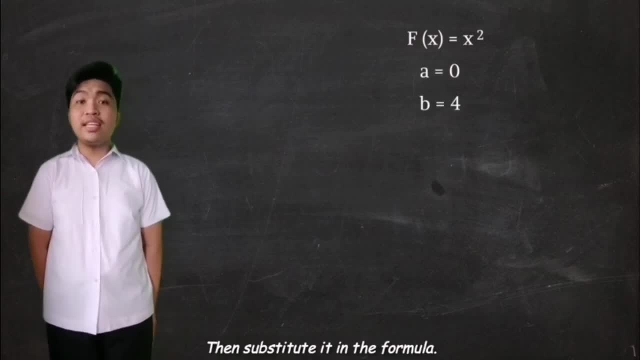 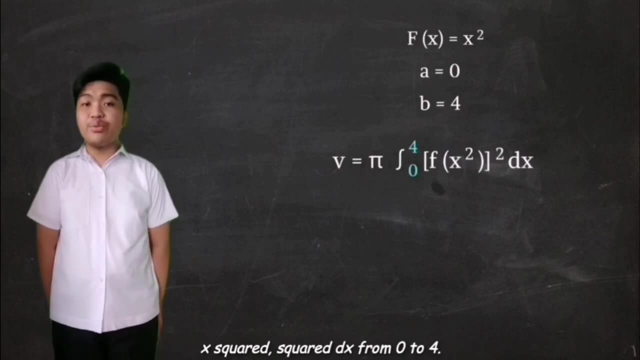 0 and v is 4.. Then substitute it in the formula: v is equal to the pi times the integral of quantity x squared squared dx from 0 to 4.. Just simplify Now. we got: v is equal to pi times the integral of x to the fourth power, dx from 0 to 4.. 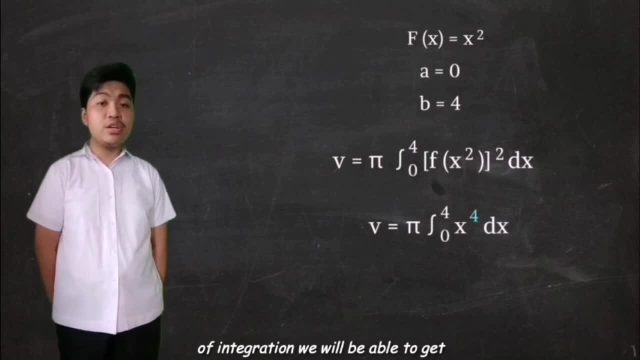 And then, by applying the power rule of integration, we will be able to get: v is equal to pi, x to the fifth, all over 5, from 0 to 4.. Now, by evaluating it from 0 to 4 and by further simplifying, 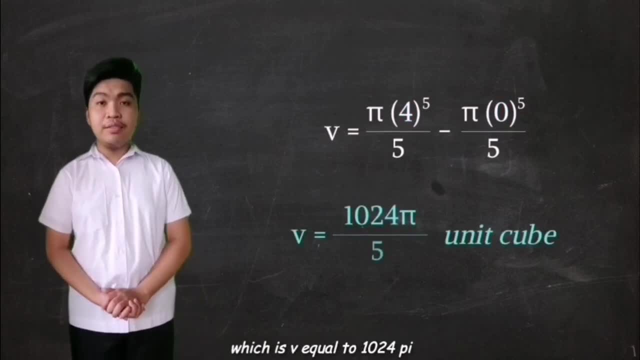 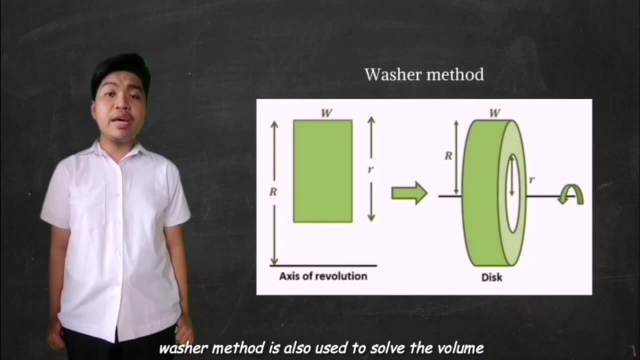 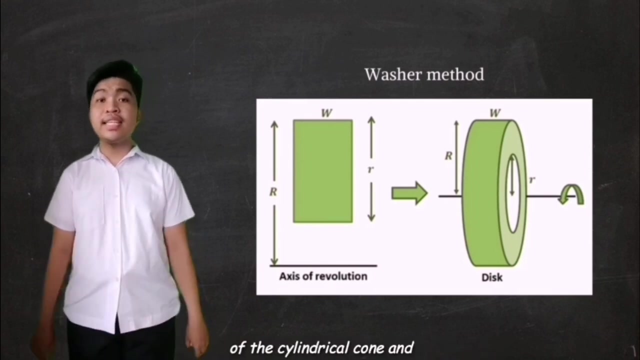 we will be able to get the final answer, which is: v is equal to 1024 pi, all over 5 unity. Similarly to that, this method- Washer method- is also used to solve the volume of a solid here, But the only difference is that it has a hole in the center of the cylindrical. 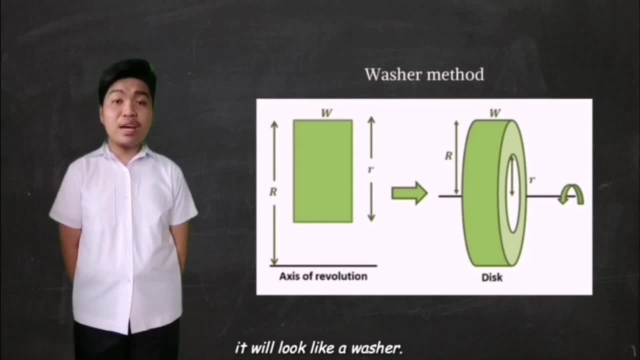 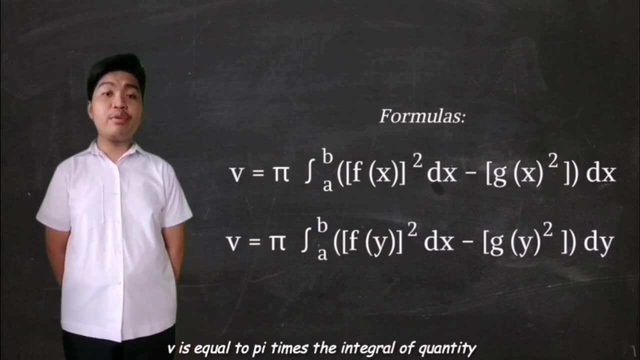 bone and when you slice a part of it it will look like a washer. These two are the formulas of Washer method. v is equal to pi times the integral of quantity f of x squared, minus quantity t of x squared. dx from a to b if it is horizontal axis of revolution On the. 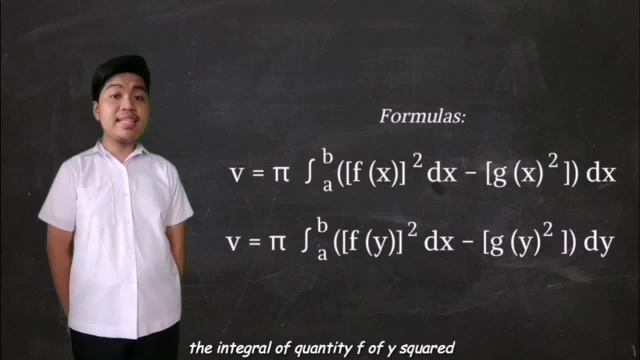 other hand we will use: v is equal to pi times the integral of quantity f of x squared dx from a to b, if it is vertical axis of revolution, Wherein our f of x and f of y is the outer radius and g of x and g of y is the inner radius. 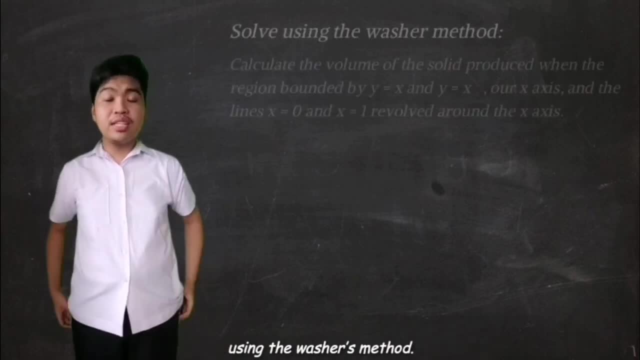 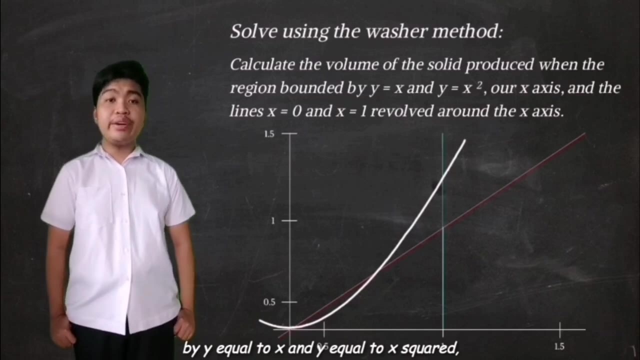 Now let's try to solve a volume of a solid figure using the Washer method. Calculate the volume of the solid produced by the region bounded by y equal to x and y equal to m. Now let's try to solve a volume of a solid figure using the Washer method: Calculate. 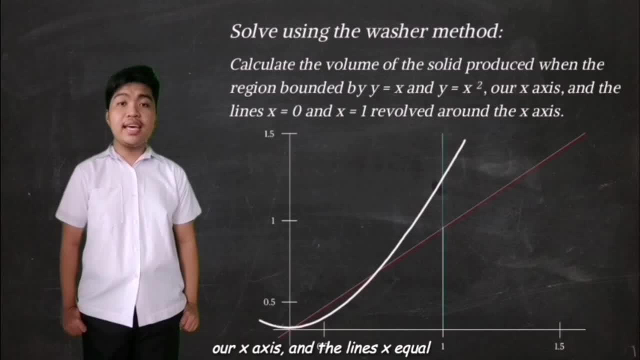 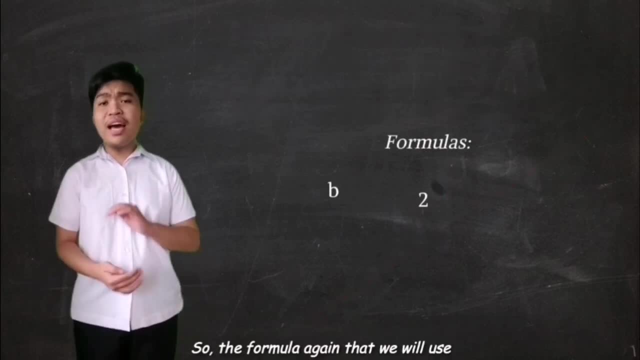 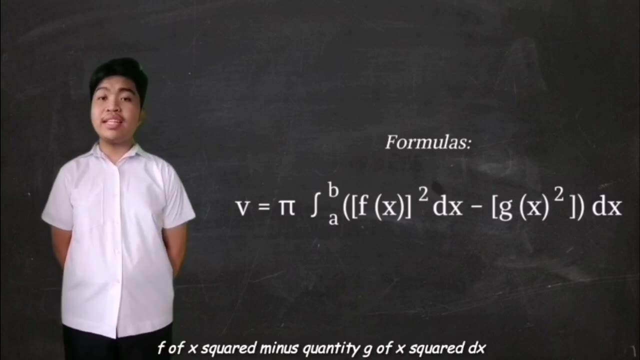 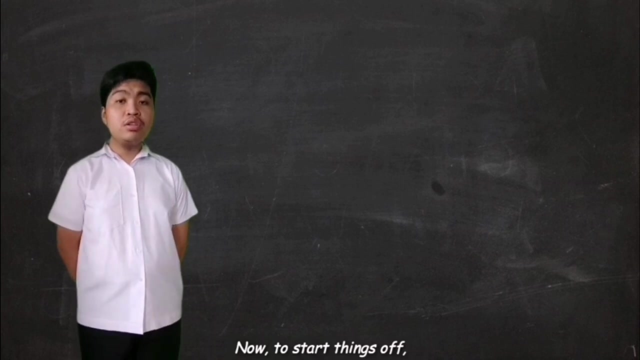 the volume of a solid figure using the Washer method. Calculate the volume of a solid figure using the Washer method Now, under the, As they say, it tries to eliminate this problemたい. So f of x is the x, g of x is the x. squared, a will be 0, and b is 1..